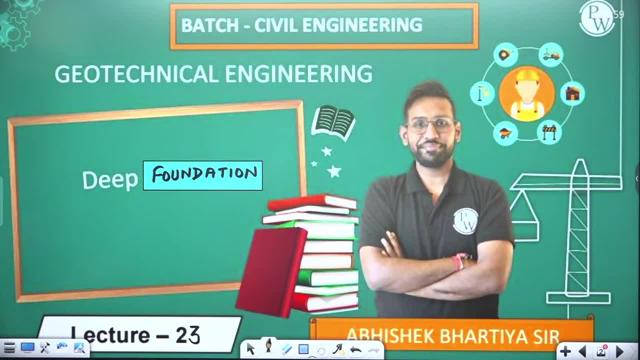 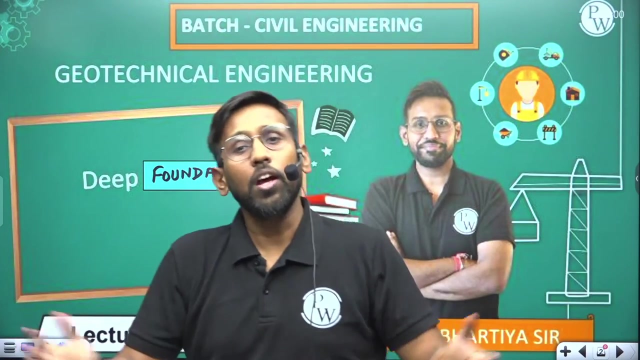 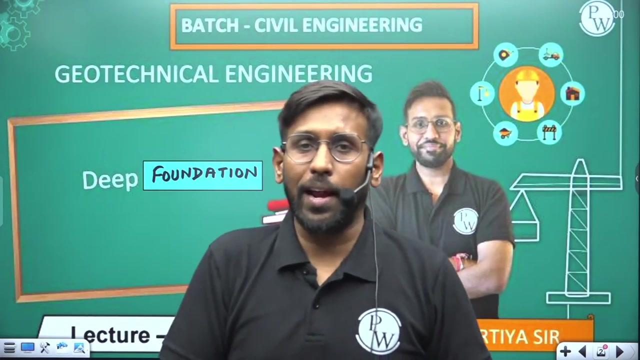 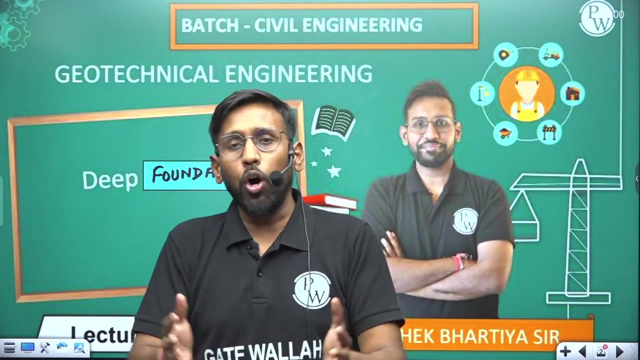 Hello to all, So very good evening everyone. Welcome everyone to your own YouTube channel: Gatewala, MEC and HC. My name is Abhishek Bhartiya Gate, all in a rank 136, and I welcome every one of you on the behalf of team Drona And my friends. we have almost finished, geotechnical. 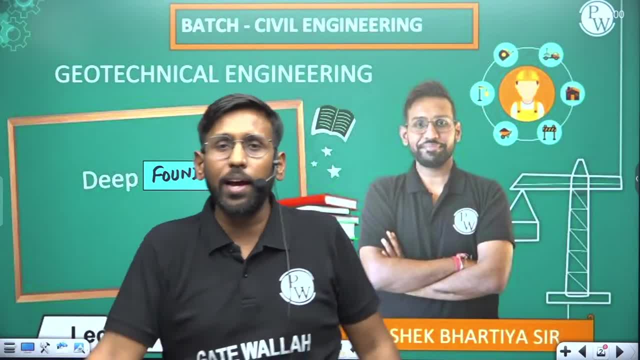 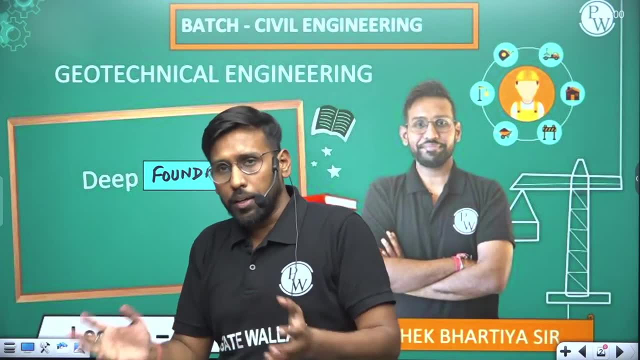 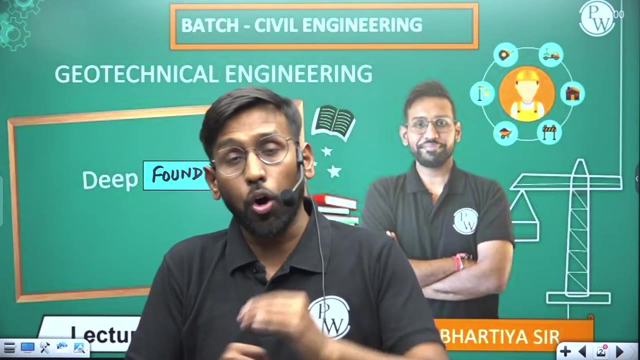 engineering. There are two lectures left, one today and the other tomorrow, And in these lectures we will cover pile, foundation and soil stabilization. That means we will very well achieve 13 numbers of geotech, Yes or no? And, my friends, I would like to know from. 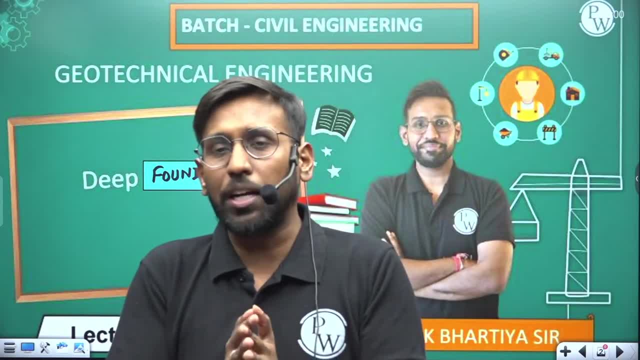 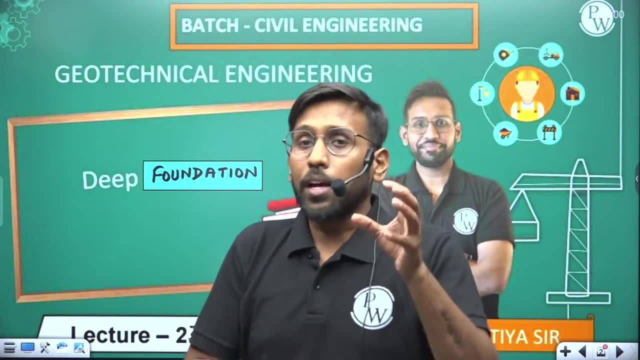 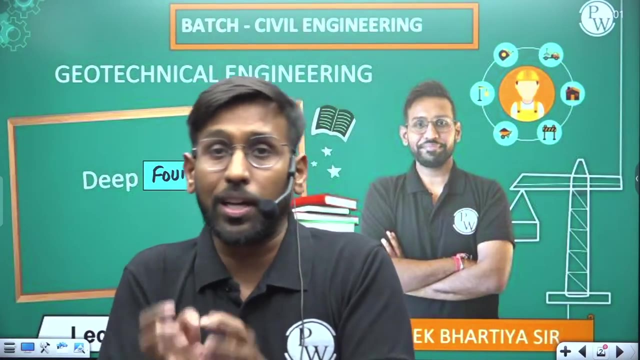 you that, whether you have covered the shallow foundation engineering, whether your questions were made well, The questions we asked you yesterday, that when you go and apply for PYQ, then the point I said that there is a formula base direct, you have to ask a lot of things. 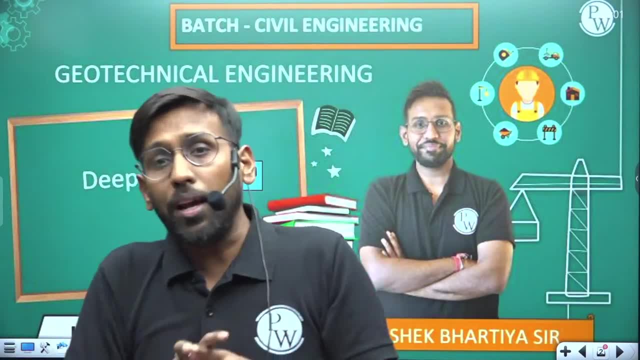 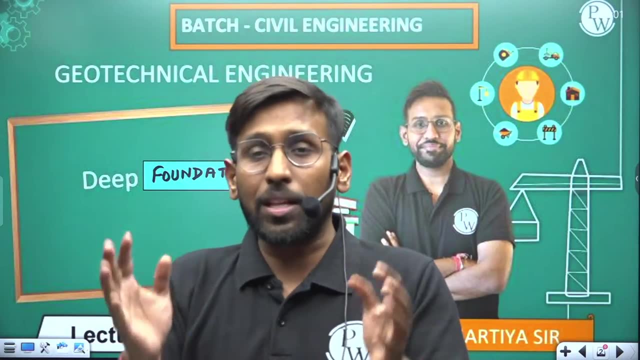 you have to apply there. Did you get all those things? If you get it, then we will make all the questions. If you have attended your proper classes, then, my friend, I hope you have done this. the questions will be made from you. then quickly make the chat session. 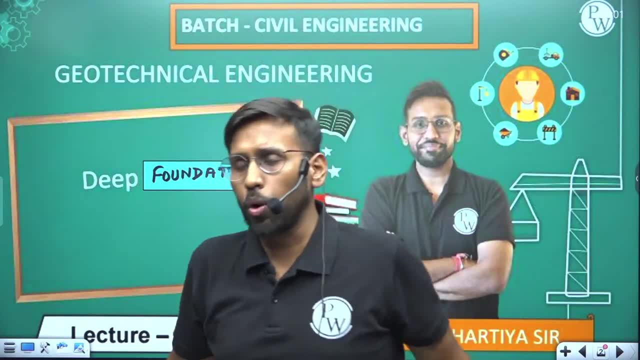 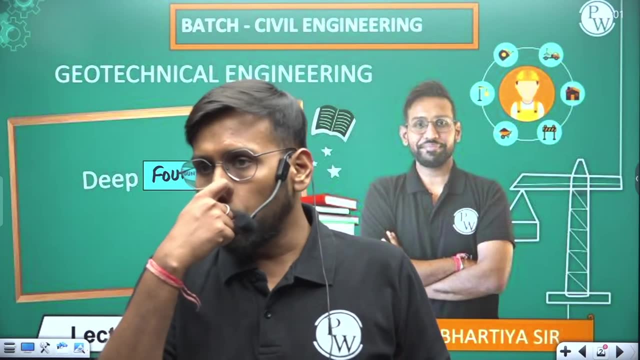 red and we are going to start the session. We are going to start the session. DPP has gone, son. before the last lecture: right, Come on. okay, we will see, we will see. okay, let's go, let's go. 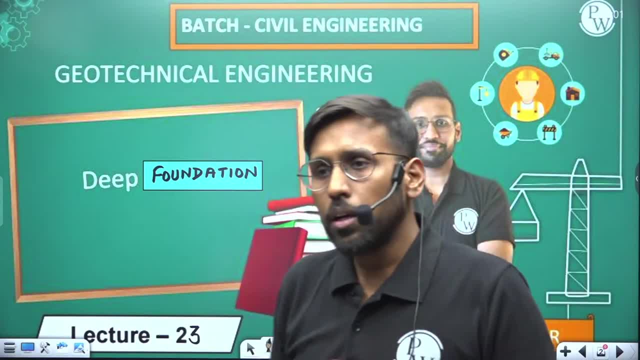 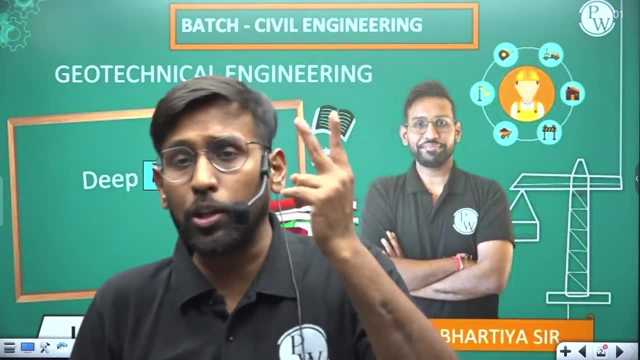 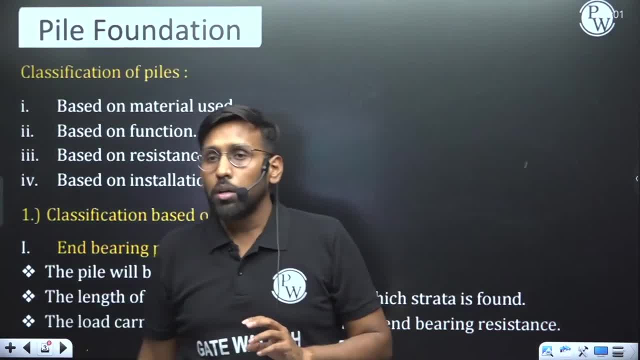 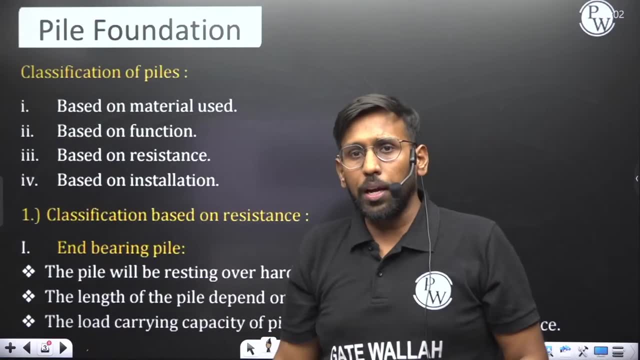 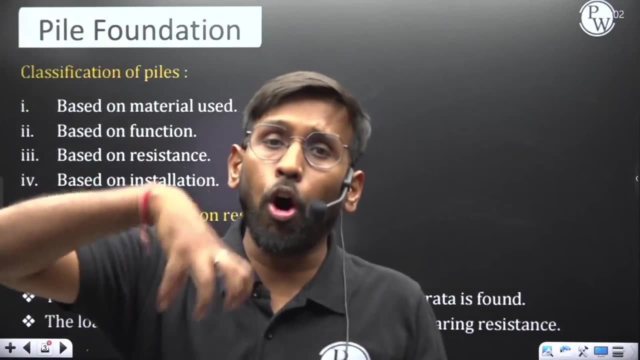 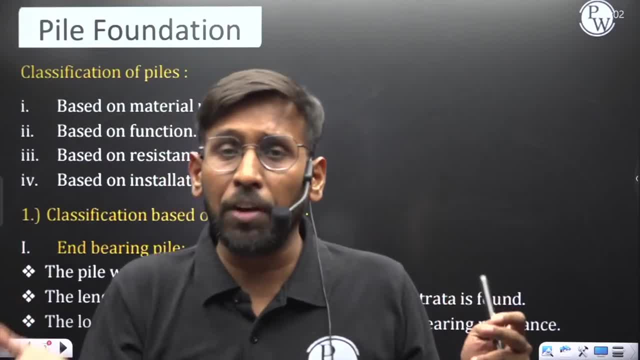 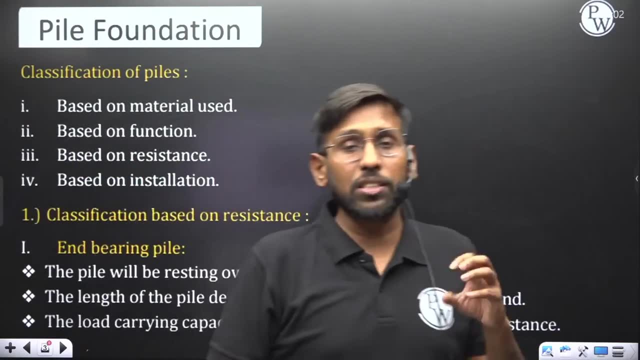 is high, this Vapcker. what do you say? what do you say faced situation? you are just doing it itself. So that player is classified in Faiz, The shaft has been hardest, which has been classified only at the four ways. So the first thing we are going to talk about is that, when we will talk, we will talk about things before we go. Okay, first of all, we will talk about clearing out the hills, and after that it will have a full year, and after that it will have a full year, and we all have to die. we have to cooperate, we have to месте feed function. we all shoulders only. So if you do, 4. 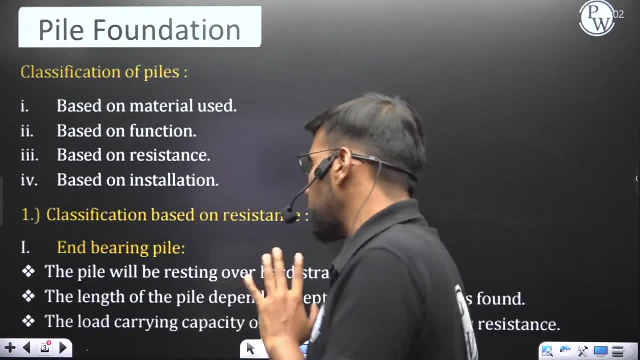 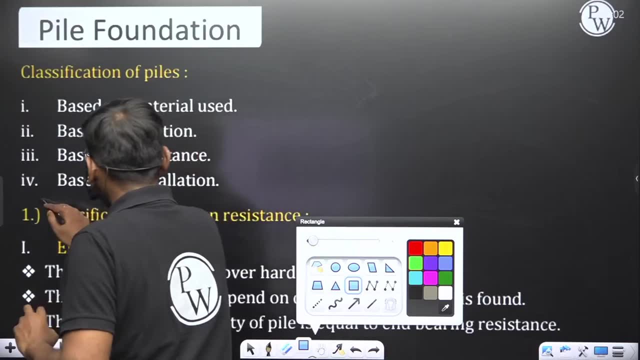 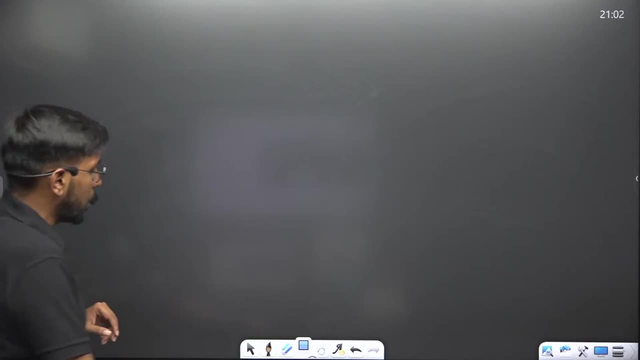 He gave chart a ricos, a classify kia gaya. Hey, what's up? Say palium, job. What can I tell you? Hey, The first point, job. What can I tell you? that is classification Based on resistance. Sunabaat could answer some. look, sub-team, I've got a kick target. So much me, I jayega. 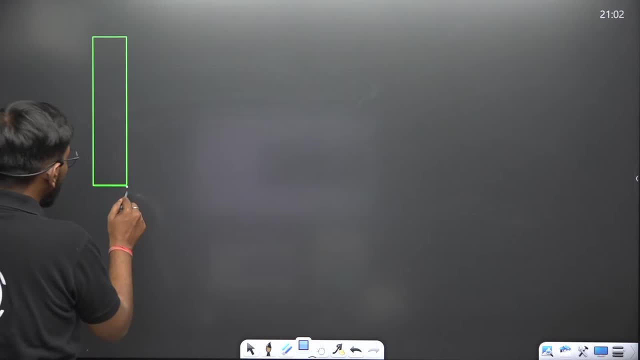 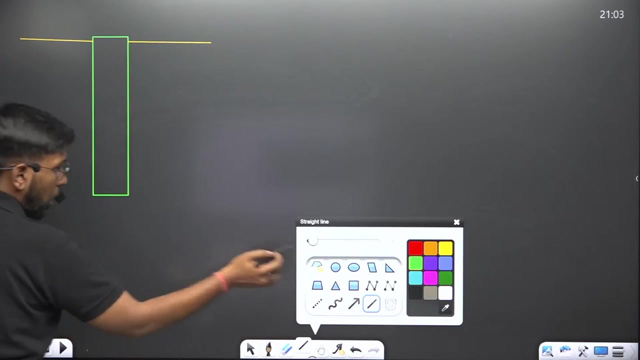 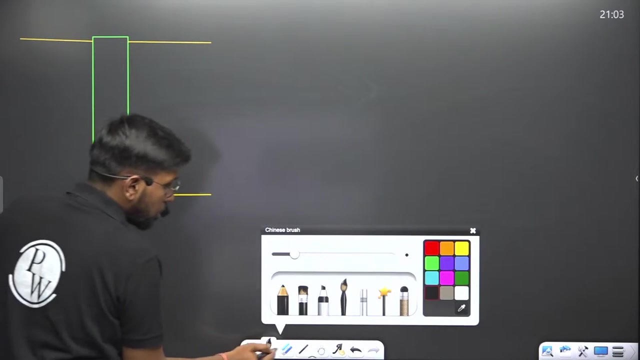 So classification based on resistance of some jockey. Yeah, I've got pilot Anna. This is a pile, This is a pile okay. and This pile is resting over a hard strata. this pile is resting over a hard strata. Here's a pilot risk. is picker Rahe here? Yes, Karai, over a hard strata. 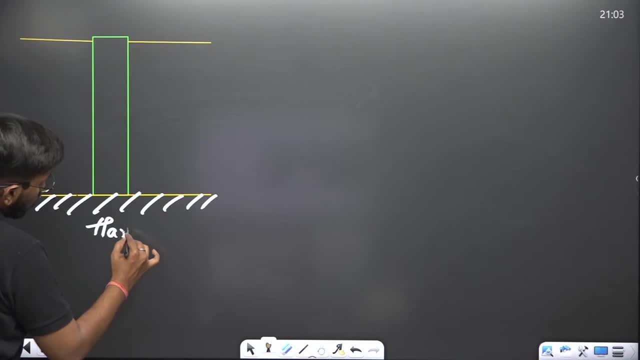 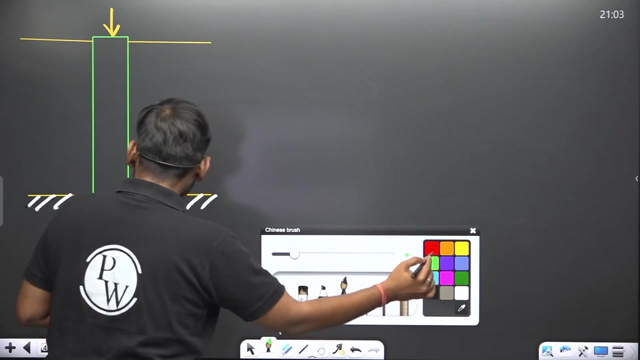 He gave, which can be, are the load. It is resting over hard strata. He came in those. It is resting over the hard strata Up agar Koi load laga rahe. ho You applying the any load for your resistance? mill a vala hai, What resistance. 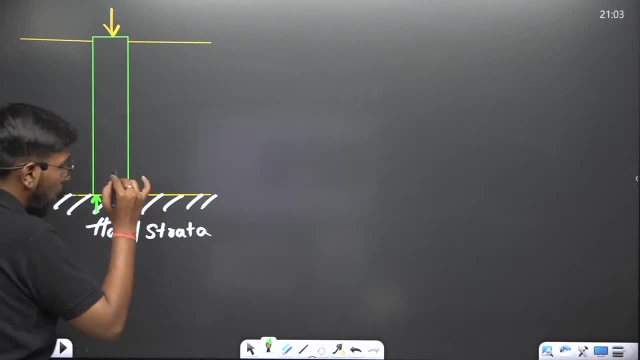 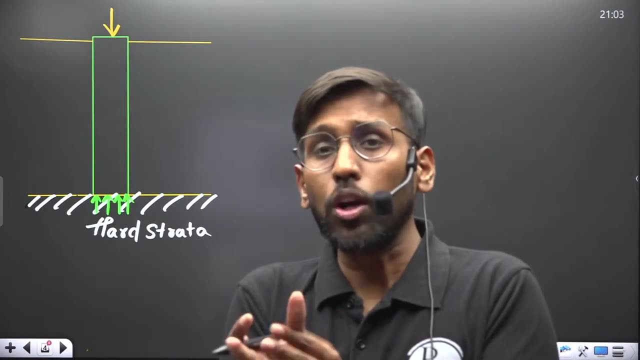 Kaha se mele ga. that resistance you are going to observed only from the bottom, That resistance is going to be observed only from the bottom. He can major your resource over. major to resistance. Oh god, What bottom? say. oh god, Yeah. visualize car pario. 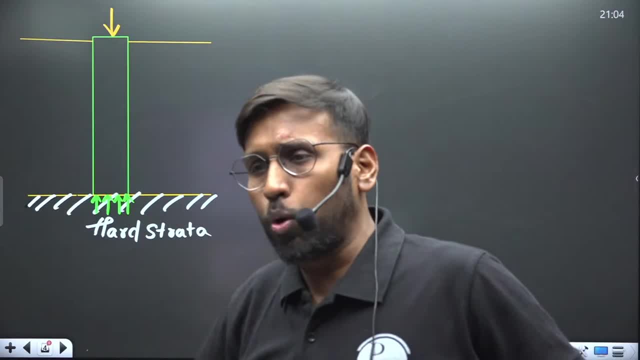 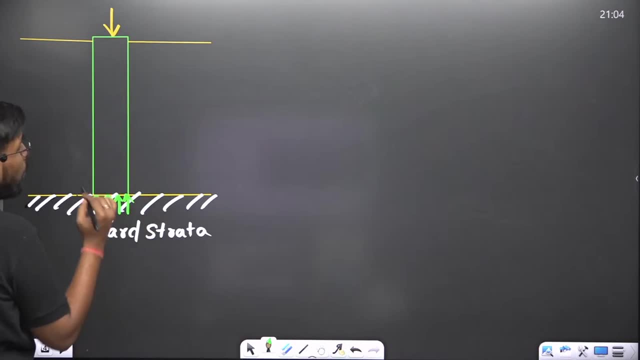 Agar apne previous class attorney care Koi baad nahi, samajh me a jayega, Don't worry, They go happen. So the rest is observed only from the bottom. or escom. kya boat a end bearing resistance There? both a my dose QEB, QEB. Kya matlabh hai. 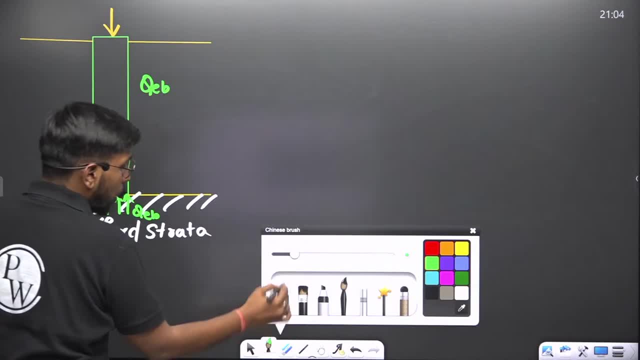 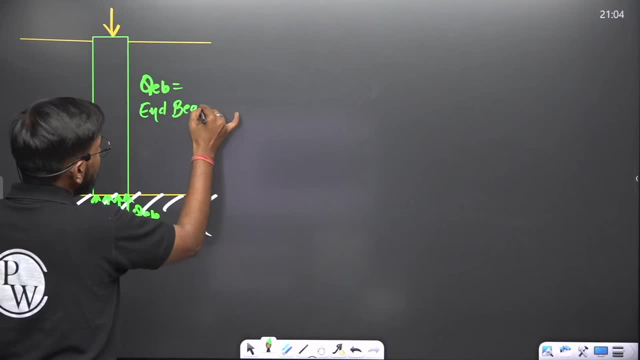 QEB Kya Matlabh Hai. QEB Ka Matlabh Hai End Bearing resistance. QEB Ka Matlabh Hai and bearing resistance. so eska jo load carrying capacity hai wo karne hai? Where is it coming from? From the bottom? So what we are writing is that the ultimate load carrying capacity is nothing but what is coming from the end bearing. 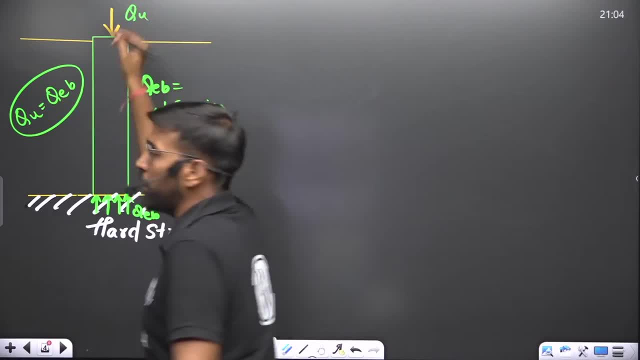 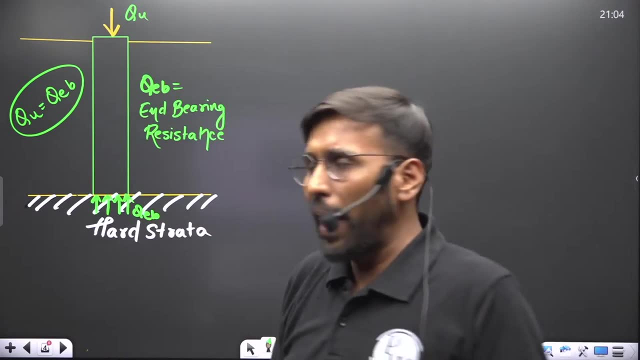 Can you say that The ultimate load carrying capacity is nothing but the resistance observed from the bottom. So we are writing the Q ultimate as simple as QEB. So what do we call such a pile? We refer such a pile as an end bearing pile. 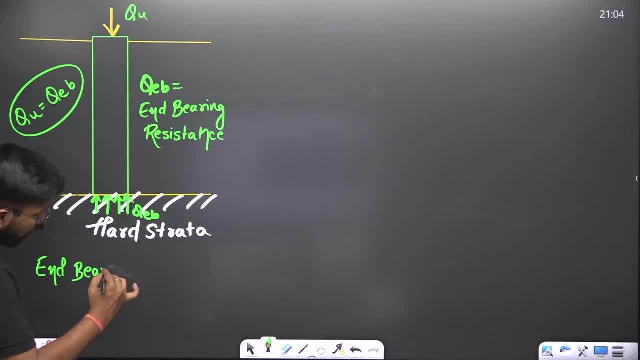 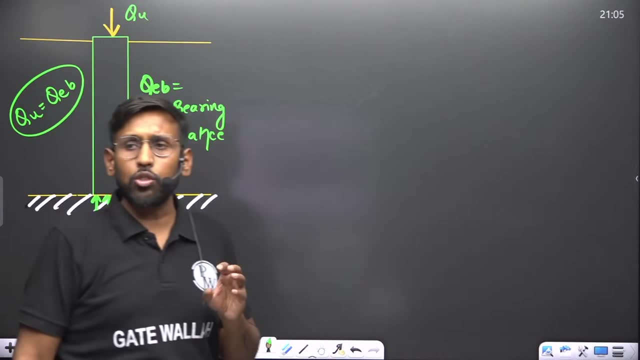 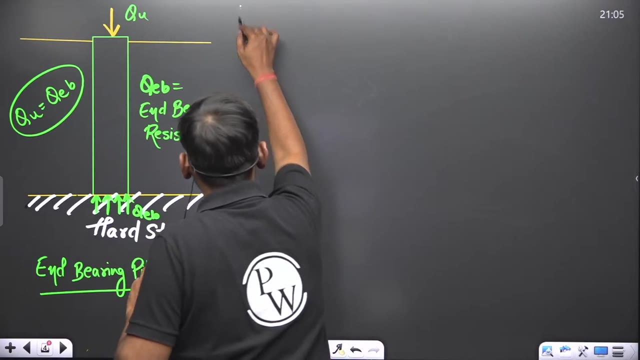 Why we refer it as an end bearing pile. Why we refer it as an end bearing pile? The resistance is observed only from the bottom. So what you observed for this end bearing pile is called operating range wise based on resistance. Now let's classify. 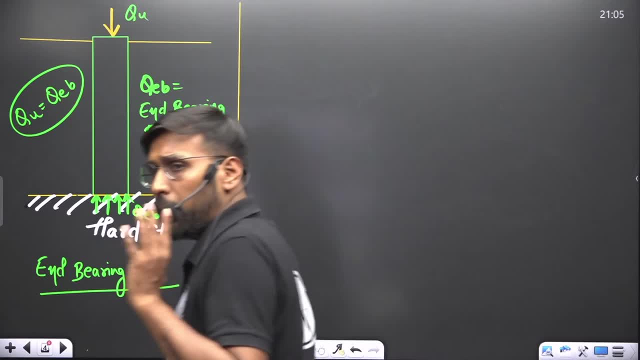 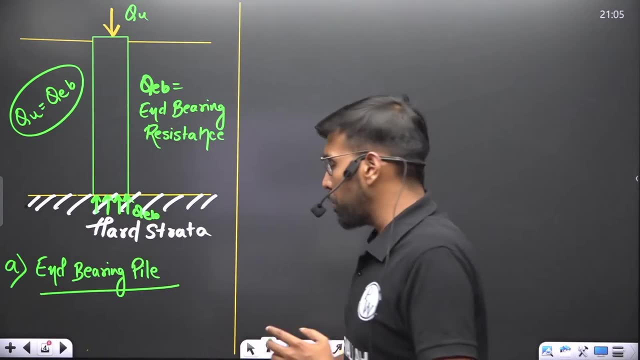 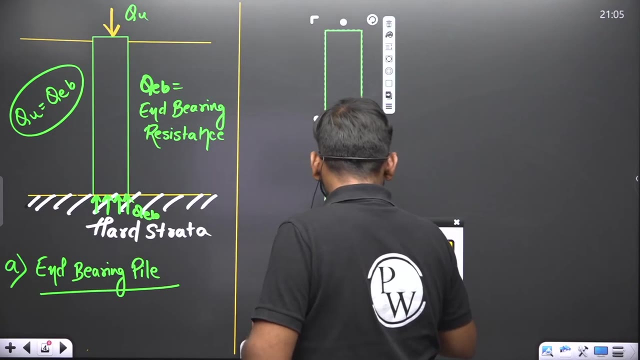 In the previous classification. what you got is the end bearing pile. First classification is that of the end bearing pile. is the end bearing pile. sorry, agla bottom curry, a agla bottom curry, a big obey. the pile length is nearly 10 meter to 20 meter, or quite support. 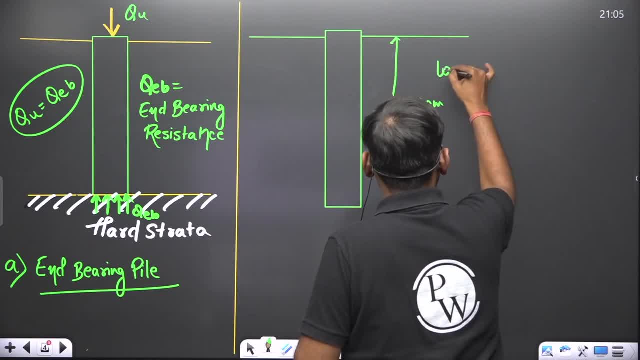 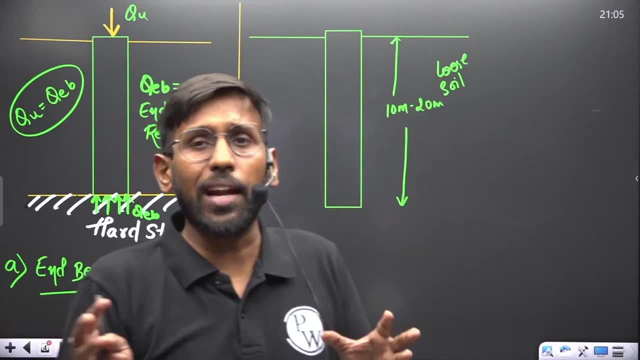 naia a kiss mail. loose soil may. it is in the loose soil as a solid present, a loose soil presenter. so I got loose soil me present at the resistance on a book house. I got your resistance me lega, your resistance me lega. who can't see me? 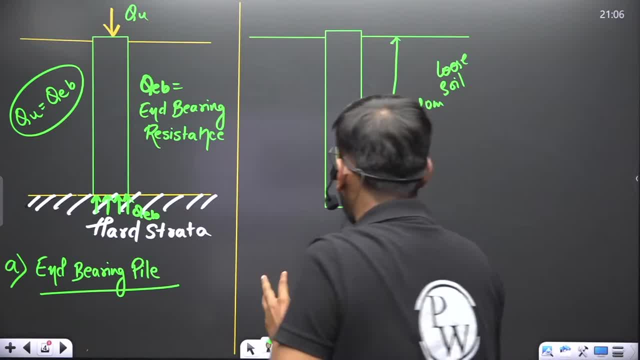 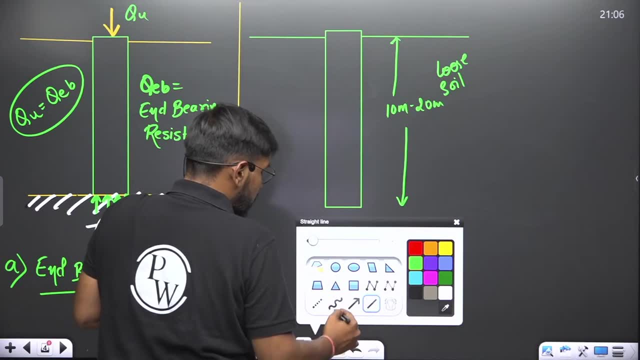 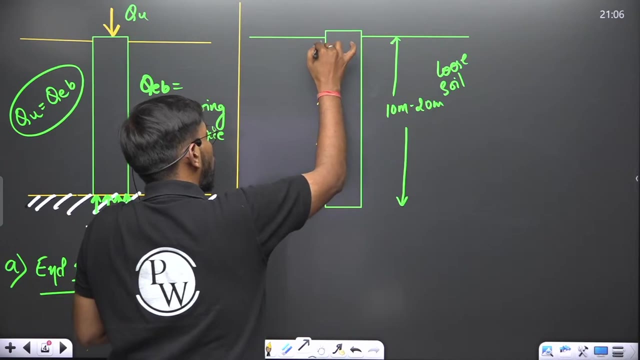 lega. but okay, well, yeah, your resistance up, Camilla. hey, that resistance loose. while the resistance will be observed only from the sites up, could your resistance me lega da? hey, poor instance of kukasa me lega da. resistance observed only from the sites. the resistance do bottom. the resistance over. Bob, come over, he get to major your. 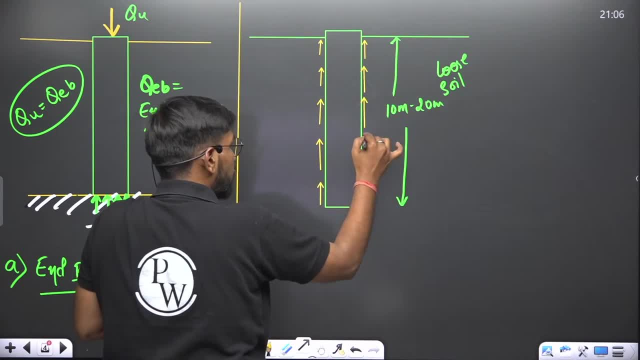 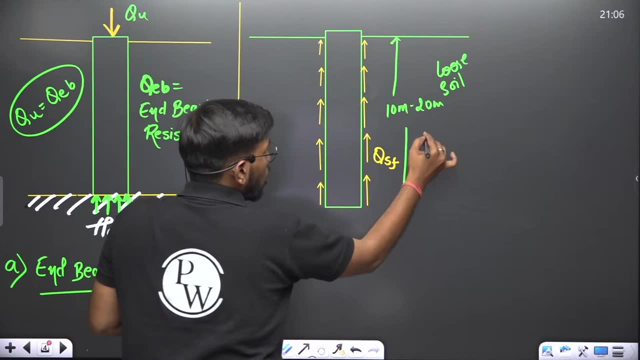 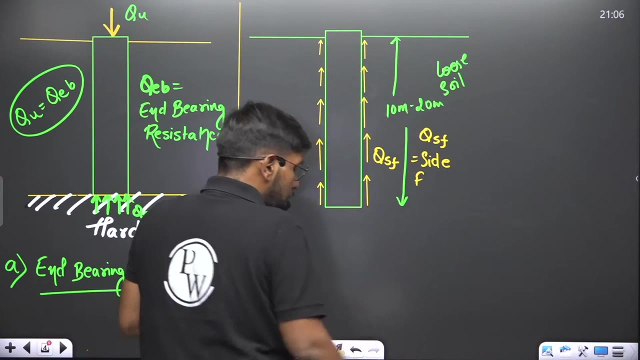 dog combination over ke skoga. Bob con friction kauga, he get the scum will take you as a Q side friction. you have some of love bride. fictional resistance, what detail upon a while a key cheese, but y'all be bottom a character, the Y'all foundation of the formula Ratna. did you see the formula Ratna in shallow foundation? 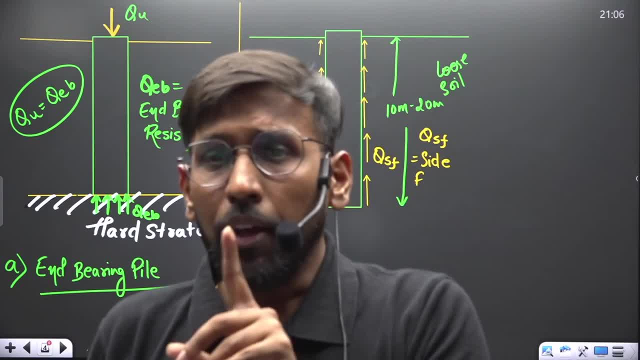 did you see the formula Ratna? did you see the formula Ratna? did you see the formula Ratna? in shallow foundation, Ratna brought on a yobico of Latina Nepal a go. you don't have to mark up any Ratna here. 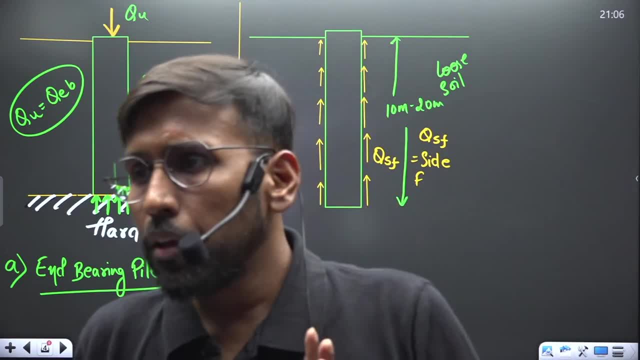 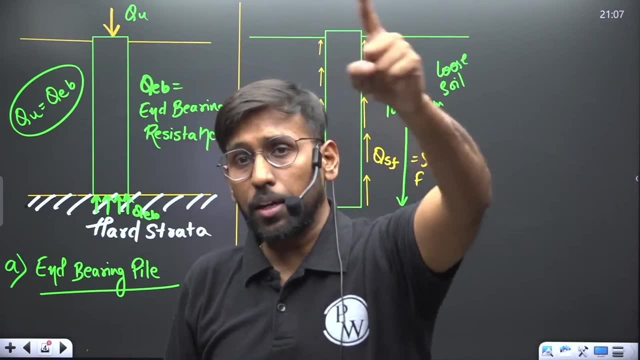 you don't have to mark up any formula yet here. Okay, Here there is no formula to be written. I will set everything here, Promise, Promise. I will set the whole formula here. It's my promise, Okay, Clear. 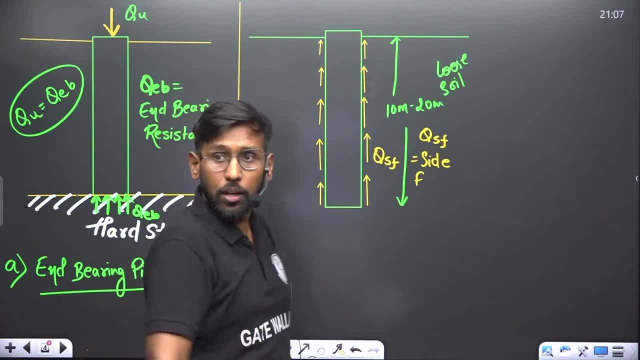 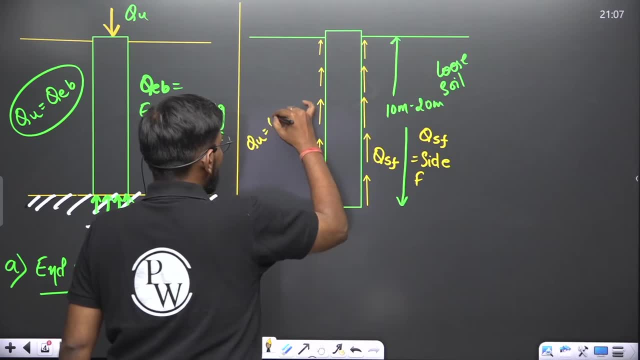 Yes, we will consider the bottom as neglect. We will consider the bottom as neglect. And what are you writing? Only side, Exactly. So here, what happened to my Q? ultimate? That is nothing but Q side friction. So in a loose soil when 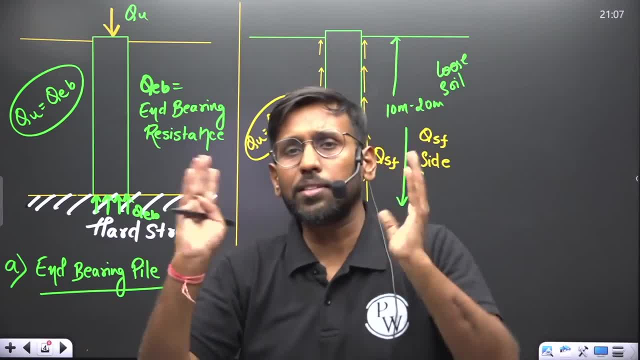 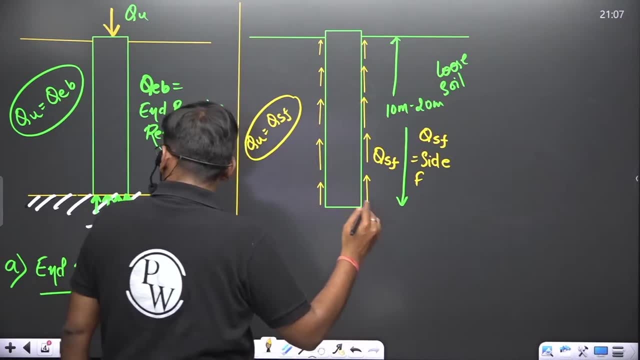 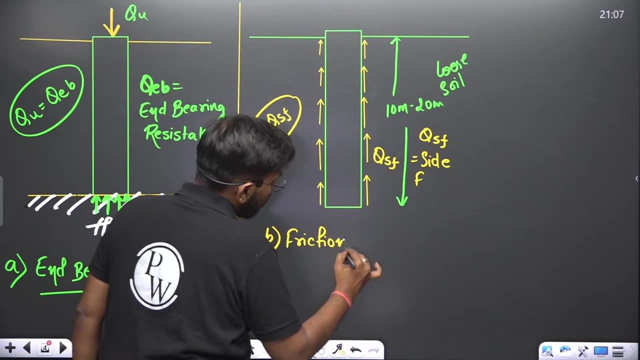 no one is resting on your bottom. where do you get all the resistance? That resistance is observed from the sides. That resistance is observed from the sides. Okay, So what is this pile called? This pile is called frictional pile, Friction pile. 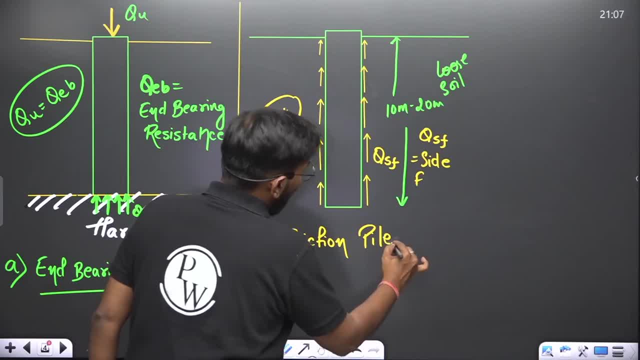 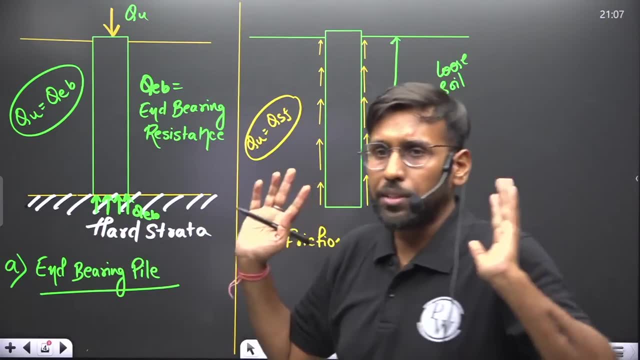 Is it clear? What is the name of this pile? We refer the pile as a friction pile. The resistance is observed only from the sides. The resistance is observed only from the sides. Is the point clear? Where do we get the resistance? 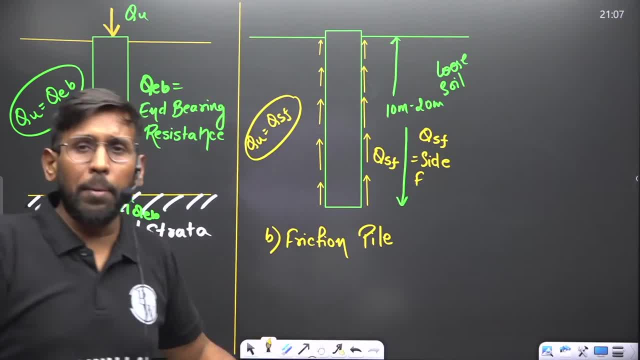 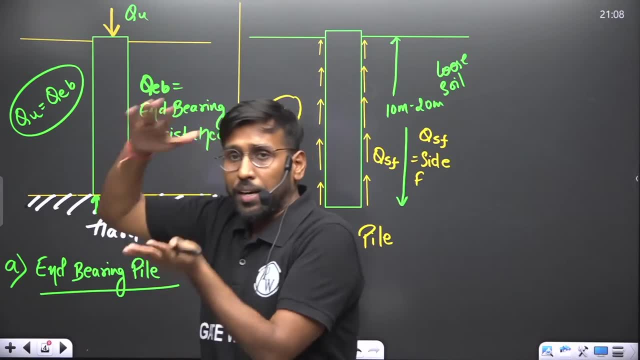 The resistance is observed only from the sides. Where do we get the resistance in the end, bearing From the bottom? In the end bearing the pile is resting over the hard strata. It is resting, It is sitting on it. So where do we get all the resistance? 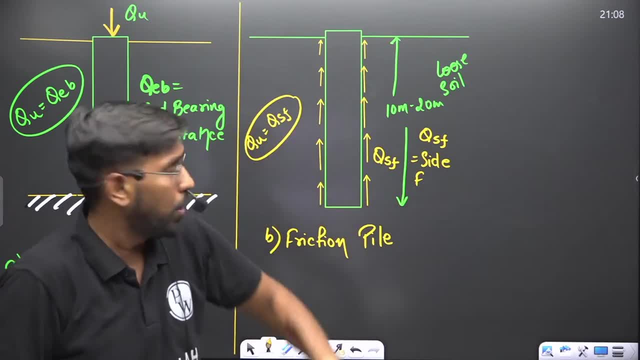 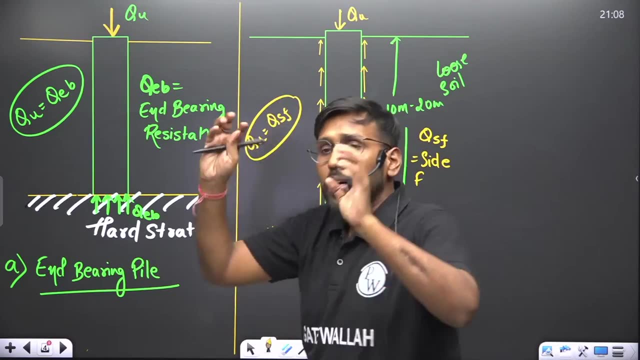 From the hard strata. Okay, There is friction, but it is negligible. Similarly when we talk about the friction pile. so, whatever load you are applying, where do you get the major resistance? The major resistance is observed from the sides. 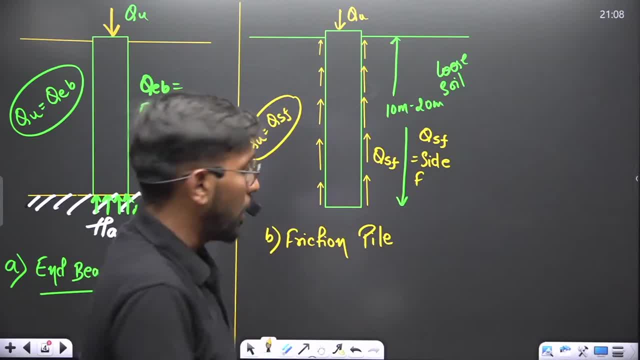 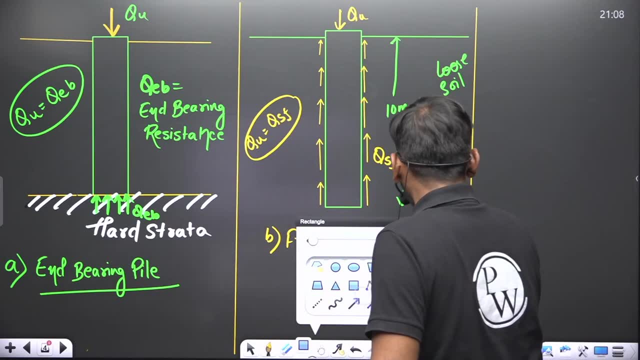 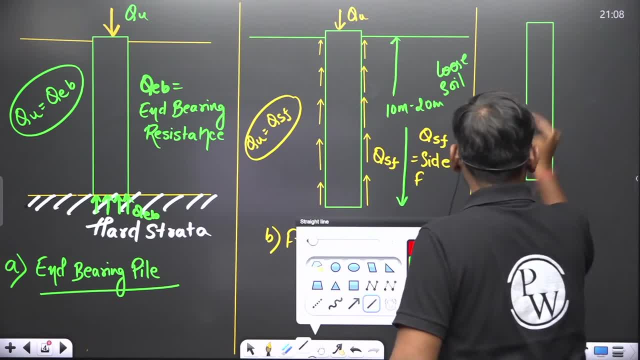 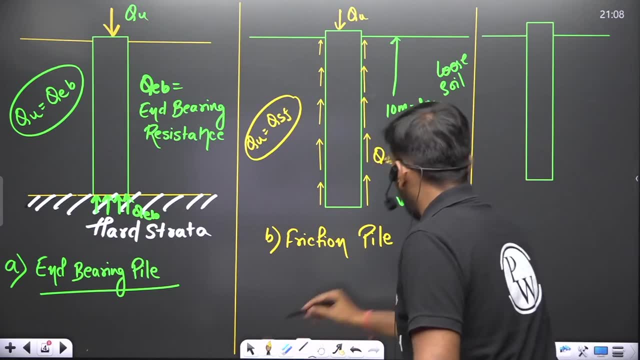 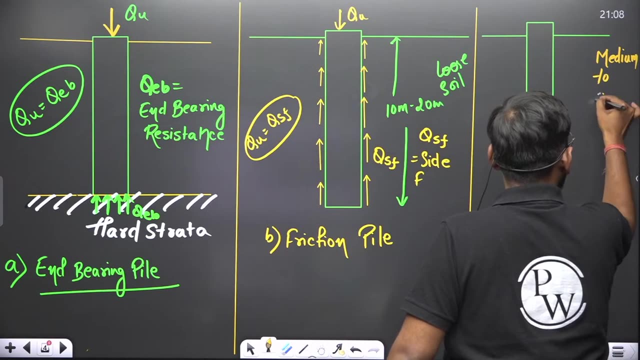 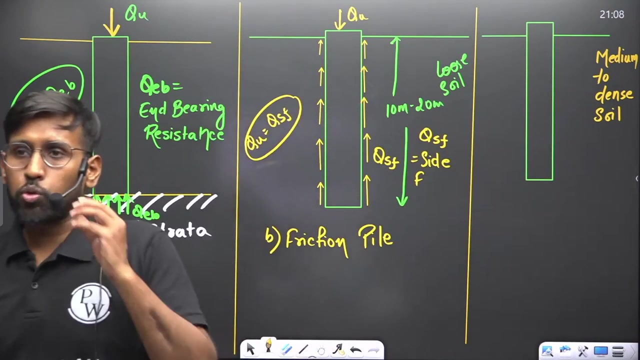 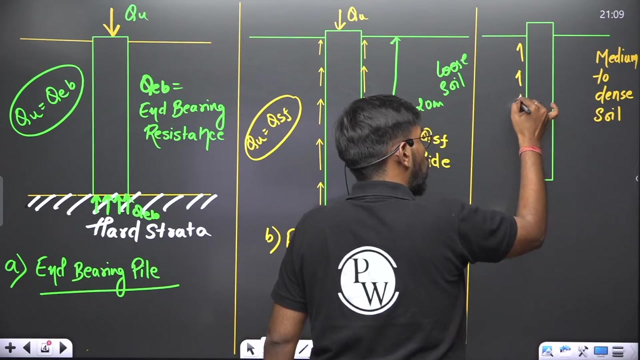 Now it will be about both. Now it will be about both. Now, let us say: the pile is resting in medium to dense soil, Medium to dense soil, The soil is resting in the medium to dense soil. Now, here what you will see: that the resistance is observed not only from the sides. 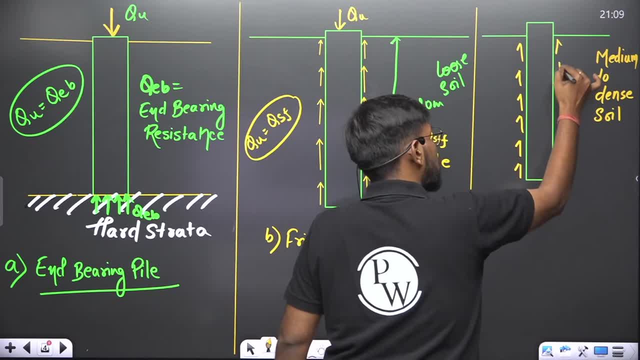 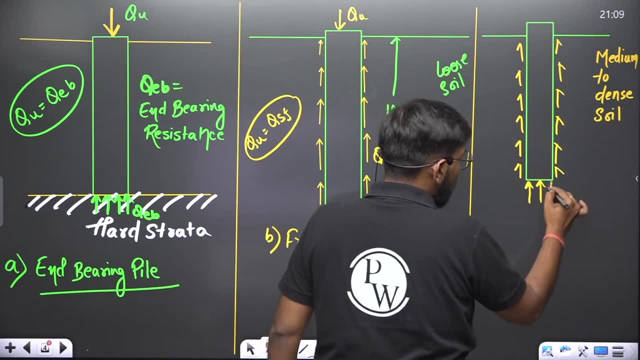 The resistance is observed not only from the sides, but also from the bottom. That means end bearing will be there. What else will we get? Side friction will be there. That means here QRD is there. That means here QRD is there. 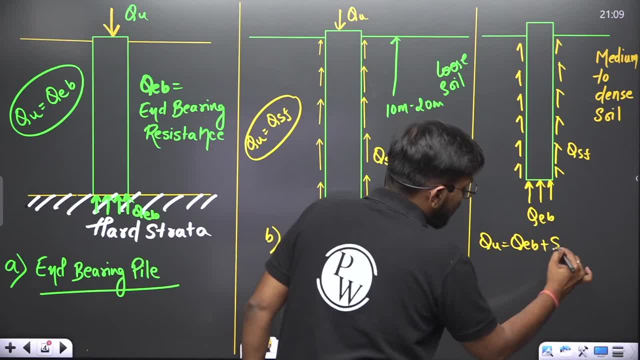 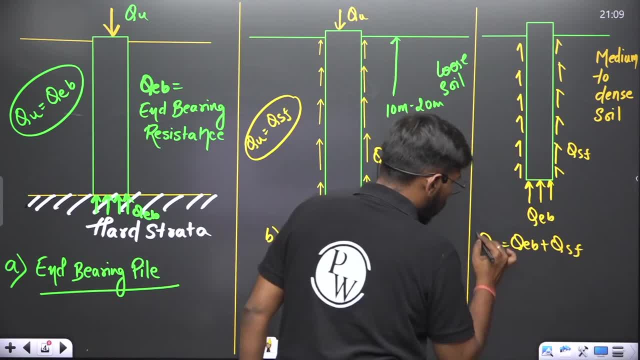 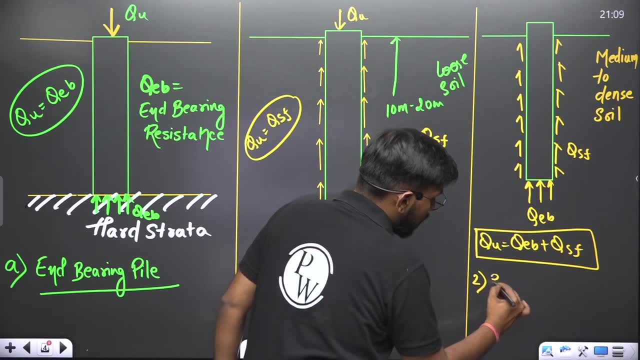 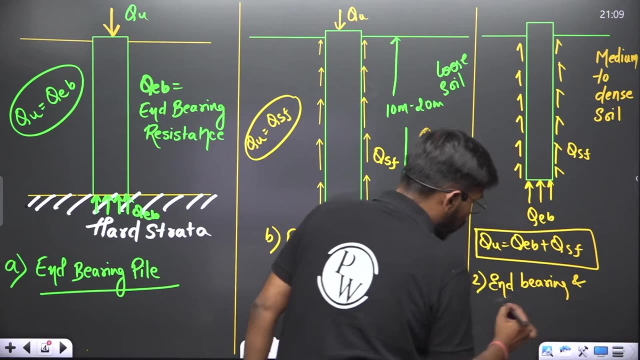 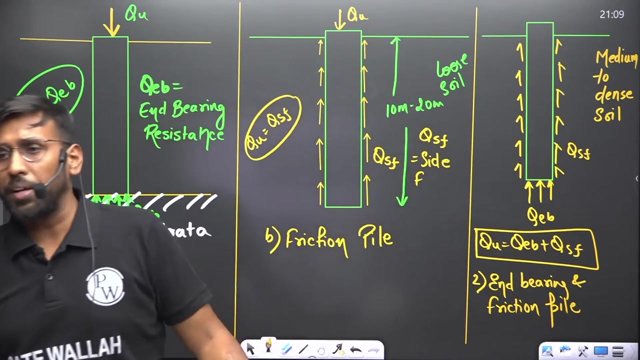 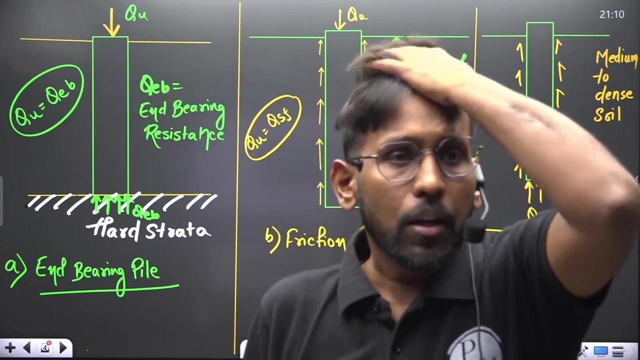 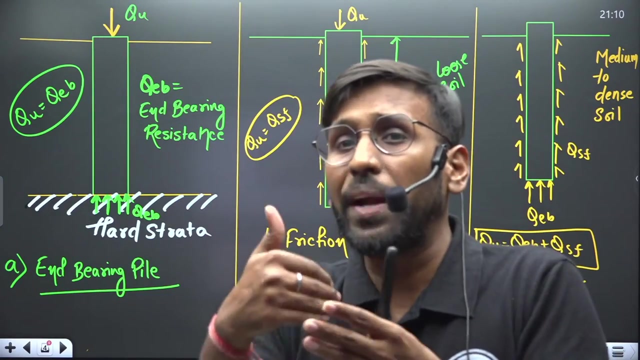 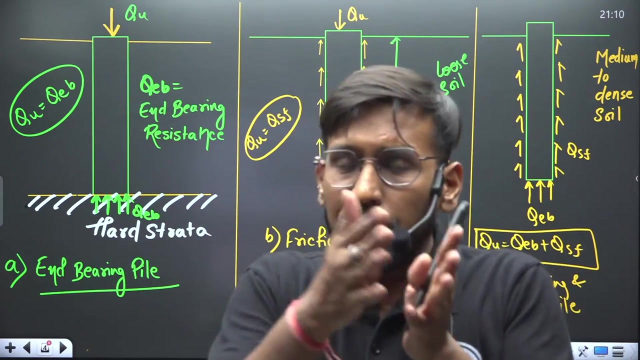 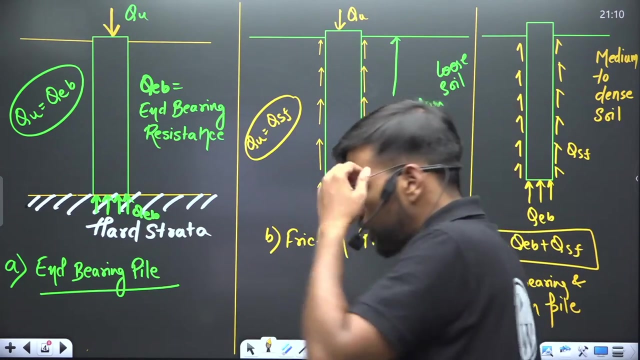 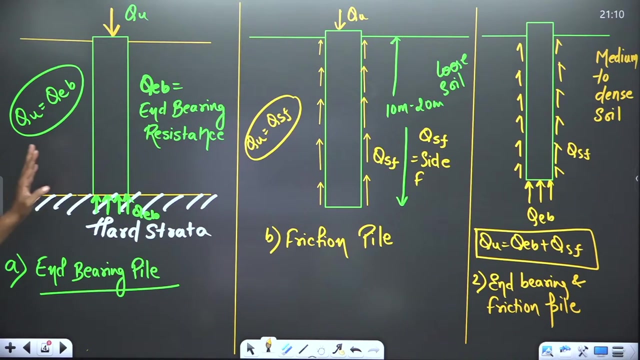 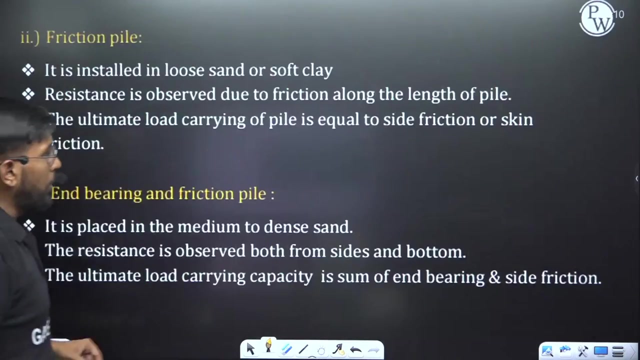 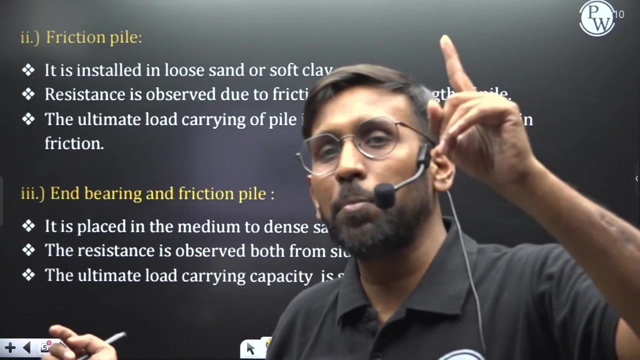 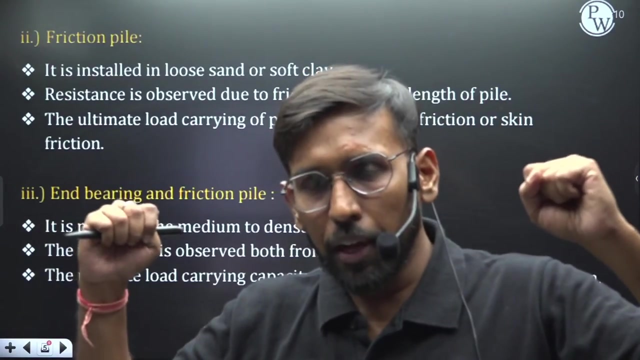 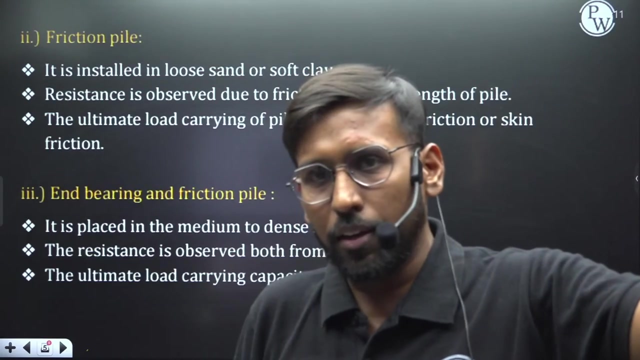 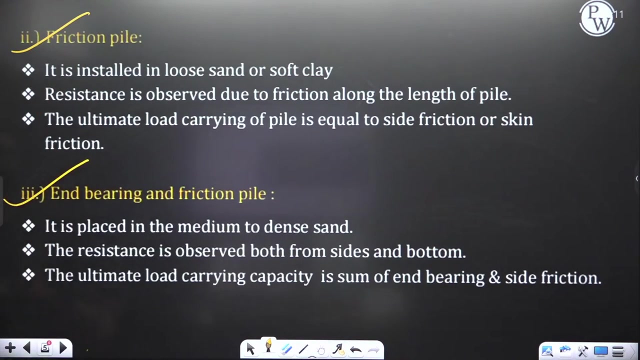 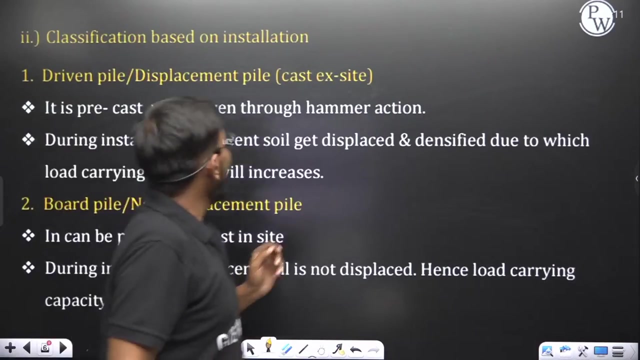 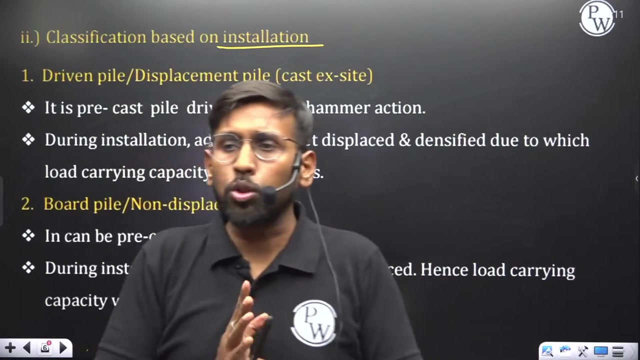 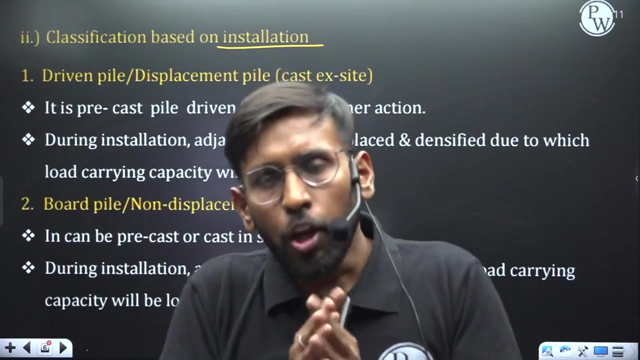 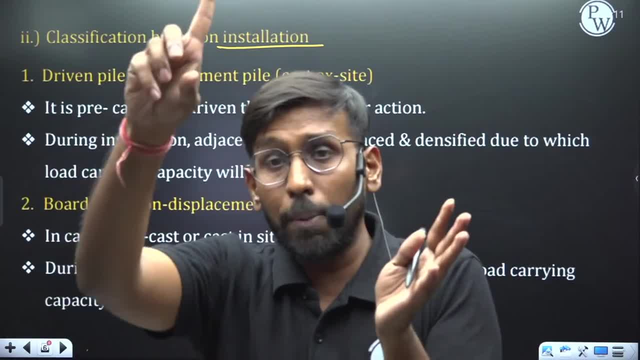 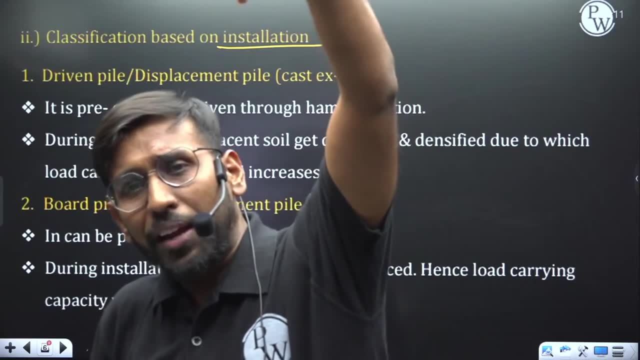 aapko field mein construct hota hai. sunna baat ko dhyan. se toh jo pile factory se banke aate hai, toh humko kya karna padega unko generally. hum kya karte drive karte hain hum generally. 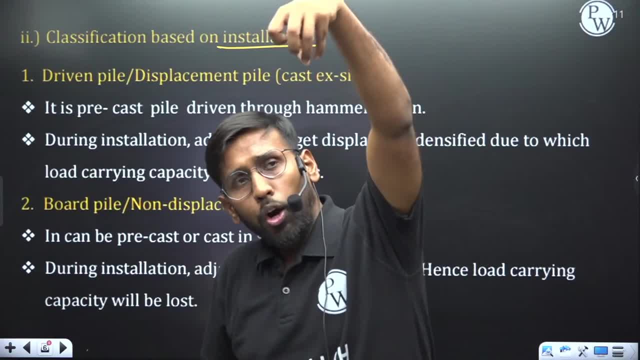 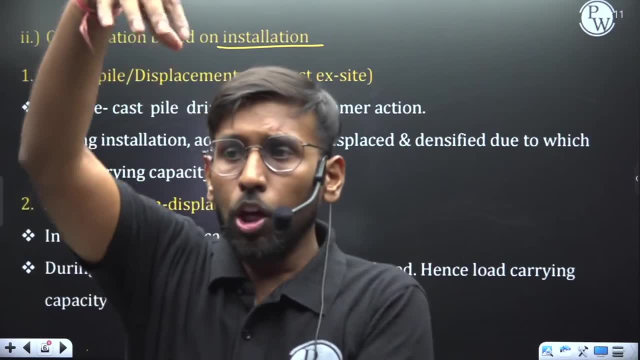 kya karte hai? we use to drive the pile inside, aur jo bhi load lagate uspe, lagate hain, toh bhi jo driven pile hota hai, hum abhi baat kare displacement pile ka. toh maal lo ye mera. 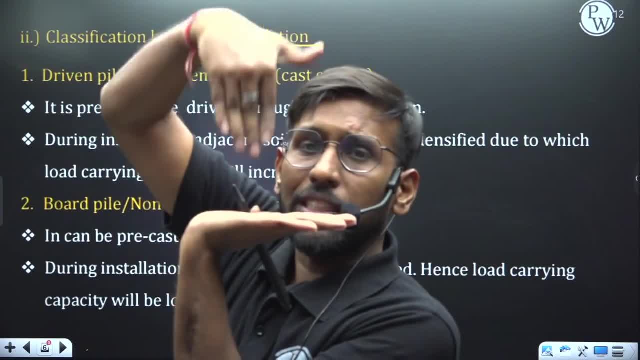 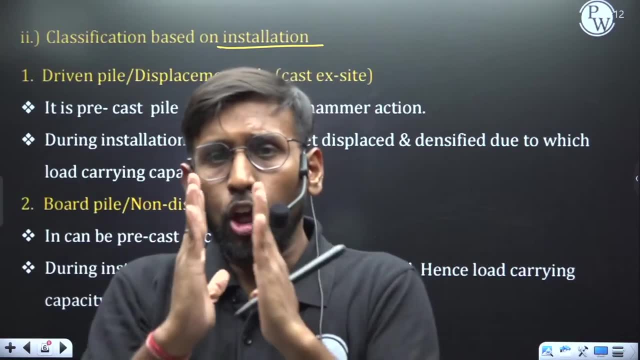 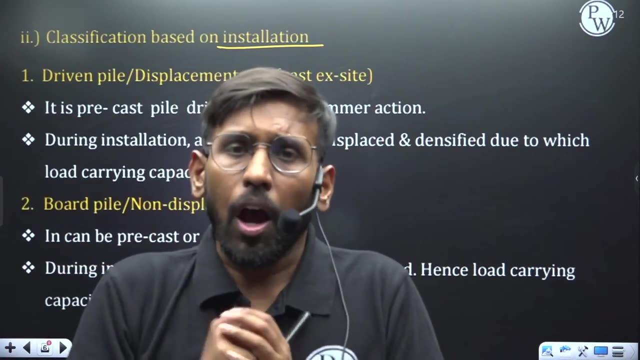 surface hai. hai na, and this is my pile. i apply the load so that the pile goes inside. toh jab pile niche jaega, toh adjacent soil ko kya karega, displace kar raha hoga. adjacent soil ko kya kar raha hoga, displace kar raha hoga. hum generally kaise soil ke liye pile. 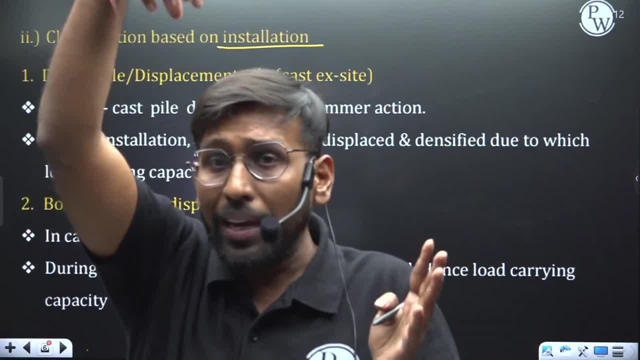 construct karein ke for the loose soil, toh agar loose soil ke liye pile drive kar raha hai, toh kya drive karein ke for the loose soil, toh agar loose soil ke liye pile drive kar raha hoga. displace kar raha hain, toh agar loose soil, toh agar loose soil ke liye pile. 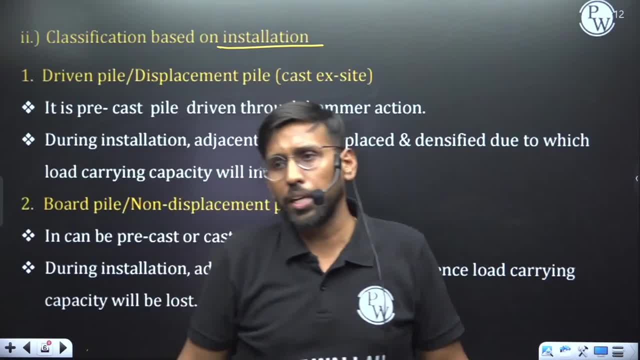 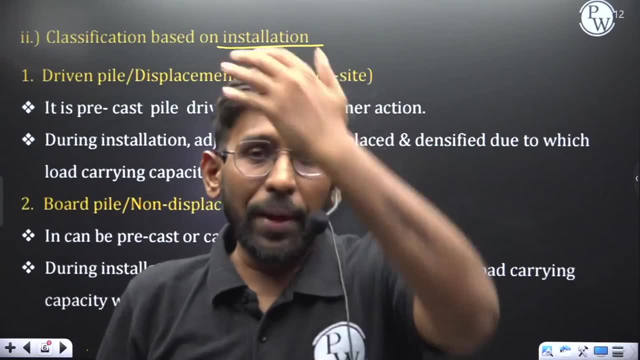 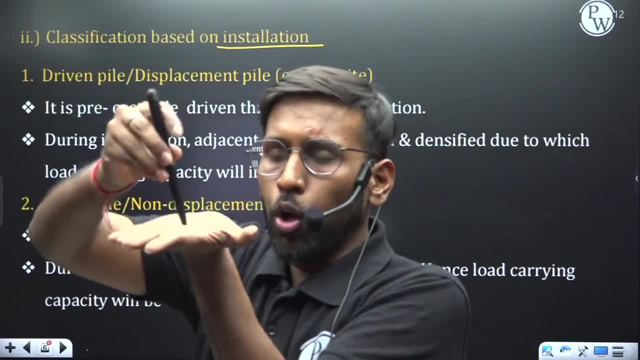 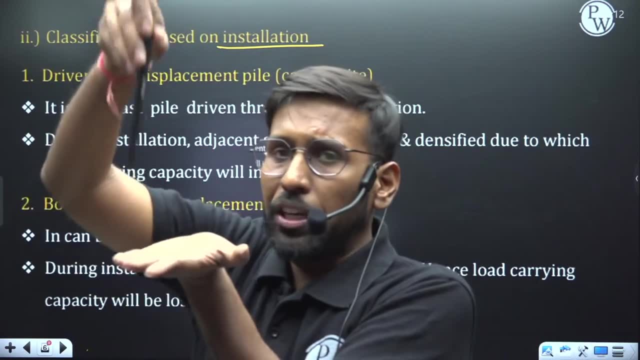 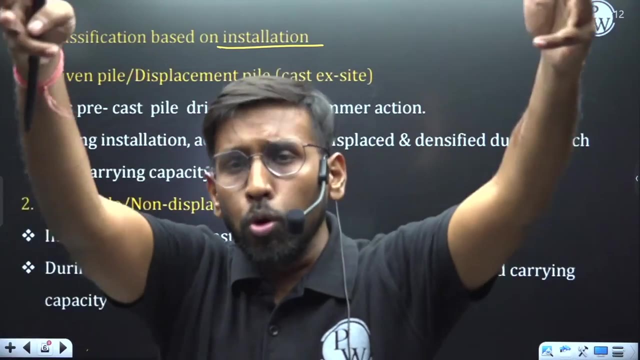 dost, there is a pile. there is a pile jo aapke surface pe hai. you apply the load and you drive it in side. the soil theek hai. toh iss driven ke karan aapka jo soil hai, jisme ye penetrate kar raha hai, wo side ghasa kar raha hoga, aur generally kyunki hum loose soil karein. 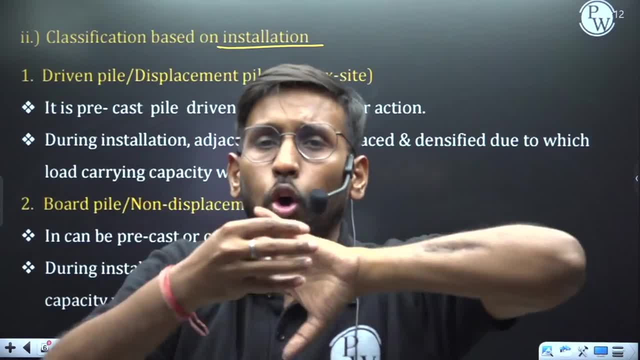 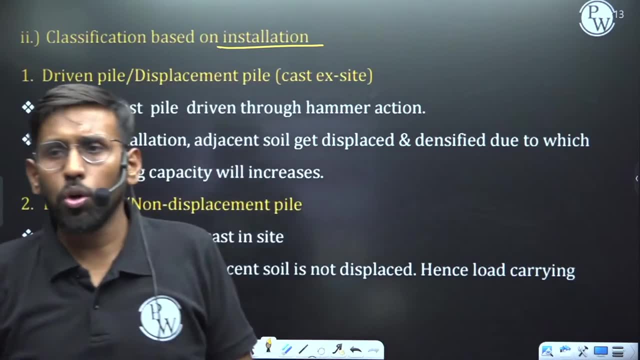 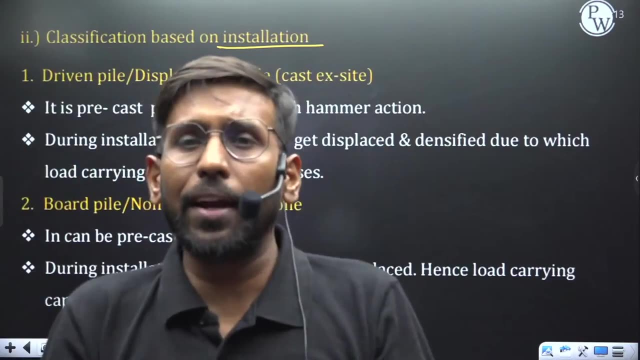 So in the case of loose soil, you don't think that the adjacent soil is going to be further densified. Hey, say yes or no. So here the load carrying capacity is good. But if this is the same with bored piles, Suppose you made a hole, did concreting, made a pile there. 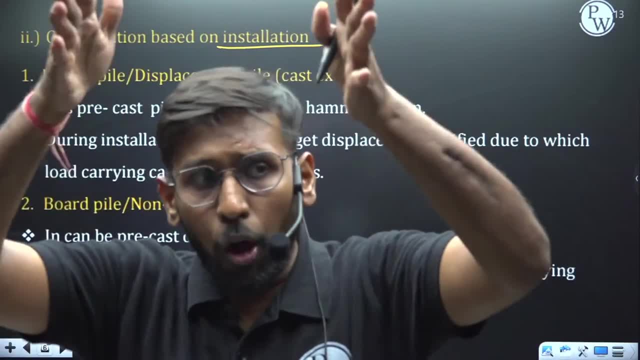 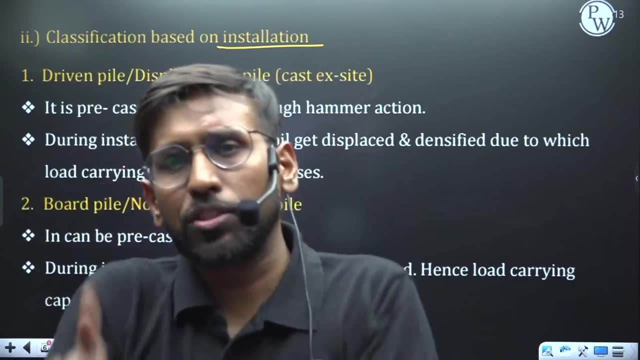 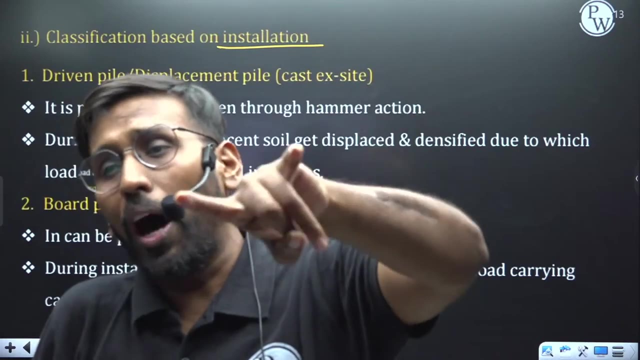 So you didn't drive the pile You have already constructed there. And what did you do? by taking it, By boring it, you have constructed the pile there. So in that situation, your loose soil is there, but it is not dense. And if it is not dense, then what happened to the load carrying capacity? 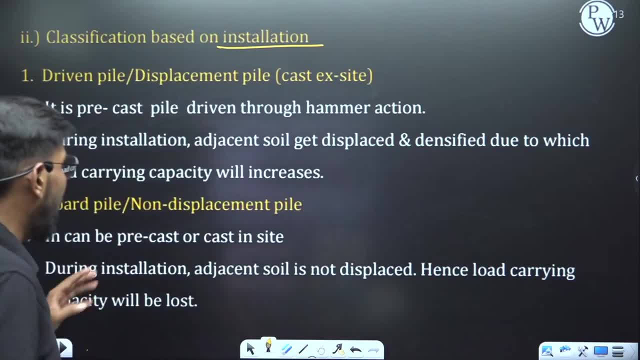 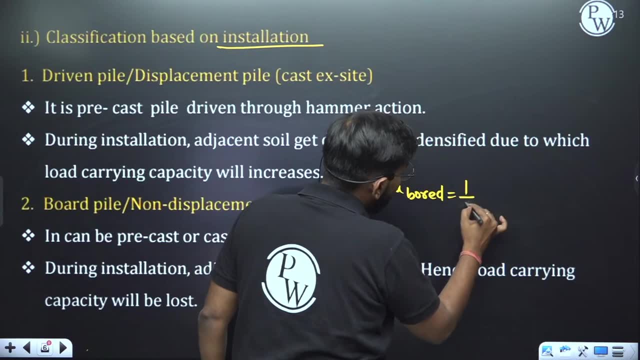 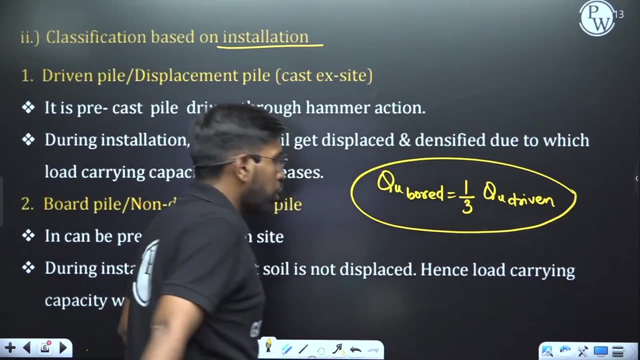 Did it decrease? Say yes. So here what we generally write: Q ultimate for bored piles is nearly one third of Q. ultimate for driven piles. Is it clear to everyone? Say yes, my friend. Q ultimate for bored piles is nearly one third of Q. ultimate for driven piles. 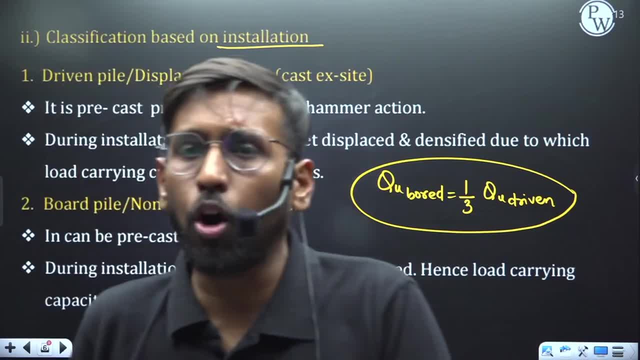 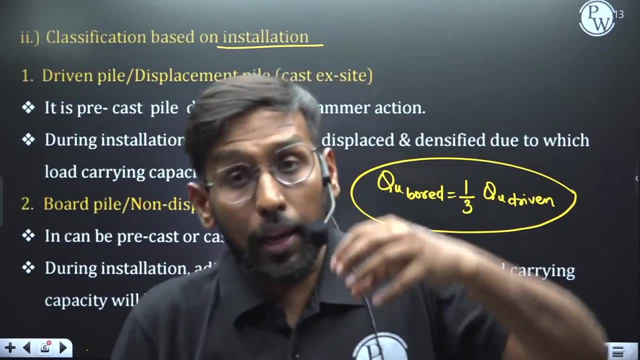 So it was said that the ultimate for bored piles is nearly equal to one third of Q ultimate for driven pile. Why, sir? Because when we are driving, the soil is becoming compact, But when you are boding you are filling concrete in it and making it a solid pile. So what happens to the adjacent soil? It's not disturbing. Loose soil is not densifying further, which is not increasing my strength. So who will have more load carrying capacity? The load carrying capacity of driven pile will be more. How much more? 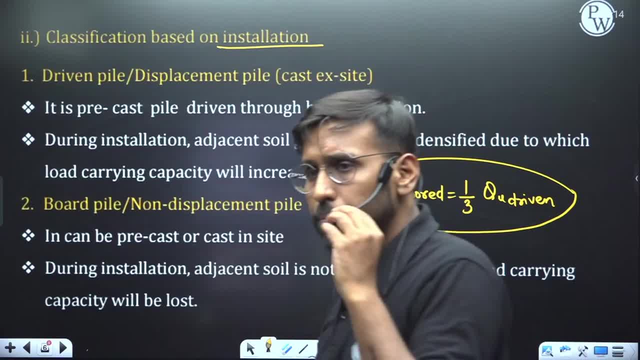 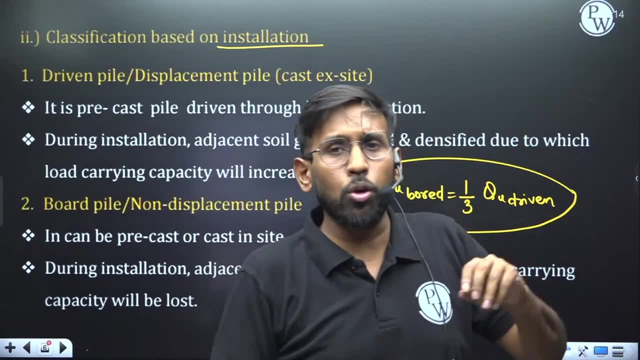 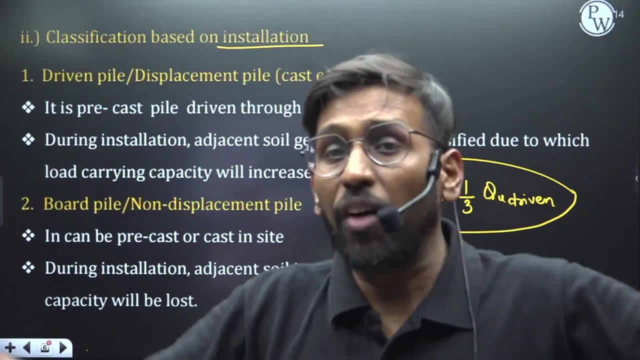 time jada board set in guna jada clear about why we match my use board files. Karen, a key agar tum they go depend karta. hey ki, apka demand, kid up just a board. pile a pile colon, chota totani a pile coffee, but I'll go heavy yoga. so, apka, transportation cost, but I 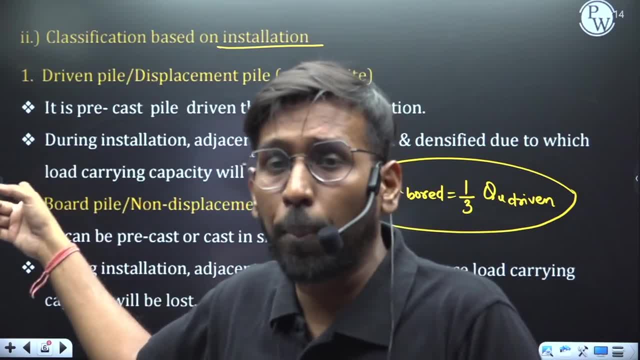 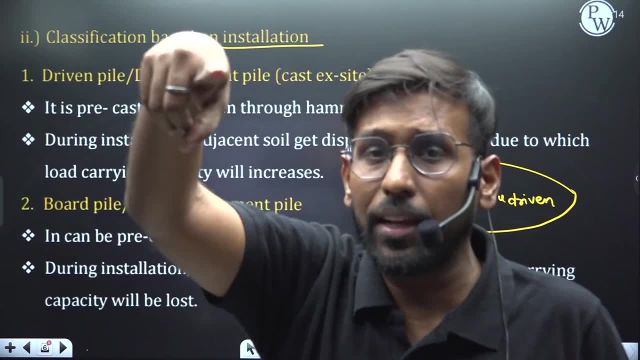 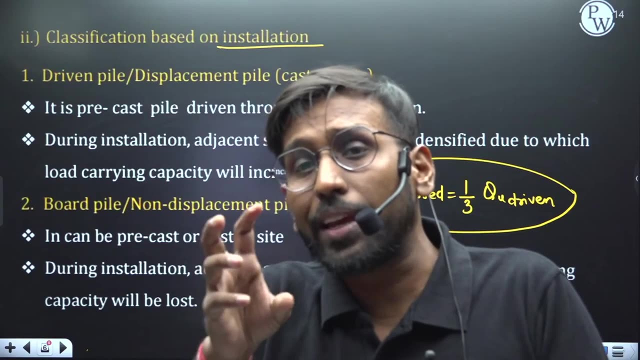 yeah, economical, come with a driven files. unless economical, yo mano para pile up hammer, get through, drive karo insight. so during the driving action, pile to take a chance a any a. so, although heavy a subculture. density by jada karstha lakin problem, kya hai what density by to karstha lakin wapa transportation cost. 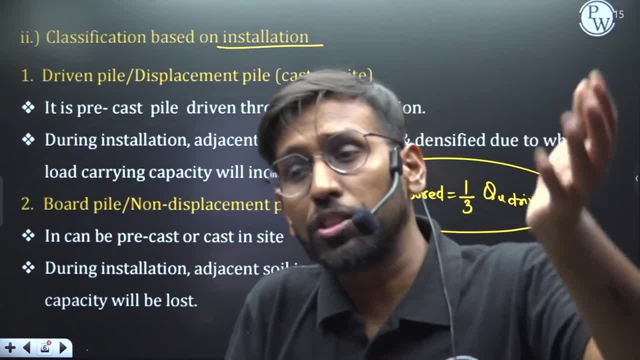 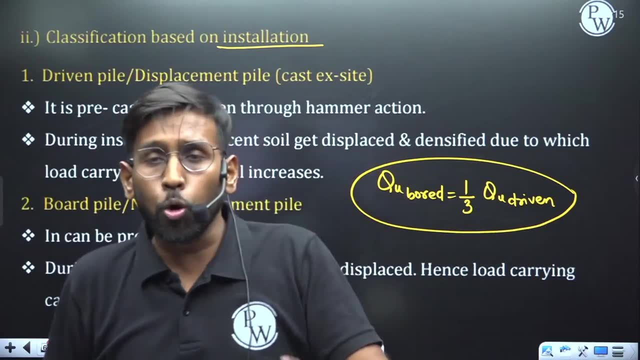 economical. apko kya hoga? come hoga transportation cause jada hoga economical. come away, see current say we go for the board files in the most of the city. oki utna demand nahi hoga. utna main strength a requirement nahi hoga. 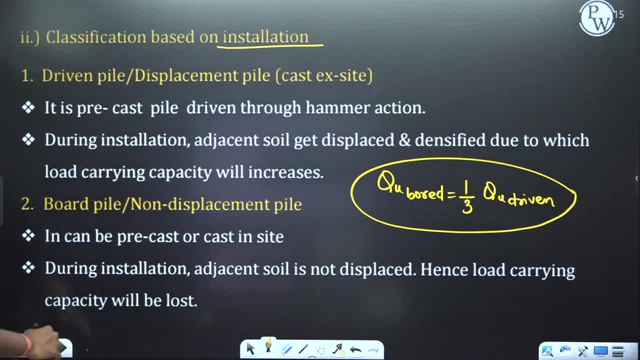 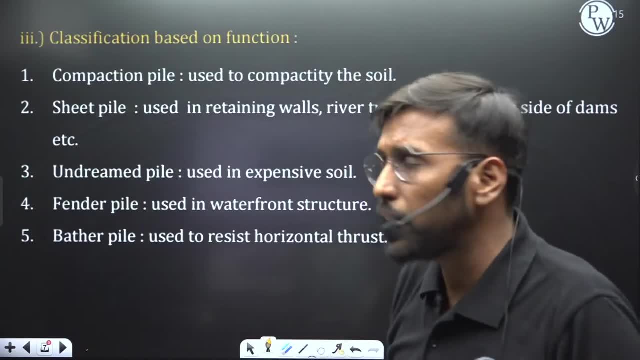 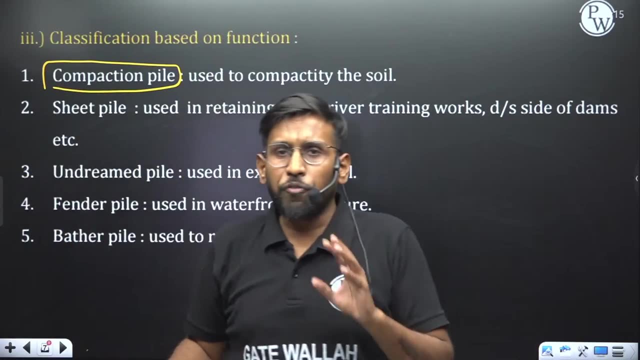 clear about the bolega now. the next is the classification based on function. next is the classification based on function. enough to pala a compaction pile. noms a clear a compaction pile. come kya function. a car role play karta a and a, they go they. 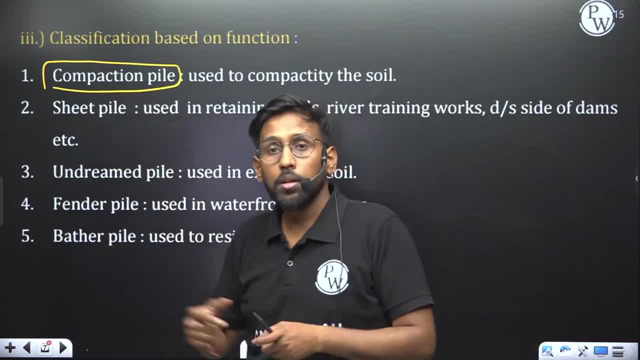 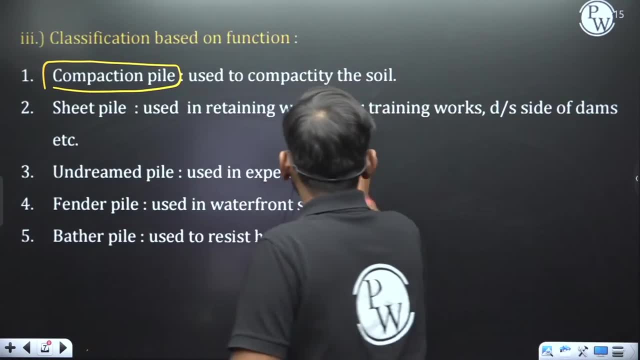 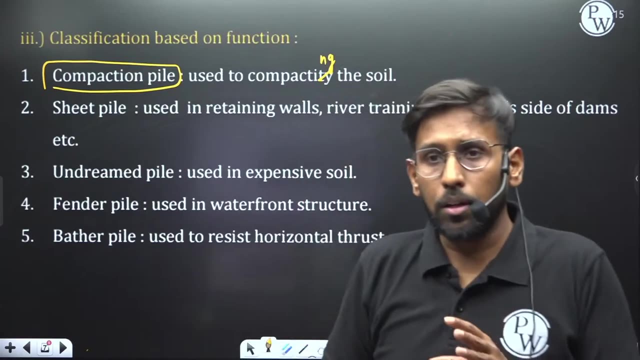 go. they go, bridge, kick all of me. they go up a follow compaction pile to compaction pile come. kya use for compacting the soil. use for compacting the soil Is idiot. compact can make the use of that. then she's pile. she is better already. take away consequent as a. 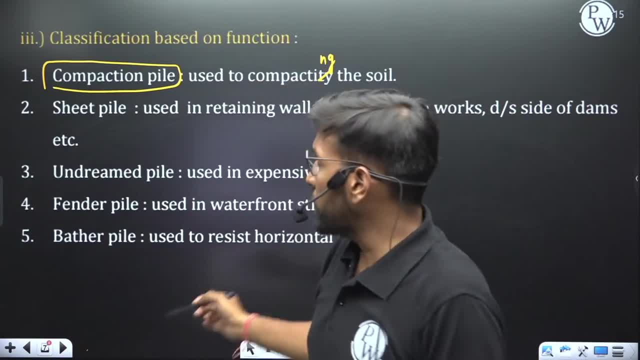 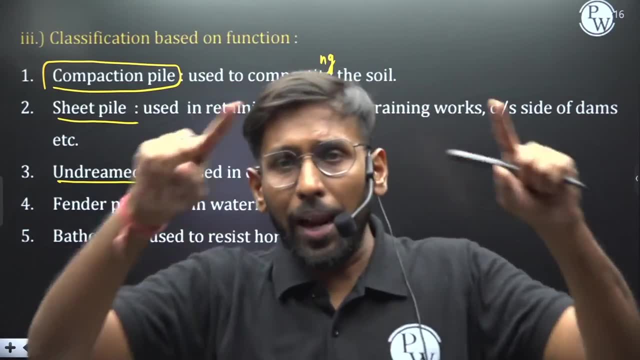 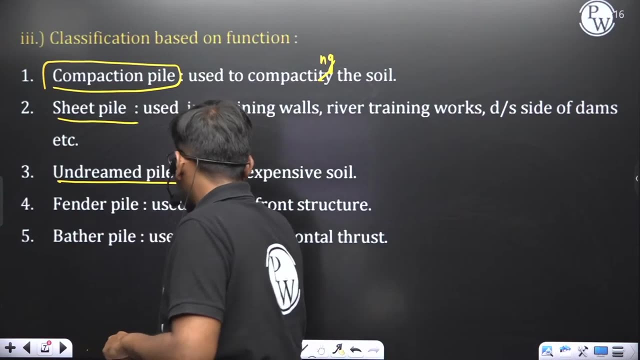 training wall downstream side of damn мина to ys розstage magishitt file again pulling it under empyrean, I guess. well, it's fancy way to have a Bulgarian structure author at choice. expansive nature. go ka kata ranges karta Odette, is your under impact? a glove up tender by Sorensening alaughs paso willnda. 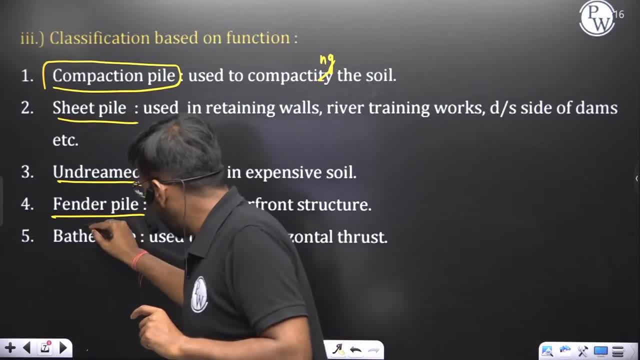 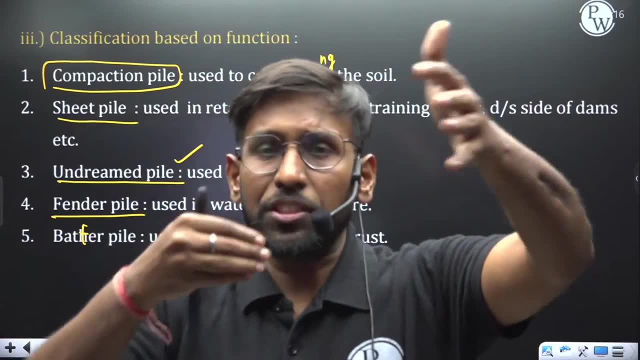 pile, sir, Suning about Kodian say: fender pile Kyoto. what is this fender pile up now? what the front structure the guy up now? what the front structure the guy? so what the front structure man of me? but I am up, we bought our I Hannah, 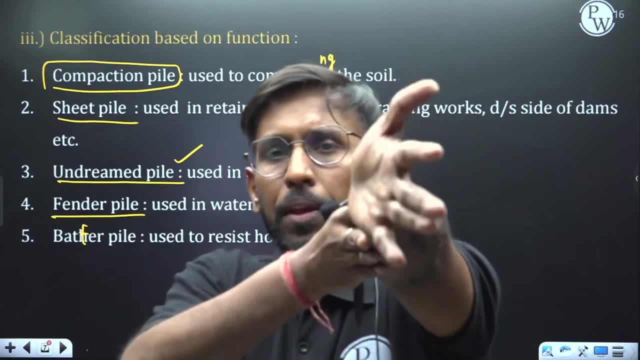 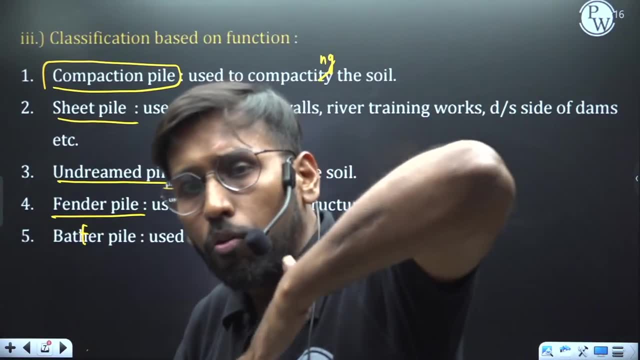 we bought our I or Pani's are case I'd most code tuck my Hannah so by a coca-cola got up quick partition. there are banana a gap, matlabic row banana para que vaya japania jab bota que tocara a to. 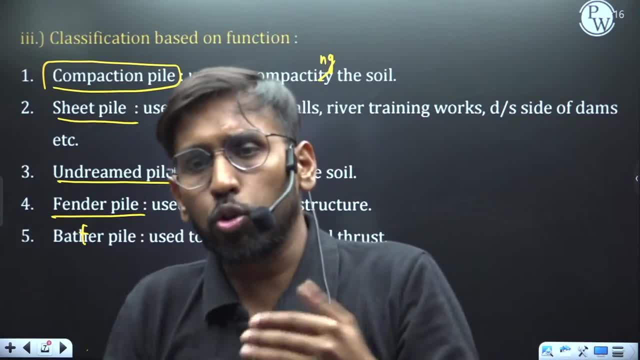 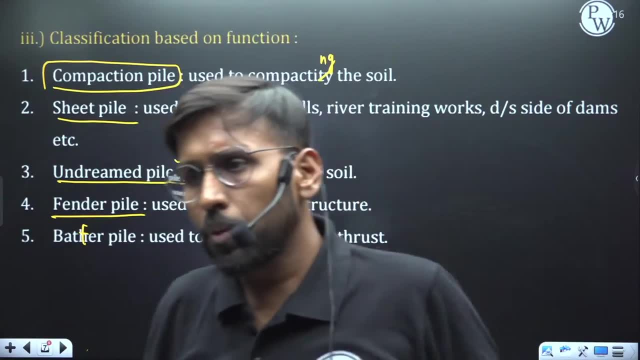 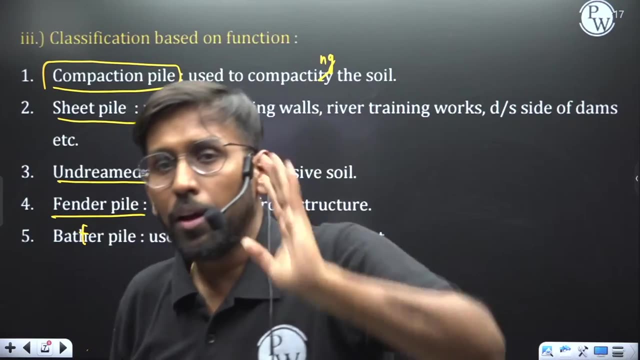 mirror job tight, say, oh, I fit now. so I'm kakaing off a fender pile along the length. I'm dating it. a key may remain just remote. disturb now. ah, here about math is weak shoe or a math is weak shoe or a mess. which Rona key her Sunday. 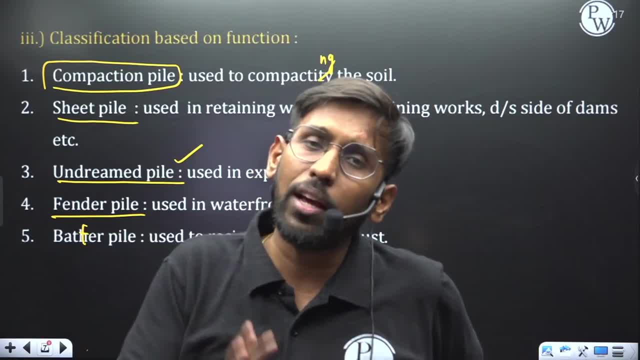 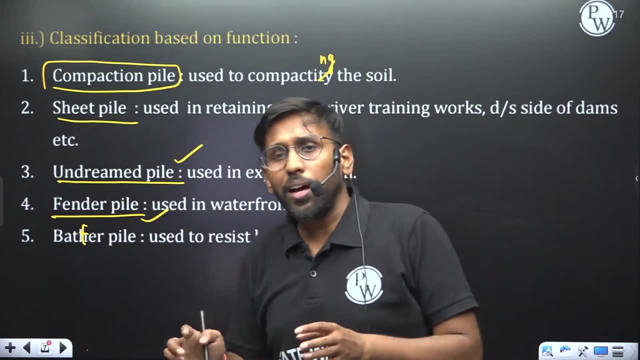 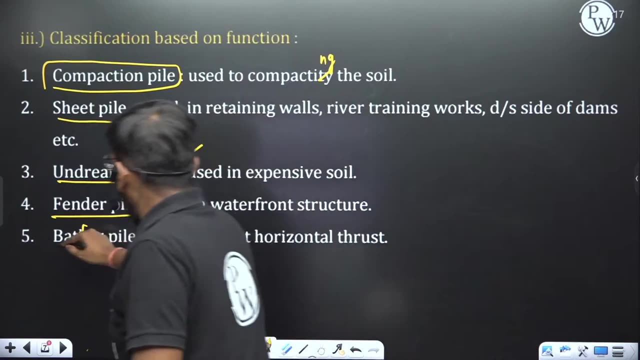 AMA session. le loom tomorrow man a boat, sorry doubt. so the fender pile kya ho gaya up agar kya karo waterfront structures? my construction karo to prevent the collision. you have to prevent the damage. we go for the fender pile. agla abka batter pile, agla abka batter a pile, batter pile kya hota. 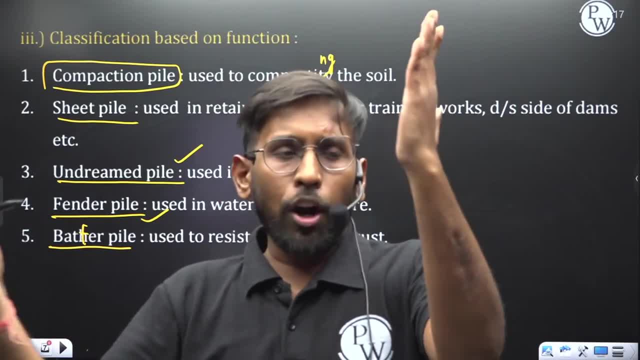 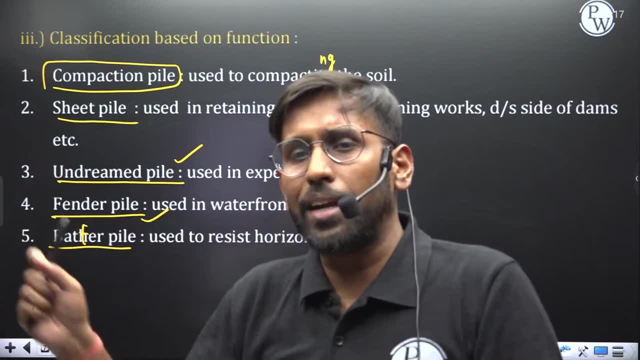 hai jaise maalo ki earthquake asatta hai to horizontal load code resist karne ke liye. horizontal load code resist karne ke liye, jo pile diya jata hai, that is the better file to resist the horizontal load under in pile. there ko kya hota padhahenge beta. 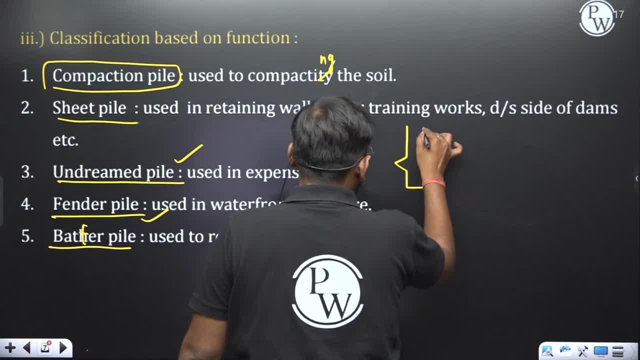 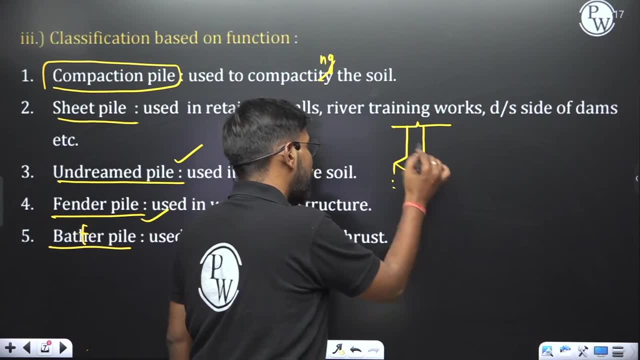 agge iss tarike ka public shape dia jata hai. so iss tarike ka bulk shake dhene se kya hota hai. the resistance increases you ok, the어가 pe kya hota hai. area bar jata Boarder of résistance ka area. 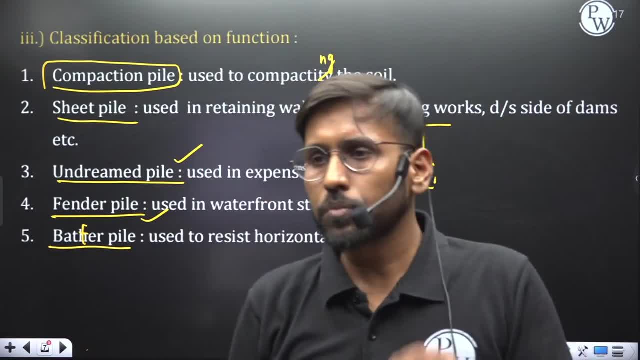 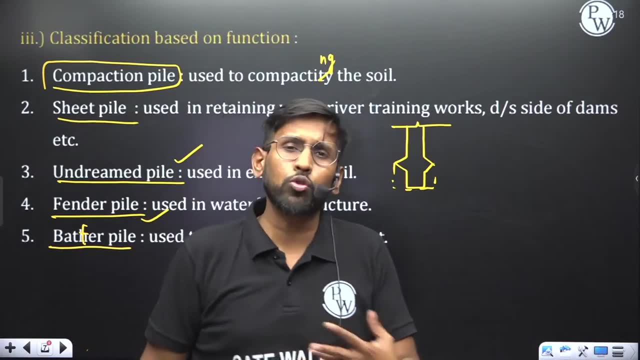 birrata hai Higa tiy. so aage discuss kare decir, sāke discuss karedge. hi ke bhai bulose Romani so hate the battering. butterden is a caste based on. indoors are best combination alleged across capital SEO. may yeah match the following got a quiz so I push the up out of this. so I've got. 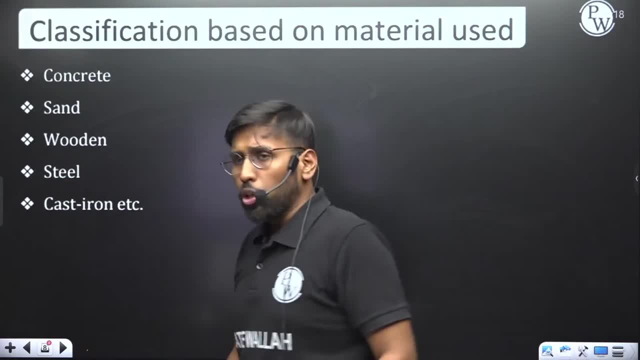 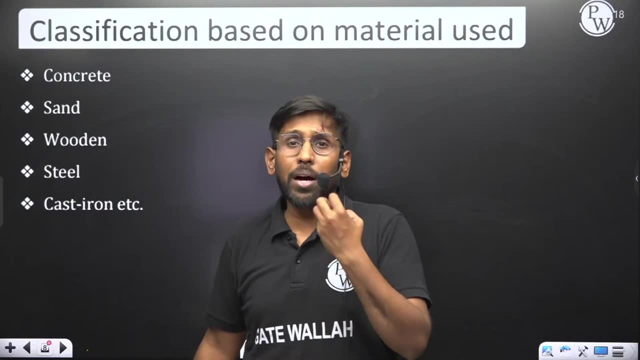 clear on achieve any. now the based on the material used above cup, I'll host at the high concrete. Sabana ho host at the pile up car wood. Sabana ho host at a conk up a pile. Joe, have a sand pile. oh, host a voice steel. 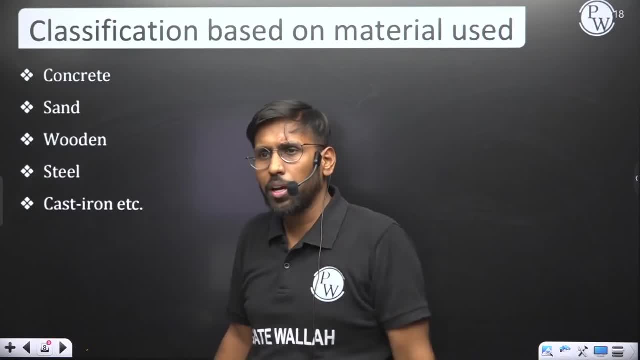 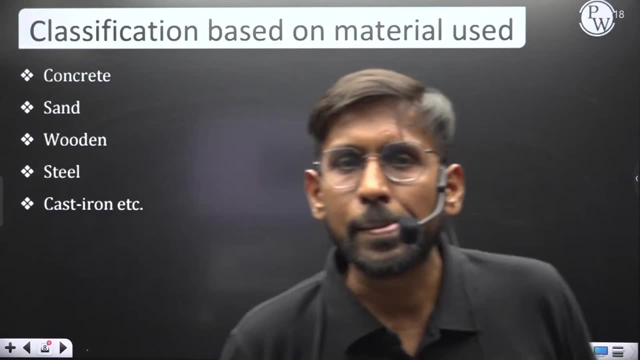 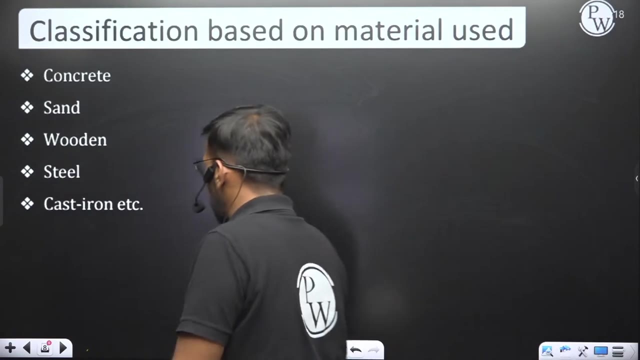 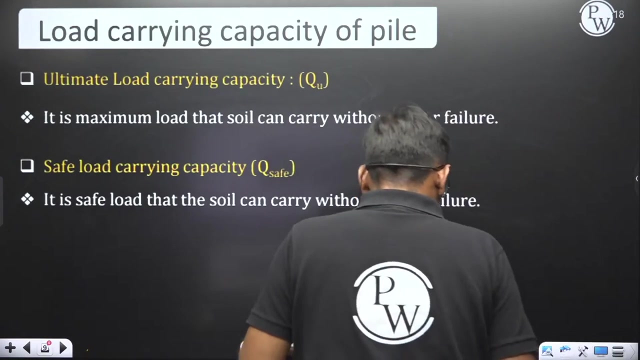 pile, a host at the cast iron pile, and many more, okay, many more. what are the flow may bridge capable column me? well, foundation, but I day. well, foundation, but I day. well, foundation, but I day. okay, they came up a bit. so sorry, I'm nice. sorry, classification: key bath. 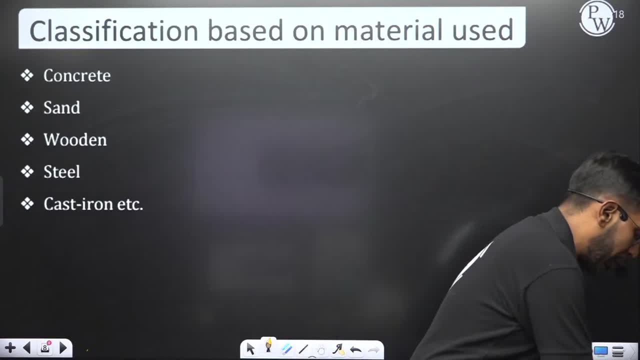 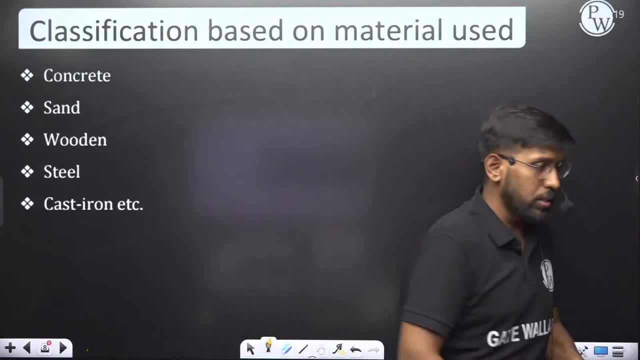 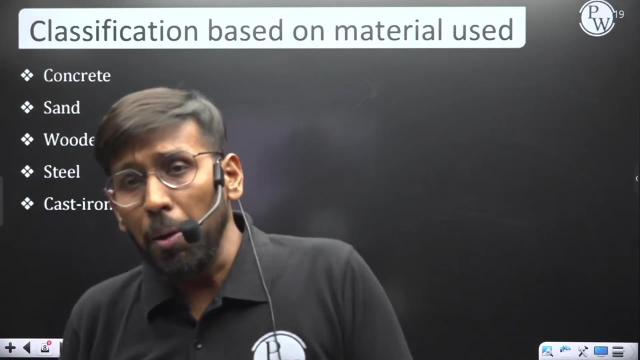 use is based on function and based on resistance. yeah, I'm a palai, so made it those. agar maibhav Karo based on resistance, so keep nether UK ke pile winning it. agar maibhav Karo based on resistance, so keep nether UK ke pile winning game. 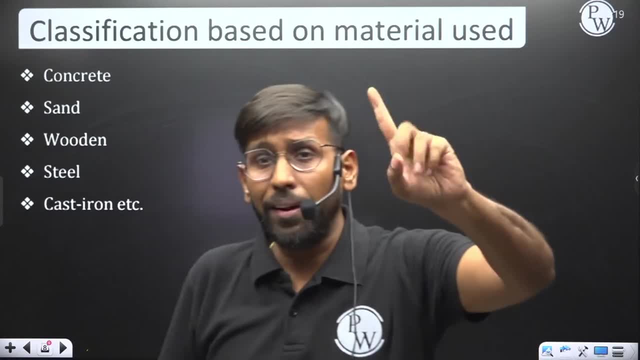 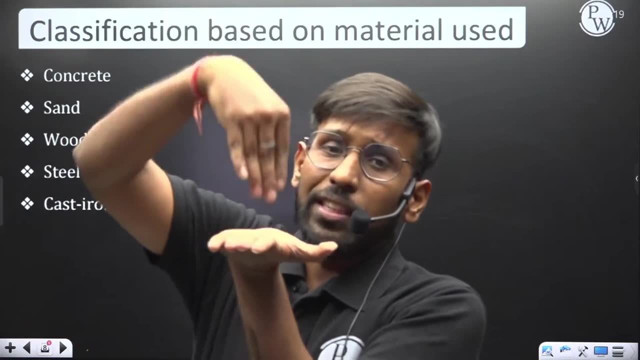 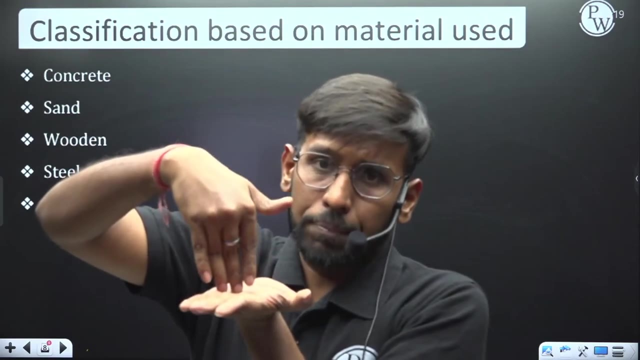 there are three types of pile: Palin bearing file- do solve corruption- file, Desaar and varying. I'm fiction file, a good a friction and wearing key Bob's curry. oh, the resistance is observed from the bottom. bottom, the resistance will Roga Anna. the pile is resting over the hard strata. next I got a fiction key. 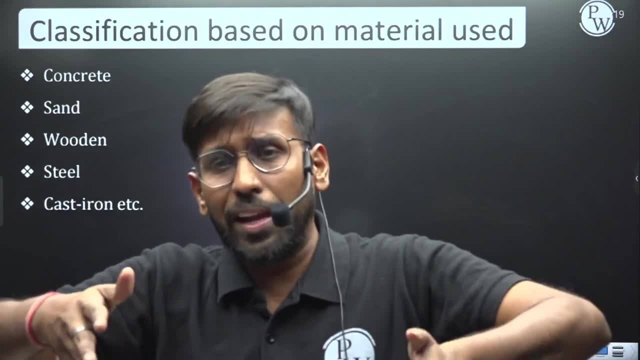 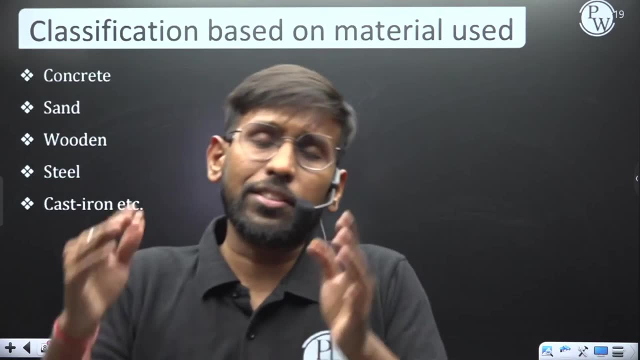 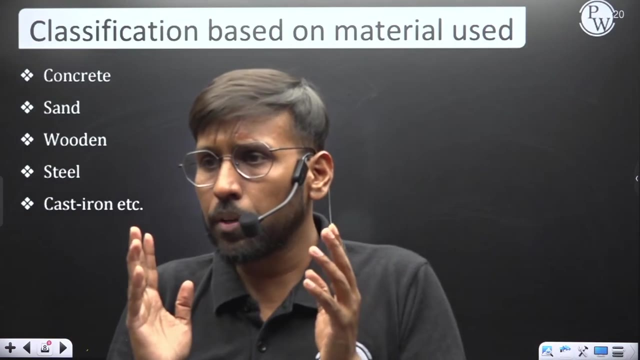 Bob Carao. the loose soil, a dust, a beast meter compiled a length, a. the resistance is observed from the sites I got a bad color and bearing and friction pile, medium to dense soil, a. the rest is observed from the sides as well as from the bottom. you know this. in sight, similar a, or bottom, similar a. you know. 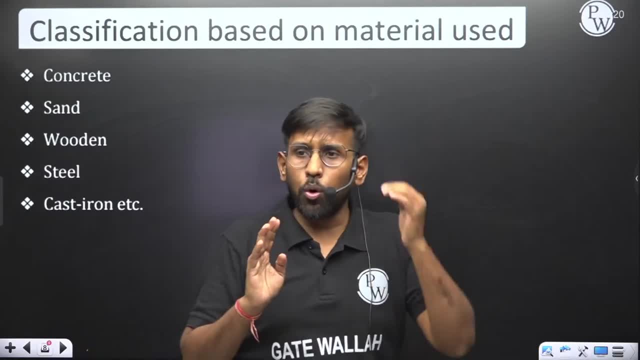 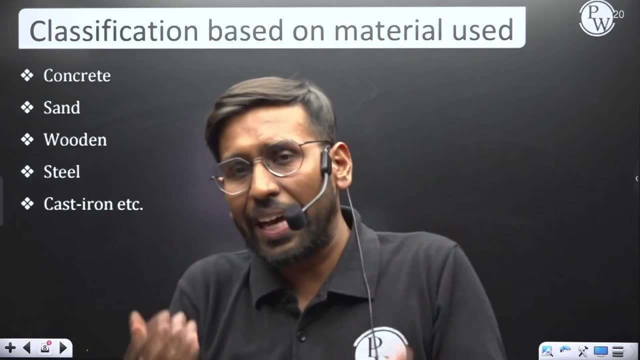 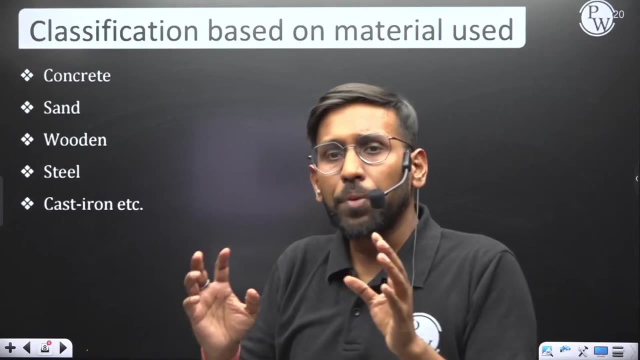 they go gaga, they go gaga, they go gaga, no, no, no, no, no. the resistance observed from the sides as well as from the bottom: Abba gaga about curtain, hey. Abba gaga, Ram Bob curtain, hey. so I'm a product classification based on installation. 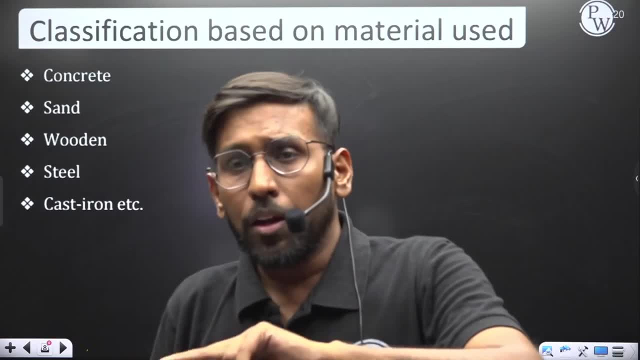 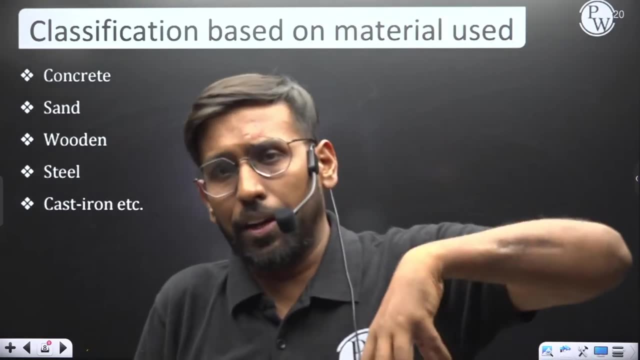 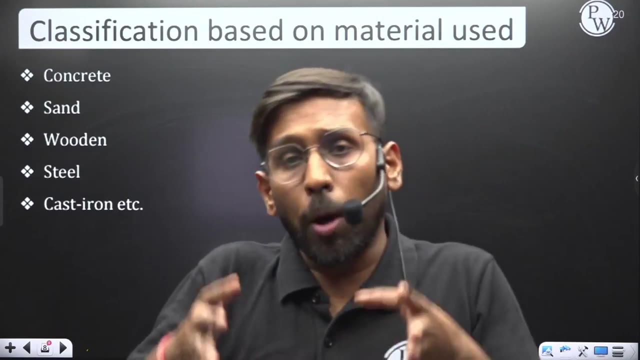 from a door, three capable driven and four pile so driven, pile, make a ball omni. it is cast at C to model a factory made. pile a I'm drive car right. so just a car and soil care at density fire. I so load carrying capacity but like like in here, you're bored. pile a, Tom Nick, a boring. 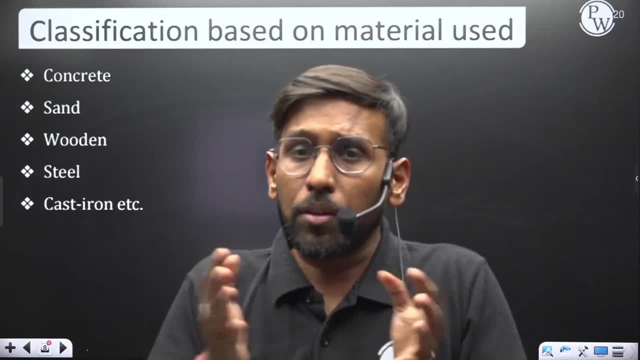 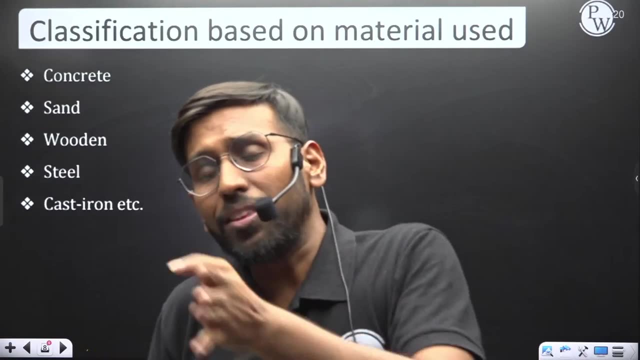 Kia Hamlet's my pile Kia to have a car. I the soil is not getting density, fight to data strength, so it's got load carrying capacity. come with a Tommy cabula Q board is one third of Q driven a glabella based on the function, the base on the 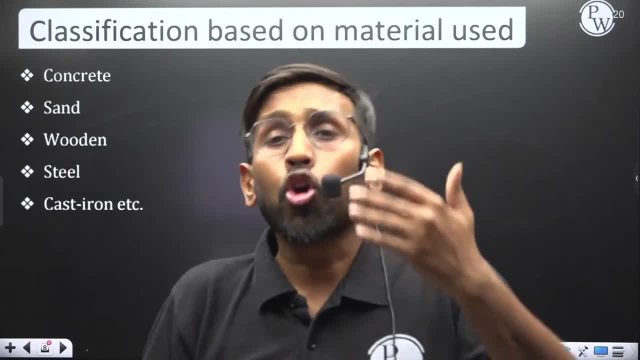 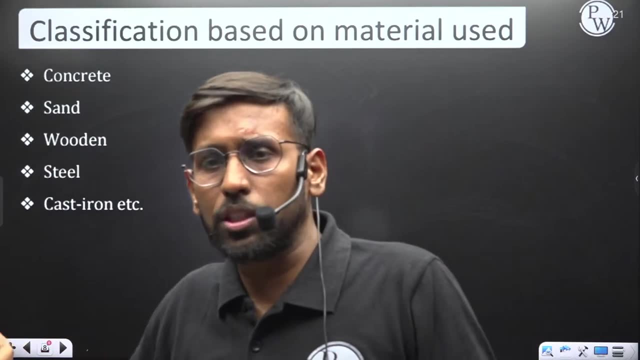 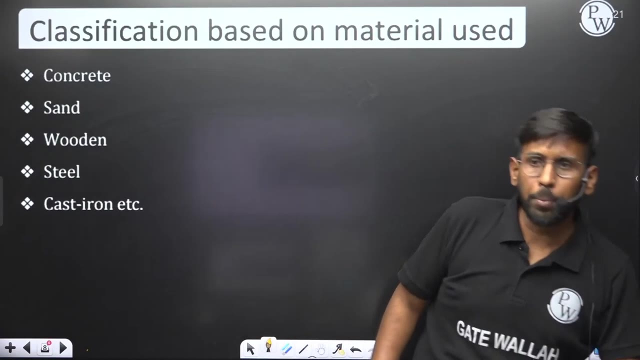 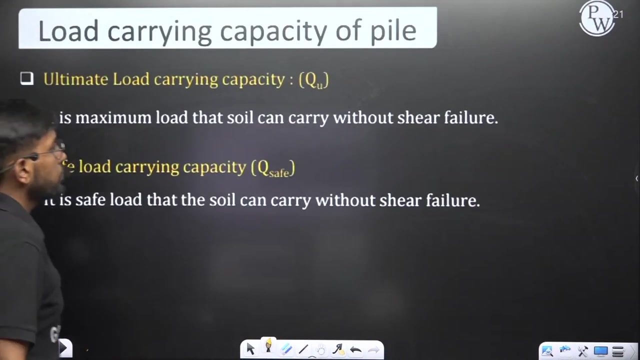 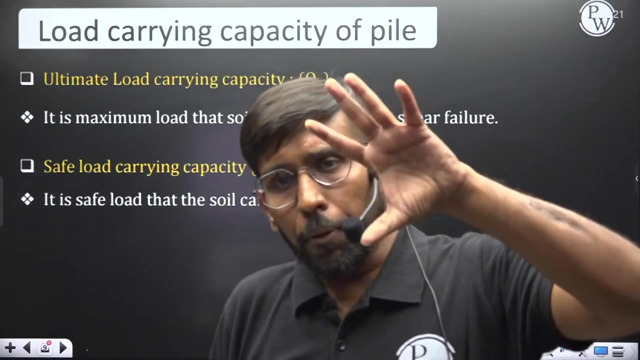 function. we have the sheet pile, we have the fender pile, batter pile, compaction pile under impile like $5, ready for all the down. an impression of this side: Sensek Ahmed, level of base on the Mandarin used to concrete sand. wooden sealed cast iron th geschafft. we have matter plant based on the maternal use. so concrete sand wouldn't season cross travel. yes, Adam may discuss clear player, a bath top, eat a kitten up on a mat. now we got awesome How to get rid of a dez. to get rid of a dez clear bad others. Hello, take on, This is a запис made today. clear thers Dzia Wieck, zia Wieck, zias, gabi blandi m Polish Wooden Michalow, lego, Buzz Thai and Mar隨 You at Surrey English. Learn French as well. the Englishduo very close to learn the Irish subject you know So veteran. so, ladies out, there is one of our Lexi refresh buddy. we learned some things about her. let us know how it all went on. 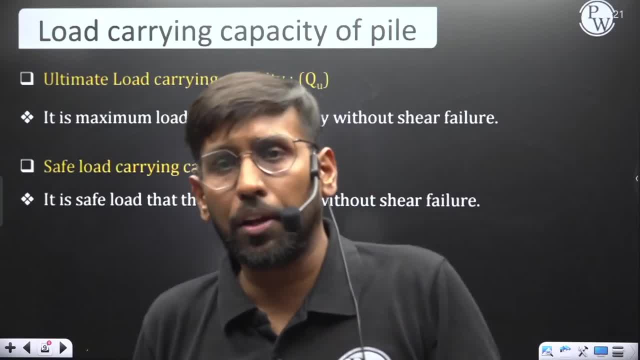 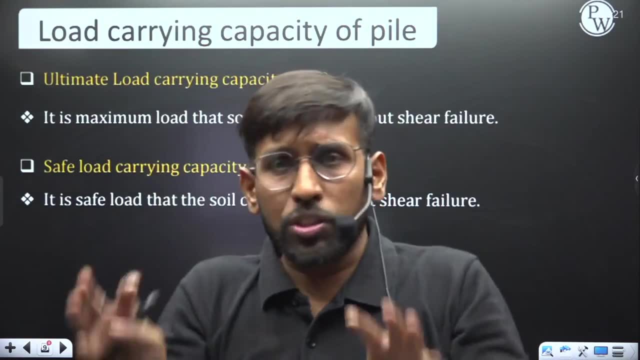 four parameters. we will not take it out here. why will we not take it out? because, my friend, whatever load you are applying, it is going on a whole concrete element. is there any soil coming in between it when you are doing construction? 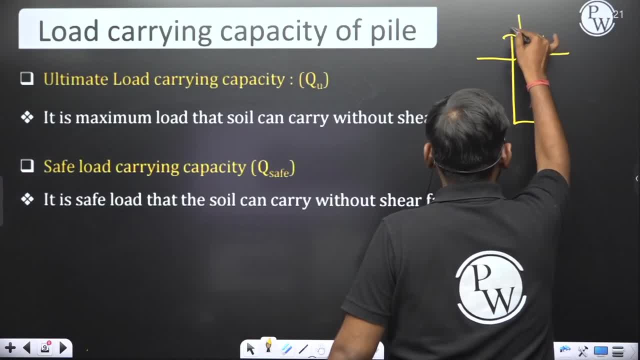 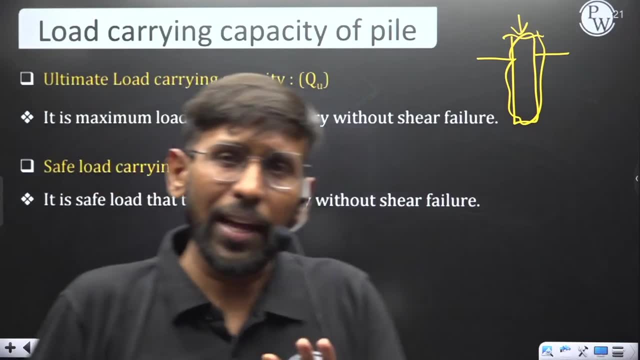 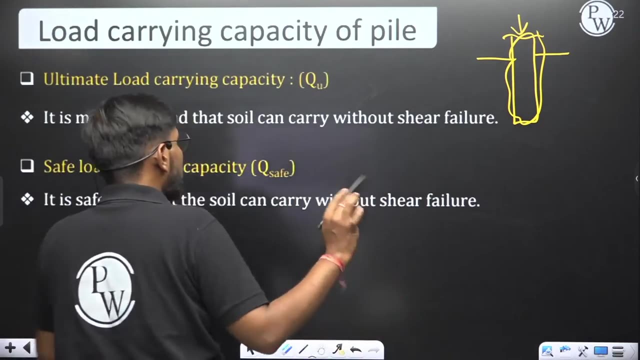 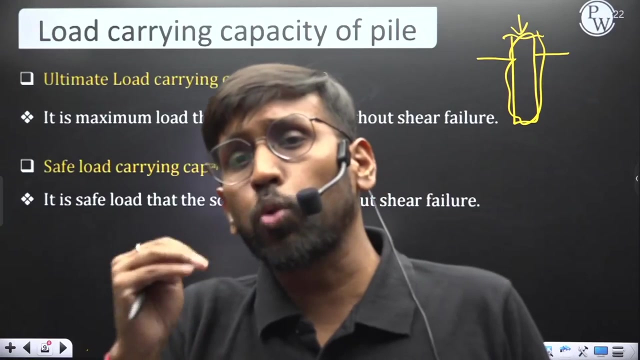 if this is your pile, then the complete load is going on it. is there any soil coming in between it? we will work directly with the ultimate here. there we will not talk about per unit area. here we talk about total load. I say ultimate load is the maximum load that the soil can carry without shear failure. load is the maximum load this soil does not carryed with no a shear failure. It is a maximum load that the PILE can carry with no a shear failure. This is a maximum load that the soil can carry without a shear failure. That's the ultimate load. 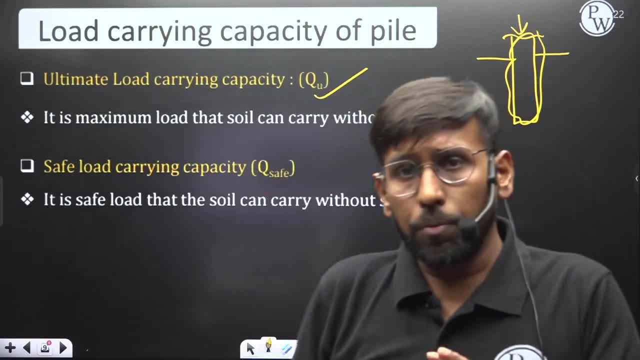 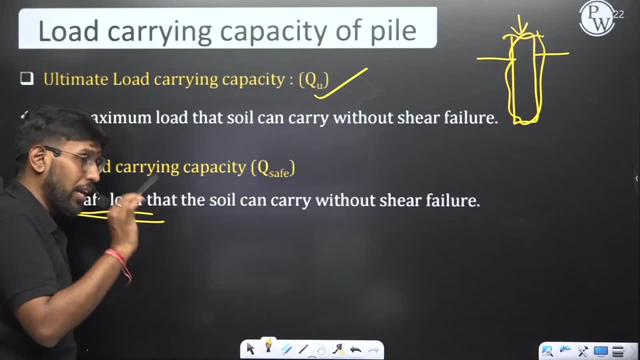 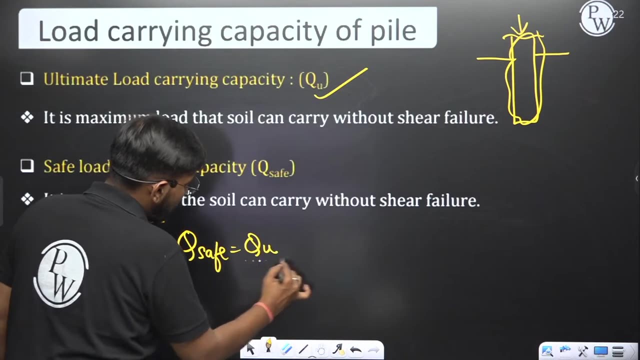 And what is the safe load? It's a safe load that the soil can carry without share failure. Right Safe, load Right, Stay safe, Don't fail. So what is Q safe? What is Q safe? Nothing but Q. ultimate upon factor of safety. 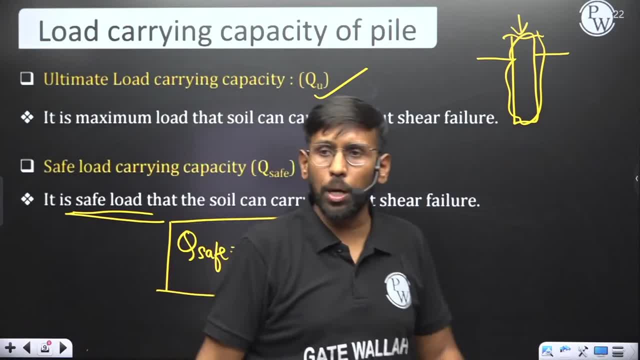 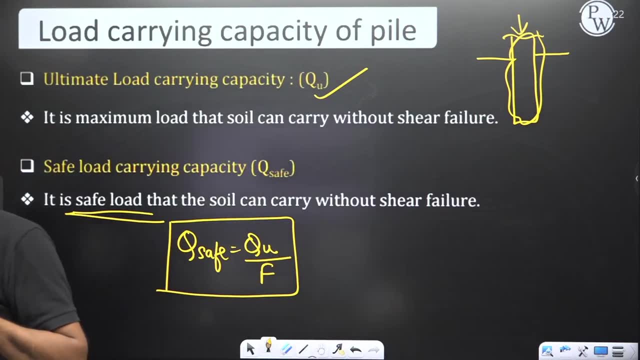 That's it Here. it will be direct Here. there is no flaw. So Q safe, Q ultimate upon factor of safety. Is it clear? Is it clear? Is there any doubt? Now, sir, let's talk further. 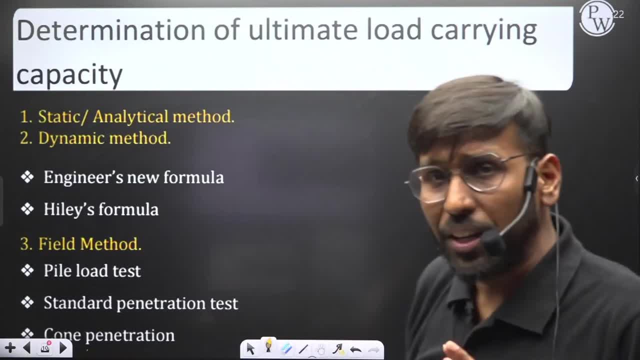 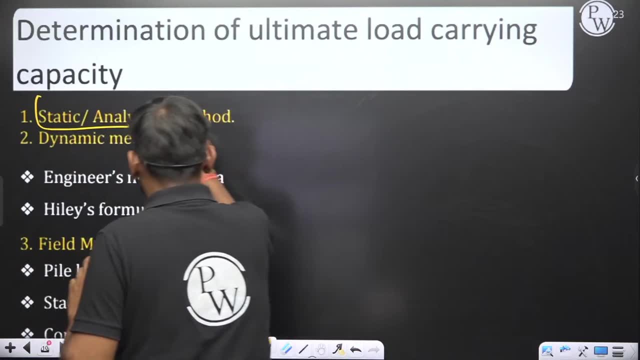 So how to find load carrying capacity? What are the different methods by which we can find the load carrying capacity? So, first of all, static or analytical method, Static or analytical method. So now see which methods will be read here. 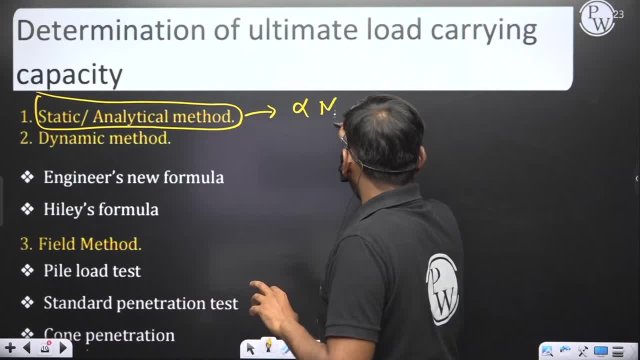 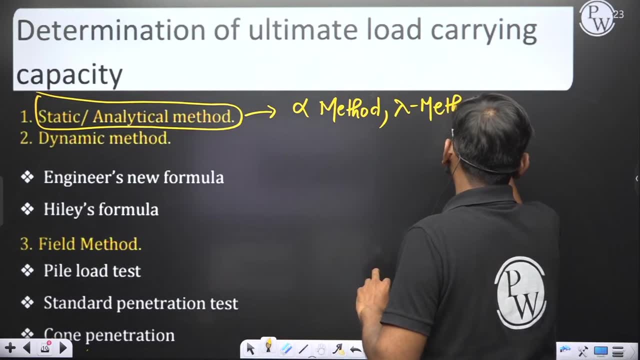 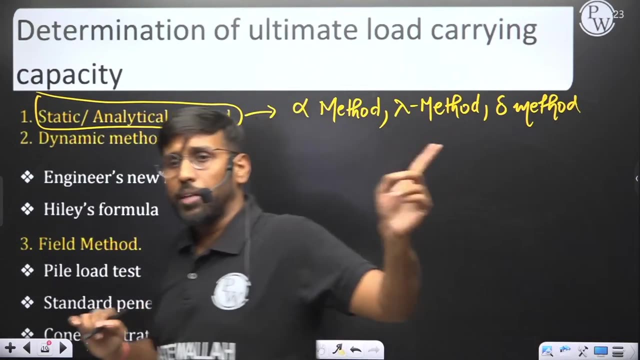 We learned alpha method. We learned alpha method, We will learn lambda method, We will learn delta method. These are all methods, my friend, And the question has come from all of these in the gate, From all the methods. already the questions has come. 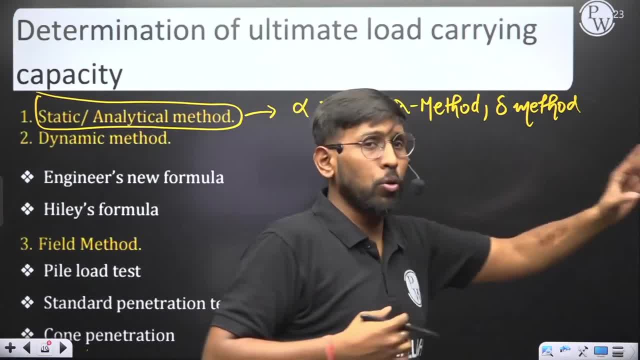 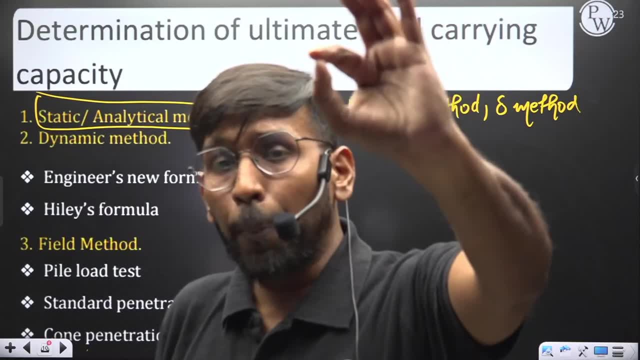 And, sir, trust me, you will remember all these methods. Trust me, you will remember all these methods, Promise, Promise. You should have a formula, ie a single glimpse in your mind, Okay, If not, then you will do day life. 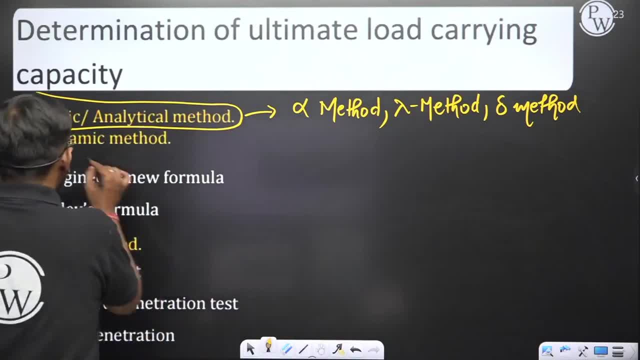 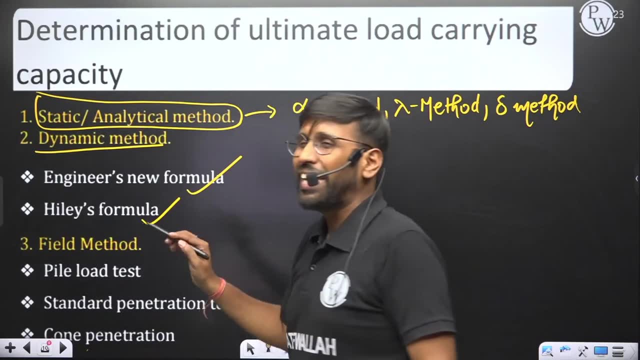 I will teach you in that way Dynamic method, which is done in the field where you have two formulas: One is your ingenious new formula, the other is your helios formula. Two formulas: One is your ingenious new formula, the other is your helios formula. 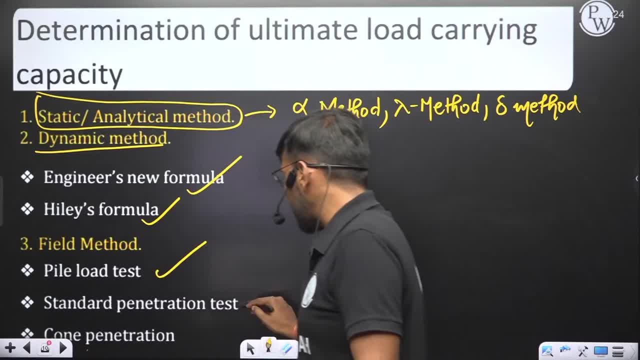 So these are your two formulas. We will do this too. Then pile load test: SPD cone penetration. These are your three methods. Okay, These are your three methods, So let's move to the first, ie analytical method. 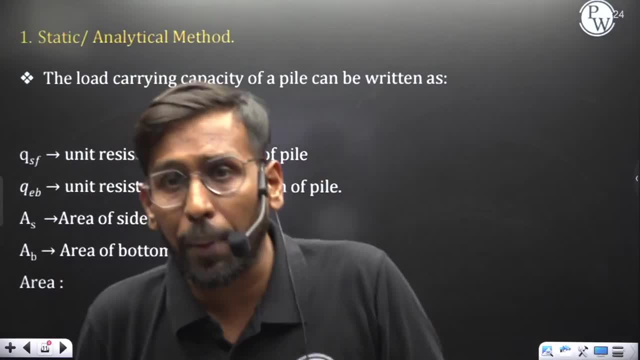 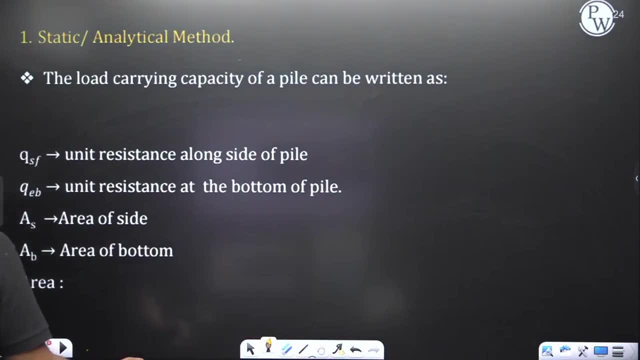 But before going to analytical method, there are some things which we should understand. Okay, Try to understand this carefully, Sir. we said ultimate load carrying capacity, Skew end bearing plus skew side friction. Say yes or no, This will be done. 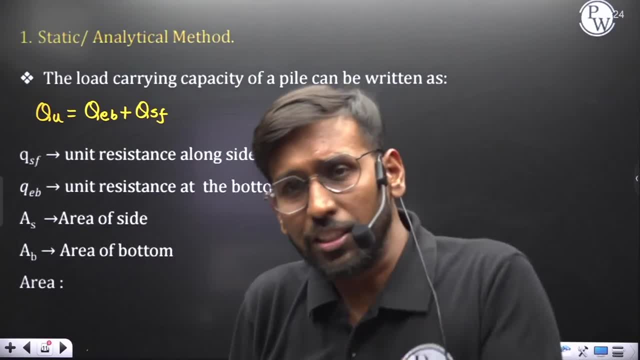 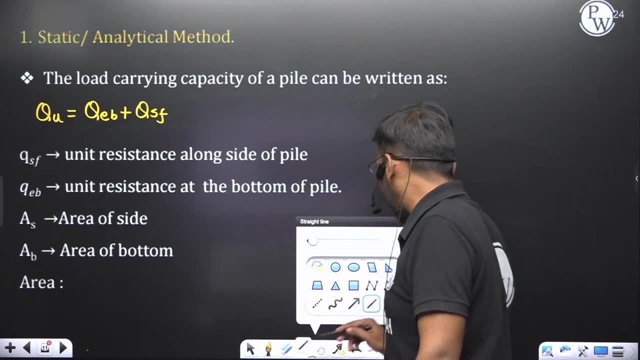 If I talk generally, then resistance will come from the bottom as well as from the side. You will say yes or no. Resistance will come from the bottom as well as from the side. Say yes or no. Say yes or no. Yes. 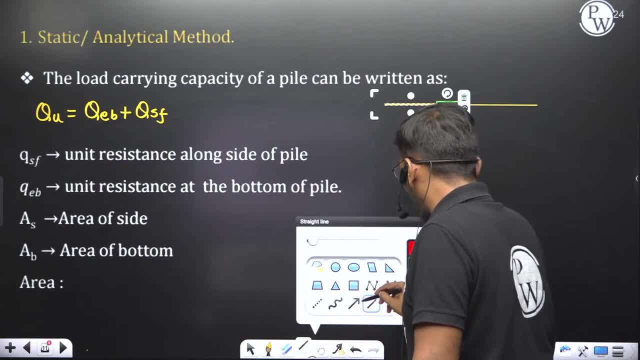 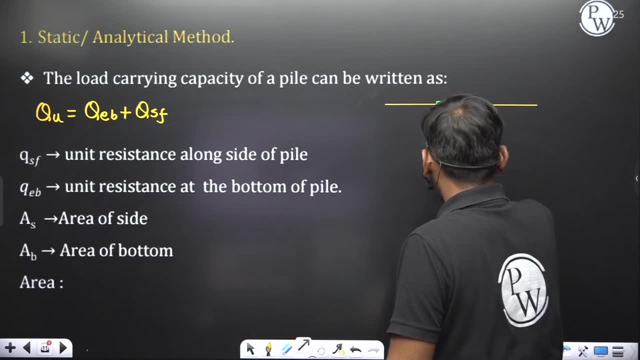 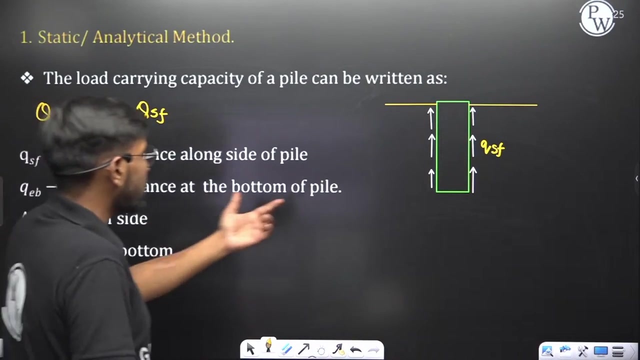 Look here. So if I say this, the resistance on the side, in terms of stress, that is your QSF, That is your QSF. Okay, The side resistance, that is QSF, Isn't it Side friction or side friction? what are you saying, brother? 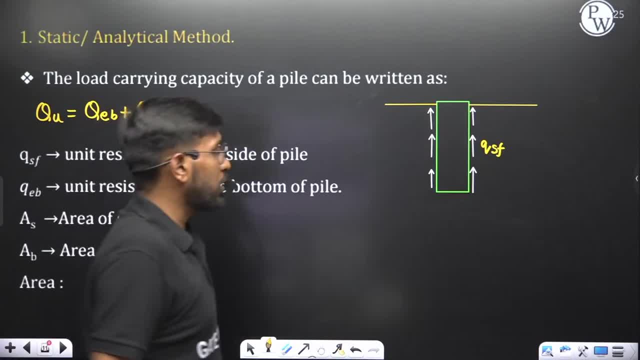 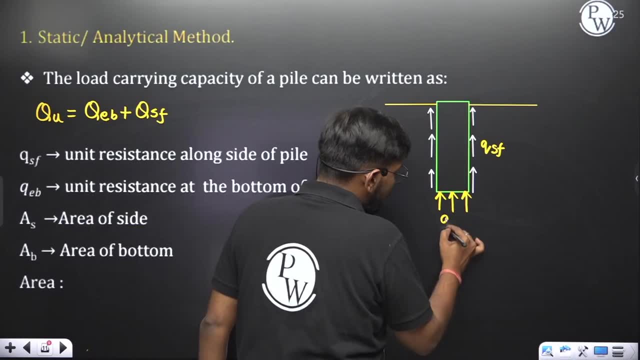 Side friction or side friction, it is the same thing. Which friction? Okay, yes, it is the same thing. Look here. The second resistance that is getting is getting from the bottom. So if I write it in terms of stress, then I am writing small q, end bearing. 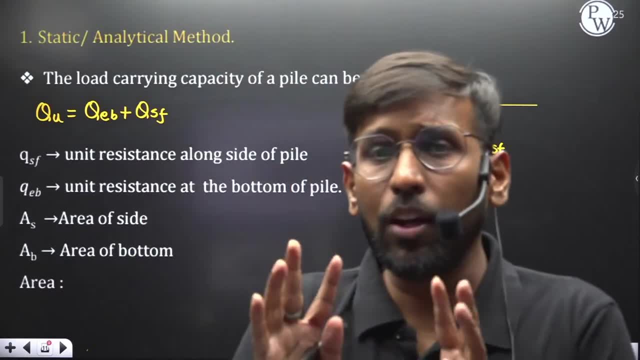 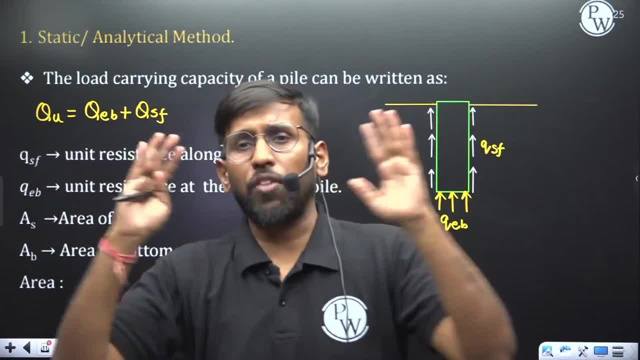 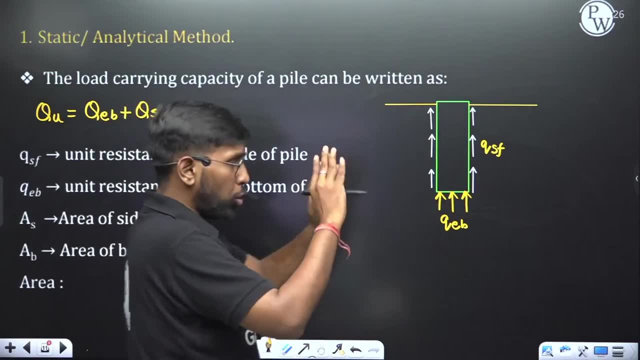 If I talk about QSF then it is on the surface. So here, the area which is multiplied, it will be the surface area. Hey, say it, brother, With QSF, if we have to take out a load, the area which is multiplied. 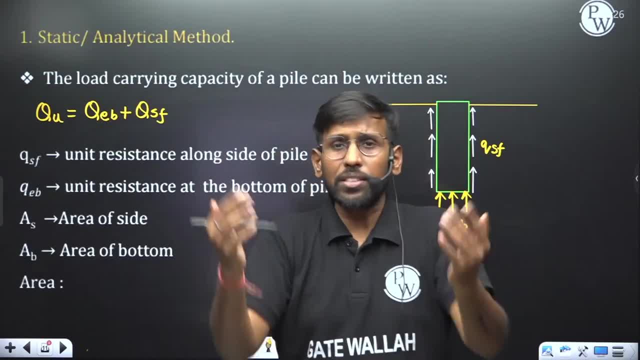 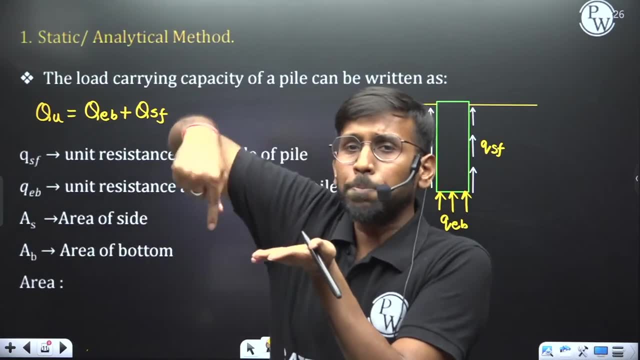 it will have its place on the area where it is. So the area which is applied is the surface area, And if I am looking at end bearing, then kis pe lag raha hai Ye end bearing, kis pe lag raha hai, This end bearing. 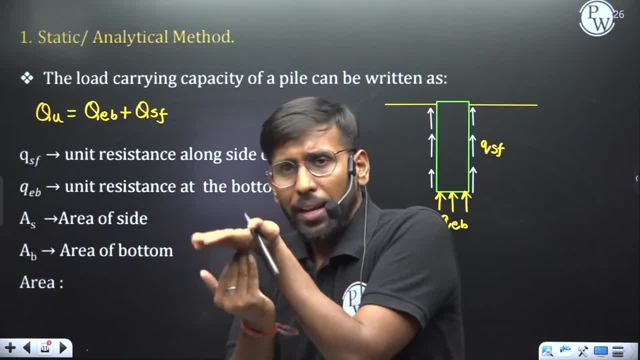 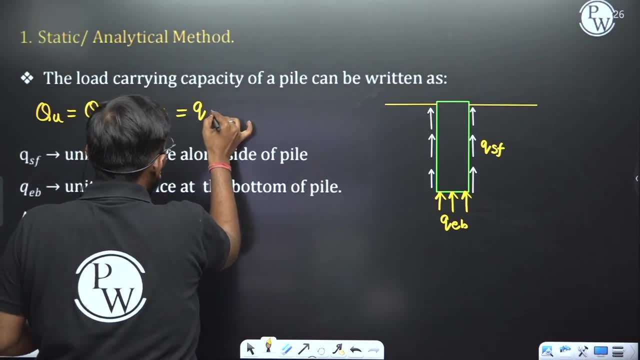 is acting on the cross section. Ye end bearing kis pe lag raha hai, Cross section pe lag raha hai To mere dost yaha pe. dekho mai, kya likh raha hoon. Small Q end bearing into area at. 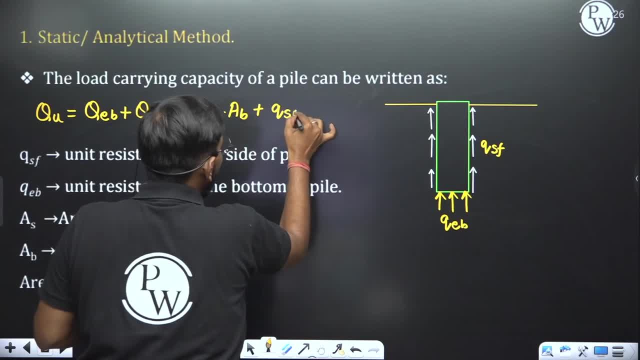 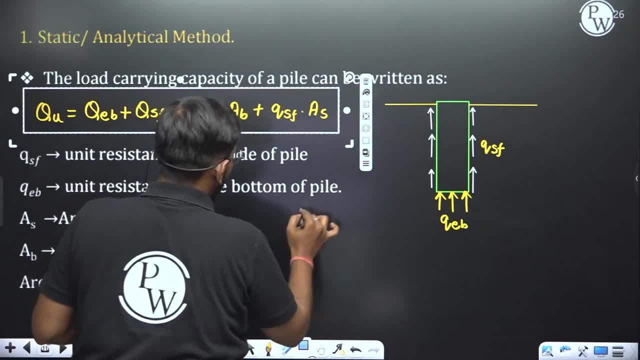 bottom plus Q side friction into area of sides. Anyone having any doubt in this, Anyone having any doubt in this, Ab sir, dekho isko aur thora elaborate karenge aapko samajh me aajayega. 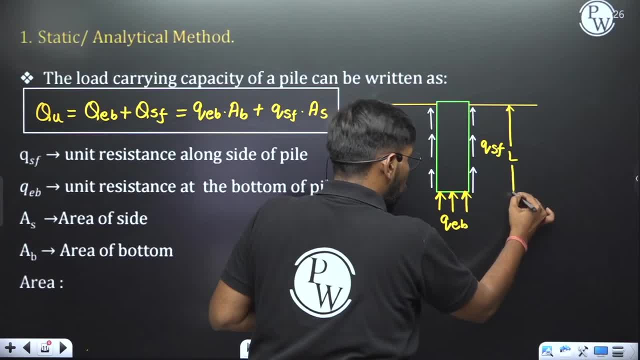 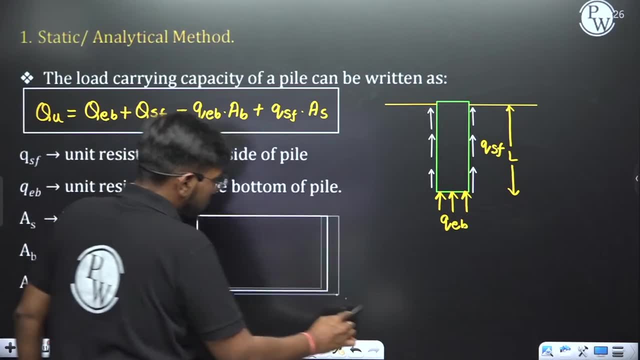 Maan lo pile ka length hai L Maan lo pile ka length. kya hai L? The length of the pile is L. The length of the pile is L. Sir, bahut easy hai, sir, Sir, bahut easy hai. Cheeje, bahut asan ho jati hai. 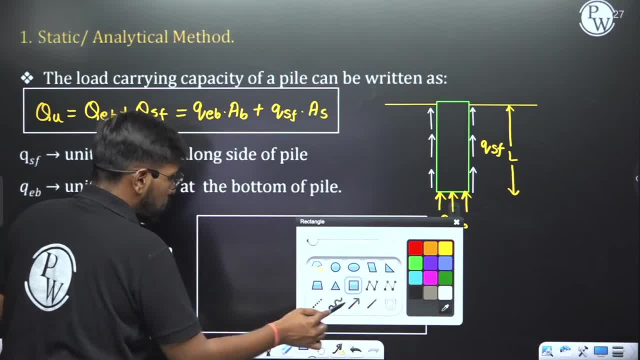 Agar hum samajh ke padhate hai, Wahi cheez muskil ho jati hai. Agar hum rat ke padhate hai, To ratna chhodo samajh na seeko, Sab samajh me aajayega. 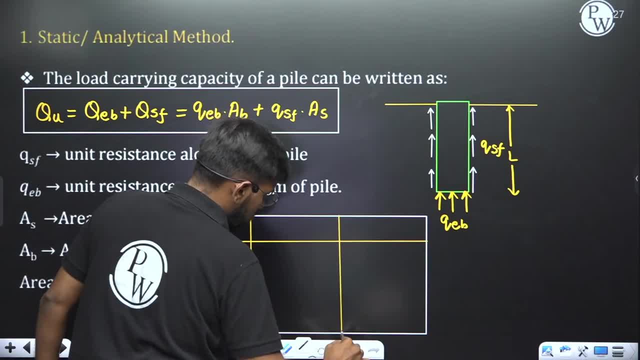 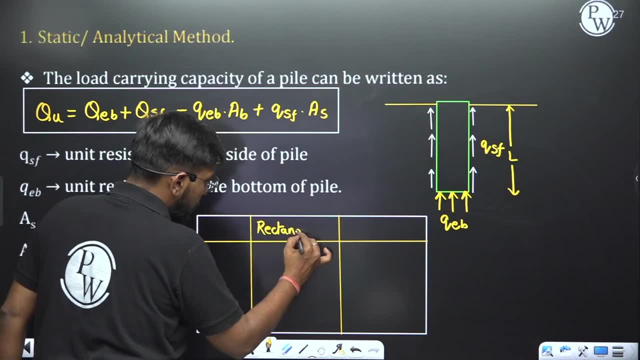 Dekho, yaha pe To pehla mai bol raha hoon kiya Rectangular pile hai Rectangular cross section hai B by B, Rectangular, nahi Square pile hai Square pile hai B by B ka. 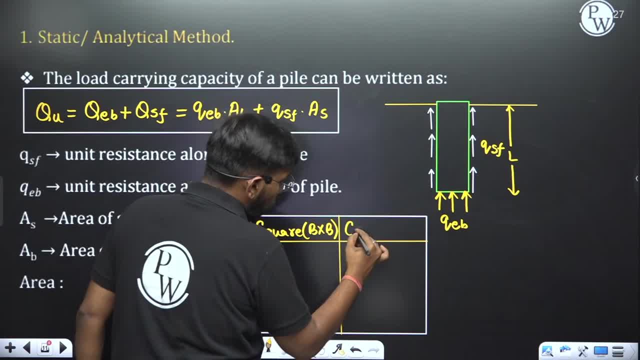 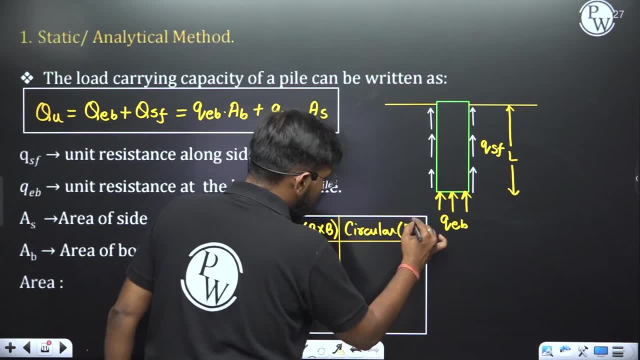 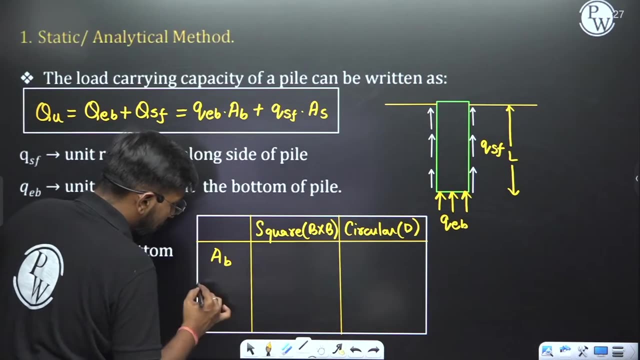 Aur dusra hai aapka Your circular pile, Circular pile of diameter D, Of diameter D To humko batana hai. What is the area at bottom? HUMKO BATANA HAI KEY. WHAT IS THE AREA AT BOTTOM? HUMKO BATANA HAI KEY. WHAT IS THE AREA AT BOTTOM? 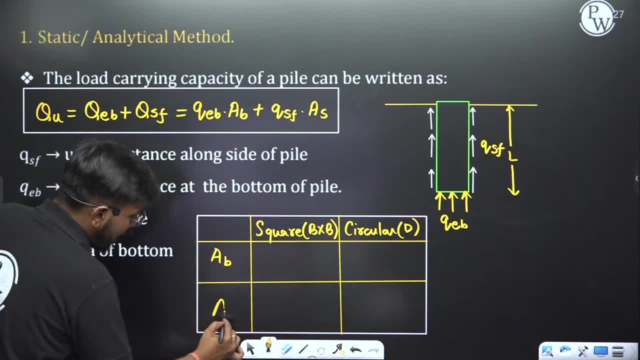 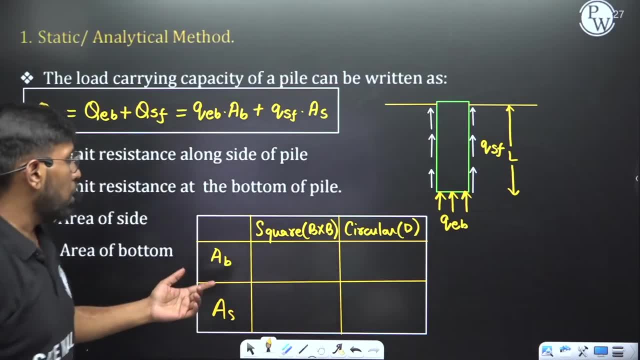 HUMKO BATANA HAI, KEY, WHAT IS THE AREA AT BOTTOM, Aur dusra humko batana hai: What is the area at sides? Bahut easy hai, sir. Bahut easy hai. Hai ki nahi hai, Sir, aapka cross section is square. 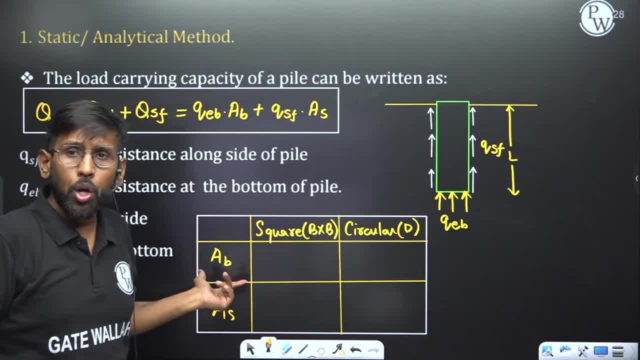 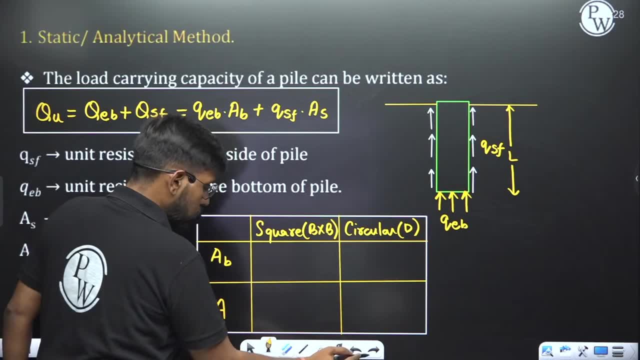 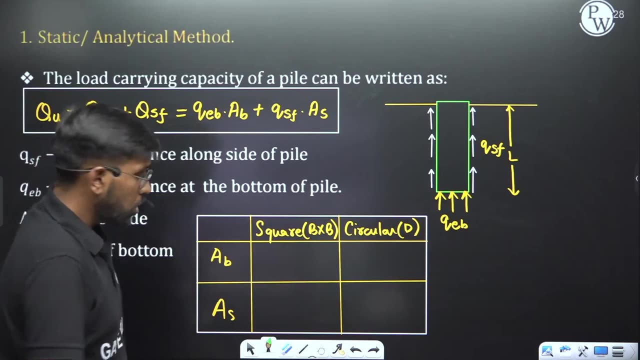 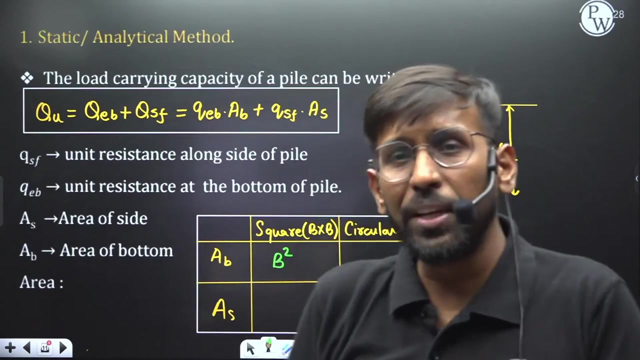 Length hai L. What is the area at bottom? What is the area at bottom, Bolo sir? What is the area at bottom, Bolo sir? The area at bottom is how much? Nothing but B square, Yes or no? The area at bottom is nothing but B square. 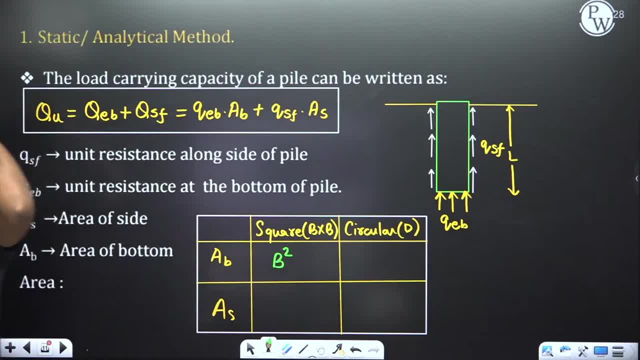 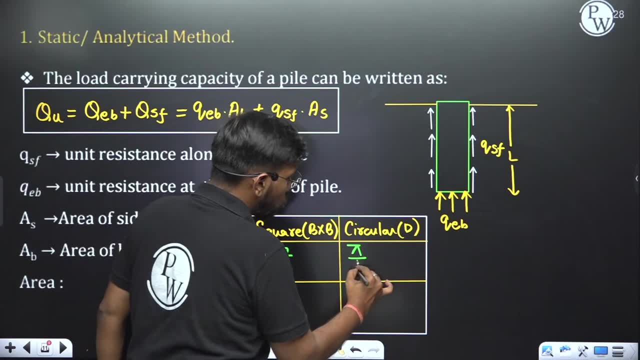 It is talking about square. It is talking about square. Area at bottom is B square. If you talk about circular, area at bottom is 5 by 4 D square, 5 by 4 D square. Sir, did you understand this too? 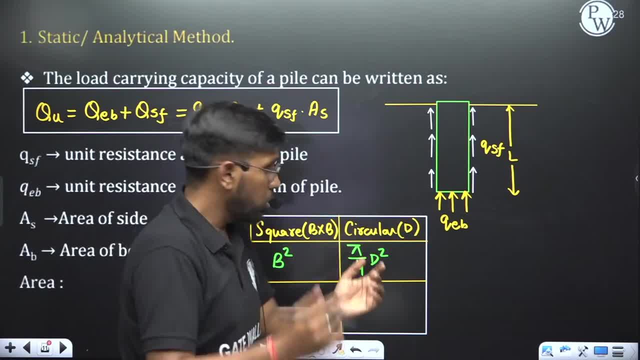 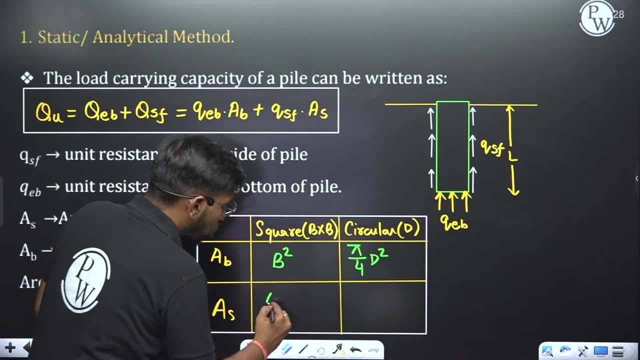 What Area at sides? Side area- What will be the side area? See perimeter. multiply with length. So what will be the perimeter of square 4 times B and this multiply with L, 4 BL. Is it done? 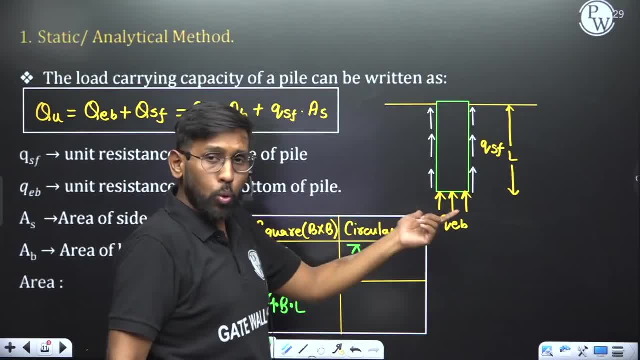 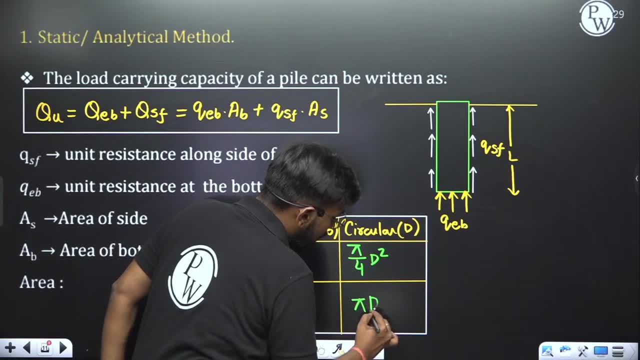 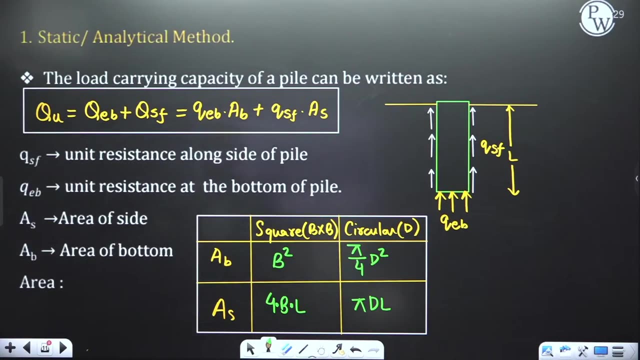 4 BL. Is it done? But if I am taking circular, then what is my circumference? Pi D, and this multiply with L. So Pi D, L. Is it clear to all Arre? he will say: Anyway, Anyone having any doubt, anyone having any doubt, please ask. 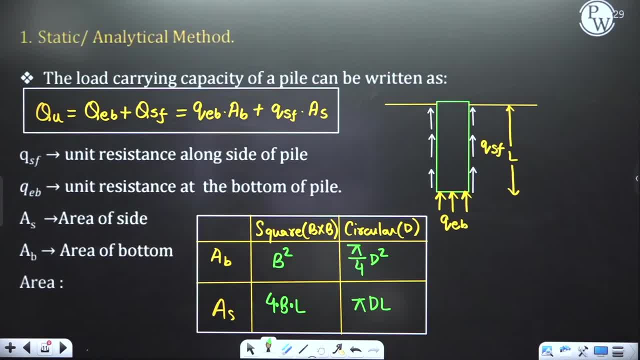 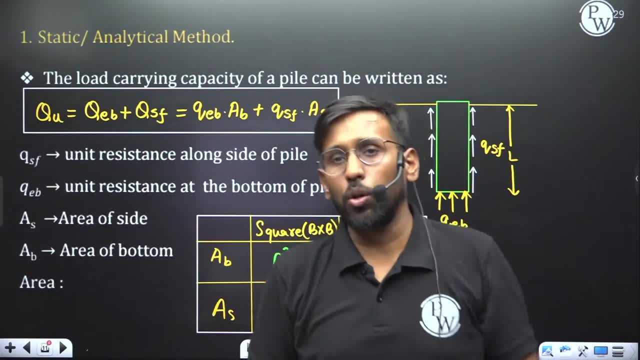 Anyone having any doubt, please ask Clear. You make all these mistakes. You make all these mistakes while coming here. You make all these mistakes while coming here. So now, first of all, we move. Now, first of all, we move, for what? 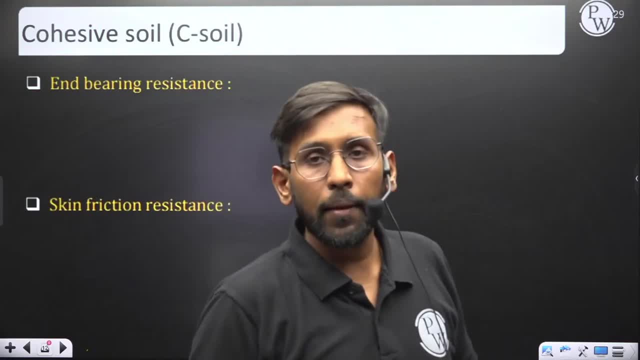 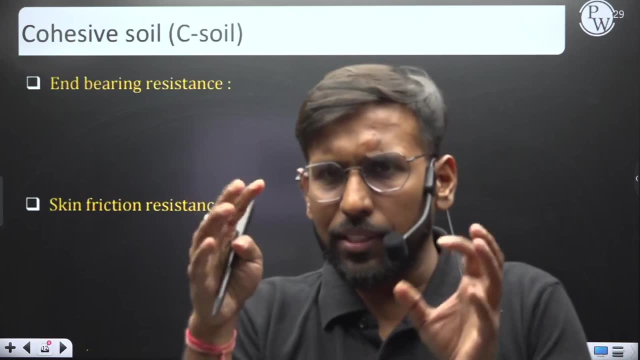 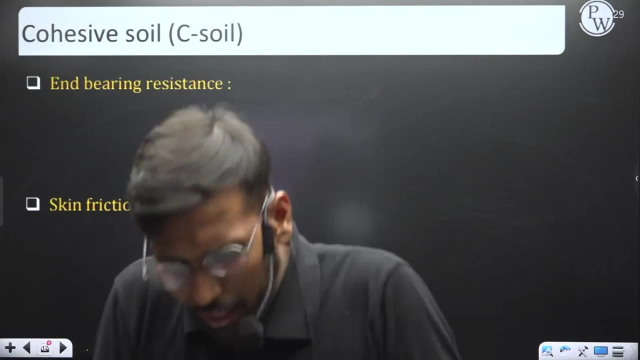 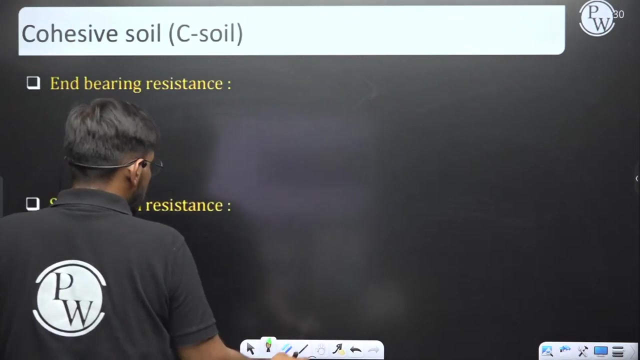 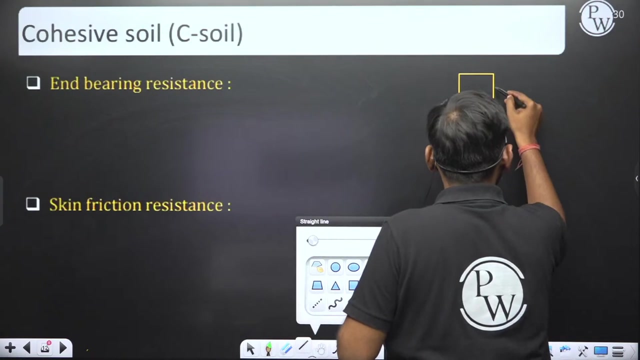 For cohesive soil. Right, Sir, what will be the resistance of soil? Think about it and see If there is a resistance of soil in which the soil will fail in the shear right. So if you are applying load, the pile is trying to go down, then the resistance will come in the shear. yes, listen to me carefully. listen to me carefully. you will understand one thing easily. there is nothing, sir. it is very easy. you have taken a pure cohesive soil. you have taken a pure cohesive soil. you have taken a pure cohesive soil. 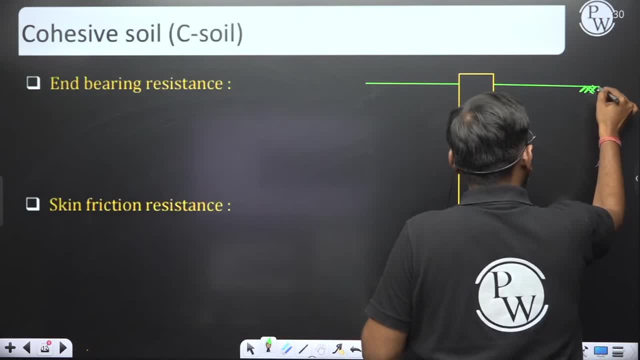 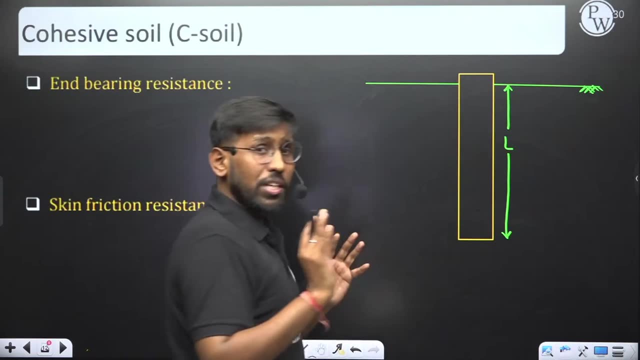 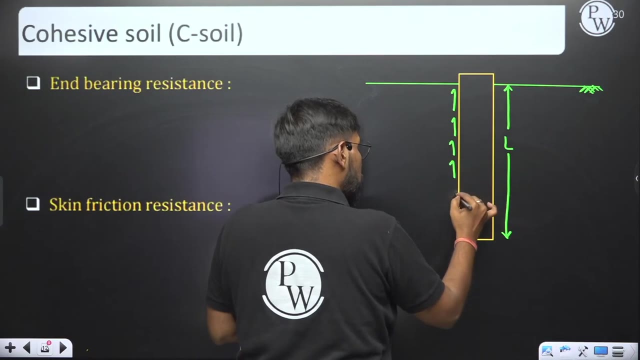 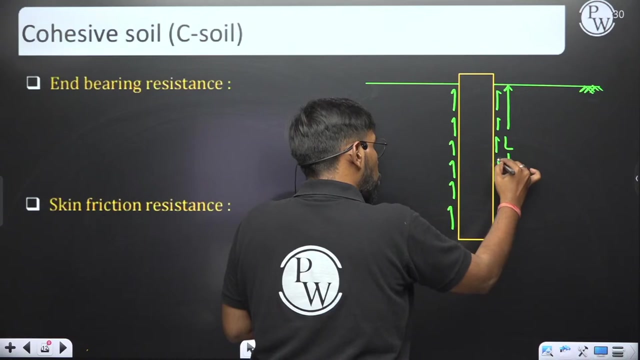 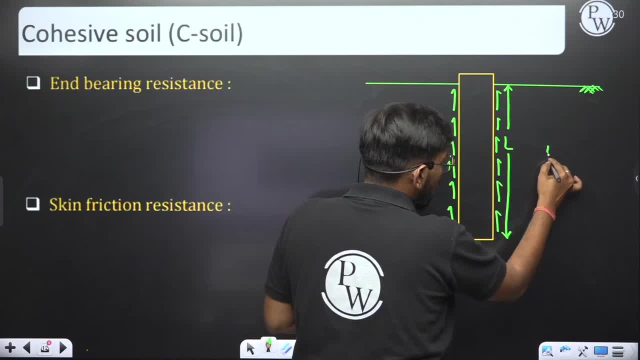 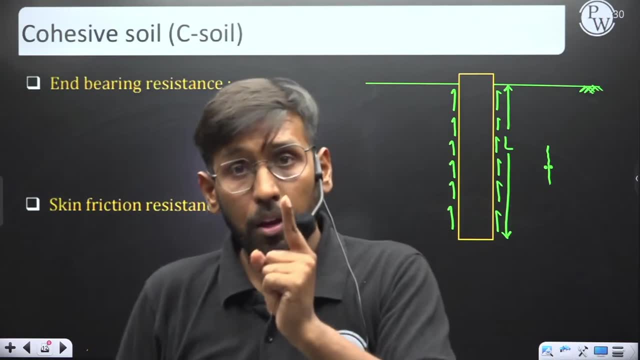 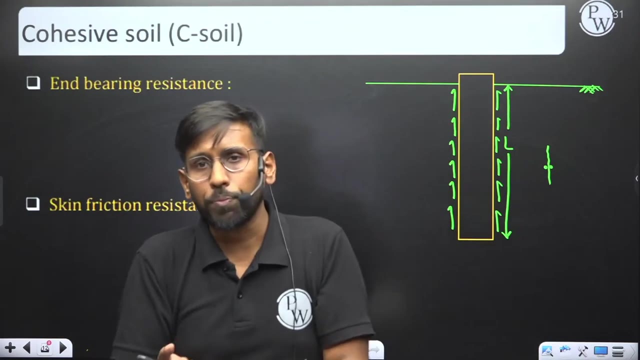 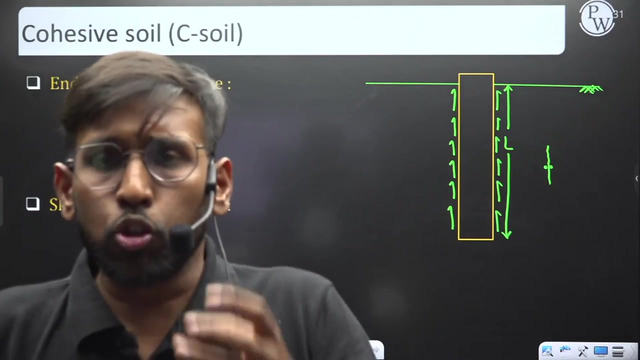 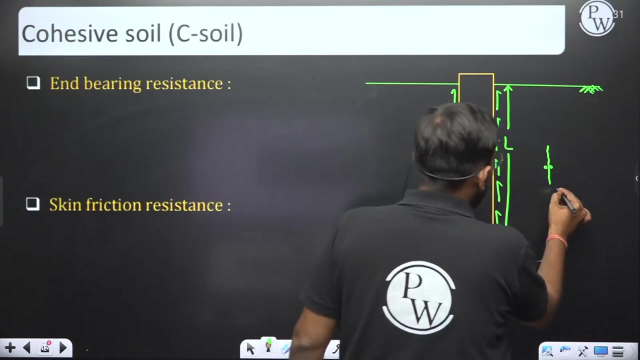 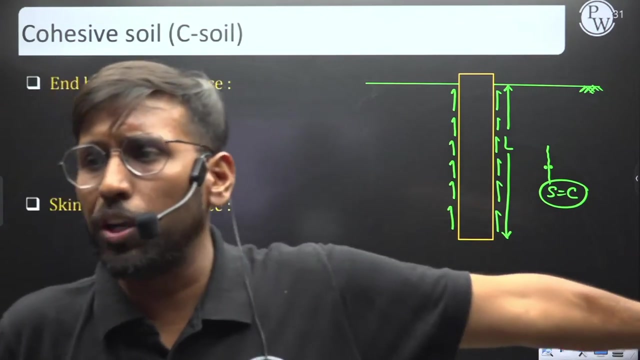 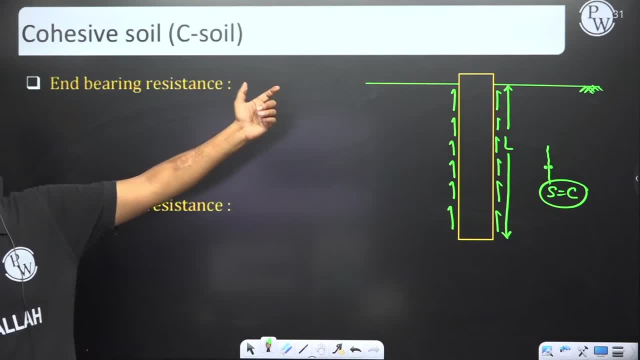 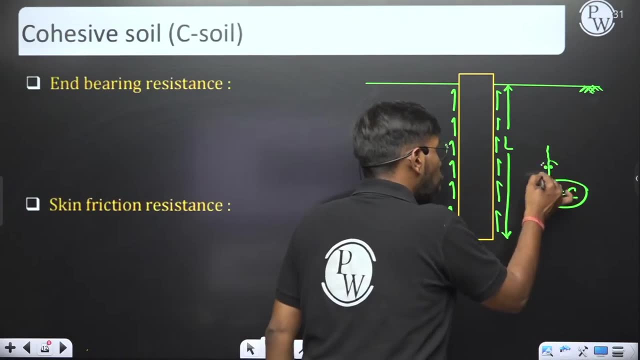 It's a pure cohesive soil, It's a sea soil. So S is equal to C, C is equal to sigma and tan phi Phi is equal to 0 as per our C. But, sir, this which you have got Is between two soil particles. 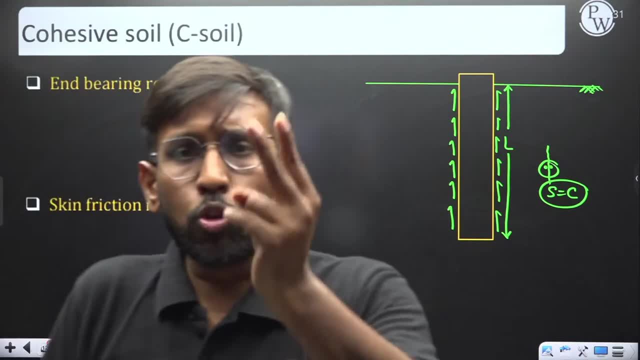 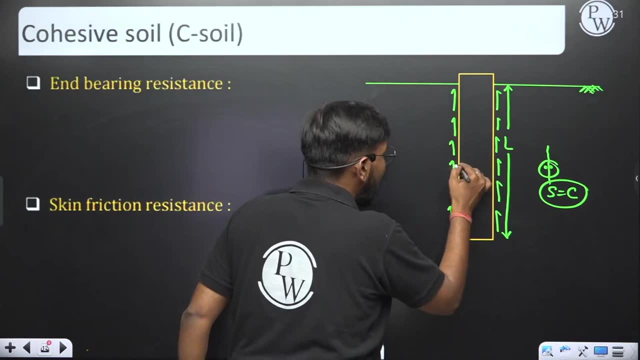 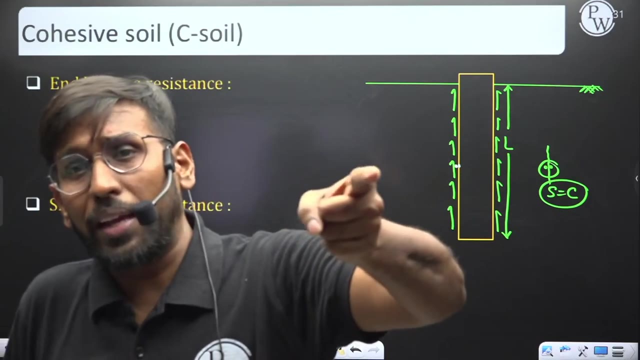 This resistance which you have got Is between two soil particles, But now What we are going to talk about. We are going to talk about between a soil particle And between the pile material. Now what we are going to talk about: Between the soil particle and The pile material. 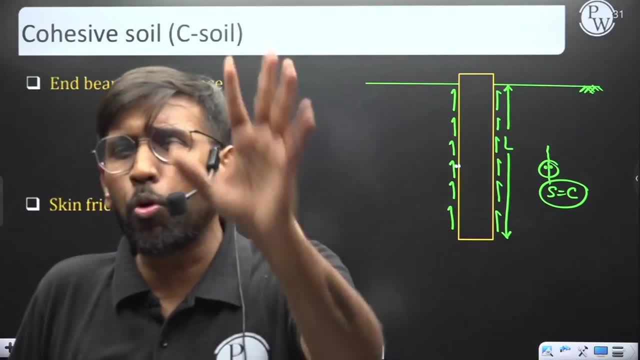 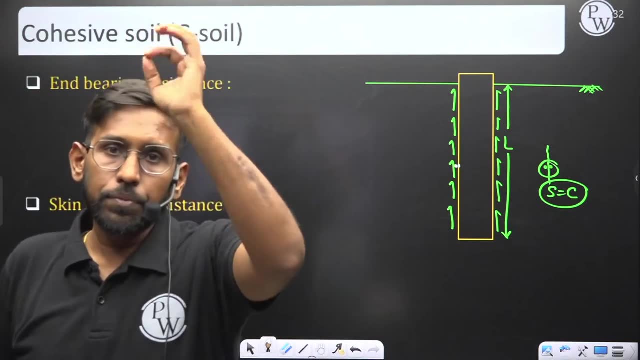 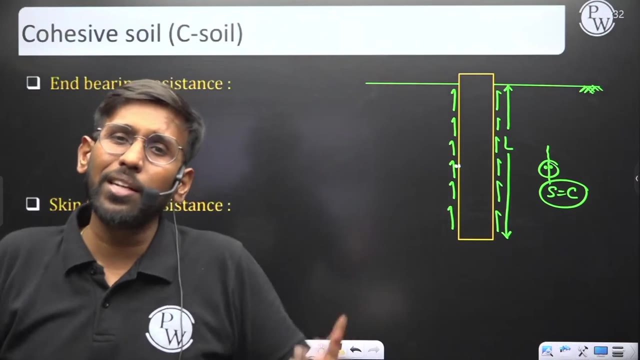 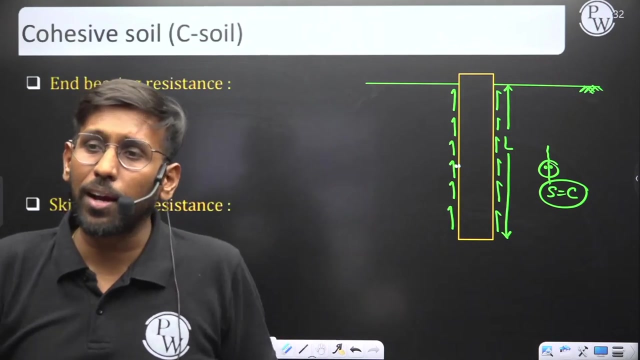 So will that resistance be more or less? Think about it. So will that resistance be more or less? Think about it. Will you get more or less Less? How will you get more? There will be no bonding. There will be no bonding. How will you get more? it will be less. 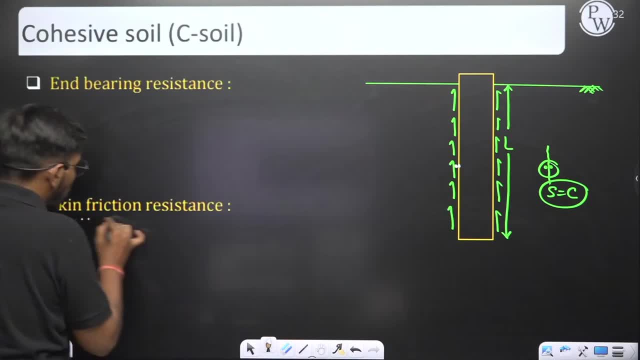 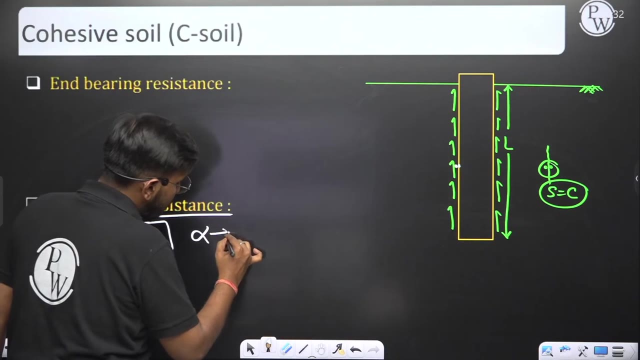 It will be less. So now look here. So first of all, let's talk about QSF. What is QSF? Look what is written here: QSF, QSF, QSF. Alpha into cohesion. This alpha is referred as Addition factor. This alpha is referred as Addition factor. If this was between two soils. 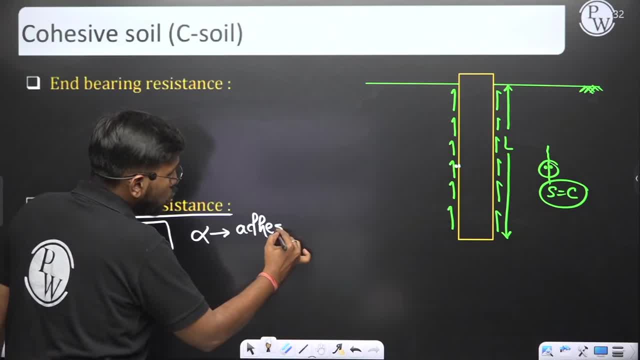 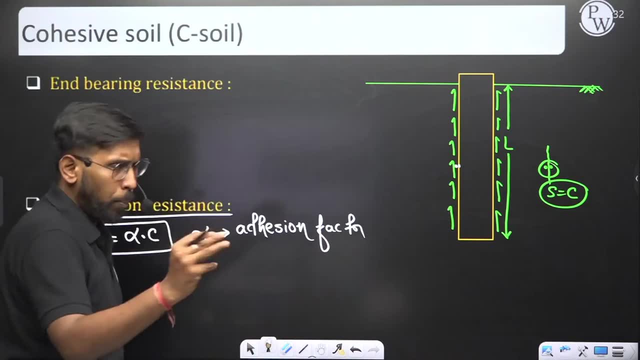 Then what would have been the value of alpha? It would have been one, Because here soil and pile. So what has happened? Alpha's value is less than one You would have been given. in the question I used to write value first. Now there is no requirement for gate. 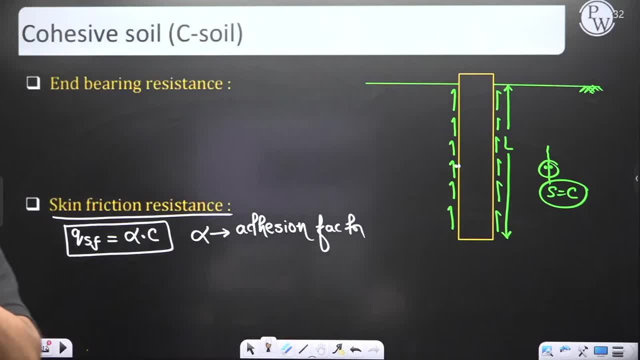 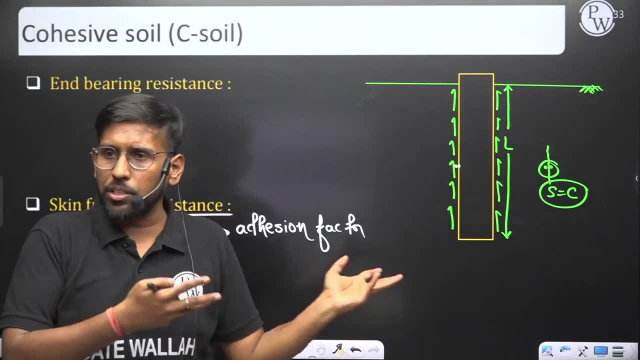 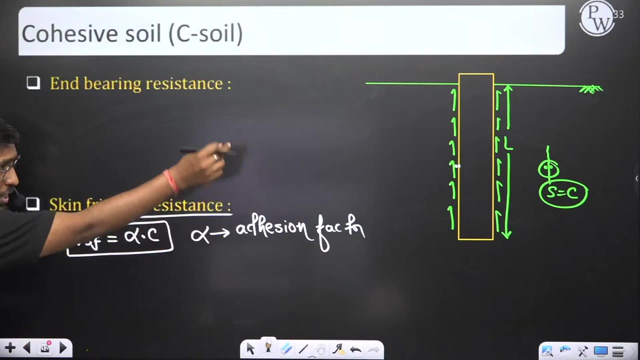 You would have been given in the question. Okay, Okay, Okay, Yes, then the resistance will be less. with the soil pile, Less will be found. End- Look here. Addition factor- Look here. So alpha has become the addition factor To encounter the same thing. This thing has been written. 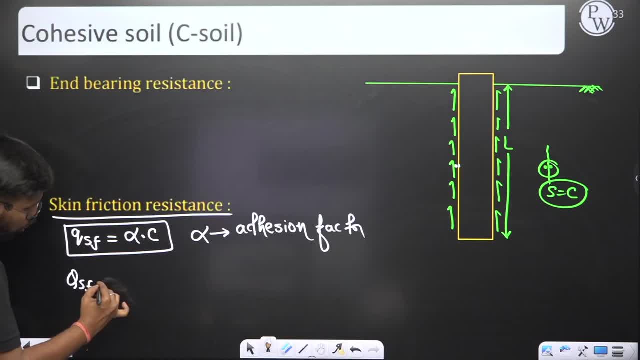 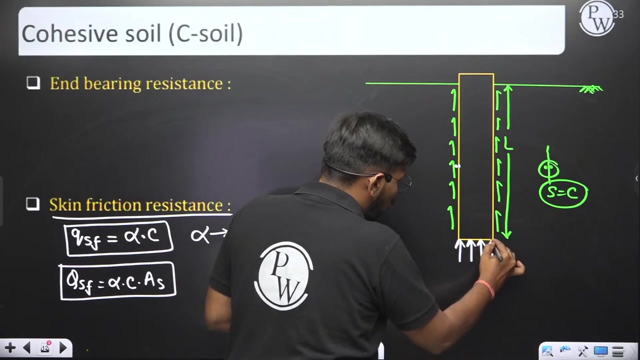 Okay. So if you are writing QSF, So what happened to QSF Alpha into C, into area of sites? Anyone has any doubt here? Anyone has any doubt here? Forget it Now, my friends. Now, if we talk about the bottom. So we said The mayor of theory is the most generalized theory. 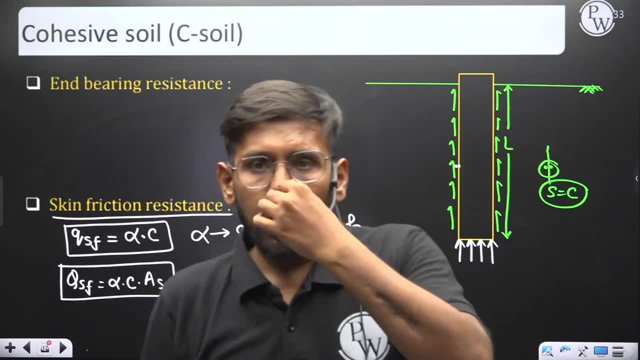 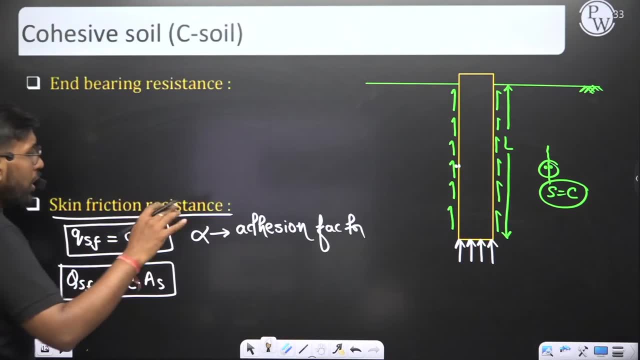 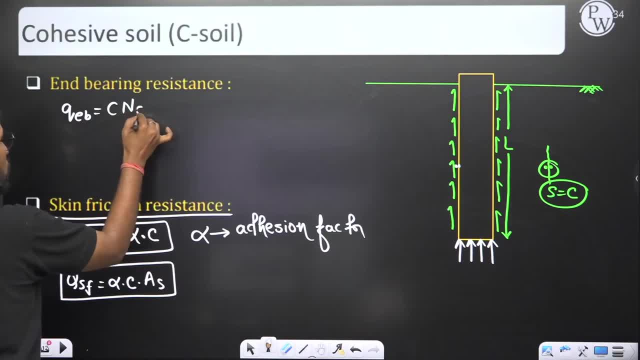 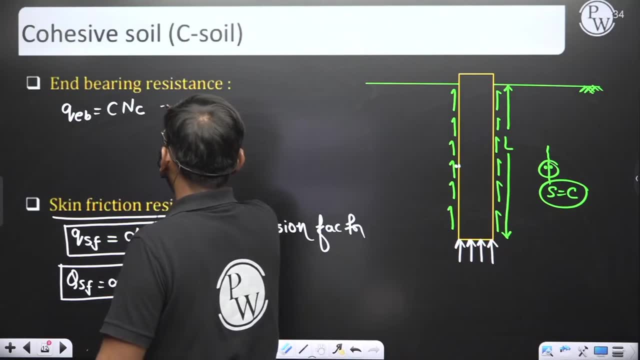 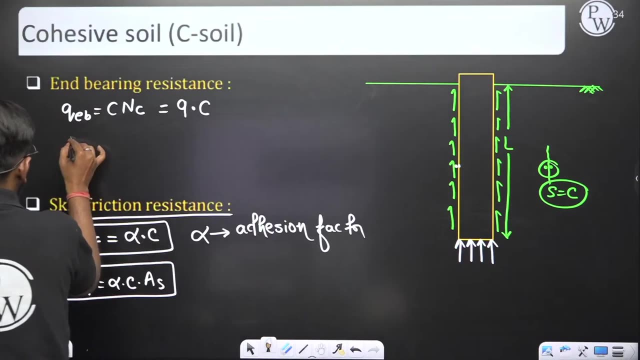 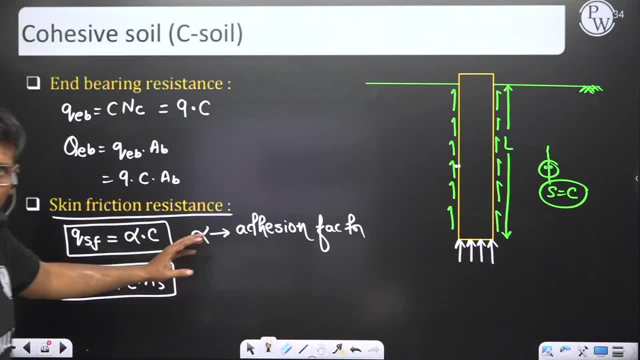 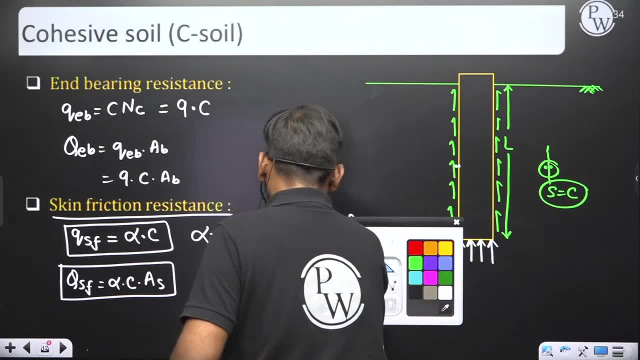 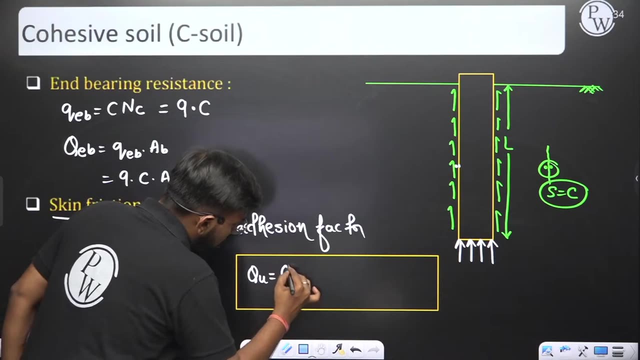 Okay, now, if I understood this thing till here. now, if I understood this thing till here, then, sir, if I had to find ultimate load carrying capacity- see here Q ultimate- then what did we say? Q end bearing plus Q side friction. 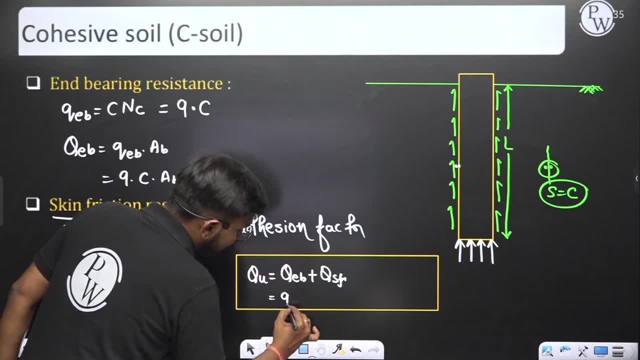 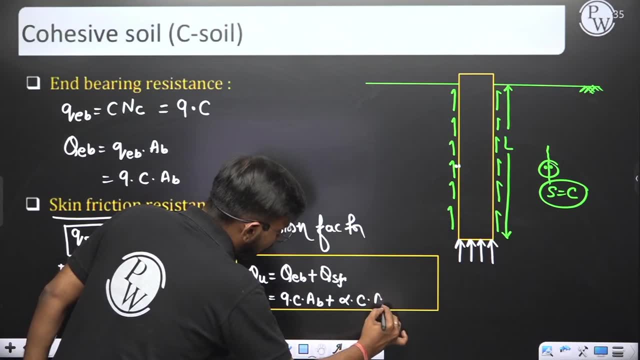 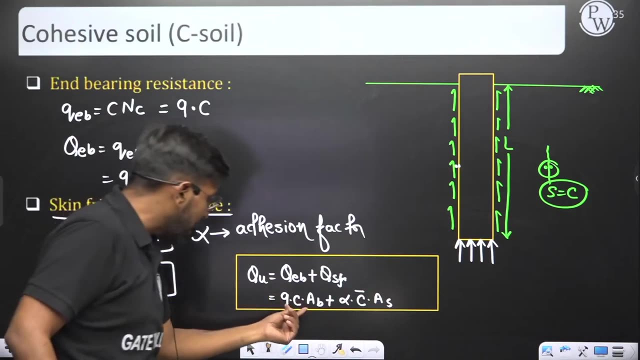 now, we said this only so what happened, my friend? 9CAB plus αCAS. So now let's do one thing: let's give it C bar, so that we can understand the difference. Now, this cohesion and the second cohesion. 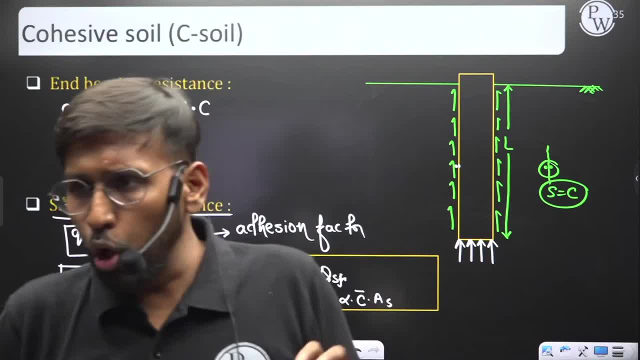 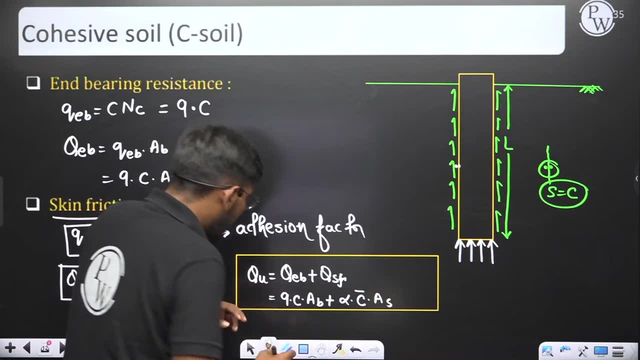 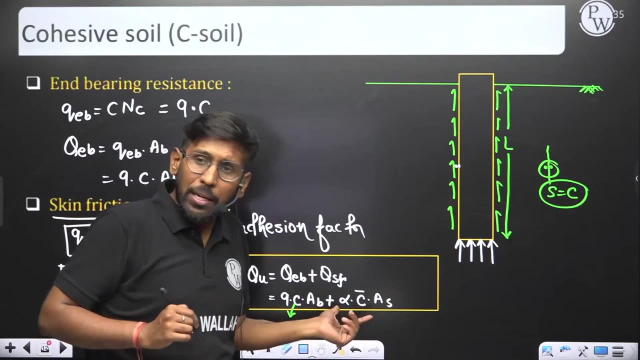 there is difference between both These two cohesion. these two are difference. Did you understand this carefully? Now, if we are talking about the first cohesion, then we have to understand that. where is the first cohesion, This 9CAB, written? where is this cohesion? 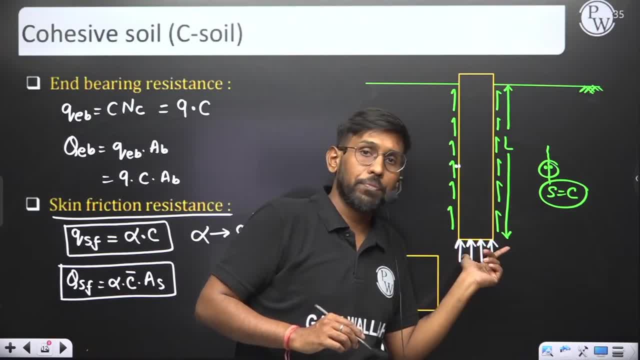 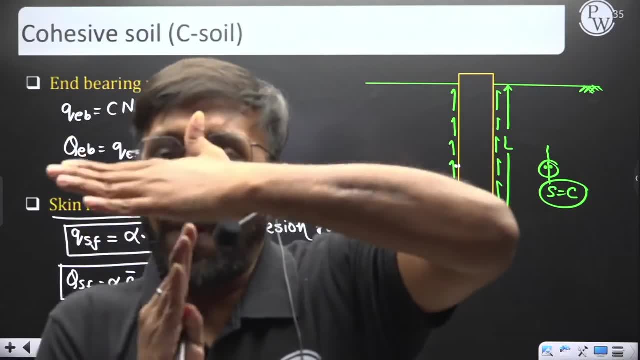 This cohesion is at the bottom, The bottom of the pile, the bottom level of the pile, because you are talking about the end bearing, so the bottom level of the pile, we are talking about that. It is important to understand all this. this is what you get lost. 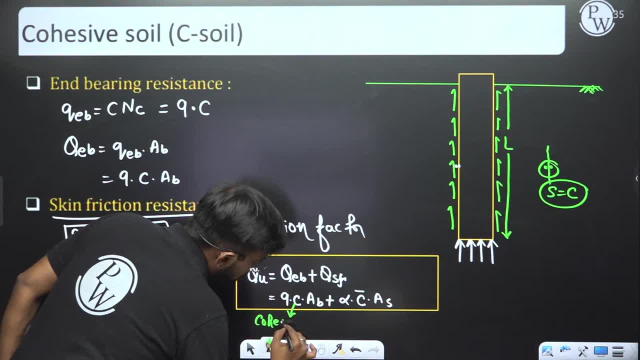 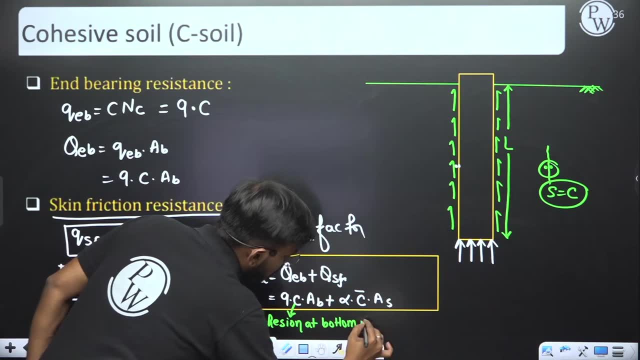 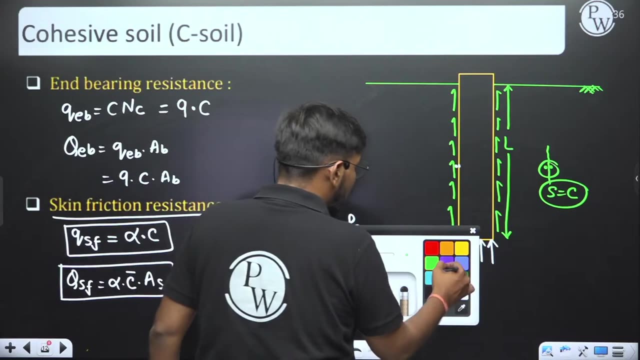 Cohesion at the cohesion at bottom of the pile. Is this clear Cohesion at the bottom of the pile? Okay, And this C bar which you have written. what is this C bar, This C bar which you have written? 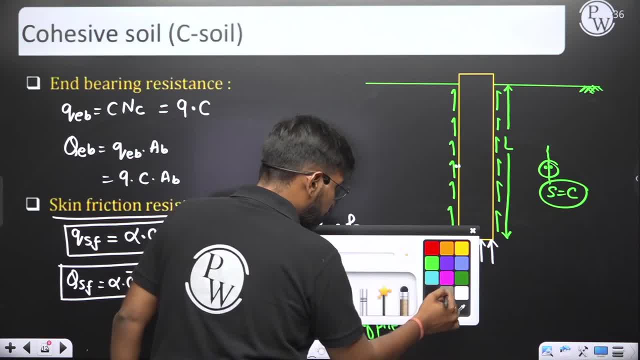 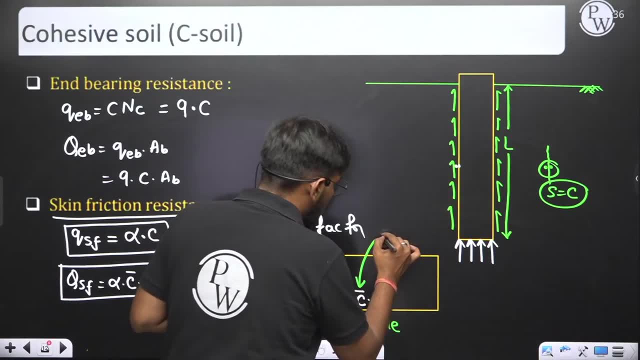 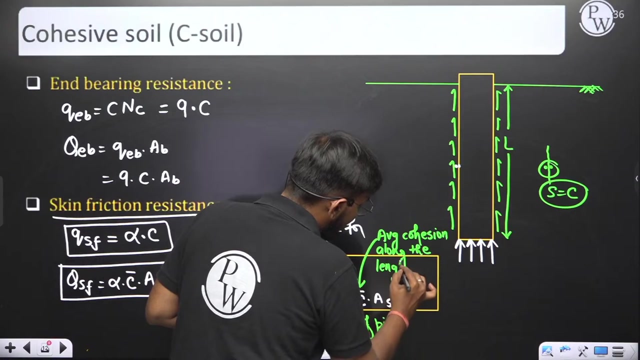 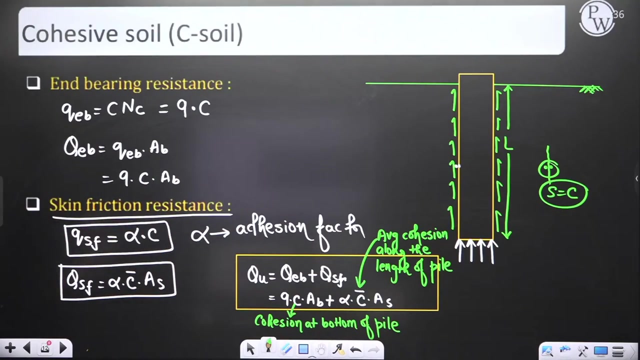 what is this C bar? Yes, sir, This C bar is the average cohesion. Listen to me carefully: Average cohesion, cohesion along the length of pile, along the length of pile. Is there any doubt? This is the average cohesion along the length of the pile. 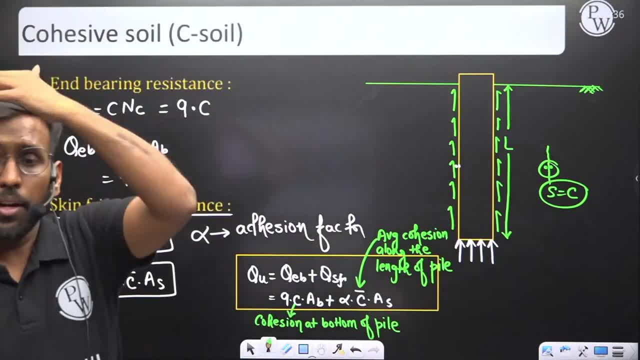 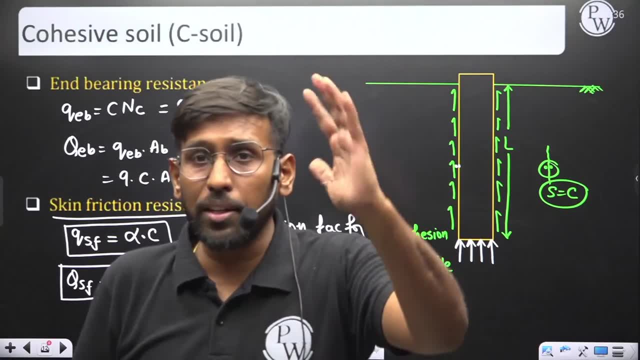 Now let's see how he can ask you a question. Did you see, Did you understand how he can use the average cohesion? Will you say, my friend, Do you want to know how to use the average cohesion? Tell me How many people want to understand. 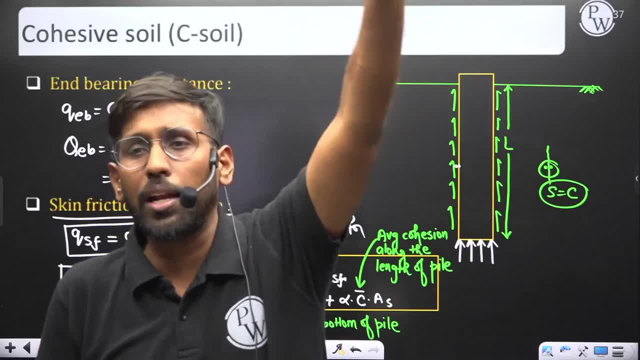 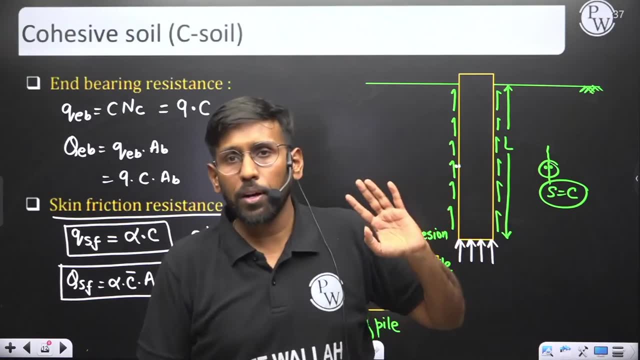 Sir, he wrote the average cohesion, but how will he ask the average cohesion, Sir? this will be given in the data Area. bottom will be given in the data. Everything will be given in the data. Yes, sir, This is the Meyerhof constant. 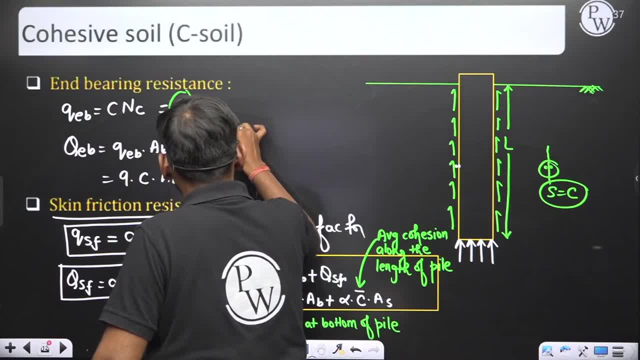 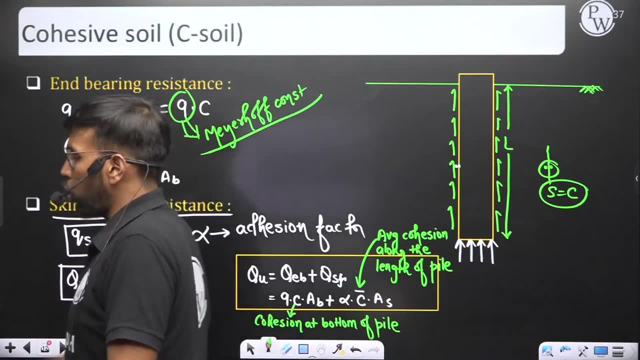 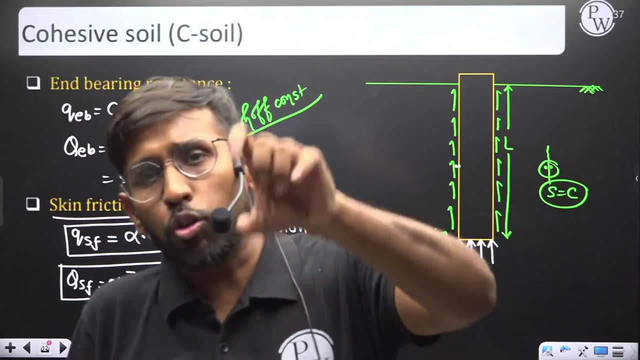 son, This is your Meyerhof constant. It has come from there. And greater depth, Meyerhof sir, has found shallow. This was your 5.7 for the foundation, But if you go deep, then the value changes. Yes, brother. 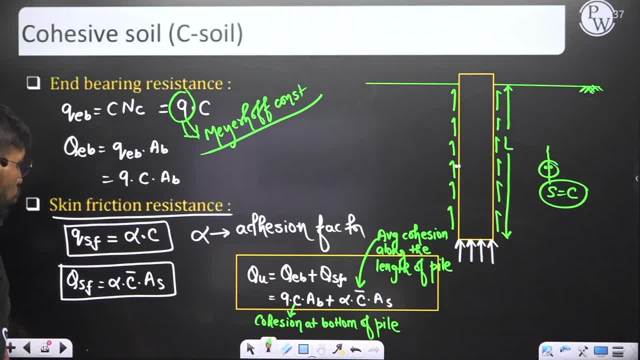 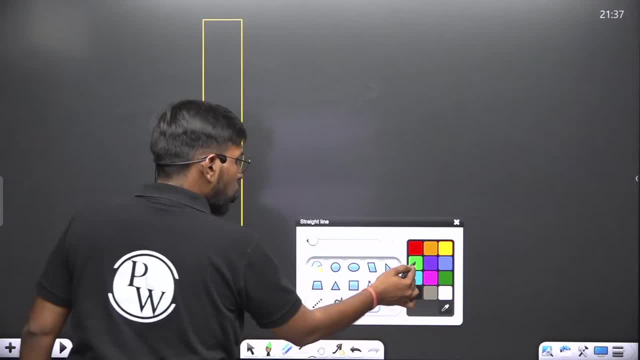 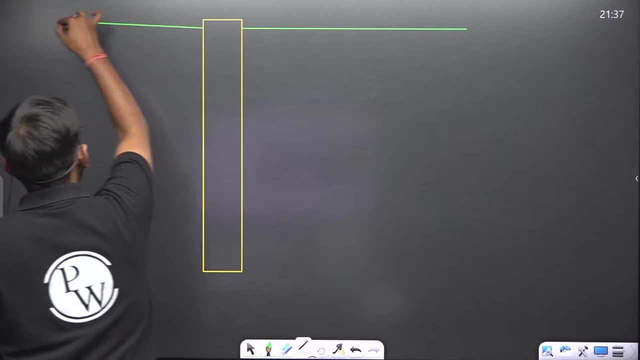 Look here. So, my friend, let's assume there is a situation. Let's assume there is a situation. Let's assume there is a situation. Focus and listen, sir. Life will be very easy. Foundation engineering is very easy, provided you understand the concept. 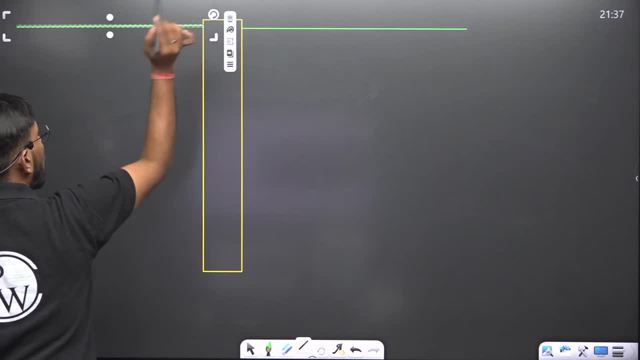 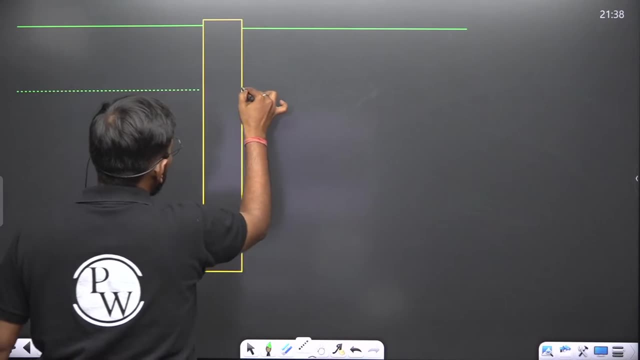 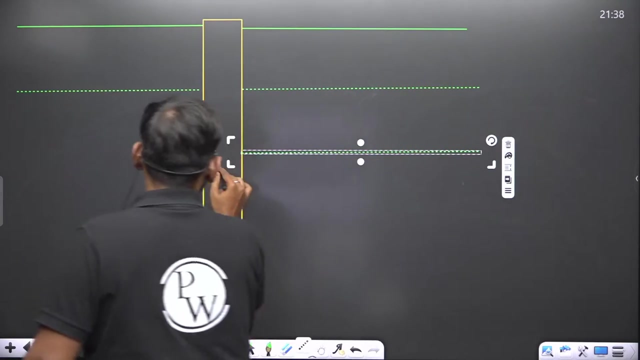 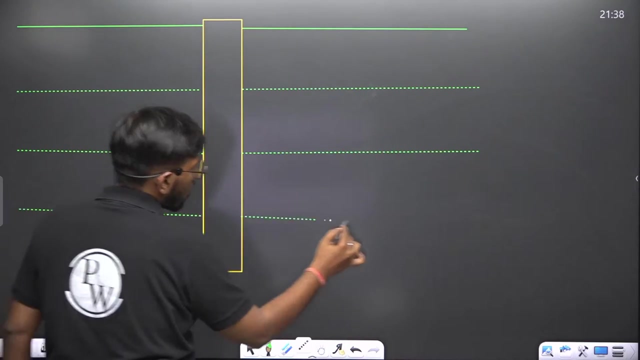 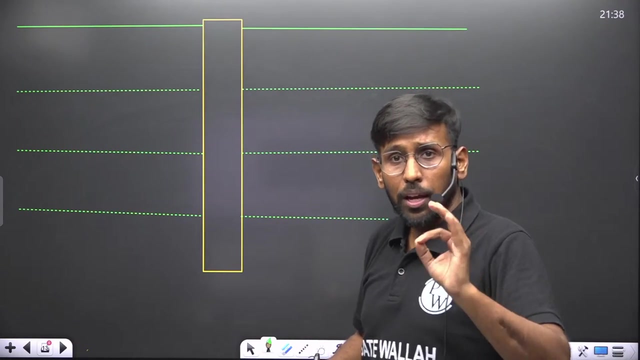 and not just focus on the remembrance of the formula, Because those who work on the formula, they just work on the formula, They live on the formula Life never moves forward, See here. 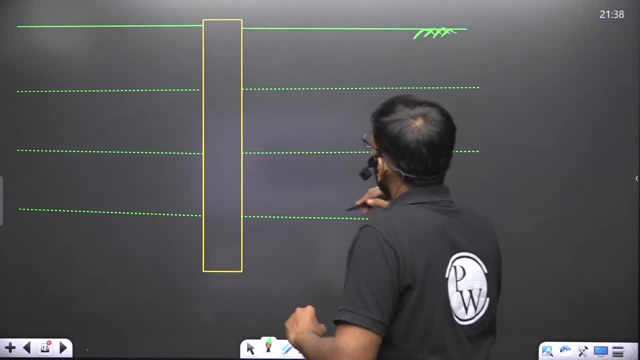 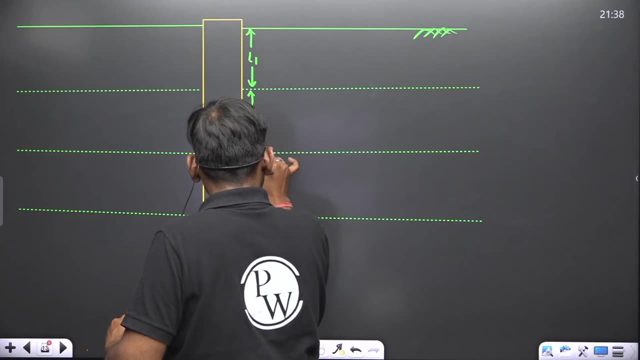 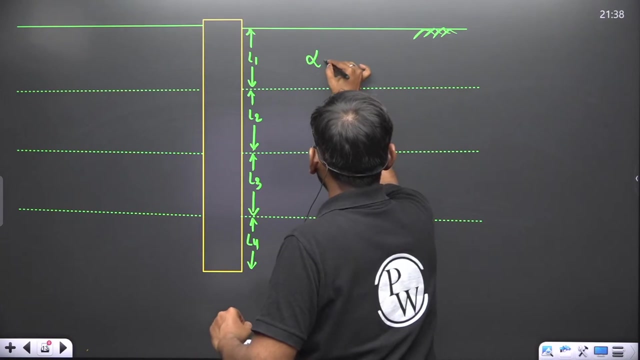 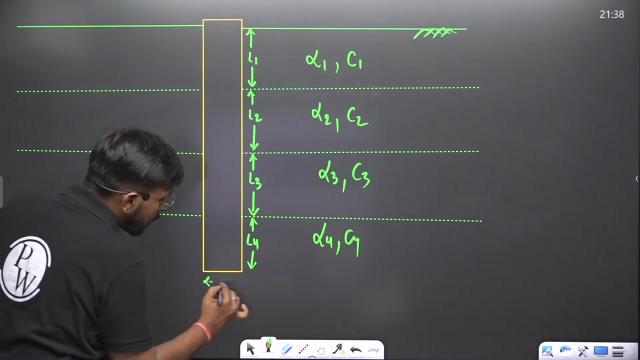 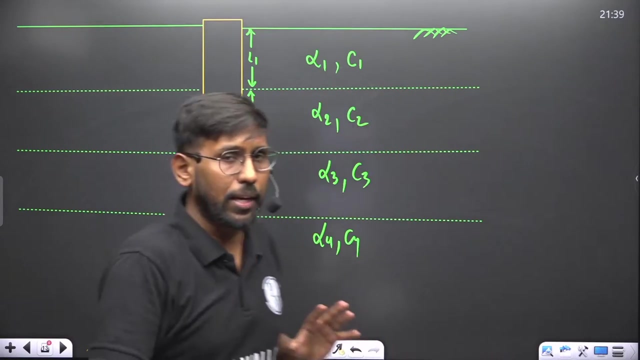 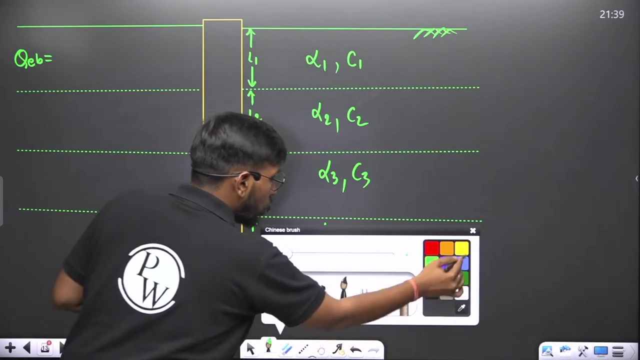 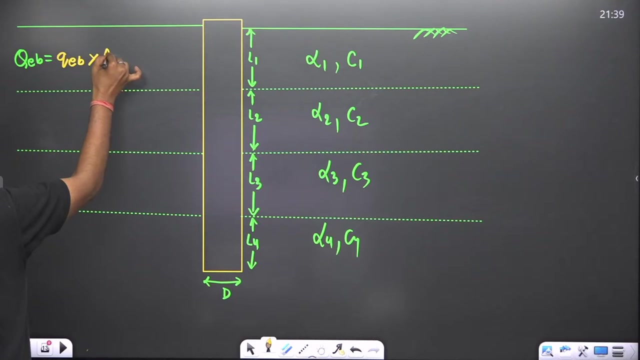 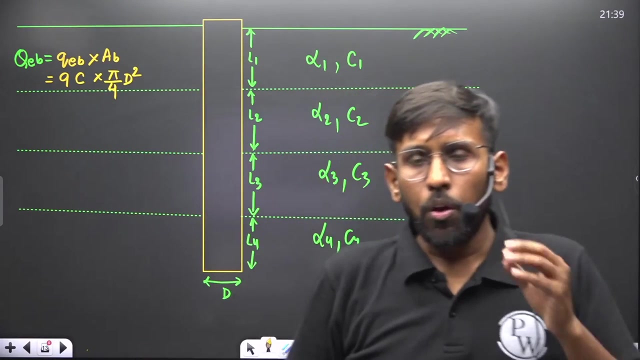 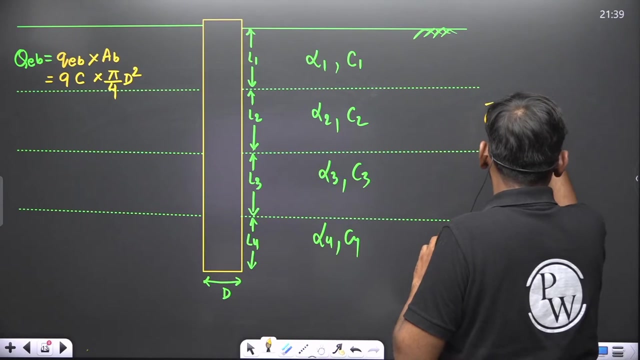 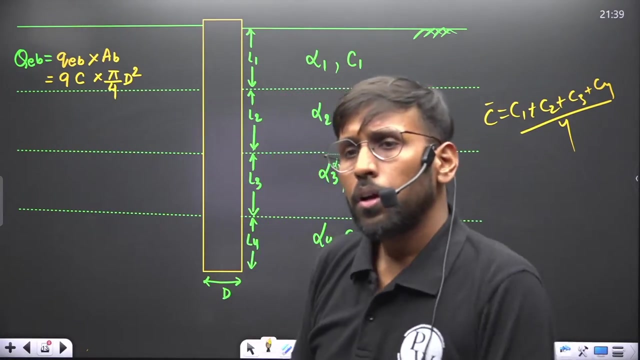 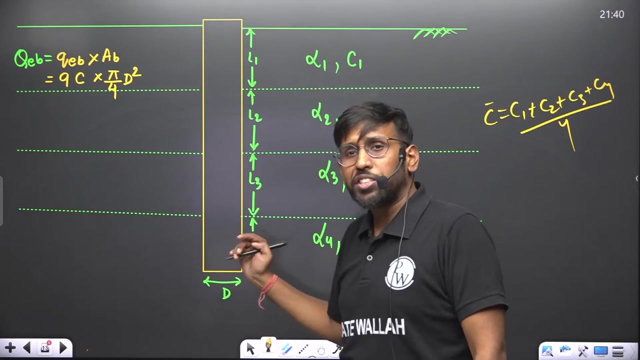 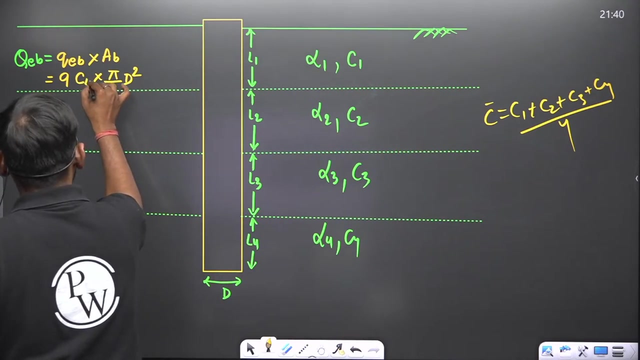 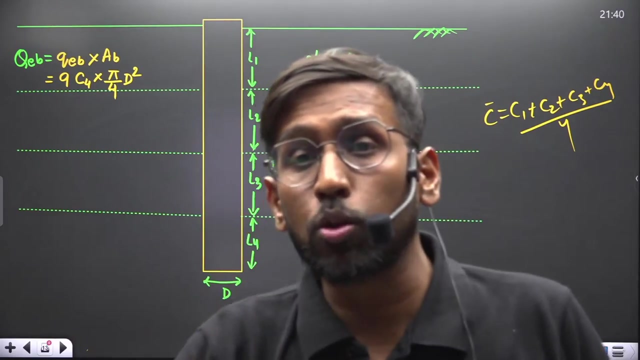 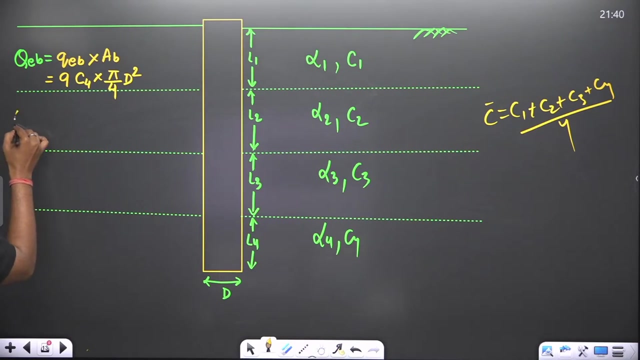 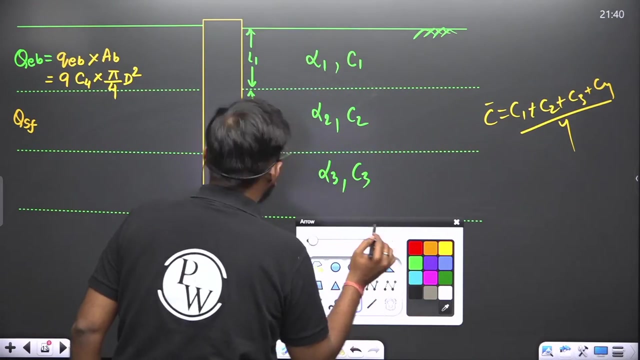 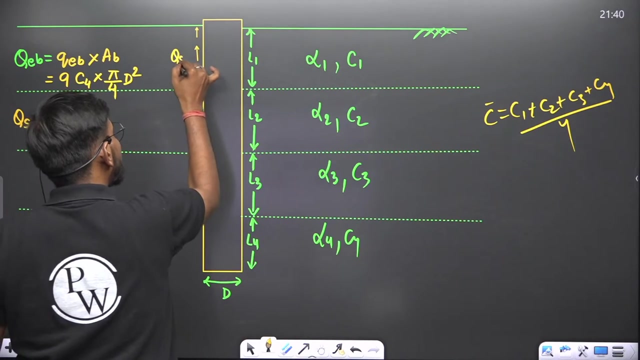 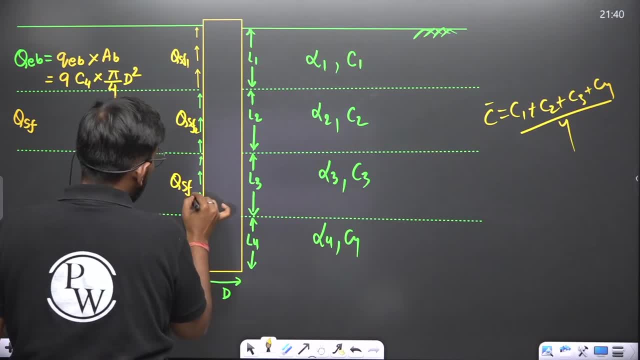 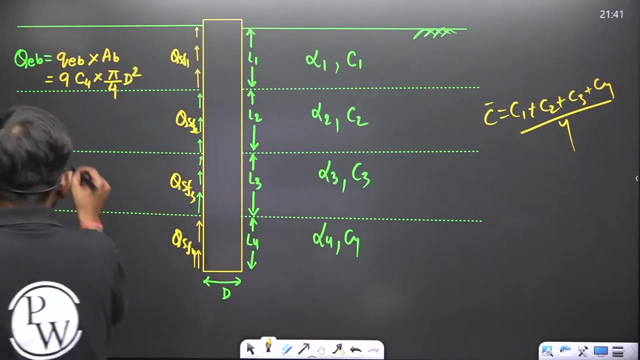 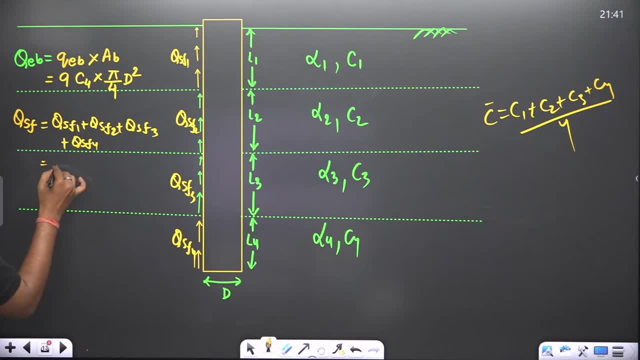 what will happen If we talk one by one? then α1, C1, and what will happen to AS1?? What is AS1? It is nothing but π into D into L1 plus QSF2. what happened? α2, C2 into π, into. 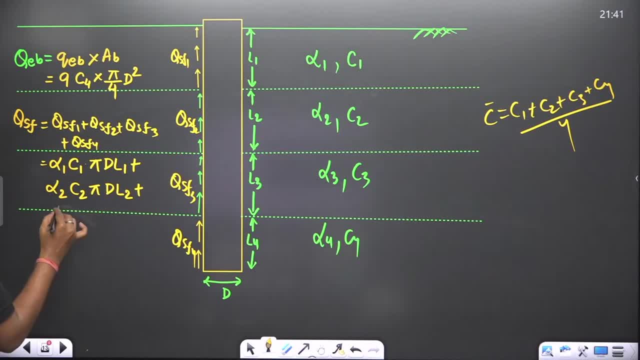 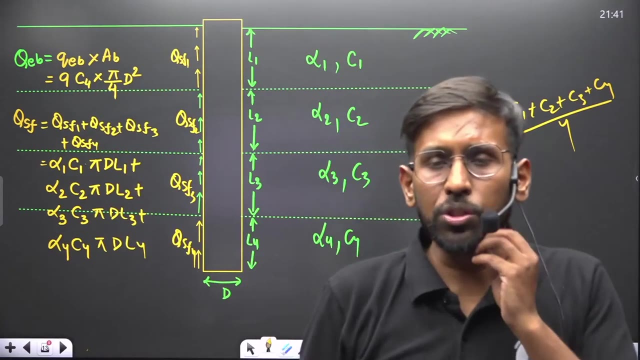 D into L2 plus QSF3. what happened? α3- C3 into π D, L3 plus QSF4? what happened? α4, C4, π D, L4.. Sir, what is there in this? What is there in this? Tell me, What is there in? 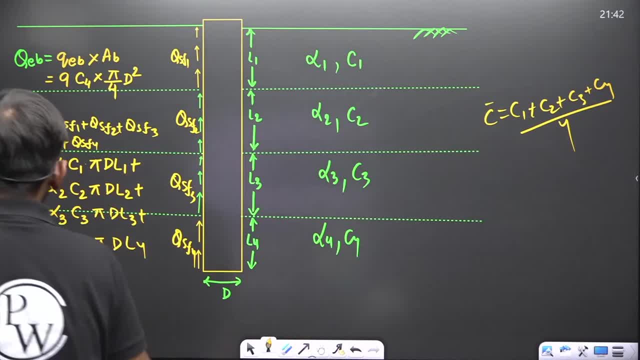 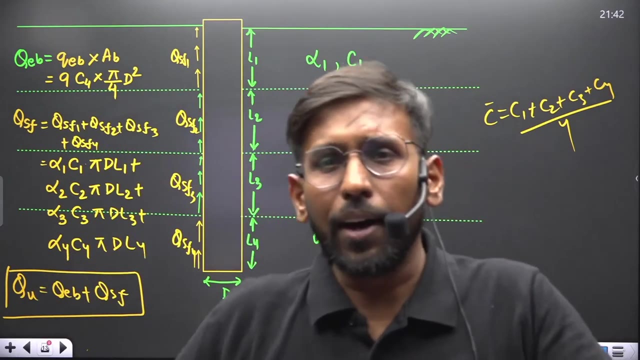 this, Will you tell me? And what did you do in the final? What did you do in the final? Q ultimate is equal to Q end, bearing plus Q side friction. What is the answer? Is it clear? Is it clear? It is easy, right? There is nothing. You have to apply the formula. 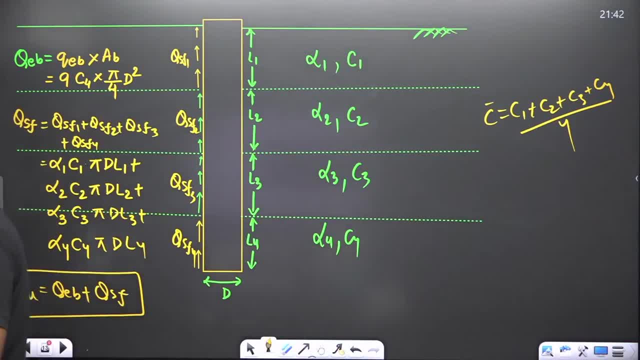 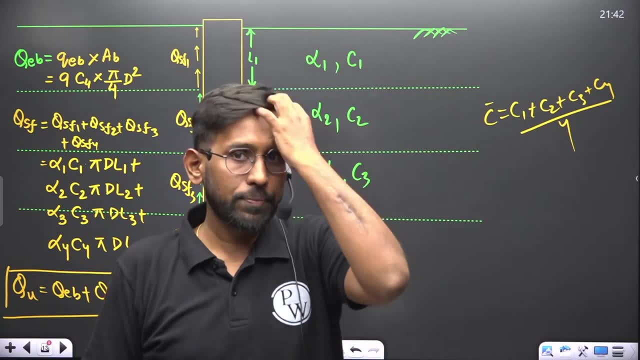 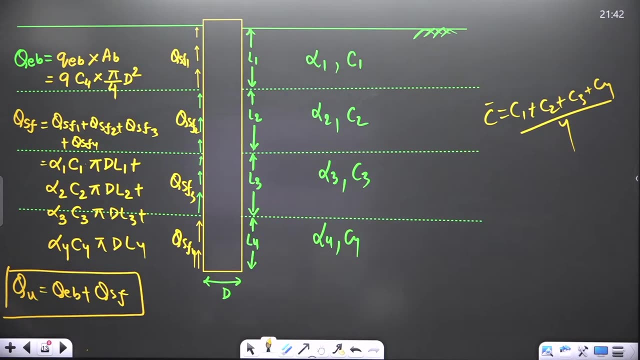 properly. That is not what happens to you. That is the problem. Did you understand? Is the point clear? Is the point clear? Is the point clear? Yes, everyone is clear. Come on. Good, good, good, good, good. So now let us move to the next In this. if the lambda is: 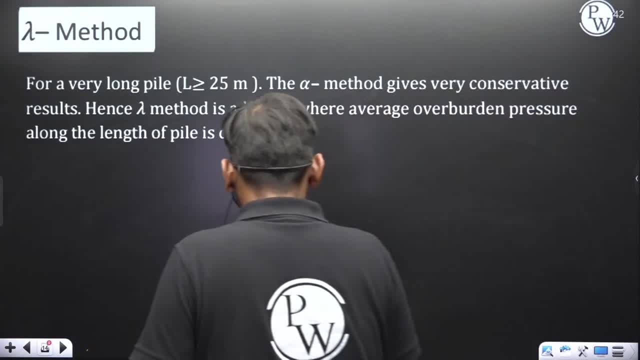 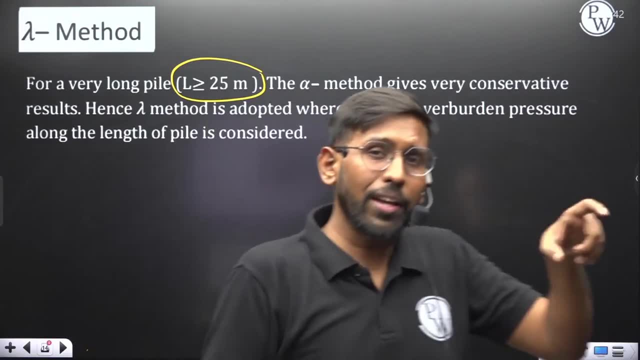 also a long pile. in that case you cannot remove it And the time is over. If the grate has a long file, You can think of it one. So in theüst 2 cases he has y Deutsch here in the middle he will have one geet, Which means he. 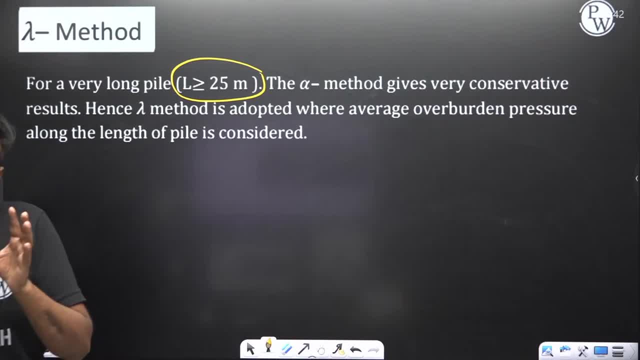 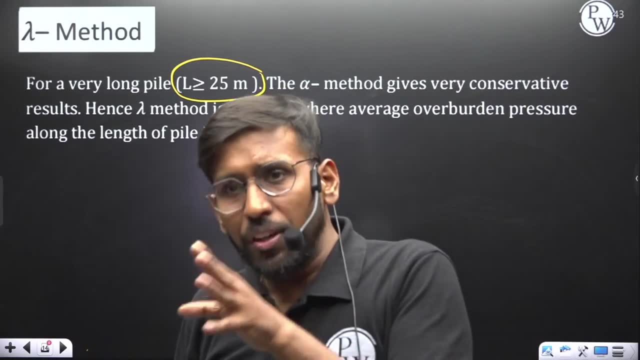 cannot remove it. If the gate on the GT is also long, then data location in this case is two per 1.. Same thing with the gate He can blanket without any doubt. Theeman used the lamda method. What is the method? What is the method鋷? m uncover it in this case. 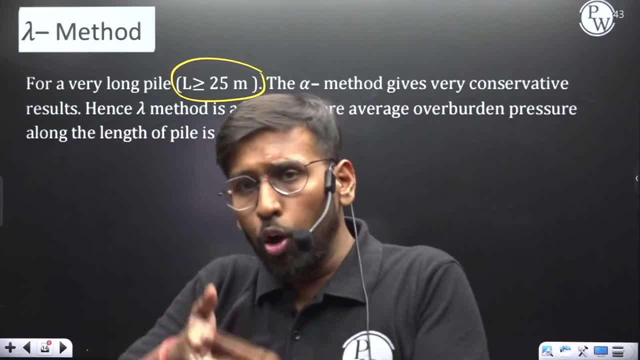 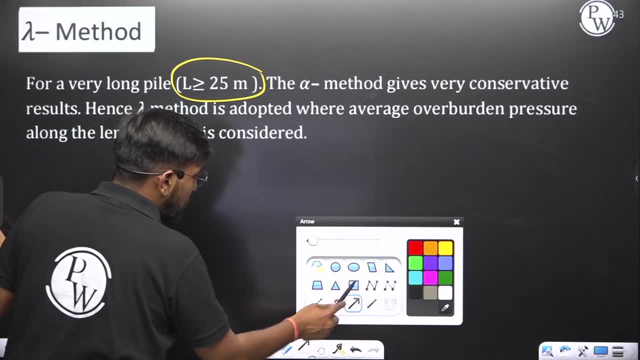 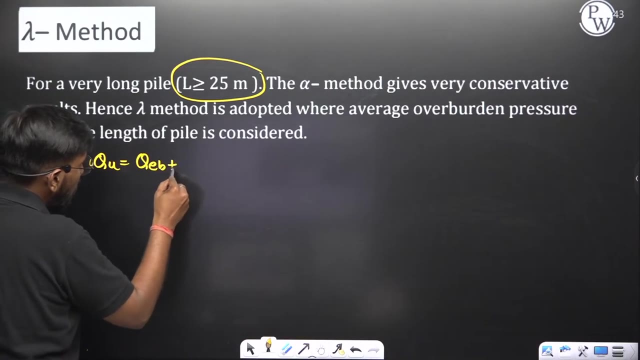 Means you are saying that its load carrying capacity is less, But if it is a long pile, then its load carrying capacity is considered to be more. So how is all this? This is all your experimental data which is given. So what it says is that Q ultimate is Q end bearing plus Q side friction. 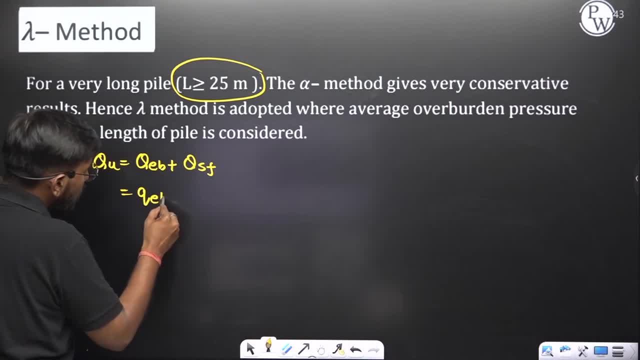 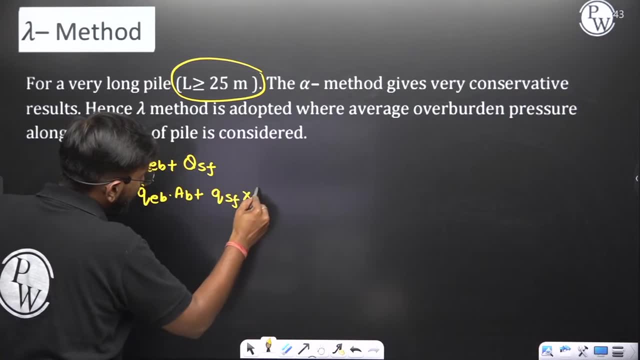 So what is end bearing QEB into area bottom? What is Q side friction? What are you writing? Sides, frictional resistance multiplied with area at sides. This is what you are writing. So see, everything is coming same. 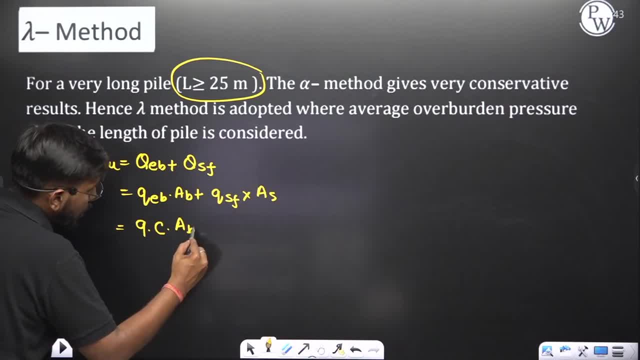 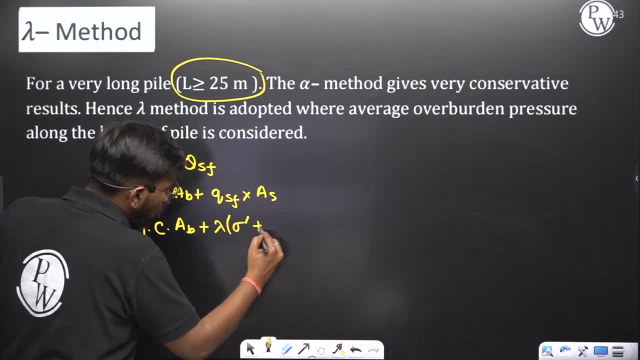 Where is the difference? Understand? 9 CAB is also clear. Here term will come as lambda. Lambda, Effective stress plus 2 times cohesion multiplied with AS, Multiplied with AS. So this is written here, In which case, 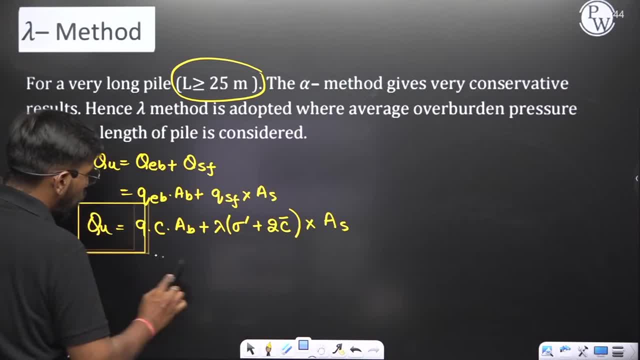 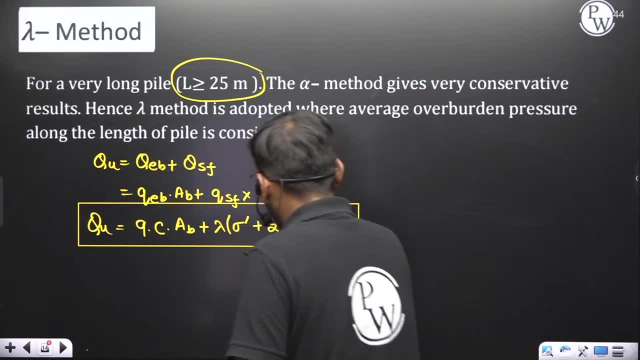 For the case of the long pile. For the case of the long pile, Now you will understand the difference here. Rest, everything is same. Rest, everything is same. The difference comes on lambda. Lambda is a constant. This will be given in the question. 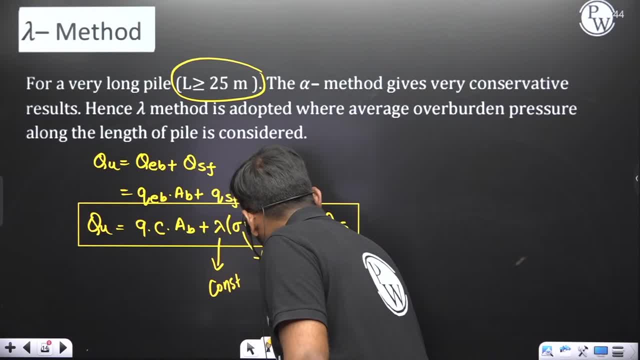 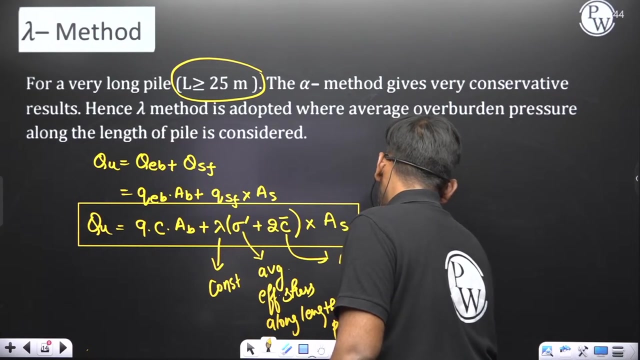 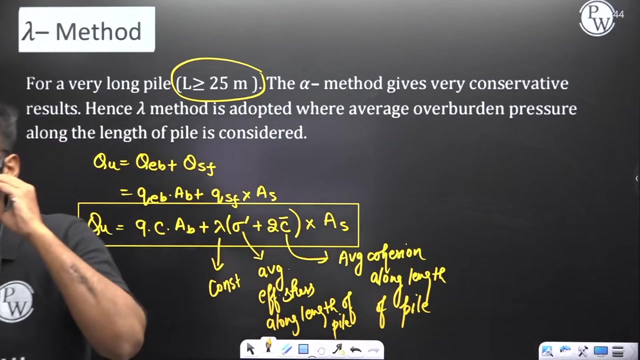 Lambda is a constant, Sigma bar is the average effective stress along length of pile Along, length of pile, And C bar is the average cohesion along length of pile Along, length of pile. So, sir, now what is the difference here? 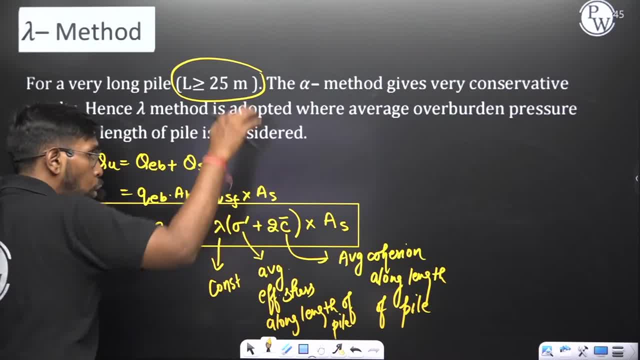 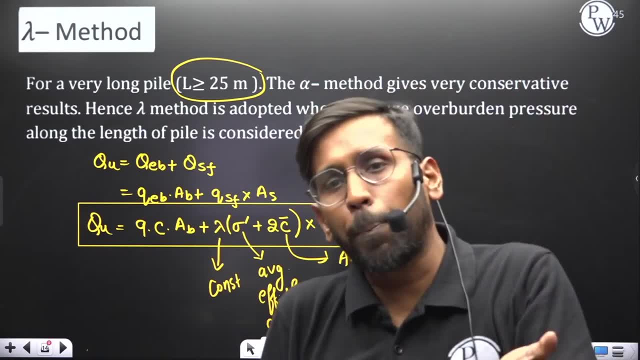 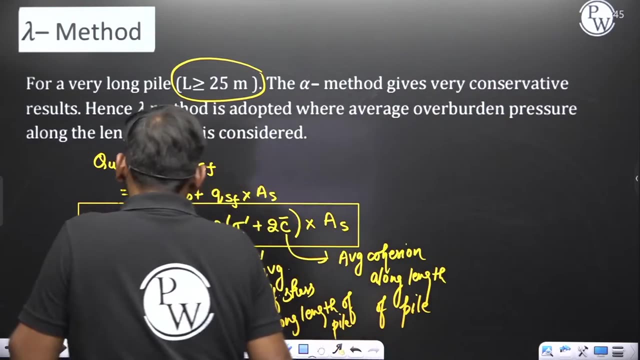 The difference is that here the overburden pressure is also included, Okay, Okay, So you have included the overburden pressure along the length of the pile, Because of which my load carrying capacity is coming more, Because of which my load carrying capacity is coming more. 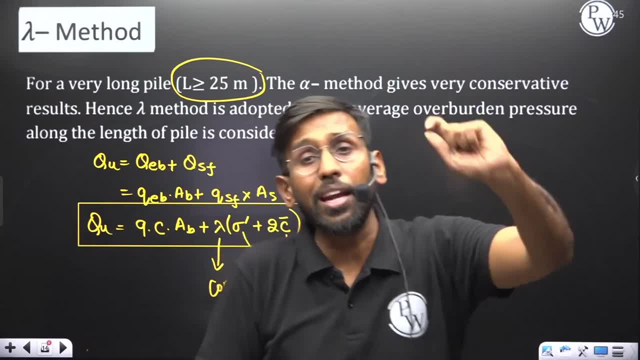 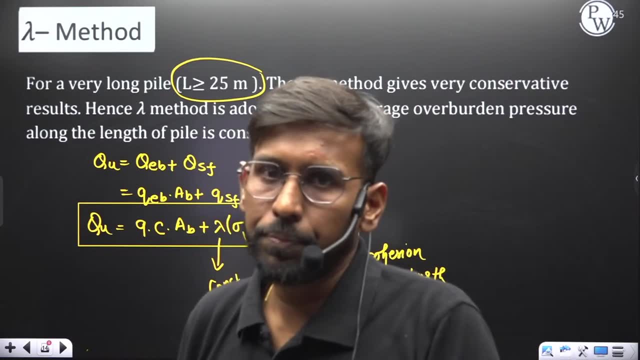 So when should we use this? When it is written in the question that long pile, When the lambda method is mentioned in the question, then only you should use it, Otherwise you should not use it. Clear: If the lambda method is used in the question, then only you should use it. 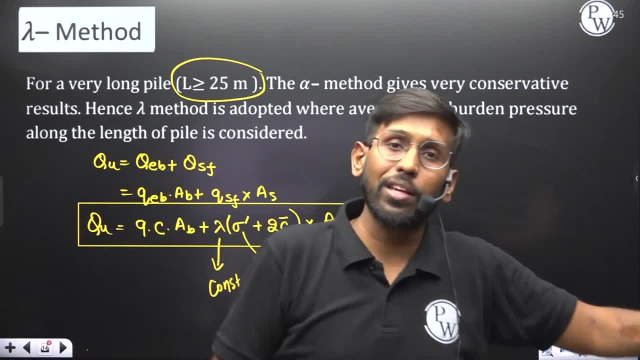 Otherwise you should not use it. Okay, apne jo pehle padha tha wahi karna hai for the cohesive soil. Okay, Tariqa, kya hoga? Tariqa, kya hoga, Dekho, yaar pe. 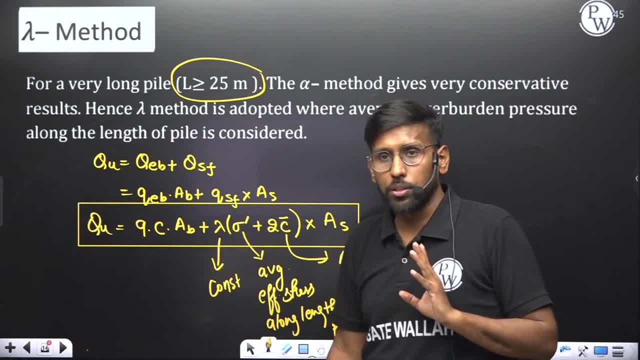 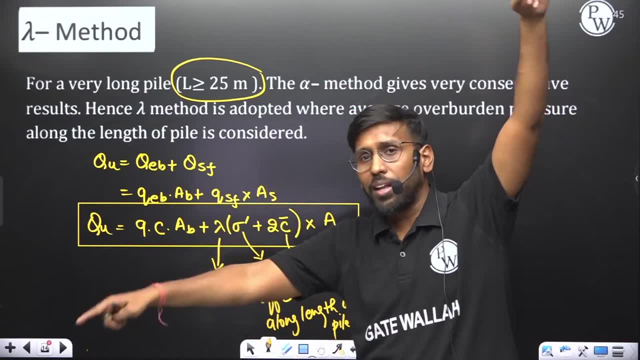 What will be the way of solving this? What will be the way of solving this? Focus karenge, Agar aapko jaisa sigma ka baat kar raha hai, effective stress linear vary kar raha hai. 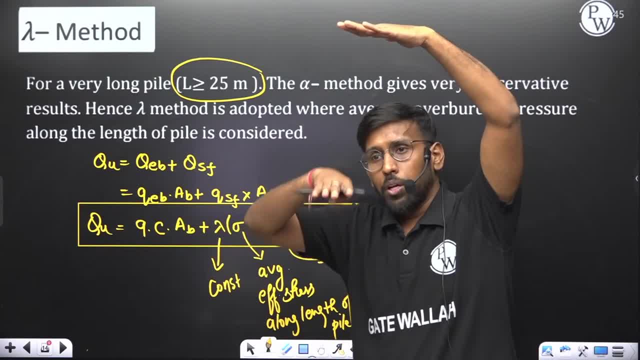 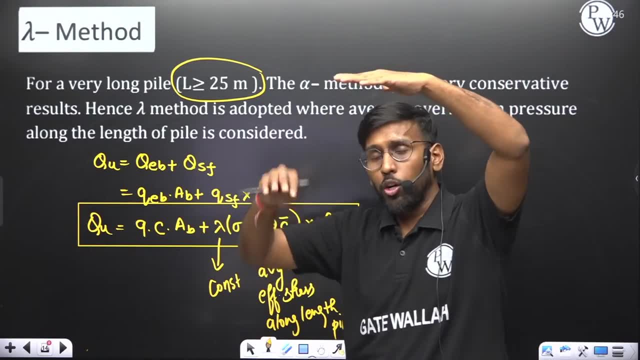 toh aapka zero wale point se leke pehle layer pe zero wale point se pehle layer pe something plus zero by two. Aage bade something plus something by two. Samajh ho na. 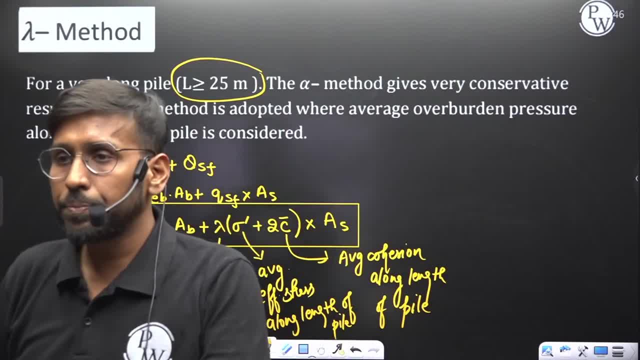 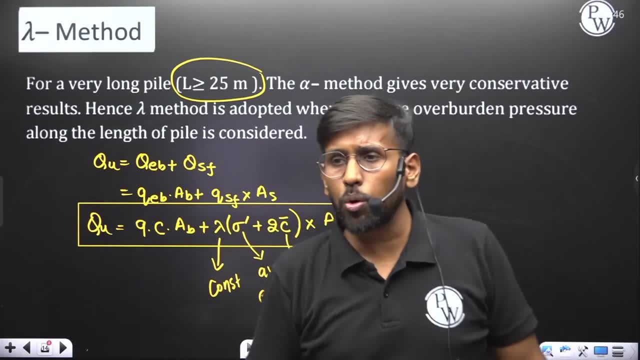 waise average niklega, Aur baaki toh aapka cohesion ke liye bata hi diye. Okay, Overbiting me. building ka load ka include karna hoga. kya Yaha pe building ka load ke include kar hoge? 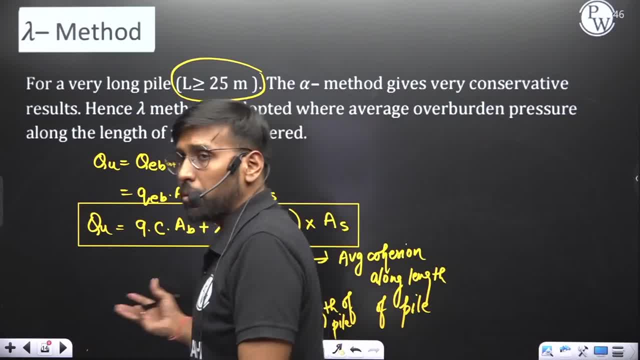 Hina Bhaiya, question kab hota hai? Pehle question sab na hoga hai ja pehle numerical, pehle concept seekh logay Pehle question, pehle kut padhogay. 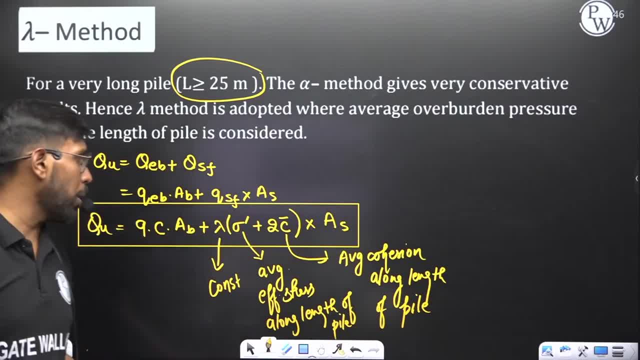 kya fayda? Pehle? dekh lo, yaar, Na ek hi baar me pehle concept hua nahi, sir question, pehle kuda do Aise nahi hota beta Chalo. 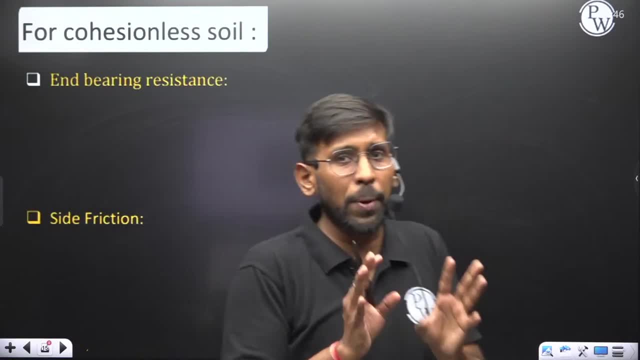 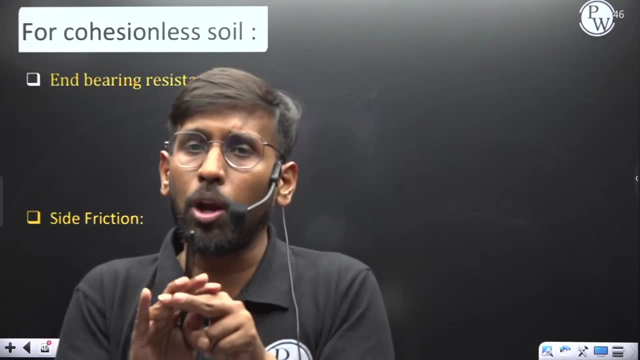 dekho me hape Toh cohesive, solve me hamar paas. do formula aaya: ek alpha method ka, ek lambda method ka, Alpha method for the general pile, jo aapko bola hoa hai, that's not a longer pile. 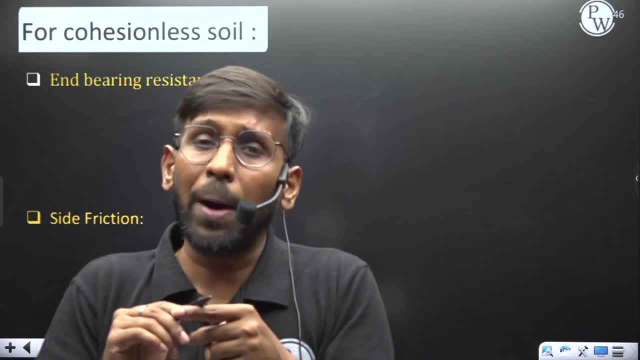 jaha pe aap bole, 9CAB plus alpha CAS Aapka. agar baat kar rahe ho, kis case me for the long pile. toh end bearing same aaya change kaha pe aaya. 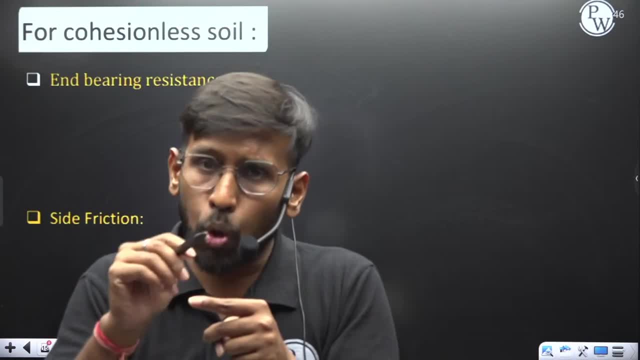 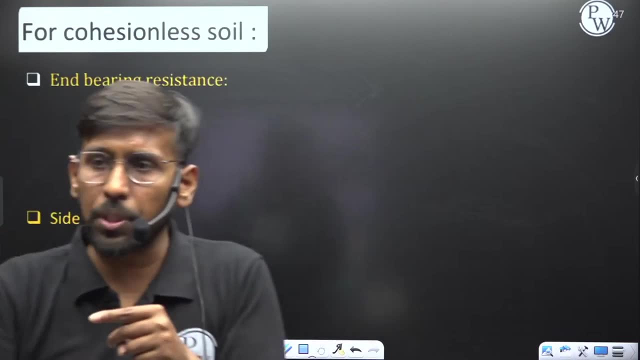 aapka change aaya side friction me jaha pe aapne bola jo QSF hai. that is lambda times. sigma bar plus 2C theek hai. ye aapka change aaya baaki sab same ta. 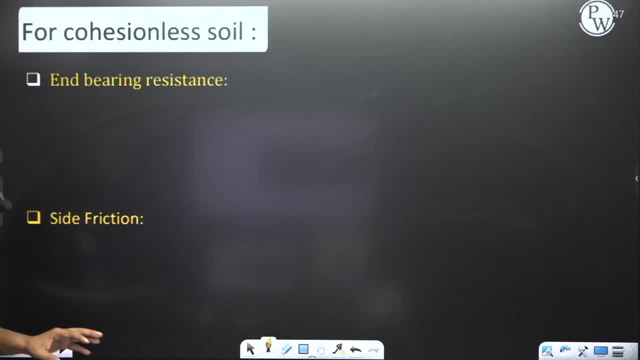 Dekho me hape, Dekho me hape. Sir, aap jo batane jaa raha ho na matlab hi itna piyara cheez hai na matlab aapne bola ho ka sir, ye am kitna bar padha hai. 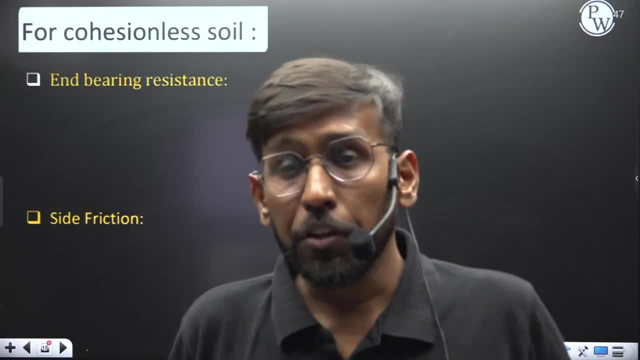 lekin, sir, formula rat, rat ke padhishan hai. Ye meri guarantee, sir, maza aane wala iss cheez mein. Ye meri guarantee, maza aane wala iss cheez mein. Dekho me hape. 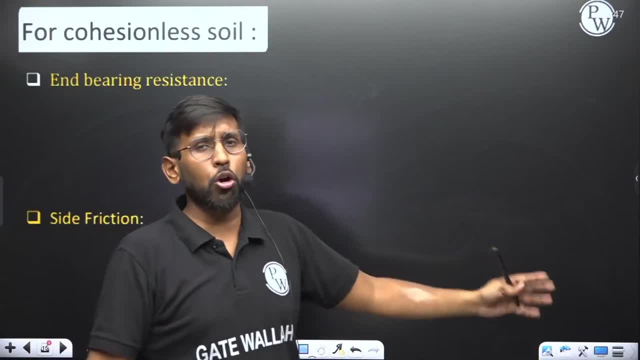 It's my guarantee, sir, aapne yaha pe jab tak jab bhi formula rata ho gaya, itna ber lamba choda formula, sir, kuch samajh me nahi aara. sir, Itna easy kar dunga na, sir. 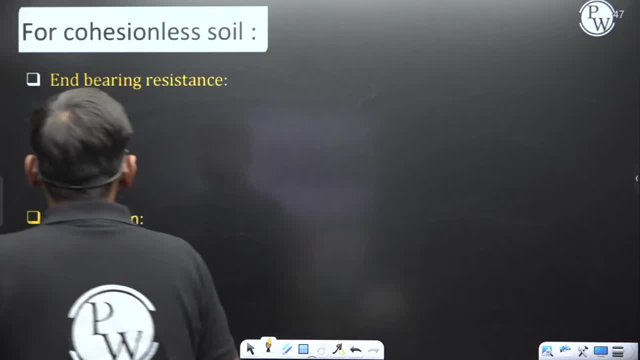 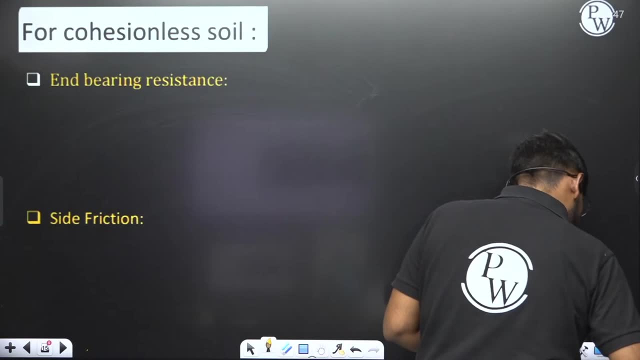 tumal di hai. Dekho for the cohesionless soil. For the cohesionless soil, Dekhenge meri dost Bola na, jabse running pe jaa raha ho na piyas bada lag raha hai. 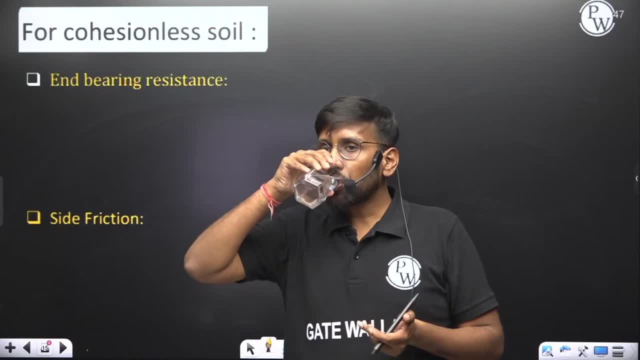 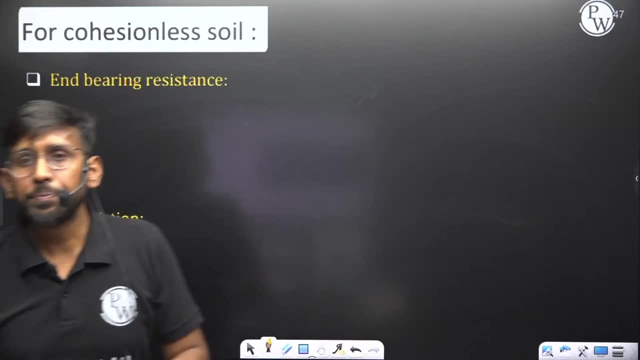 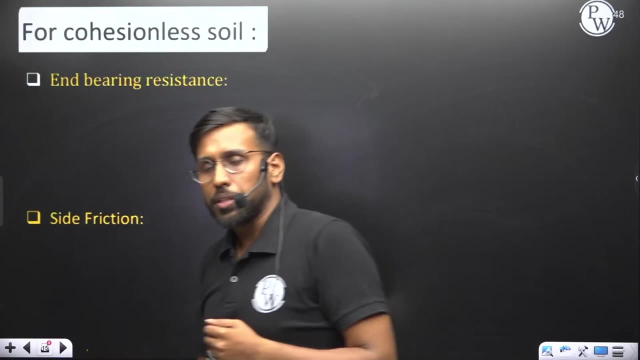 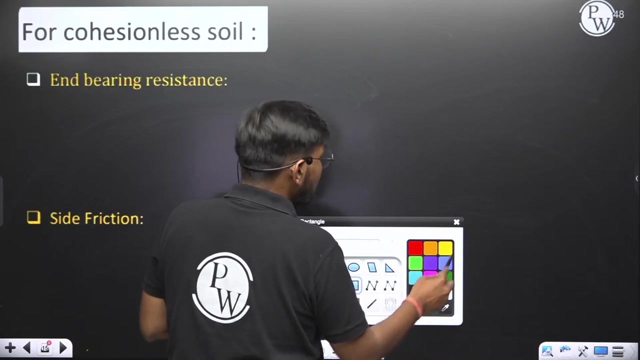 A second day tha running ka. Dekhe, Dekhe. So end bearing resistance, End bearing resistance. Dekhenge, samjhenge, Sir, ab yaha pe mera soil kaisa hai? The soil is a pi soil. 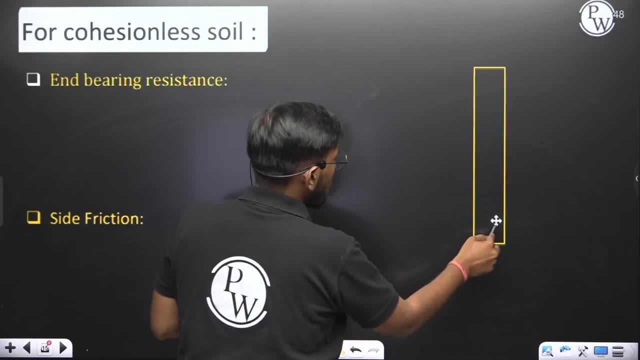 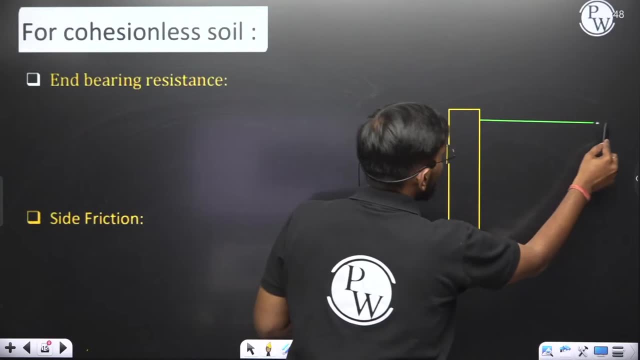 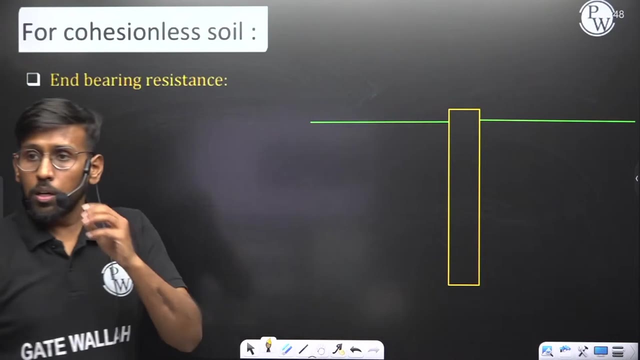 The soil is a pi soil. Right, The soil is a pi soil. Dekho me hape, Dekho me hape. The soil is a pi soil. The soil is a pi soil. Dekhe Now my dear friend. 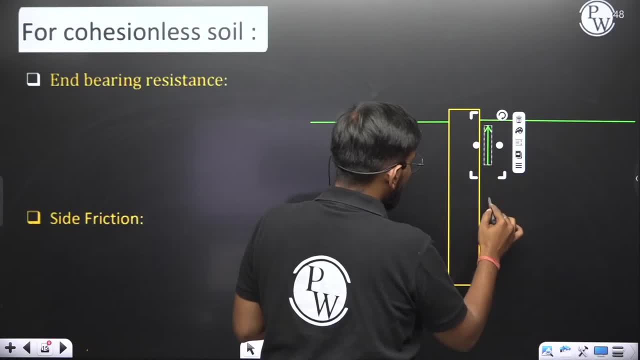 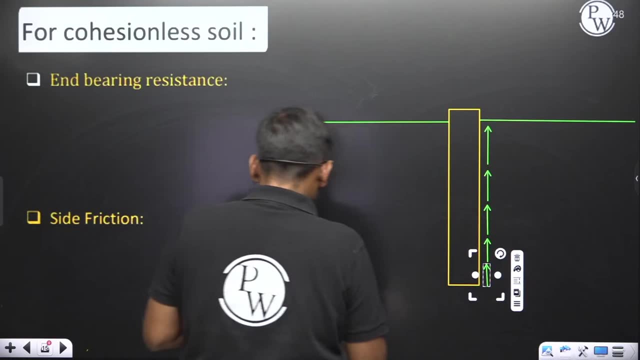 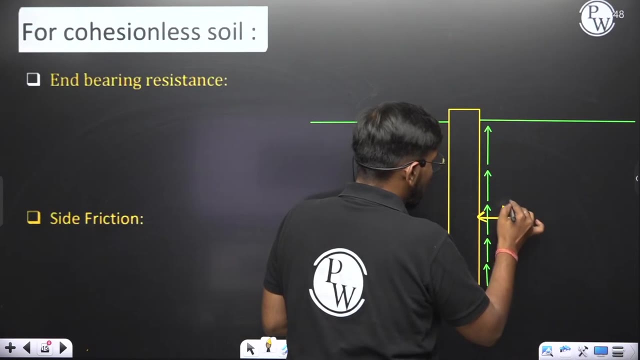 mera yaha jo resistance aara hai, ye frictional resistance hai. Yaha jo resistance aara hai, ye frictional resistance hai. Ab sabne bachman me pada hai ki agar mujhe normal load pata hai, agar mujhe 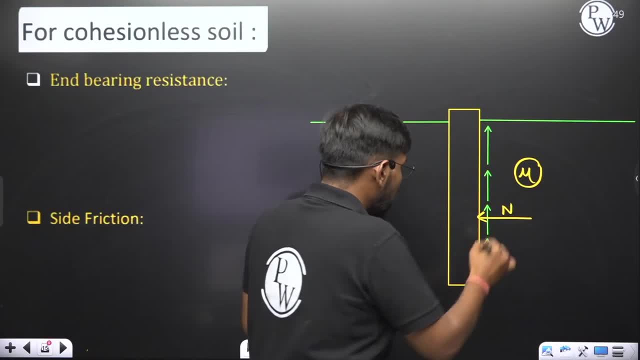 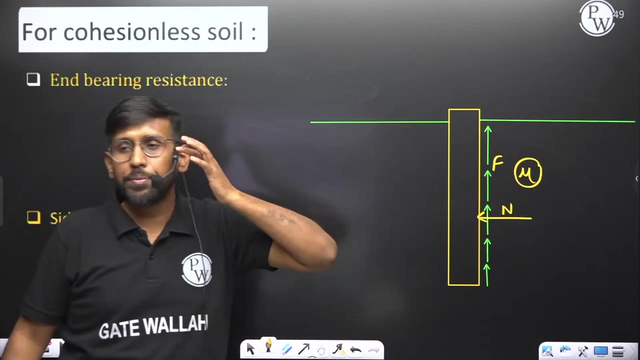 mu pata hai, toh mujhe personal force pata hai, Yes or no? Bolo mere dost pata hai kya Ye sab ko pata hai, kya Bachpang ka paap hai? Bachpang ka paap hai Yes. 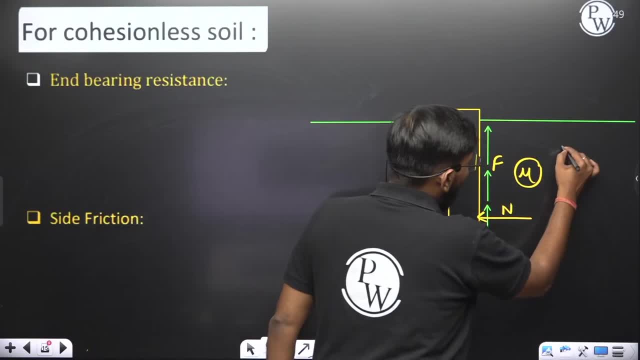 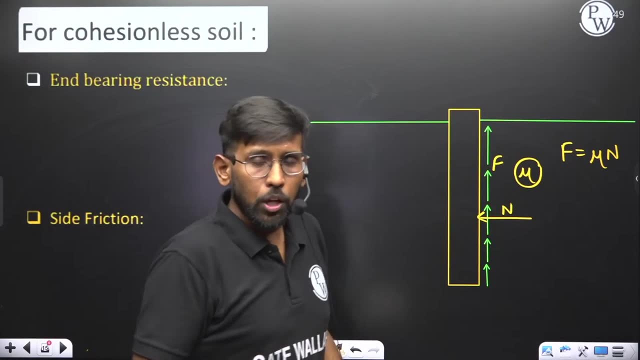 Yes, Toh, f bravara, kya bolte ho, f bravara. bolte ho mu times n Mu, kya bolte ho Jo angle banta hai usi ke li bolte ho Hai. na Toh mu bravara. 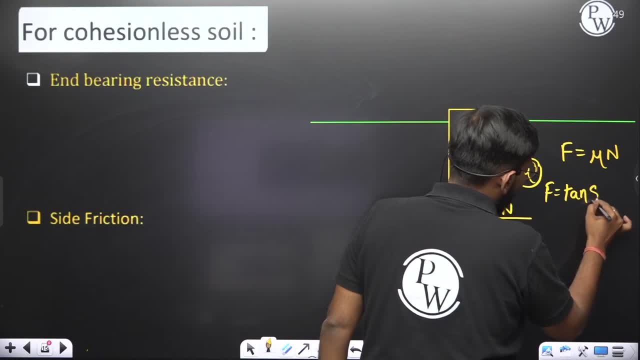 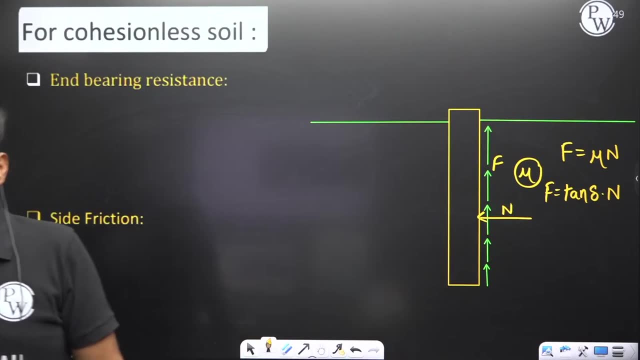 kya bolte hai: tan delta, Tan delta and this multiply with n. Aapko delta sawal me diya hoga, Aapko delta sawal me diya hoga. Toh, mu bravara, tan delta multiply with n. Aap dekho, ya pe Ye normal force kaun deyega. 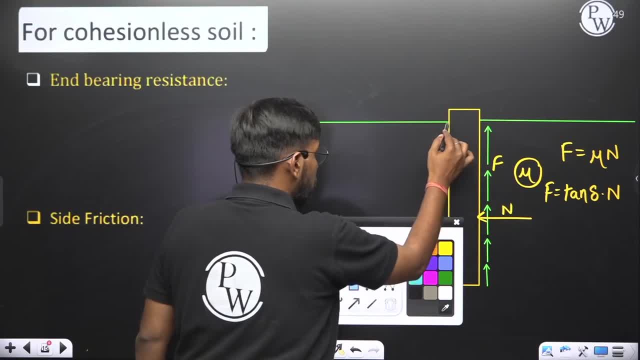 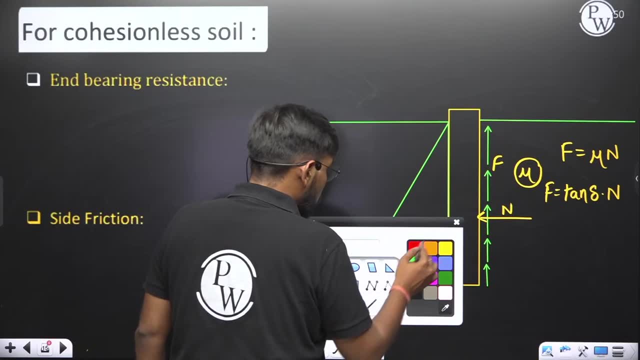 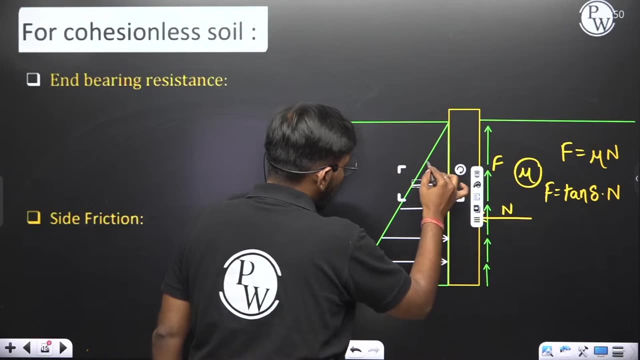 Ye, jo normal force aapko dik raha hai. ye, kaun deyega Ye normal force aapko earth pressure deyega, Jo mitti aap ke paas me, aapke surrounding me hai. yahi aapko deyera hoga, Bolo yaar. 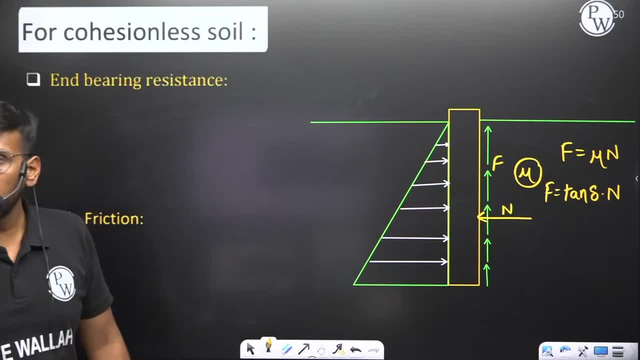 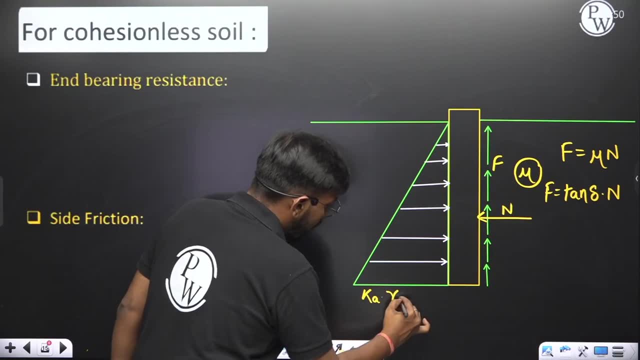 Arey bolo yaar. Yes, Yes Toh yahaan pe kya ho gaya. This is yahaan pe active situation le rahe hai Ka into gamma, into L Kik hai Toh mere dost. 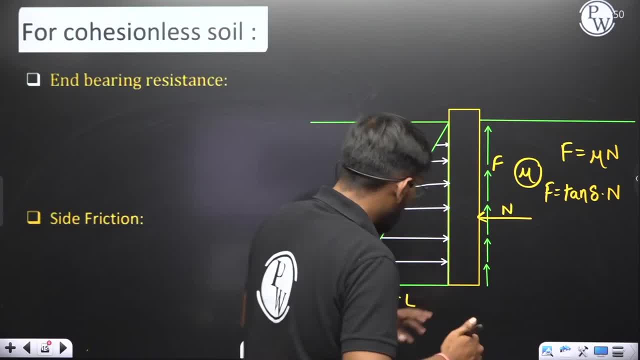 agar mujhe normal force nikalna hai, toh normal force kaise nikalengae? Average stress multiplied with area. Agar mujhe normal force nikalna hai, toh normal force kaise nikalengae Average stress. 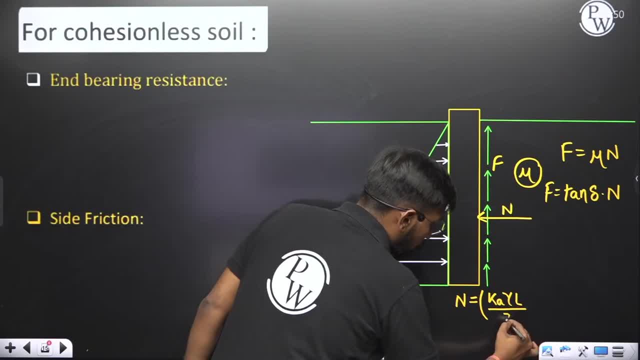 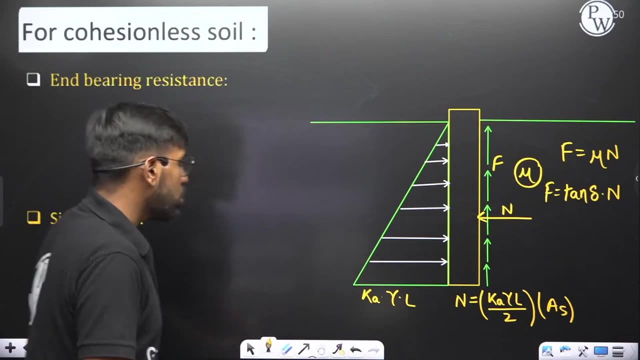 Average stress multiplied with area Aria, kya hoga? What is the area? What is the area? That is nothing but area of sites, nothing but area of sites. So, my friends, if I want to find side friction here, QSF. 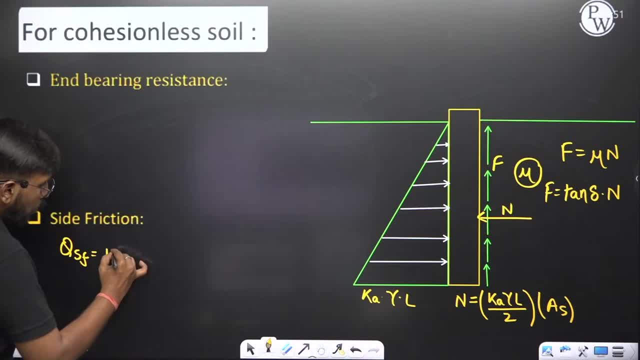 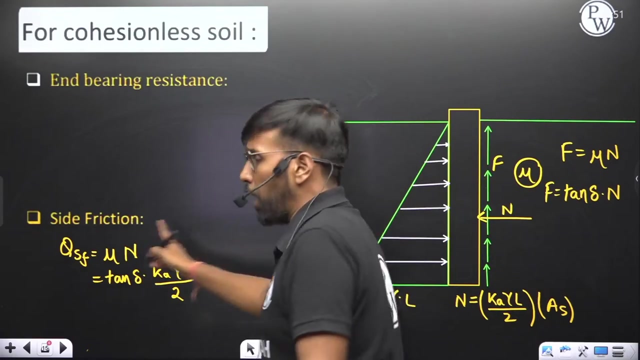 then what do I see? I see it is nothing but mu times n. Mu is nothing but tan delta and n is nothing but Ka gamma L by 2 multiplied with area of sites. Yes or no, Sir? we have to write the formula. We have to write the formula. Tell me, Do you have to write this formula? 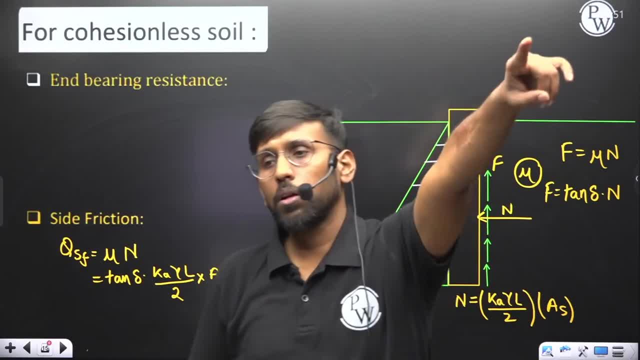 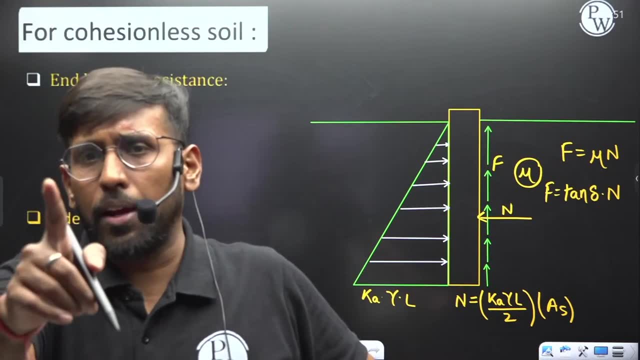 Tell me the truth. Ask me with your heart, sir. Do you have to write it? Tell me, man. Ask me with your heart. do you have to write this formula From now on? I will never write this formula in my life, Sir. 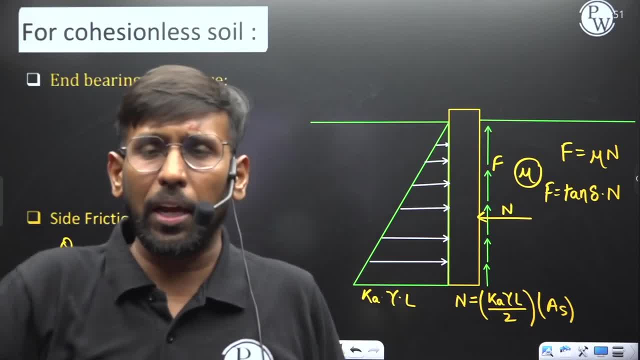 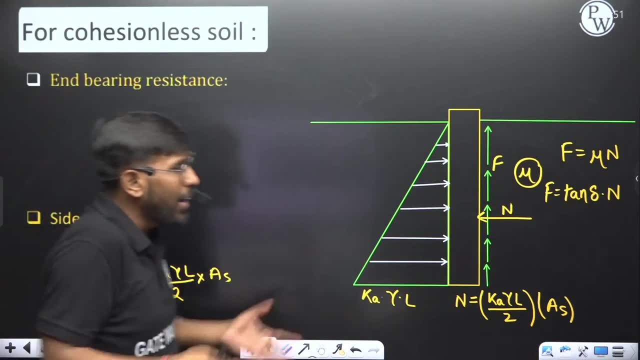 I forgot delta, I forgot to put tan Somewhere. I didn't put K, I didn't put gamma. Don't talk to me today, Okay, Because everything is understood. You understood how it came. And the day you understood how it came, sir, that day leave the formula. Forget the formula in life. See. 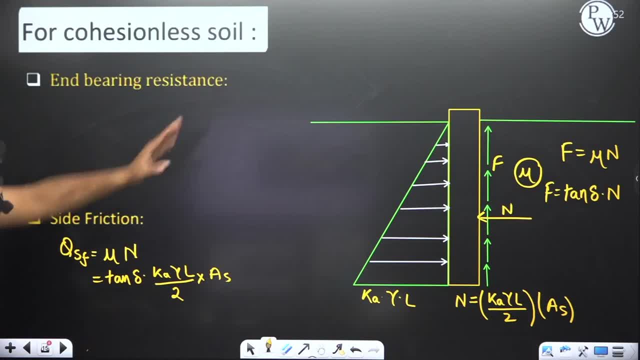 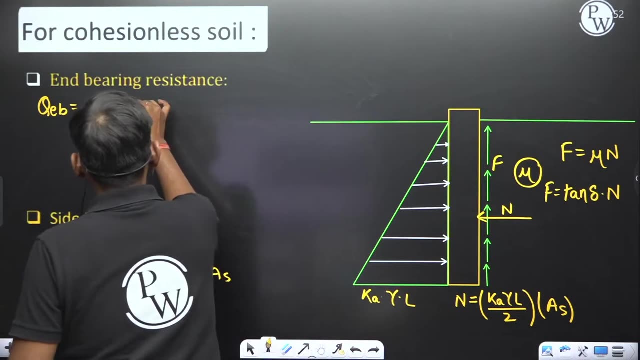 me here. Now let's talk about end bearing. Now, let's talk about end bearing. So, sir, let's go back to Merov theory. What did you say? C and C, alpha C and C, gamma D. instead, 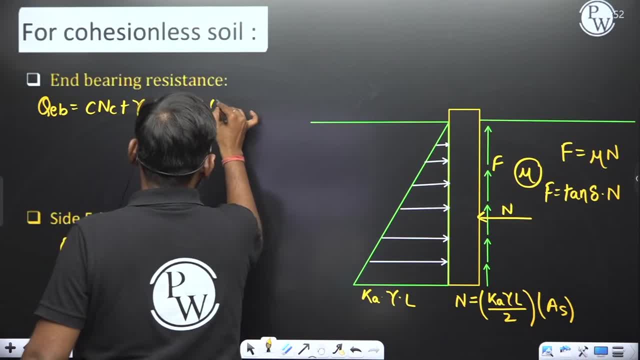 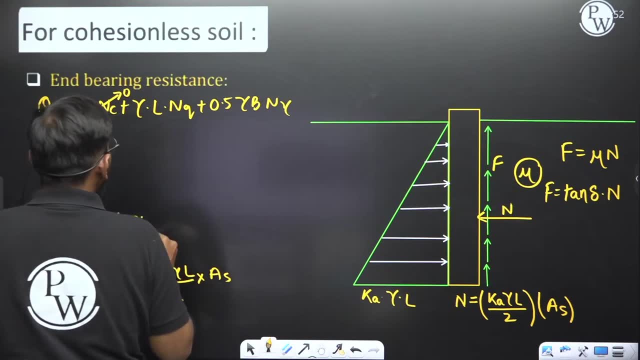 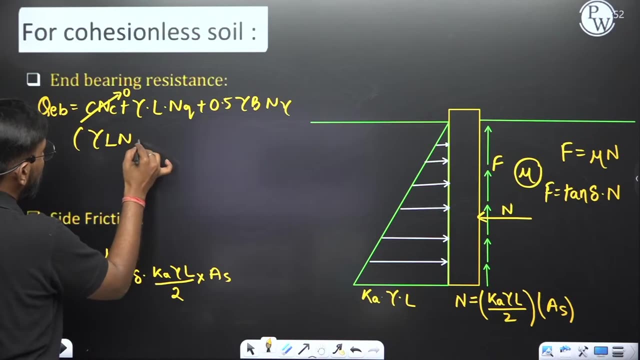 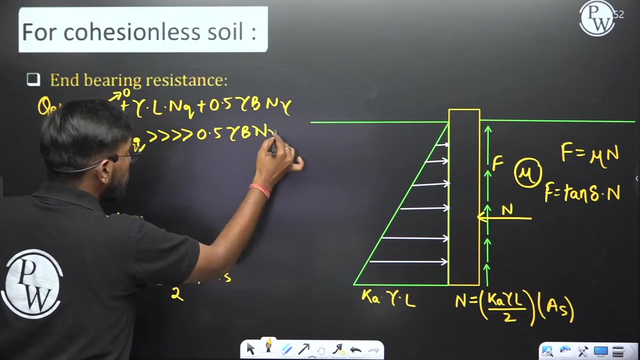 of L, thank you, plus 0.5, gamma B. Okay, Now cohesion is 0.. See what will happen here. See what will happen here. This gamma L and Q is very much greater than 0.5, gamma B and gamma, Because B is very less Right. So for this reason, 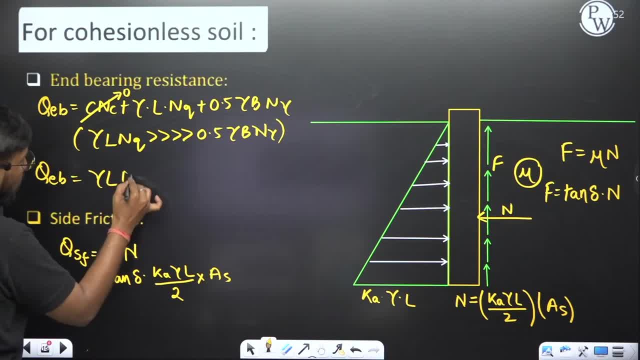 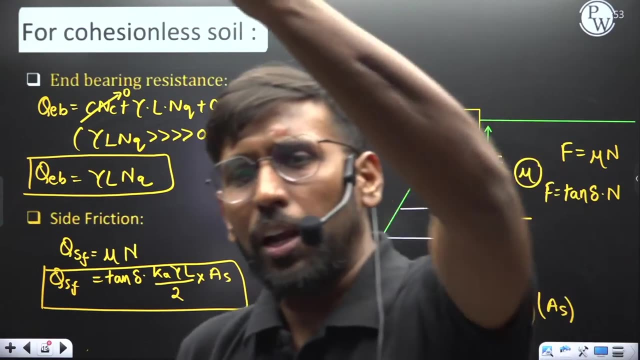 what has become your Q and bearing Nothing but gamma, L and Q. It's easy. Is there anything? Is there anything Over QSF? this is your QSF, Sir. you have read the theory that C and C, gamma, L and gamma. 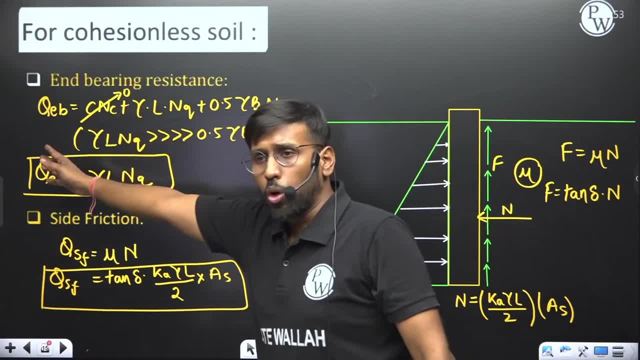 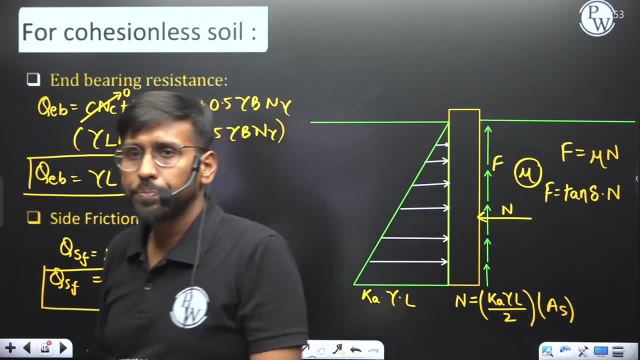 D and Q, plus 0.5 gamma B and gamma. Instead of B, put L. If you say that gamma L and Q is much greater than 0.5 gamma B and gamma, then I have got the result. My result has. 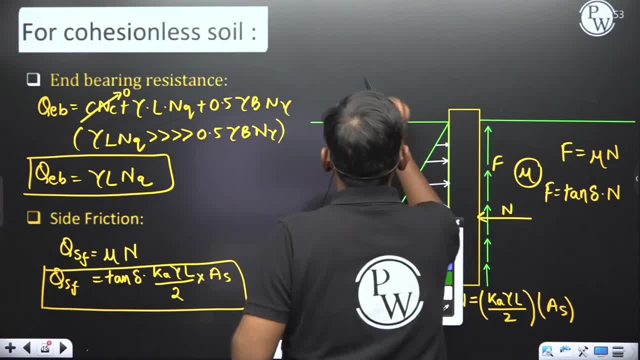 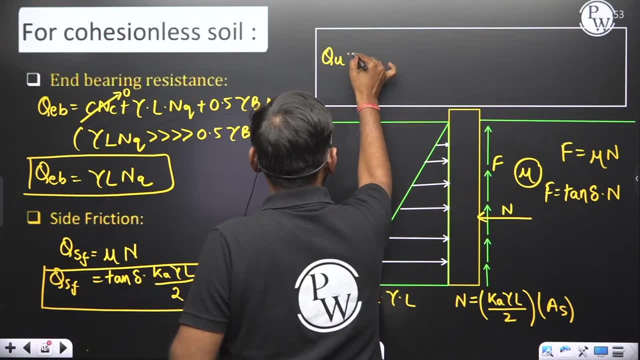 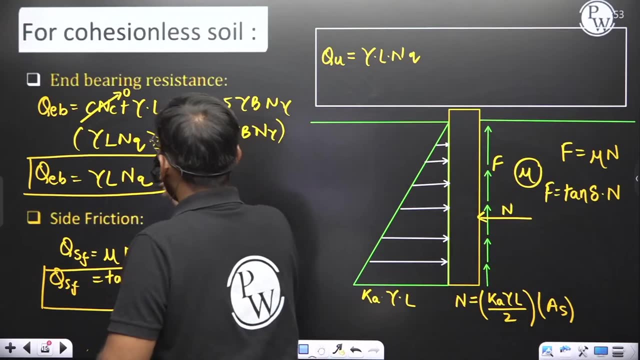 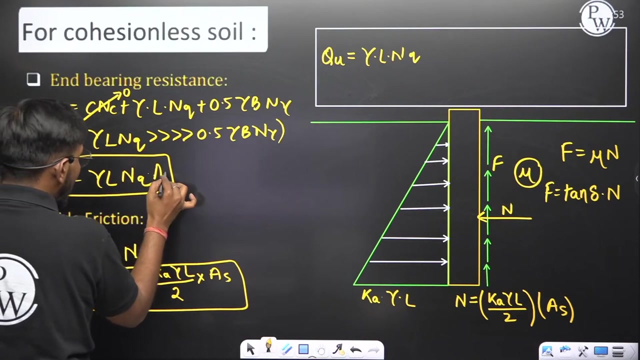 come. Okay, brother, If you say: Then, if I summarize this, if I summarize this, will you say that the answer is yes or no? No, So what I can see? I can see Q ultimate is equal to gamma, L, NQ. okay, here what I have to do. I have to do one more thing. this is small q e b, so multiply with area at bottom. 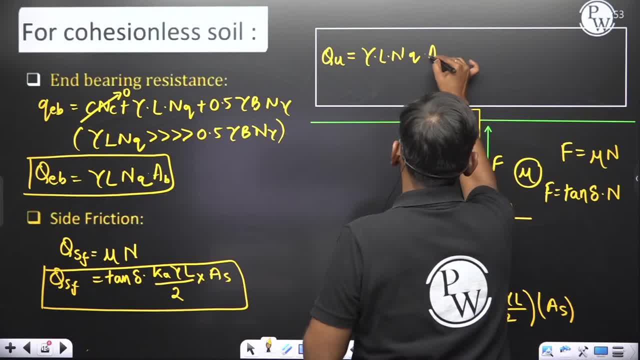 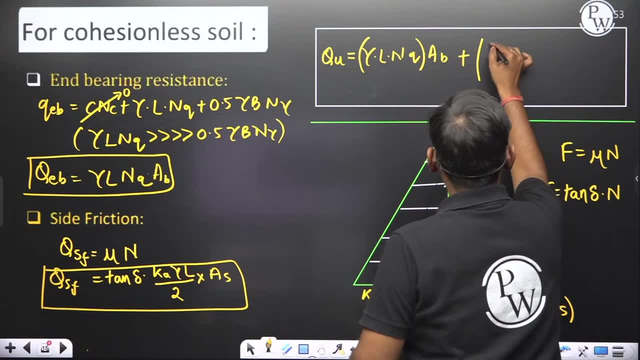 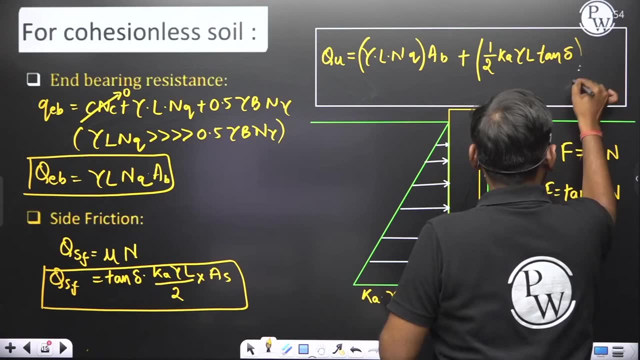 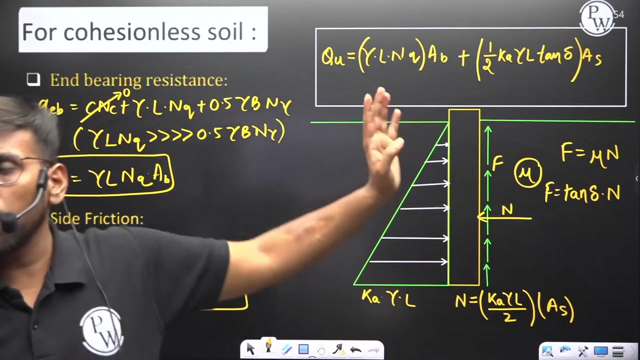 So gamma L NQ multiply with area at bottom, because this is your resistance. plus, here, what we can see: half k a. gamma L tan delta multiply with area at sides. Sir, this formula saves the band of adho by looking at it. this formula saves the band of adho by looking at it, is it right? 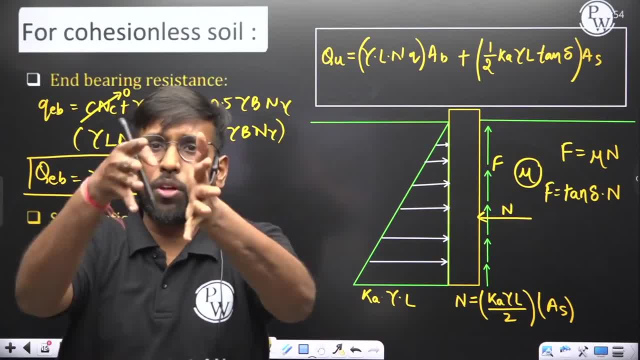 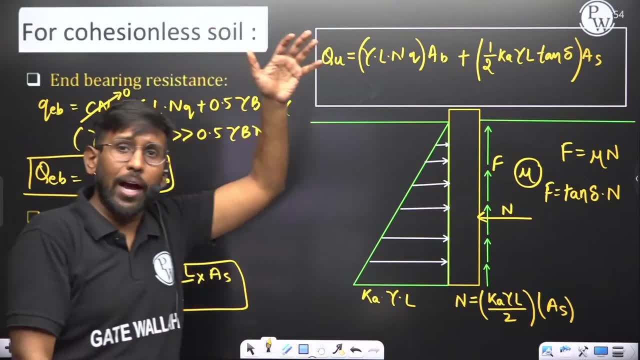 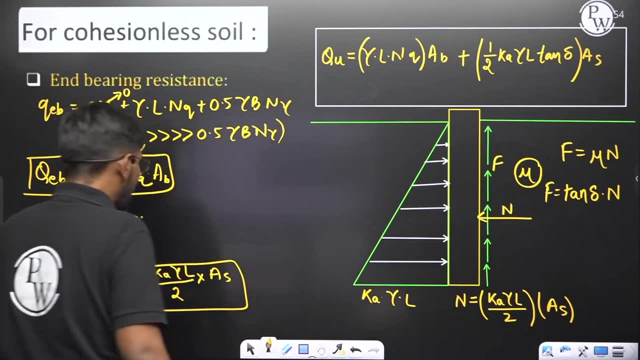 Why will it be greater? Why will it be greater? Length is very high compared to that of the width. Your length is very high compared to that of the width or diameter, or your width. okay, See what is done in side friction. again, understand basic mu times N. friction is nothing but mu times N. 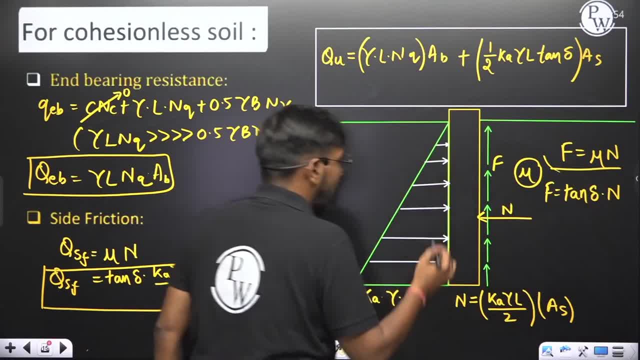 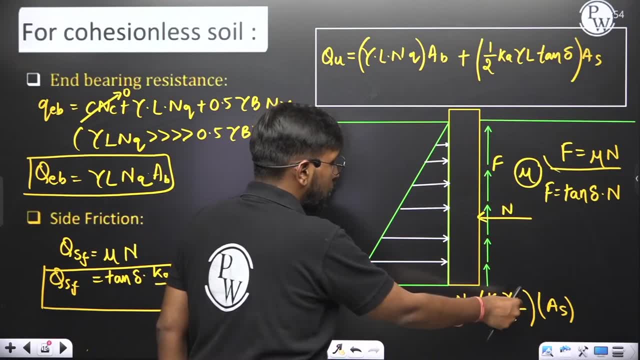 So what is F equal to Mu, is equal to tan delta. where will N come from? It will come from where you are getting horizontal pressure. So your vertical Multiplied with the earth pressure coefficient, Okay, that is giving you horizontal. 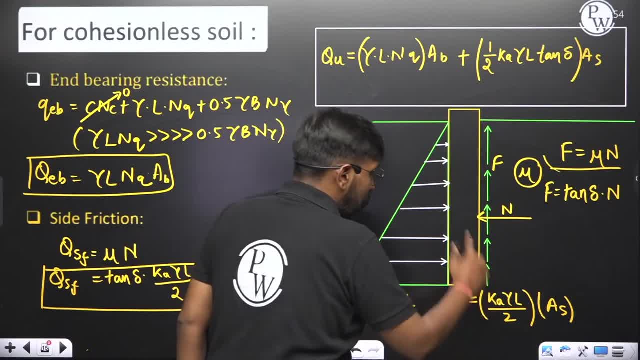 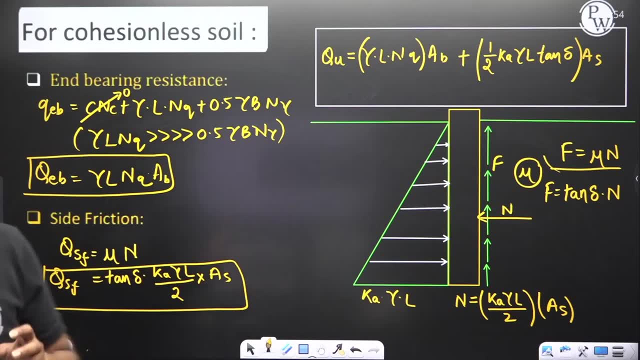 If you want to take average, then by 2, because the upper one is zero and linear variation is there, so your average stress is gone. What will be the area? Surface area will be there. N will give Clear, Will you say. 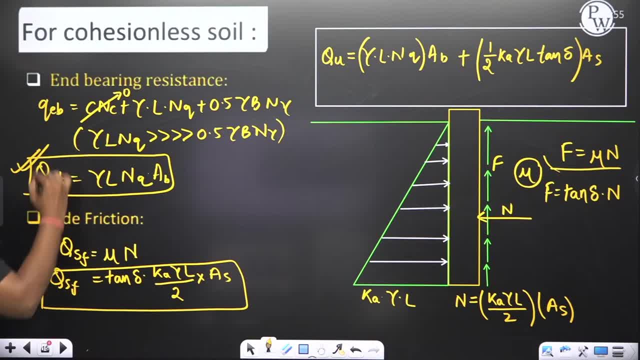 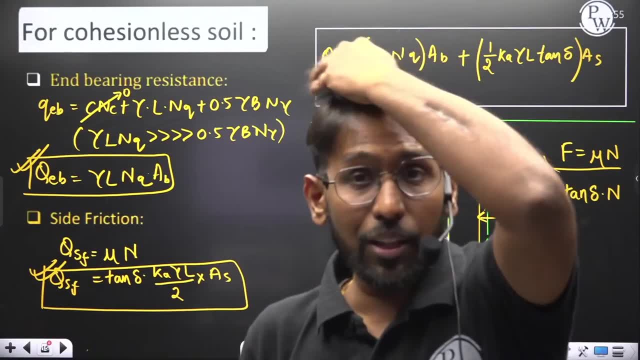 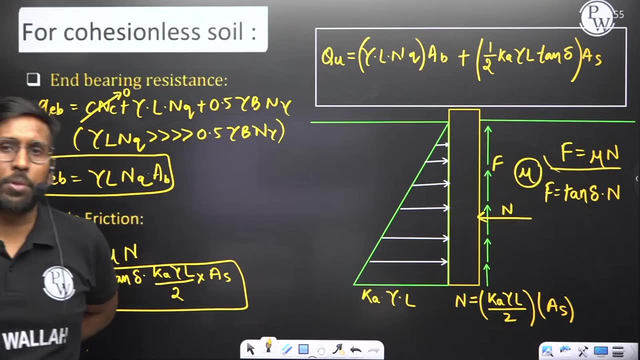 Krishna, is it clear? Say it, Is it clear to everyone? Now it will be fun Now. if you understood this, then you will answer my next question. How many people will answer my next question? dena chaate ho itne log mere hagle sawal ka jawab. dena chaate ho bolo agar tumne yaha. 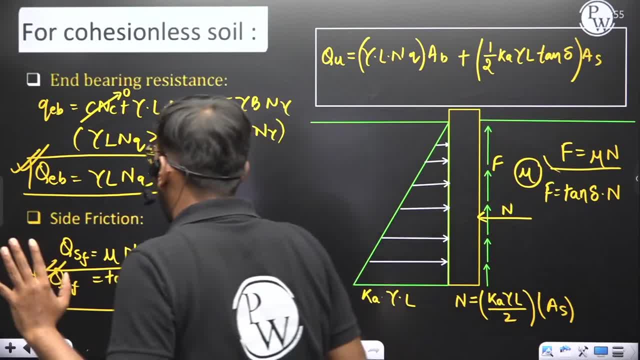 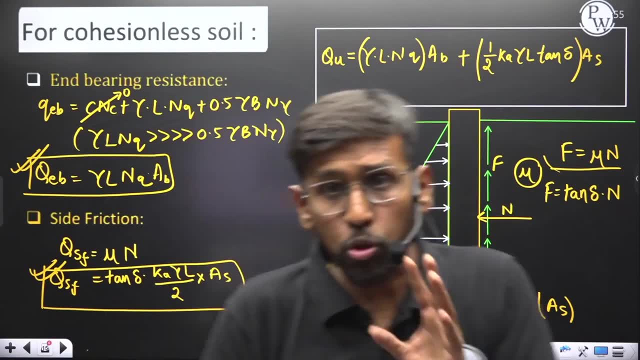 pe ek, ek concept samajh gayo ab, sir, kuch nahi ratna hai, kuch nahi ratna hai, kaisa bhi kariv, kariv, kaisa bhi sawal dede. aap jawab dedhoge ab, sir, tum soch ke bata na, can water? 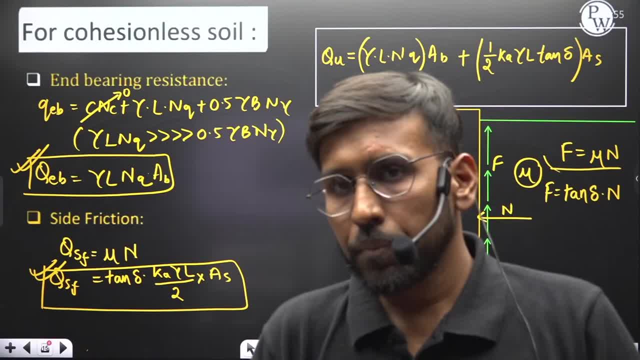 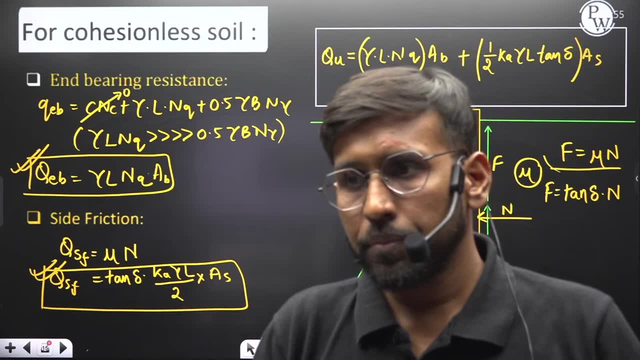 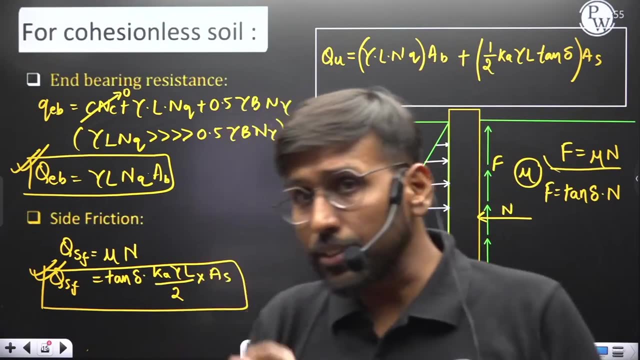 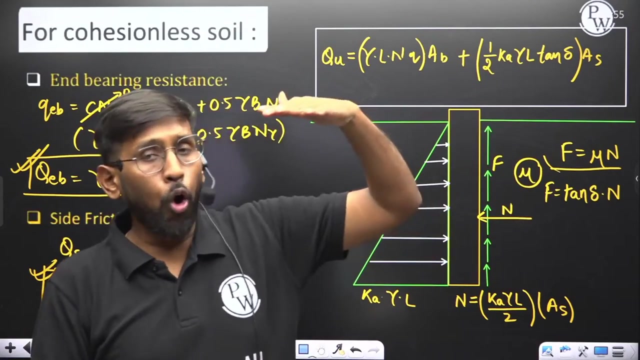 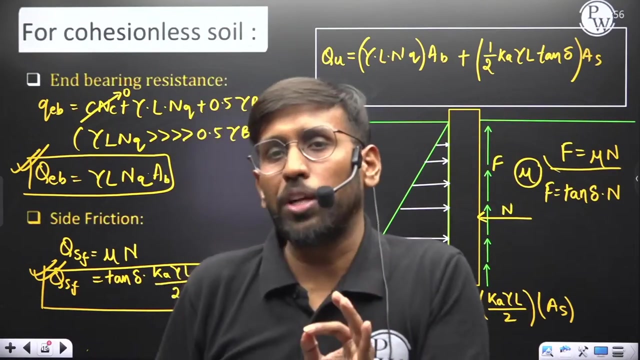 resist any shear? kaisa earth pressure coefficient can water resist any shear? no, water cannot resist any shear. right now let us say, if this is submerged ground water table jo hai, wo ground level pe hai, jo ground water table hai, wo ground level pe hai. so us situation me kya antar aayega, pehle wale me end bearing, me koi antar nahi aayega. 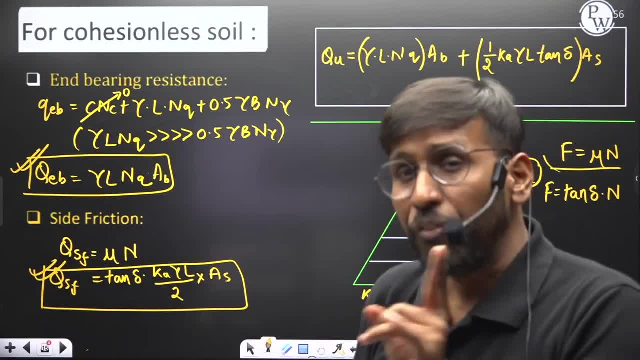 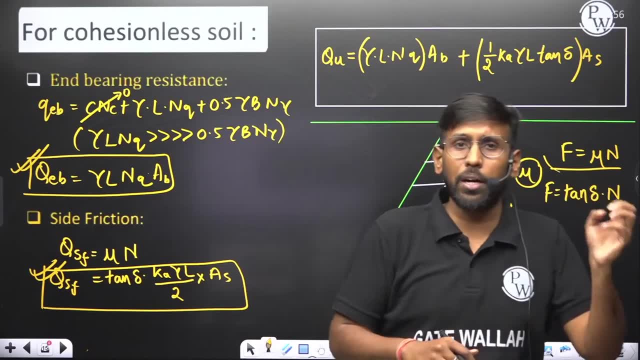 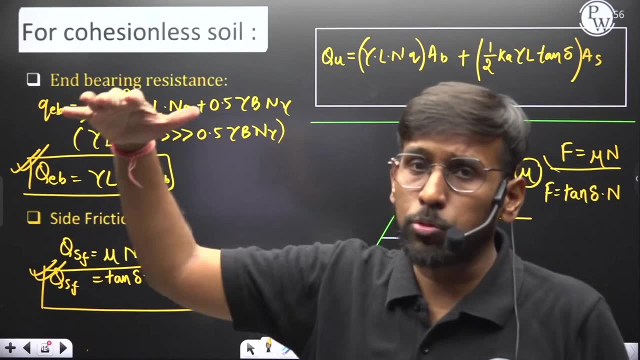 end bearing me koi antar nahi aayega side friction ke case me kya antar aayega? let us say submerged, hum gamma submerged rik raha hai gamma w hai kya antar aayega, agar water table ground level pe hai matlab soil submerged state me hai to us, case me kya. 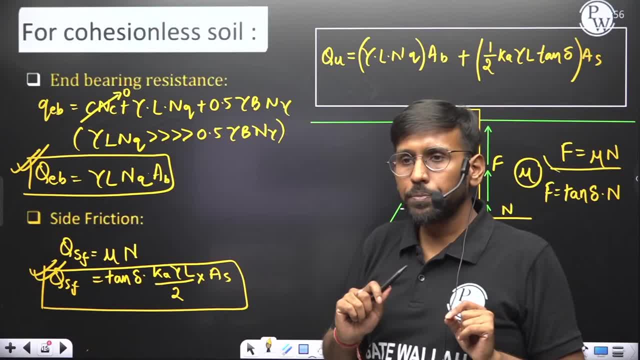 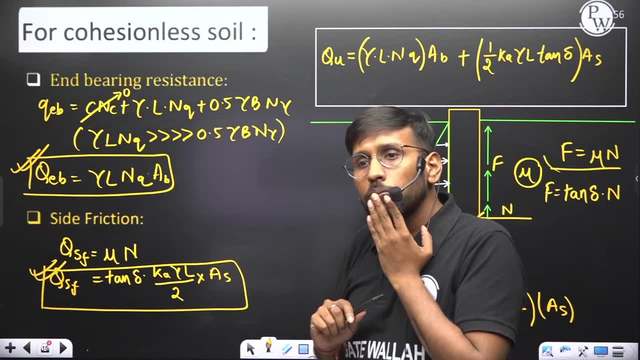 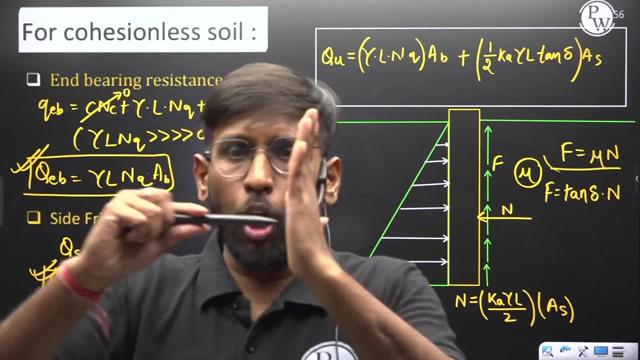 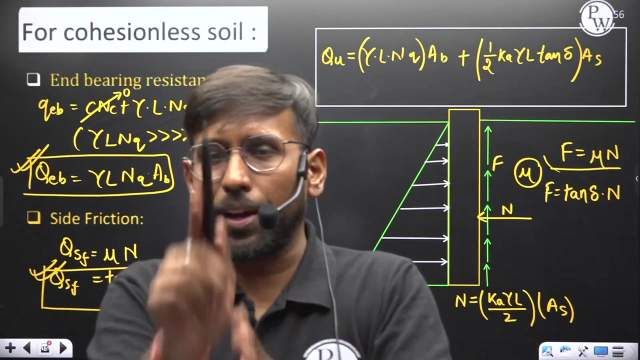 antar aayega is formula me. kya antar aayega end me change hoga? kaisa change hoga? water pressure lagaega in the vertical direction, ki nahi lagaega. water horizontal pressure toh laga raha hai. water horizontal pressure toh laga raha hai, lekin kya vertical lagaega? 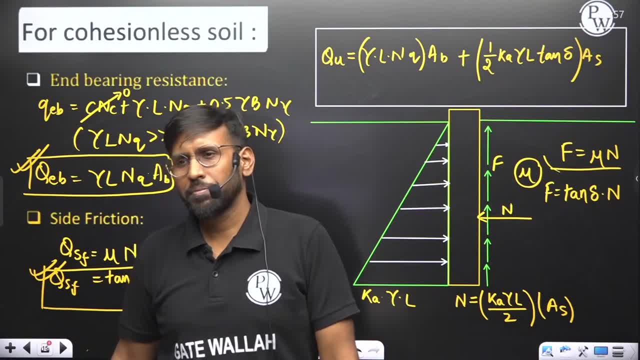 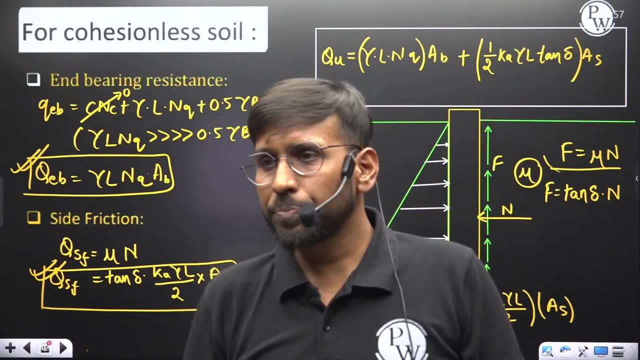 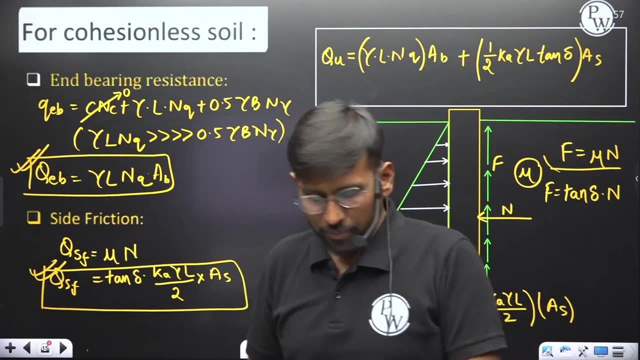 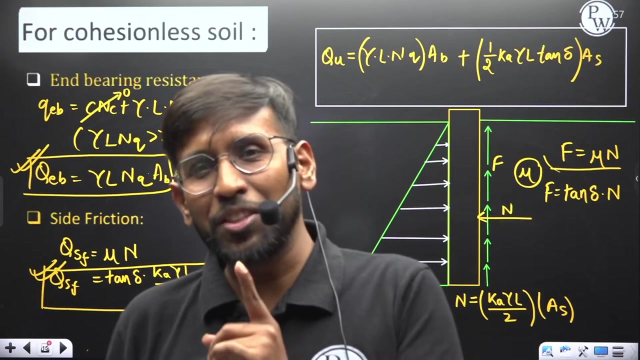 risk ke place. kya maths, kya Africa raha hai? Bao de water horizontal pressure, toh laga raha hai any way. that say, jab humo brother parRun raha hai, toh any wa th stuck, toh laga hand. tak humour ka i hingao noh hain ho man toh. 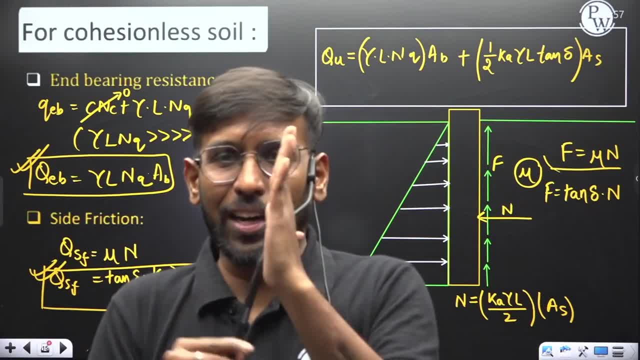 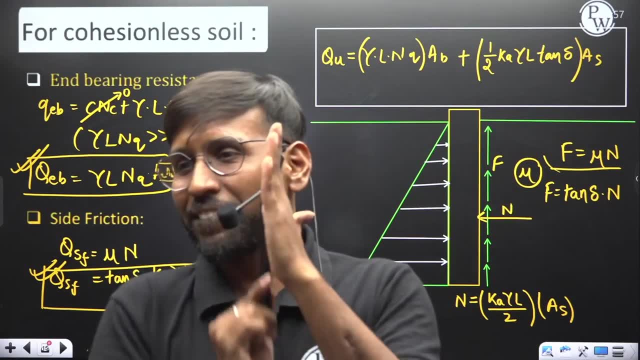 things ke qaoubt hai, siis k Parala pra wein man se hai aag apwa okaricha hai, agar aap�ỏ jauntal laga raha tha, but kya uska effect? but kya uska effect nahi rahega re murk nahi. 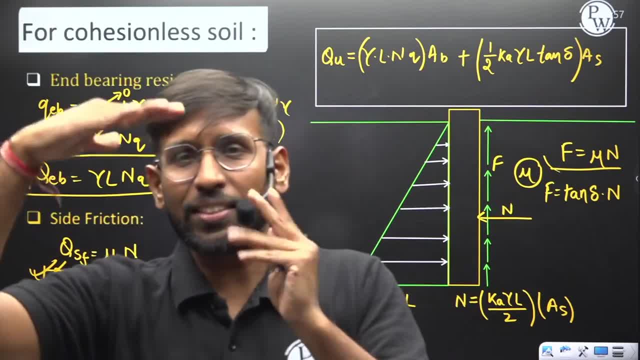 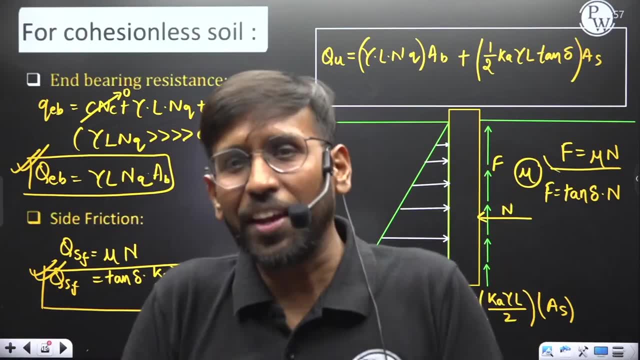 rahega, toh aapko jo effect. agar submerge hai, toh aapko jo effect dik raha hai, sirf solid ke kaaran dik raha hai, jo resistance aara hai, sirf solid ke kaaran aara hai, aur sirf. 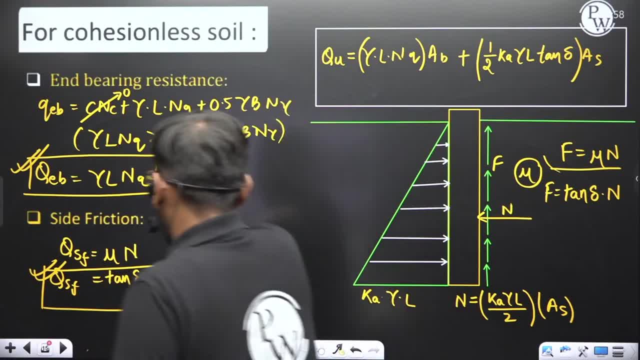 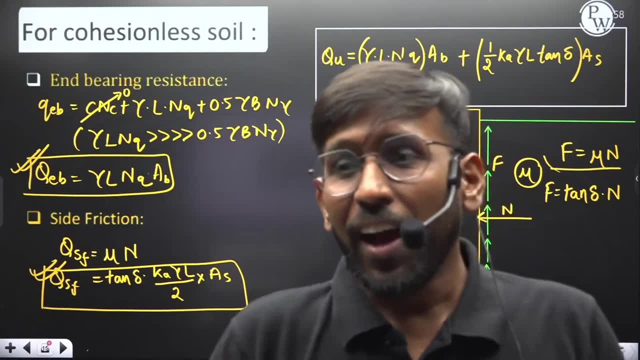 solid ke kaaran aara hai, toh yahaan pe gamma ke jaga kya ho jayega. yahaan pe gamma ke jaga, kya ho jayega gamma submerge aa jayega, agar water table hai aur aisa situation? 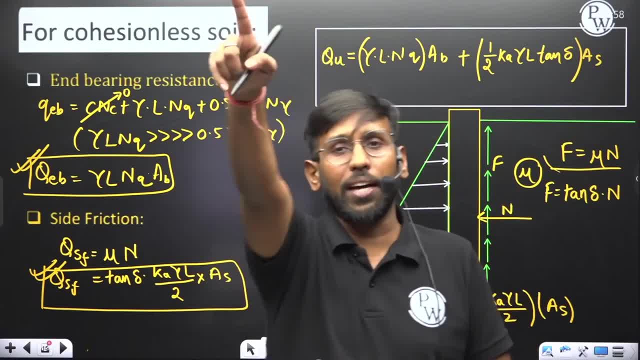 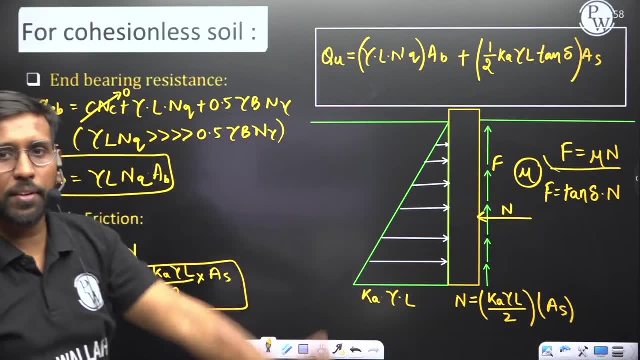 hota toh yahaan pe gamma ke jaga sirf aur sirf, kya aajata gamma, submerge, aajata maza aaya sirf. yeh hota hai, concept, concept, sikhogay, tab toh numerical banane ke layak. 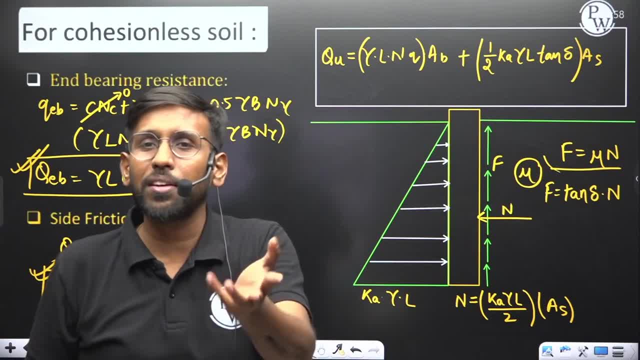 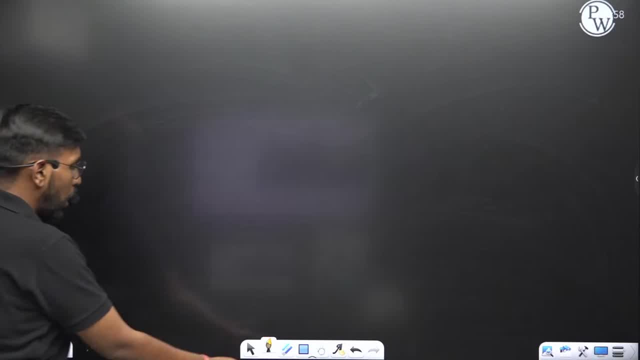 banogay. abhi, tum layak hi nahi hu, numerical, numerical banane ke liye toh pehle concept sikhlo hai, na sirf. toh, agar yeh concept sikh gaya, toh ek numerical dekho, yahaan pe ek concept, dekho, ki aapko ek situation. 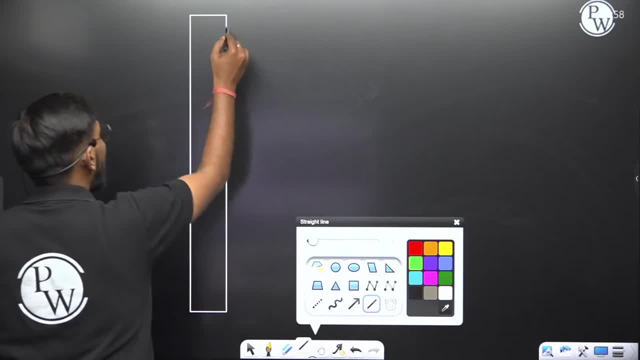 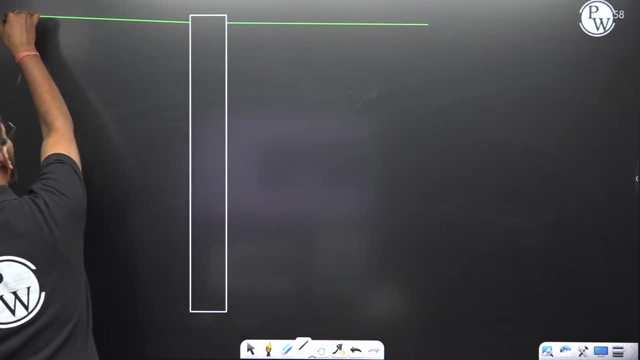 hum dete hain maja aayega maja lana hai ki nahi lana hai sirf complex se complex dedo koi fark nahi padta mera concept strong hai hai, na complex se complex question. 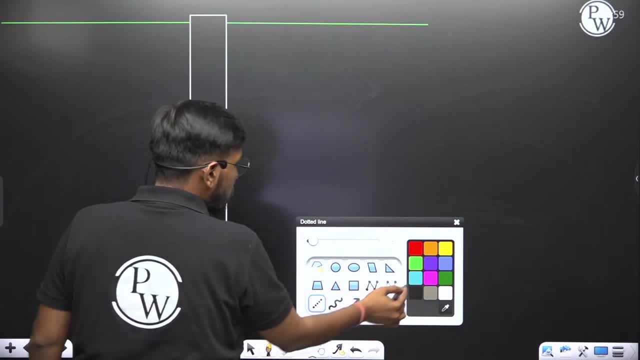 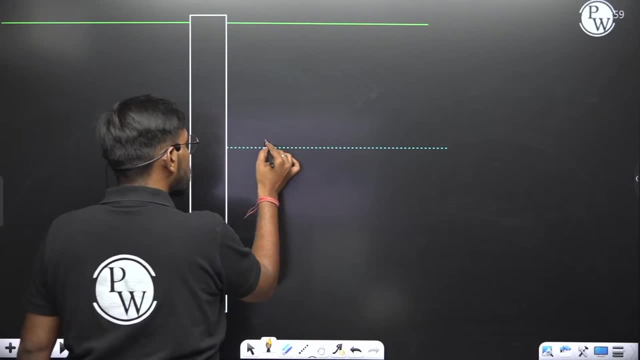 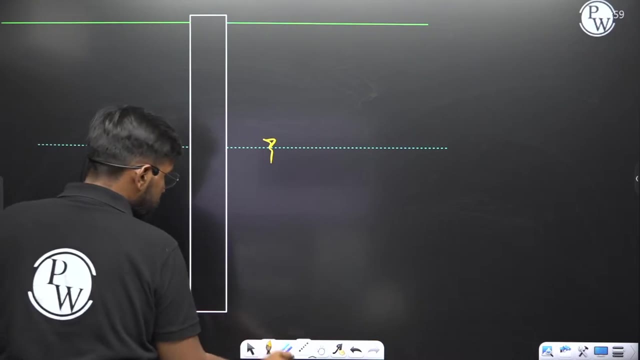 aap dedo sirf koi fark nahi padta sirf. mere concept strong hai hai ki nahi hai. kya hi fark padta hai sirf, kuch bhi do sir hai na. kya hi fark padta hai sirf. 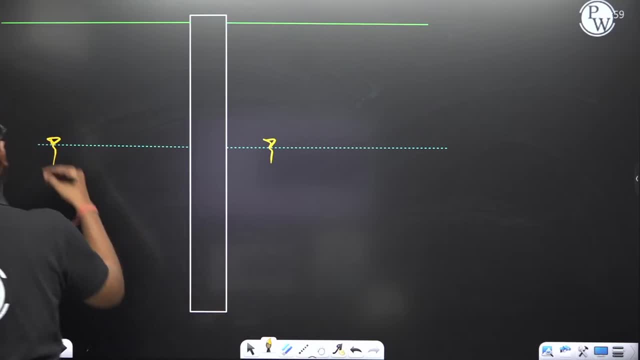 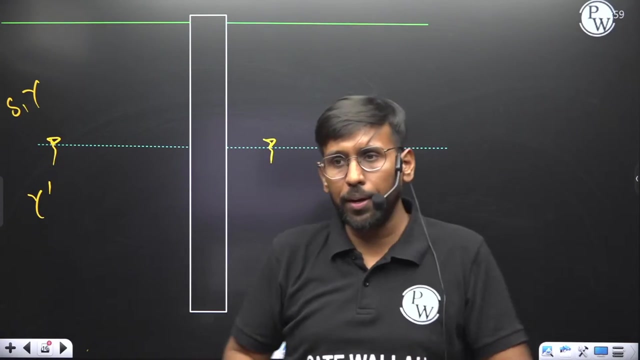 so, throughout the same soil, delta aapko given hai, delta, aapko given hai upar me ek koi. Up there is Gamma, and below we are writing Gamma Submerge because we have to use it. Up there is Gamma, and below we have Gamma Submerge. 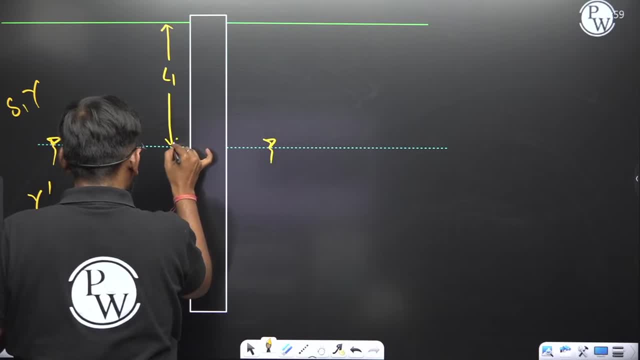 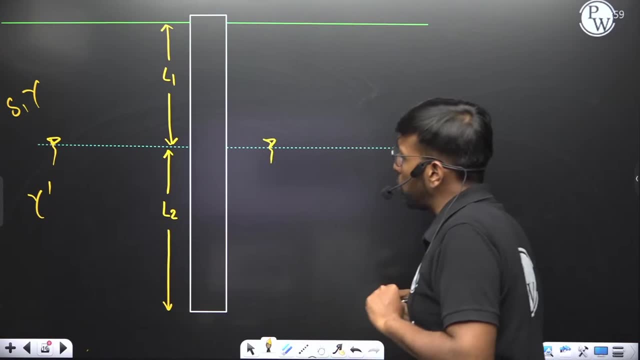 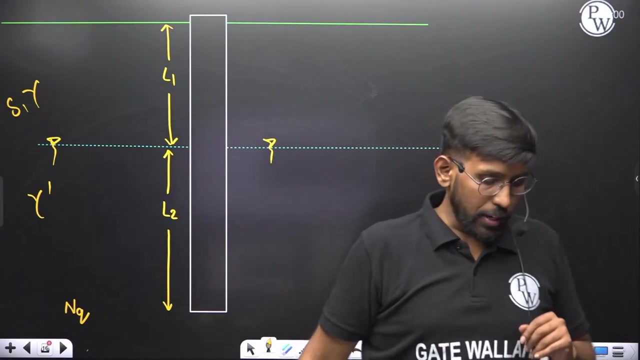 Here we are saying L1 and below we are saying L2.. L1, L2 and what else? You have NQ given in your question. You have NQ given in your question, Right? You have KA given in your question. 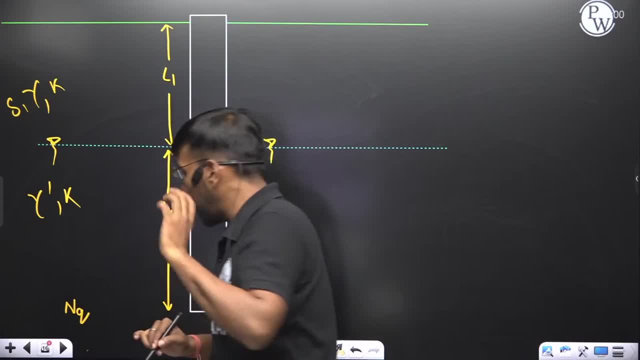 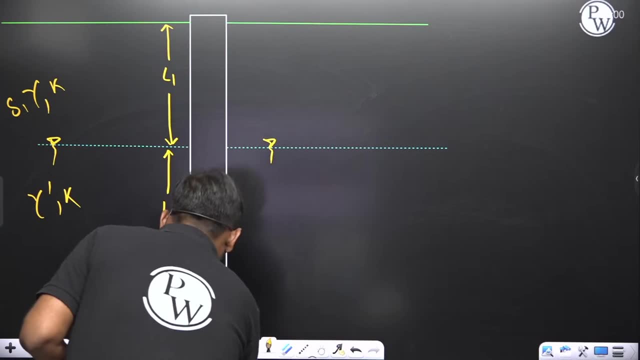 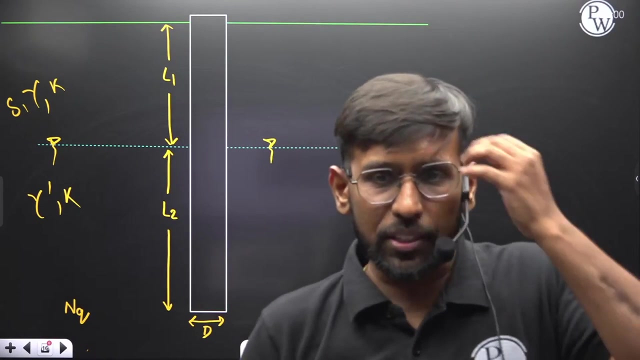 Here we are writing: K. This is given to you, Right? This is given to you. This is your circular footing of diameter D. This is your circular footing of diameter D. This is the circular footing of diameter D. This is the circular footing of diameter D. 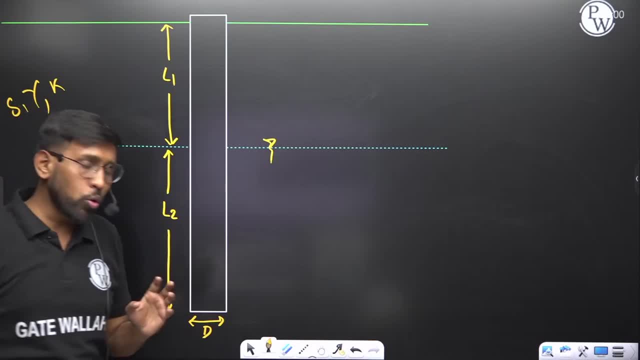 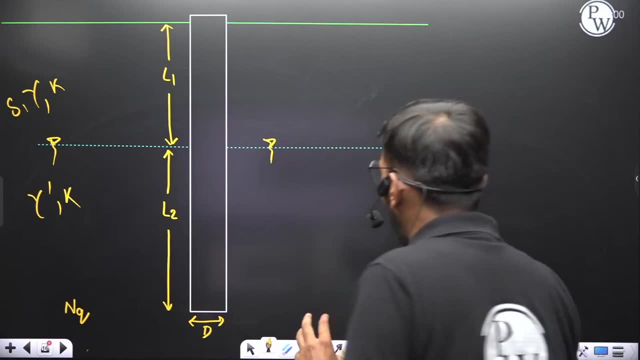 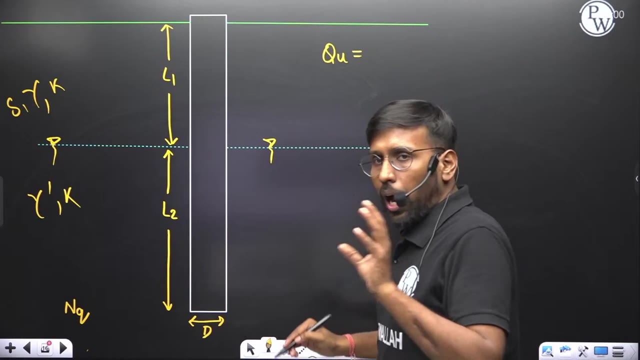 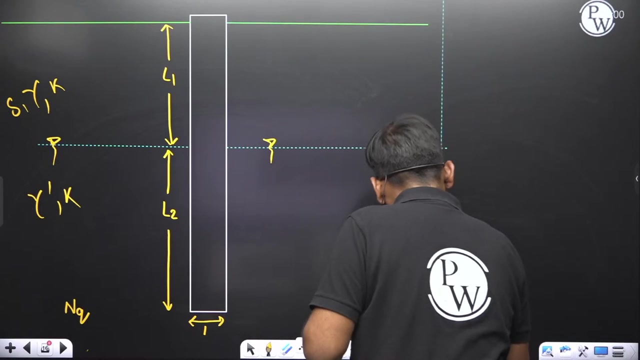 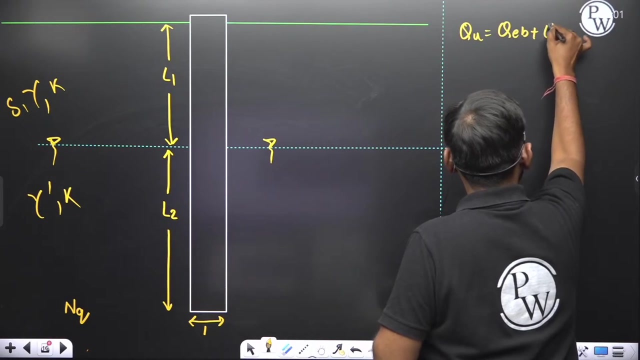 And in this situation we need to find the ultimate load carrying capacity. In this situation we need to find ultimate load carrying capacity. Sir, the ultimate load carrying capacity, The ultimate load carrying capacity, is nothing but Q end bearing plus Q side friction. So if I talk about end bearing, then this is very easy. 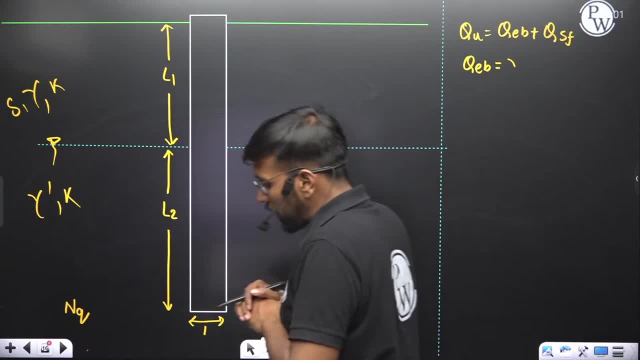 This is very easy. Tell me, this is very easy. right, The Gamma you will take? will you take the Gamma bottom? So you will take 5 steps? ok, If you will take Gamma, then how will you take the Gamma? 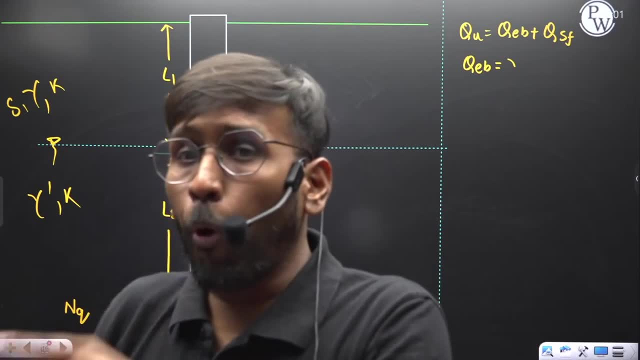 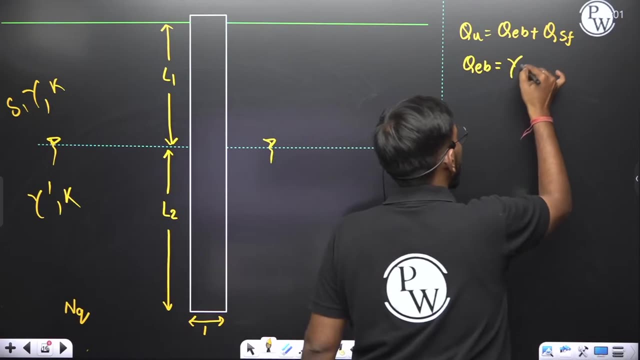 the Gamma will be taken from bottom And how will you take it in the bottom state? If you take Gamma in the submerged state, then what will you take? Then what will you take? Will Gamma become submerged- Speak mentioned earlier Here- in this level, if you are talking about here? so how will you saturate? 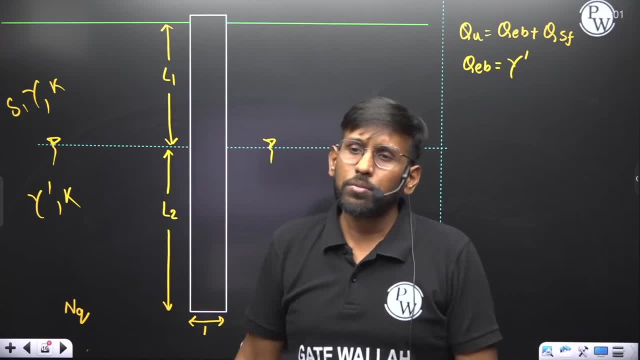 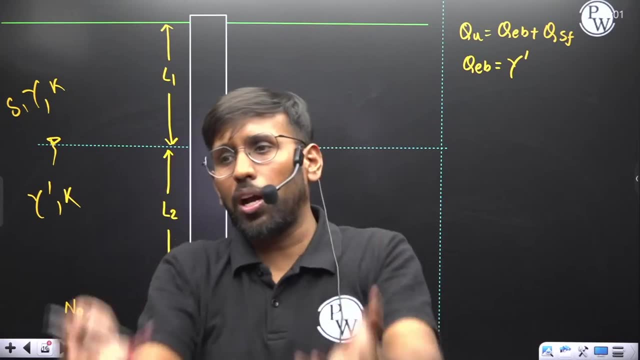 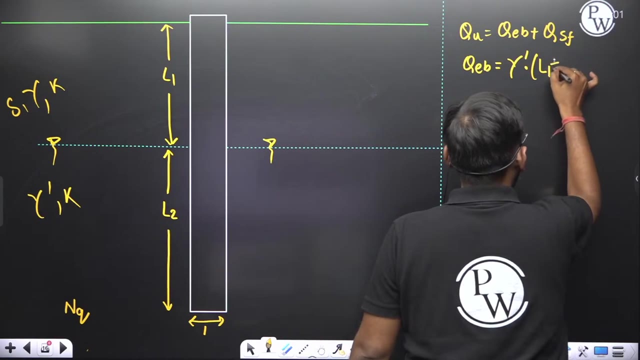 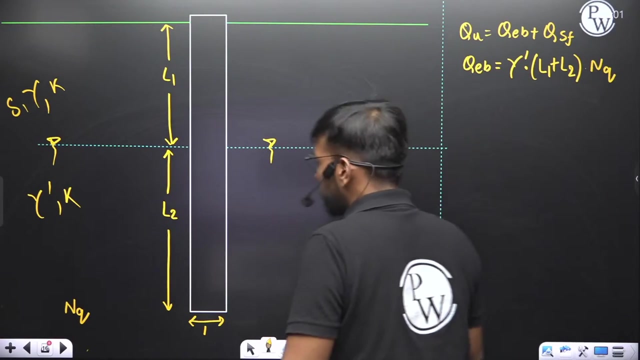 See if the resistance is given, so the water will not be feeding too much, The water will not be loading from the upper sideência. You will not be getting that high level. merge into L1 plus L2, gamma LNQ. this will be done. this will be done. tell me, this will. 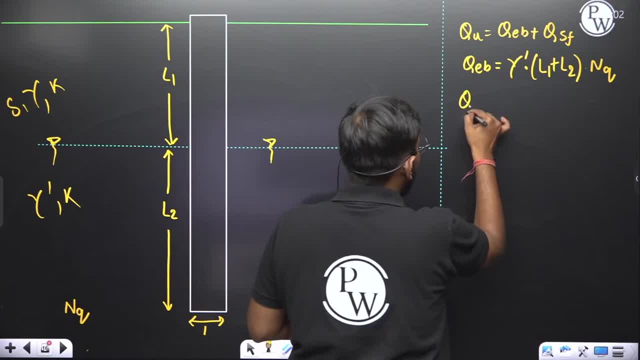 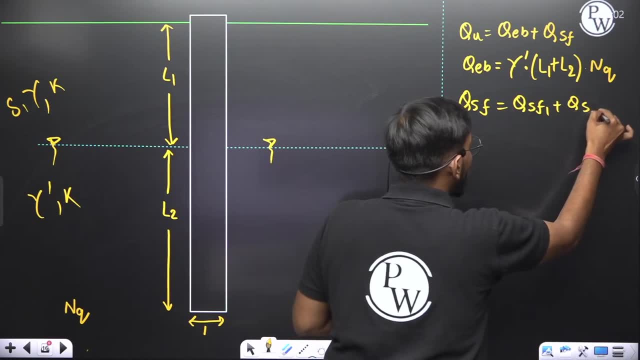 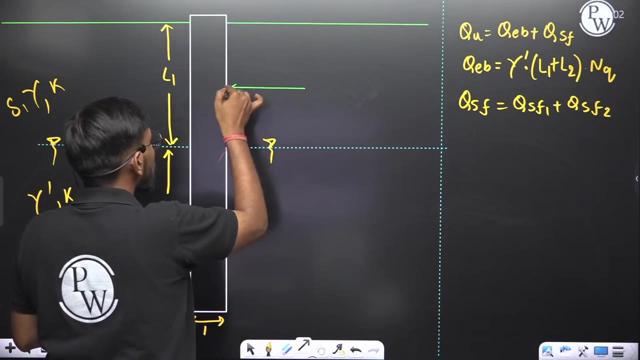 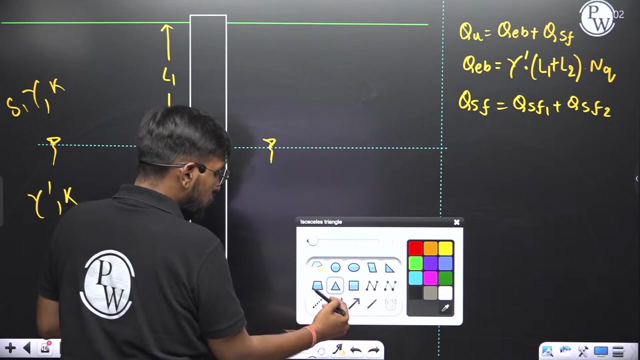 be done? next, I am talking about Q side friction, so I am dividing this in two parts: QSF1 and QSF2,. it is very easy, sir, understand it easily. understand it easily. If I make a diagram, we will focus. if I make a diagram, then how will my diagram be made? 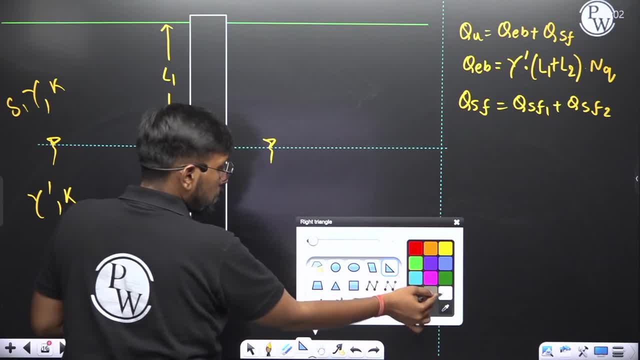 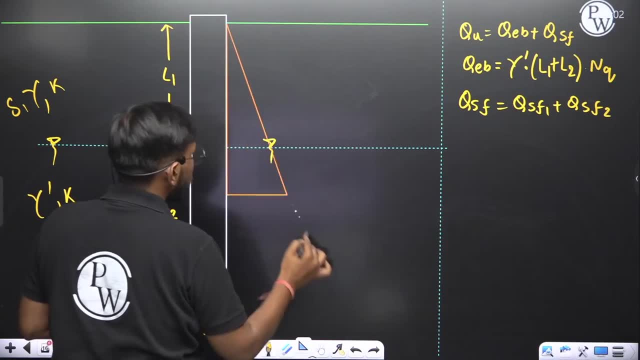 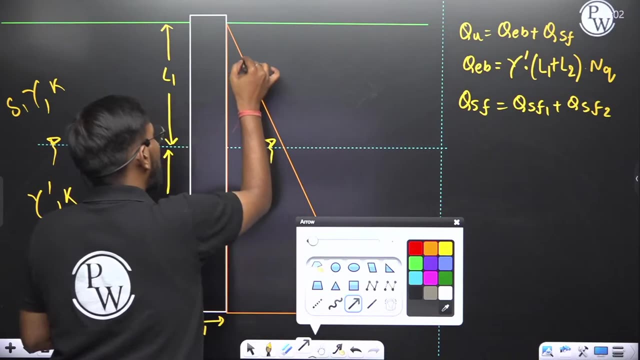 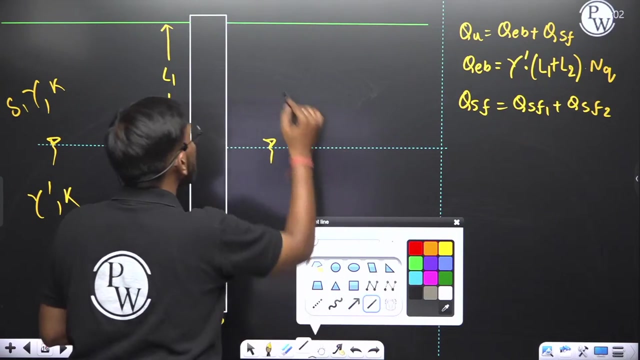 See, if I make a variation of horizontal stress, then it will be like this: we will not take the pressure of water here or we will make it separately, because there is water above and not below. we will make it separately, see. 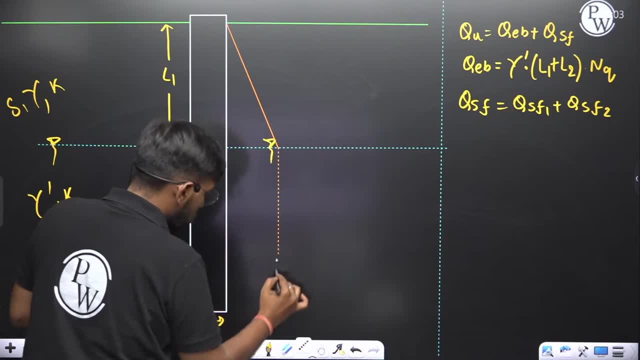 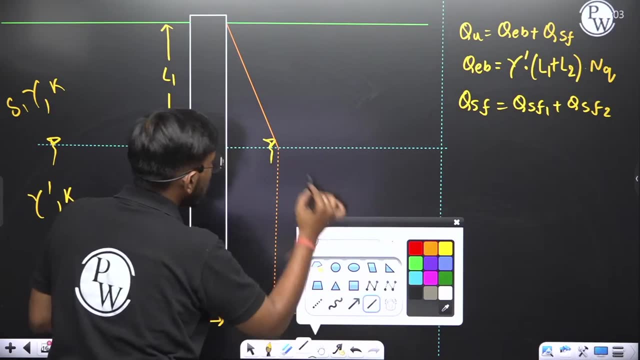 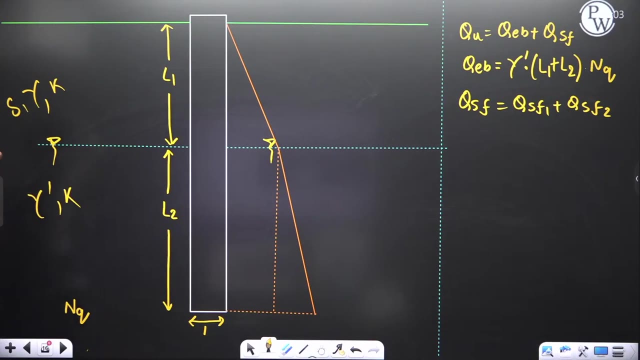 Digitization. so in this part, my friends, your value is the same. it is the same value, correct? Okay, You can see it here. Okay, friends, I have taken your value. What is your value? k, gamma, l1.. This will be it. 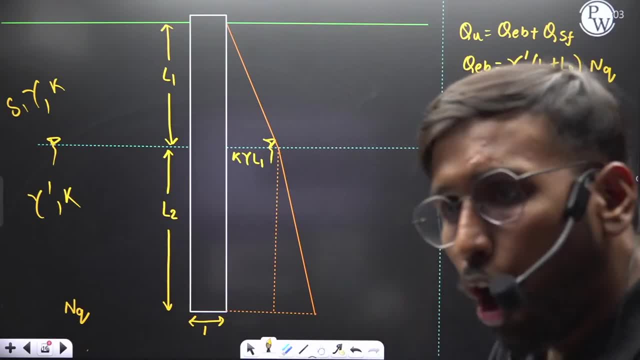 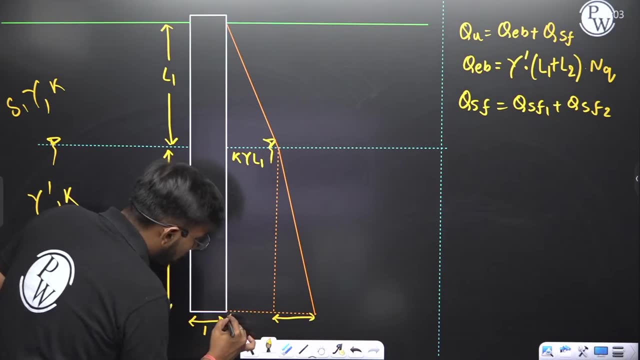 k gamma l1.. This will be it, And if I am talking about the second part, then what will happen here? First, your k gamma l1, as it is, has come. We have already read all this. And what is the second one, my friend? 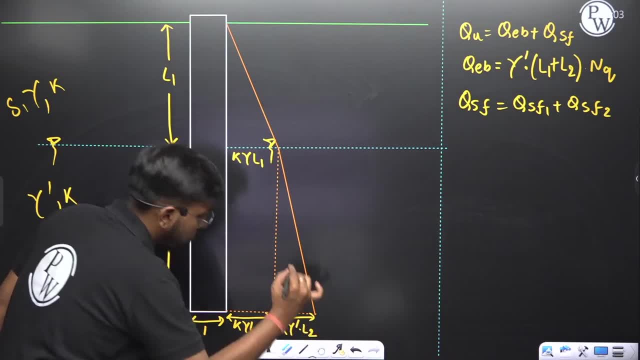 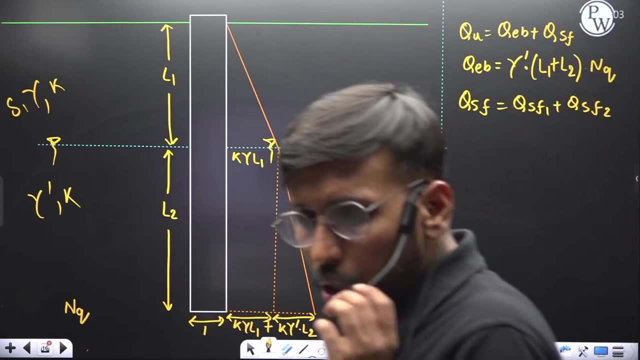 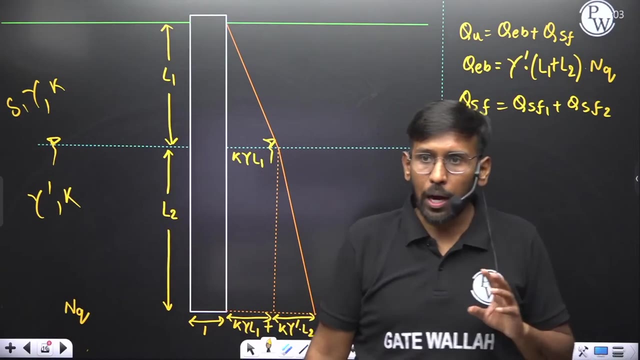 k gamma submerge into l2.. Tell me yes or no. Yes or no, One is k gamma l1.. Second, is your k gamma submerge into l2.. Right, So first of all we will talk about QSF1.. 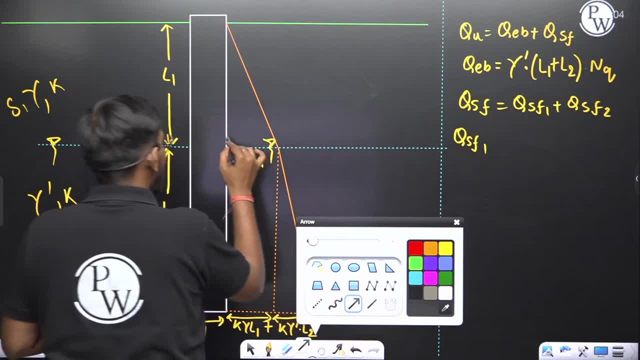 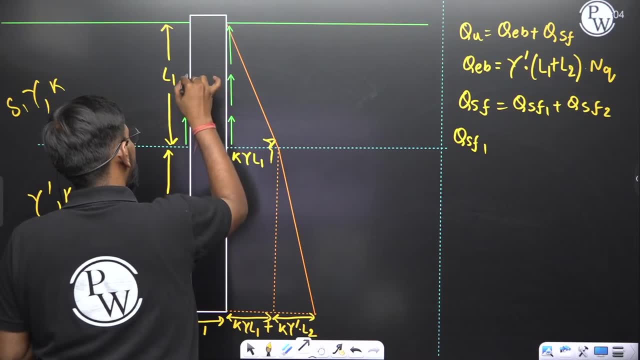 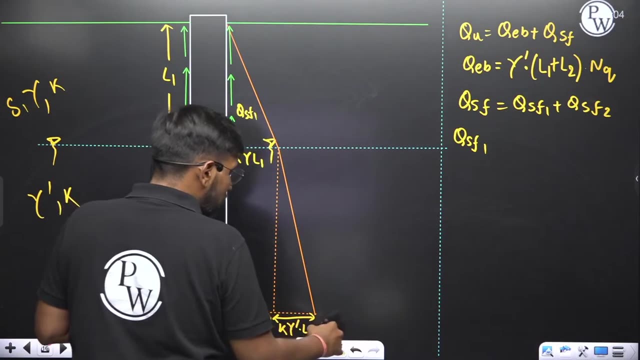 So where have you given QSF1?? QSF1 you have given here. What is your part? QSF1.. QSF1.. Okay, And what is QSF2?? What is your QSF2?? This part, This part. 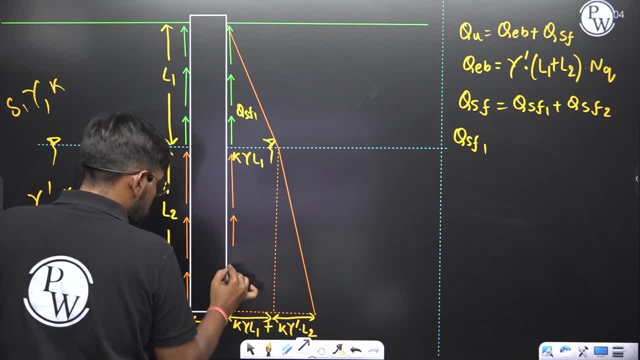 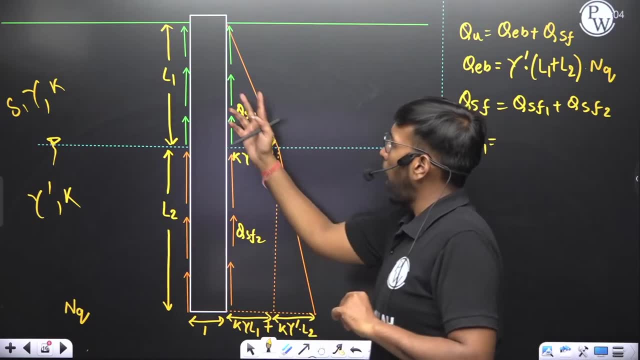 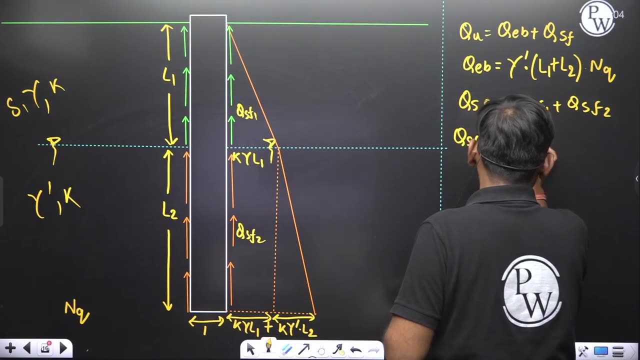 What did you call this part? This is your QSF2.. See here. So what is your QSF1?? If you see, you have to consider this portion only. So what will happen here? First of all, do tan delta for mu. 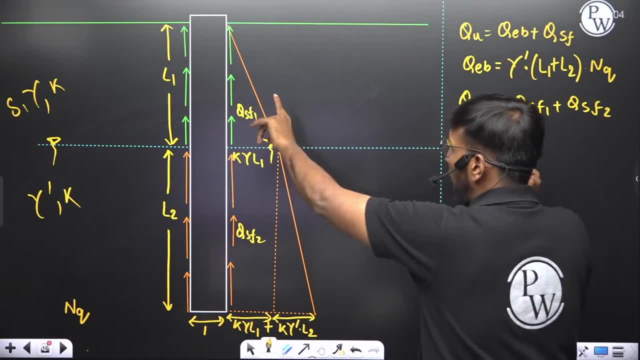 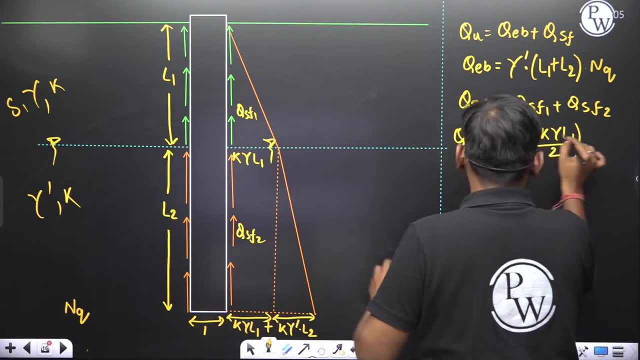 For n. first multiply the average stress with the area. So what is the average stress? k, gamma l1 divided by 2. And how much area is it taking? That is nothing but pi d l1.. Any doubt here? 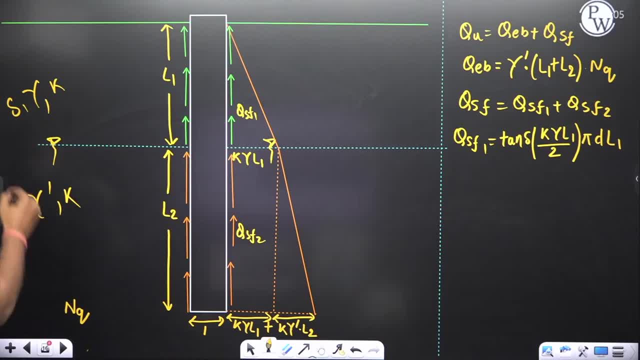 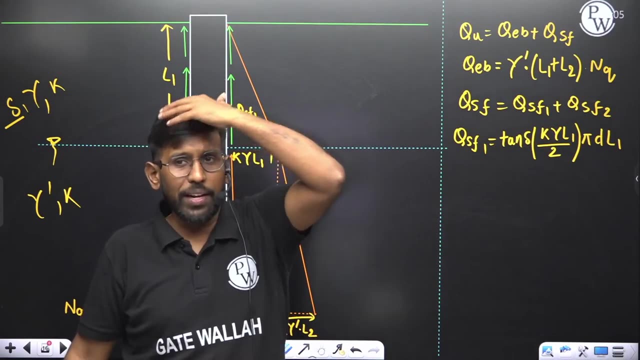 Any doubt here? Hey brother, delta is given only when phi is there. Think about it. Come on. Yes, brother, Is the point clear? So QSF1.. How did it come? Is it clear? Anyone having any doubt in QSF1?? 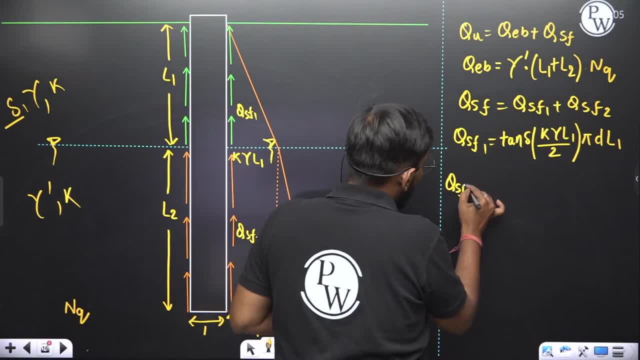 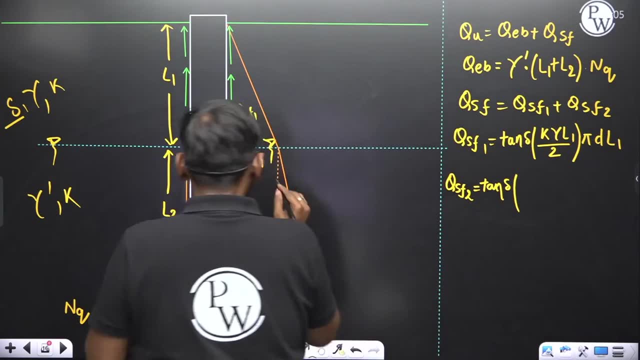 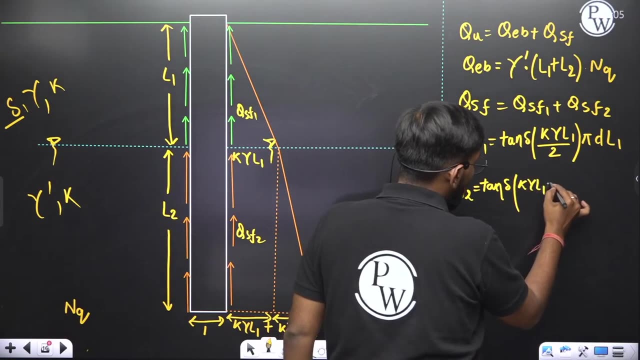 Next let's take out QSF2.. See here carefully: QSF2.. So tan delta, Delta is same. If you are talking about the average stress, then what is the average stress? k, gamma, l1. Plus. 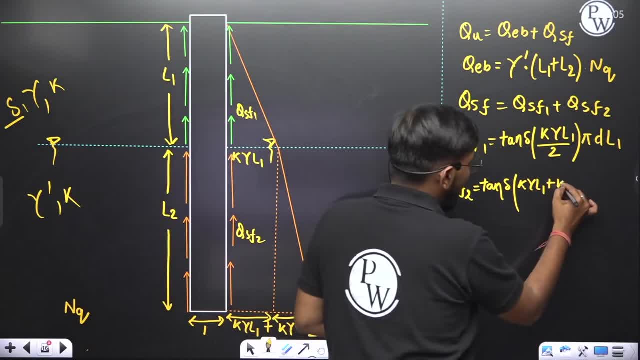 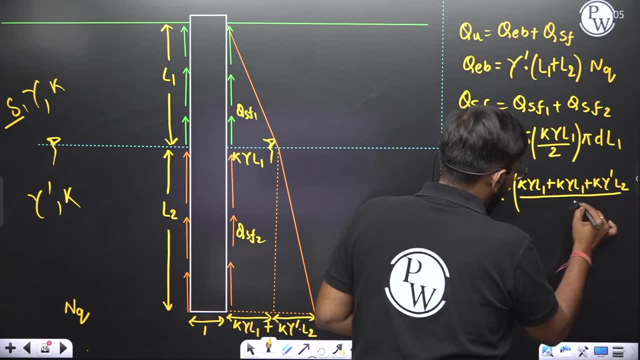 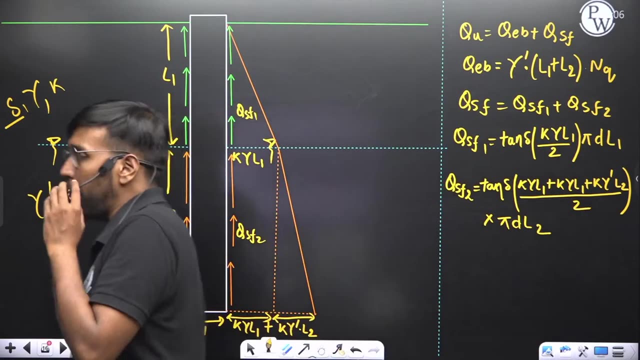 This lower value, That is how much k gamma l1. Plus k gamma submerge l2. Divided by 2.. This is the average stress And multiply with pi d l2.. Multiply with pi d l2.. 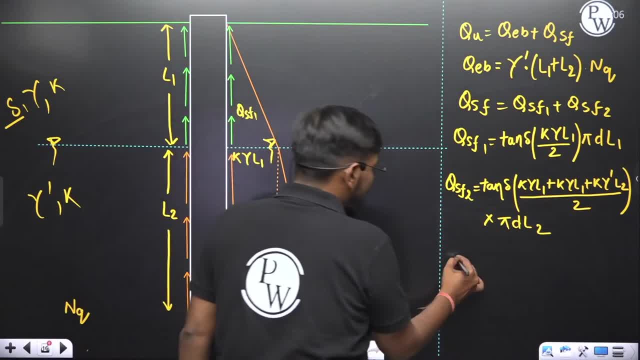 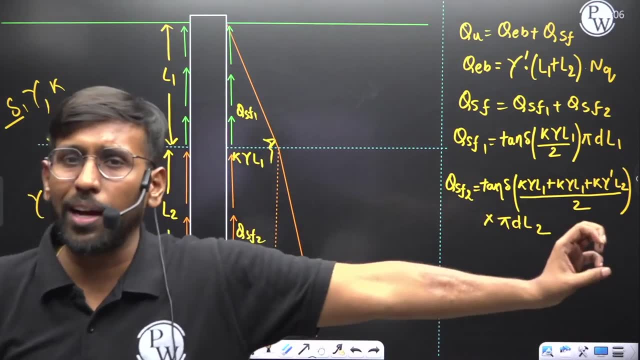 Hey sir, It is big just by looking at the formula, But is the concept also big? Tell me brother. It is big just by looking at the formula, But is the concept also big? Tell me brother. Is it clear? 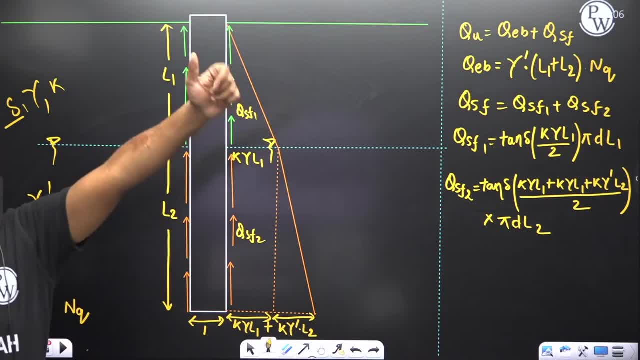 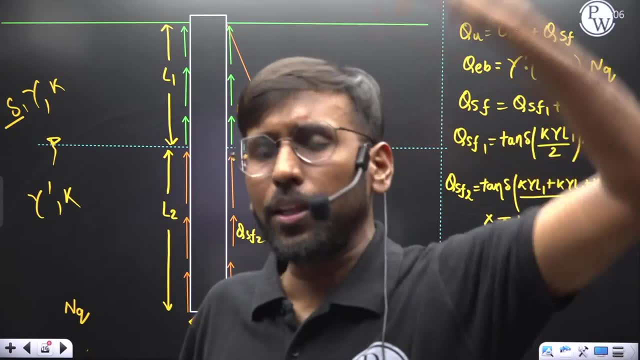 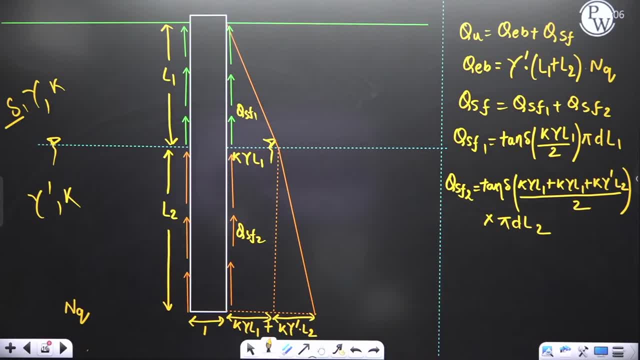 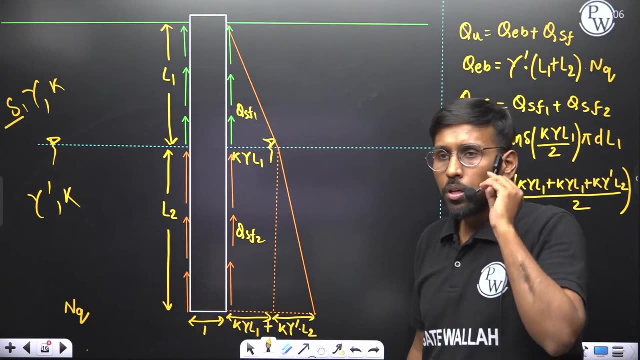 Yes, Today. it is all set in your mind. It is all set in your mind. Come on, come on, come on. Look, I am repeating again. There is nothing, Isn't it? Isn't it? I am retaining wall barrier. 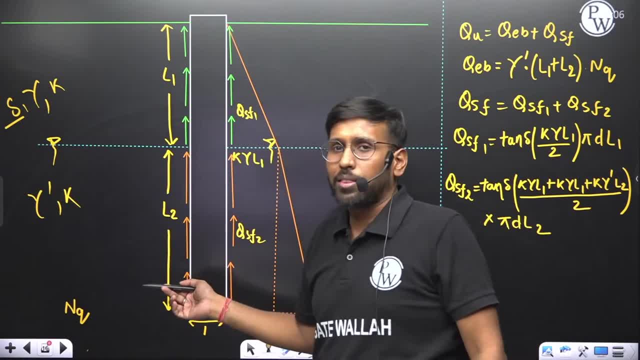 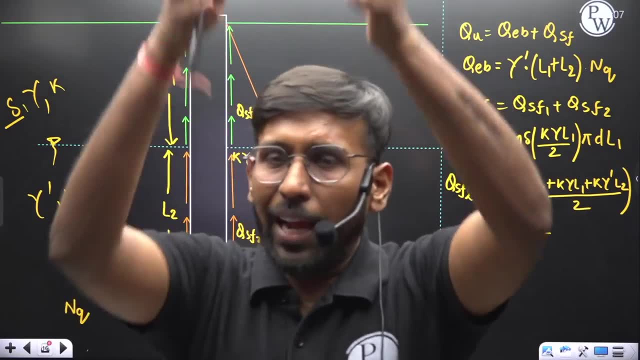 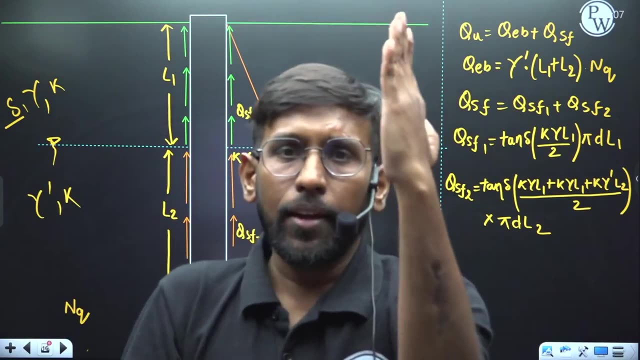 You stupid person. Horizontal pressure is applied, So horizontal is not sheer. Water is applied here. When you have tanks or gates, does water pressure apply on the gate or not? So it is normal pressure, It is not sheer pressure. 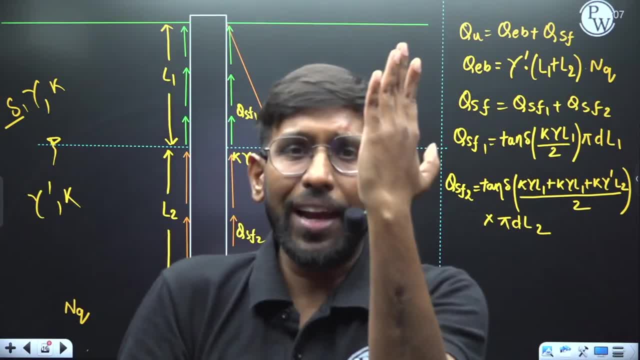 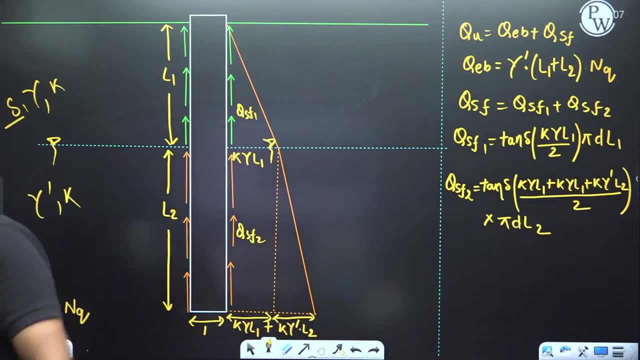 Water is not resisting in the vertical direction. It is sheer, It is horizontal, It is vertical, Then it is horizontal. The air pressure will come at the battery level Now in QEB. all this will be there Now. it will be at the end barrier. 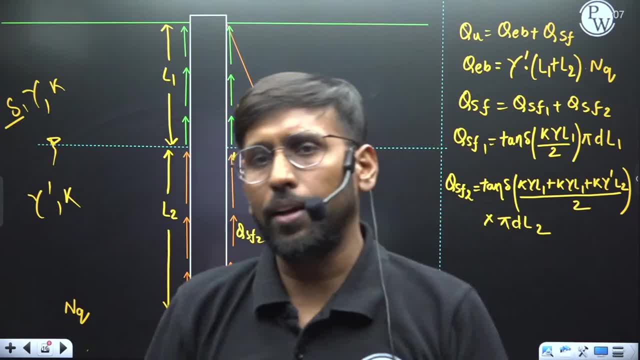 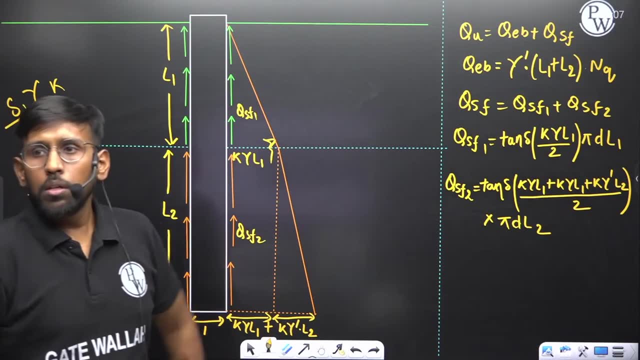 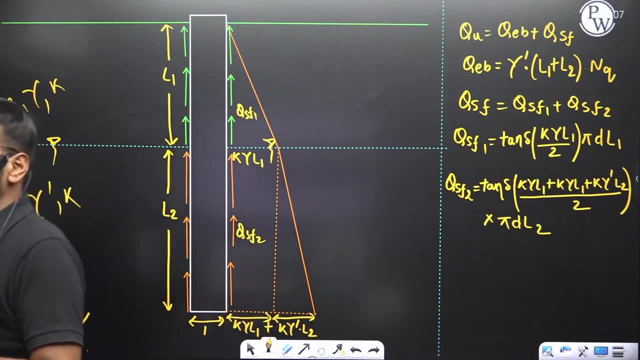 Now, why will it come in the QEB? Why will it come in the end barrier? I just said that It is applied like this. It is not applied on top. Come on, Is it clear? Is it clear? So it is nothing. 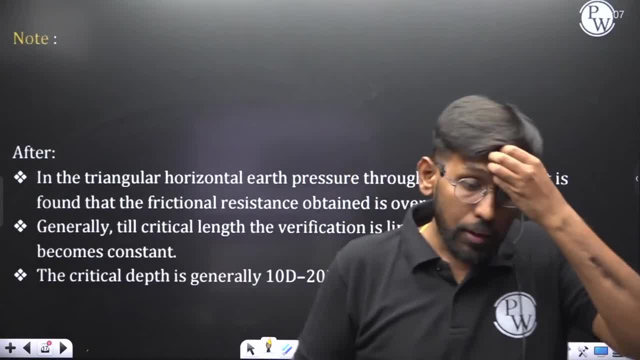 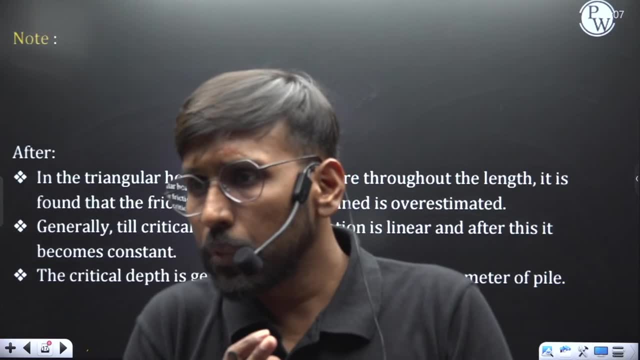 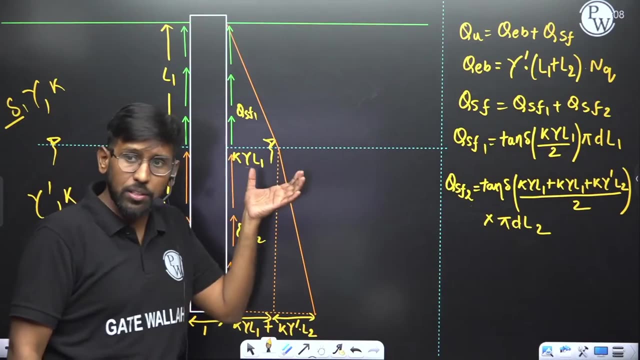 It is very easy, Everything is easy, Provided you understand. Here it is said again: what you are doing here is that you are underestimating. Okay, Listen carefully here, Sir QSF2.. Look, brother, Listen When you say revise, listen. 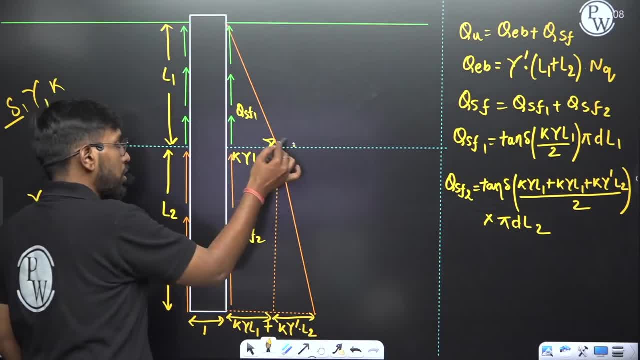 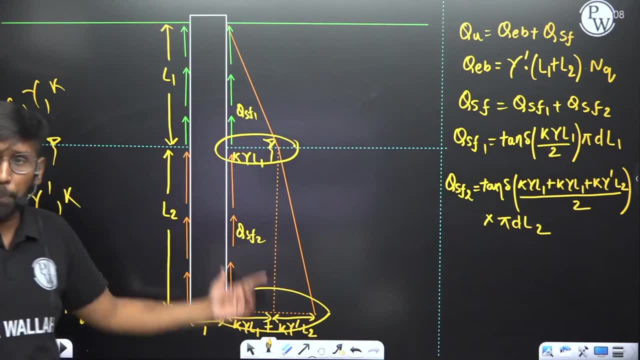 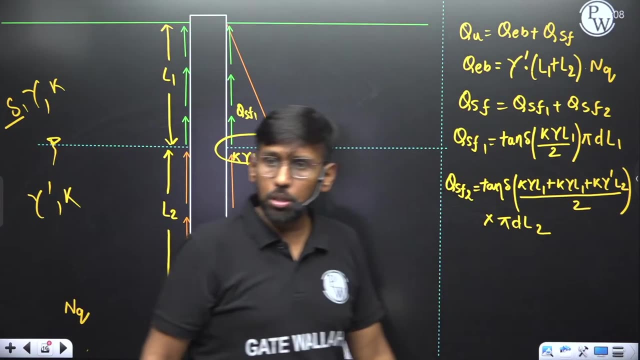 QSF2 is just the concept of average stress, right, So one stress minimum. this is the maximum divide by 2.. Minimum plus maximum divide by 2.. Finished Minimum plus maximum divide by 2.. Hey, is it clear? 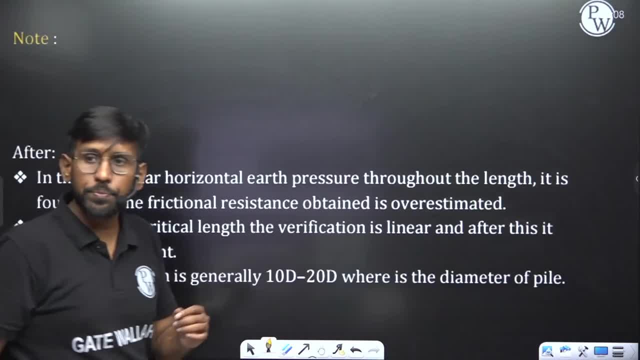 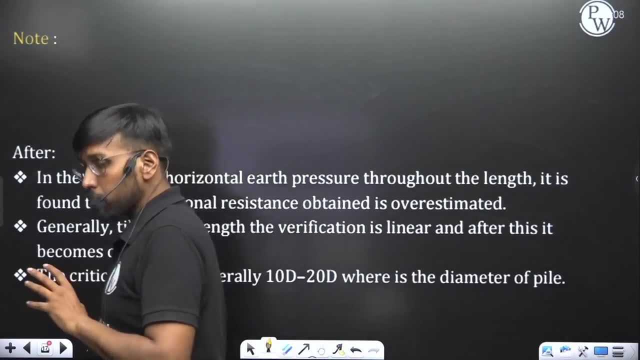 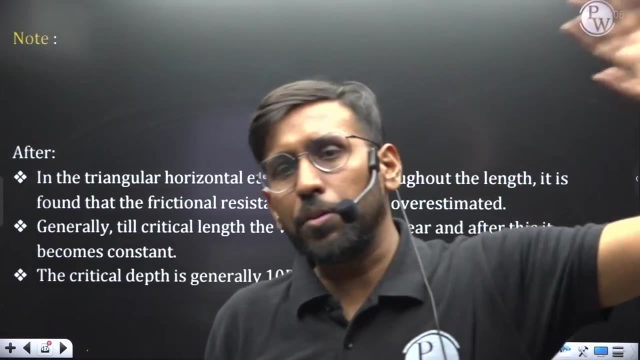 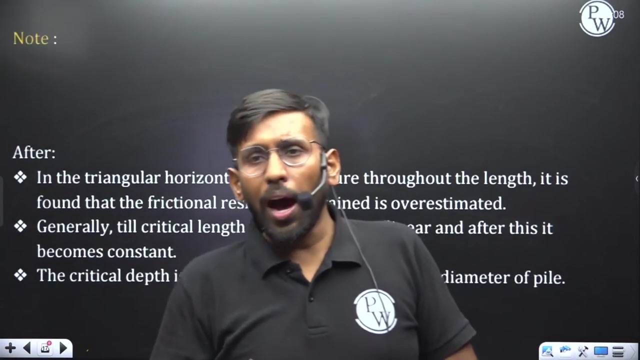 Is it clear? Look here. So what it says, what it says? that, sir, sir, what you are doing here is that the result you are taking is underestimating. So what it says? What it says is that this stress, after a certain level, after a critical height, this stress becomes constant. The stress becomes constant. Okay, The stress becomes constant. So this till a critical height, that is, 10 to 20 times of dia. There is a question on this too. Look here, Look here. what it says is that till a particular depth, this linear will vary, but after that it will be a constant. 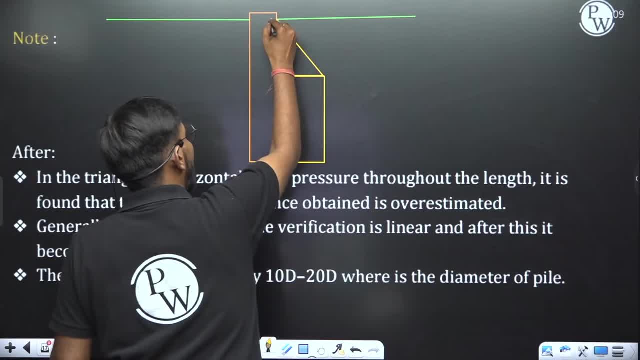 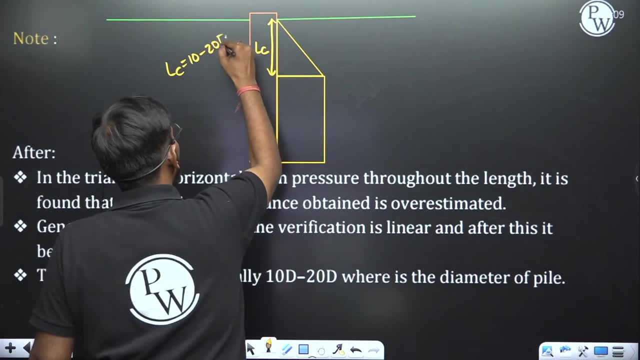 It will be a constant. So till a depth that is critical length, LC. What is LC? What is LC? 10 to 20 times of dia. This is your linear. it is varying After that what it becomes. 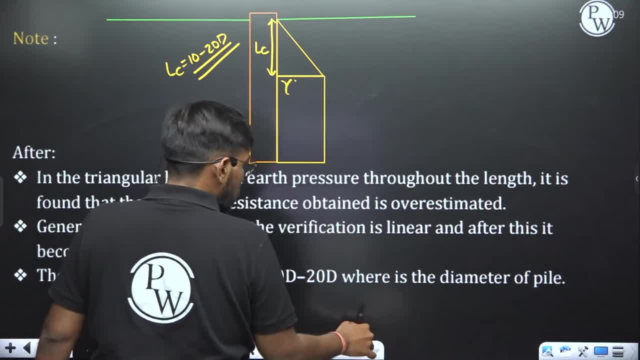 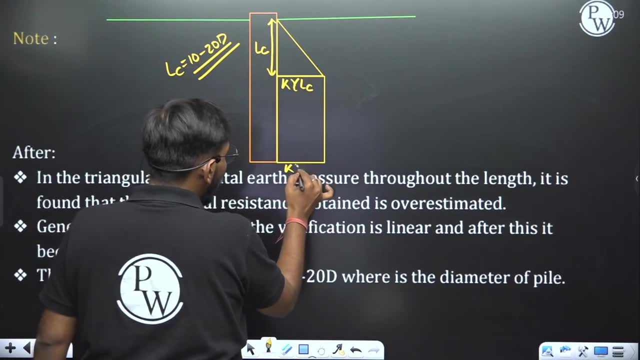 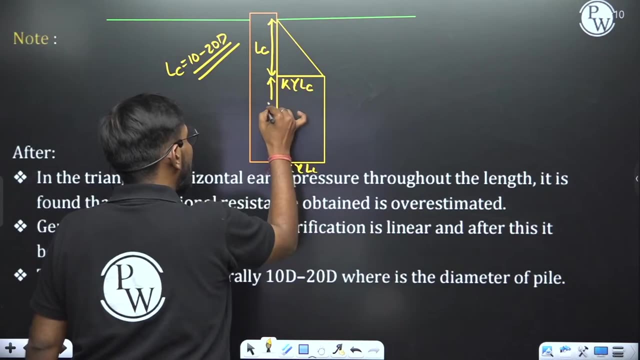 Constant, Like suppose, if we are doing gamma, if you have pressure, K, gamma, LC, So what it becomes? It becomes constant K, gamma, LC, Is it clear? So if I say that this is your L2, this length is L2.. 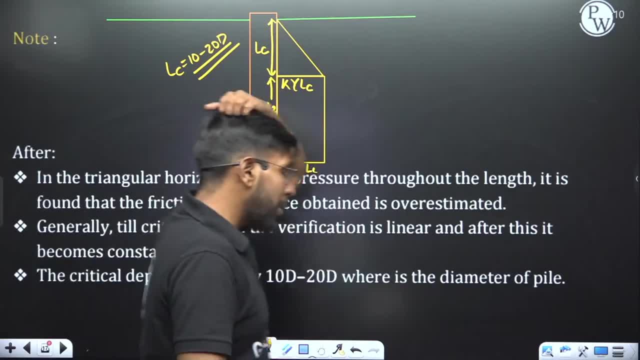 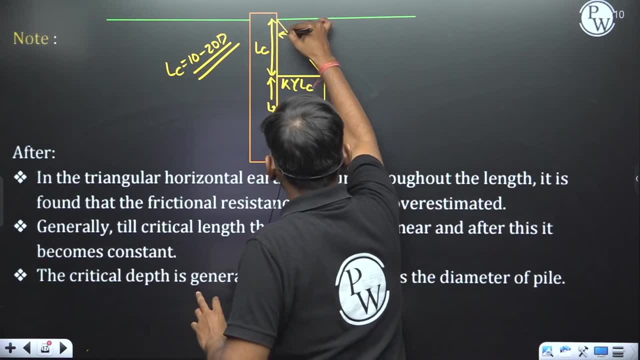 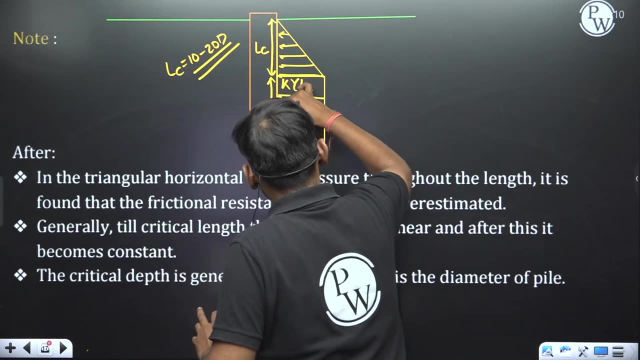 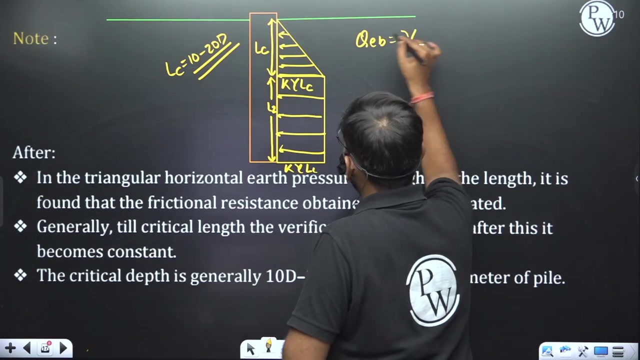 This length is L2.. Okay, Now, how will we write here? Just check, Just check, how will we write this question? Check how will we write it. The basic method is the same, sir. Your Q end bearing. that is nothing. but if I am saying what is your total length, 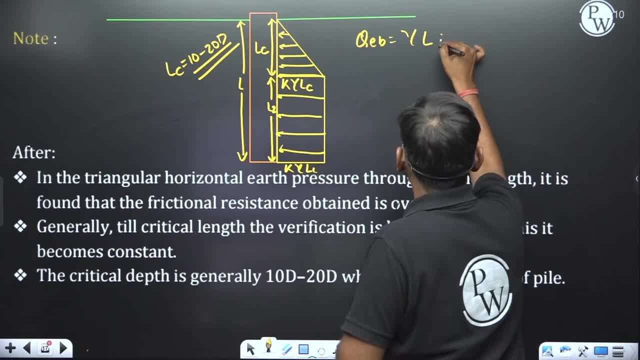 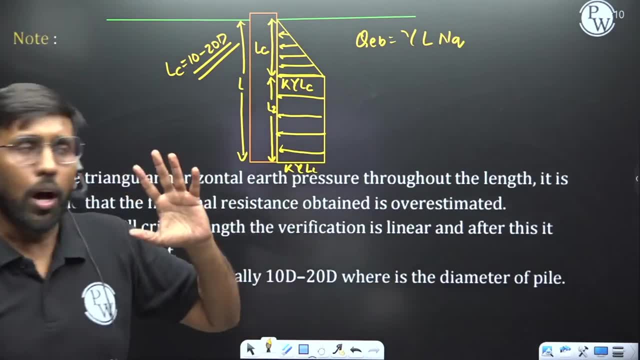 L, So gamma L and Q. This is Q end bearing right, This is your Q End bearing right. Now, my friend, if I am talking about what is Q side friction? so again, I am dividing this into two parts. 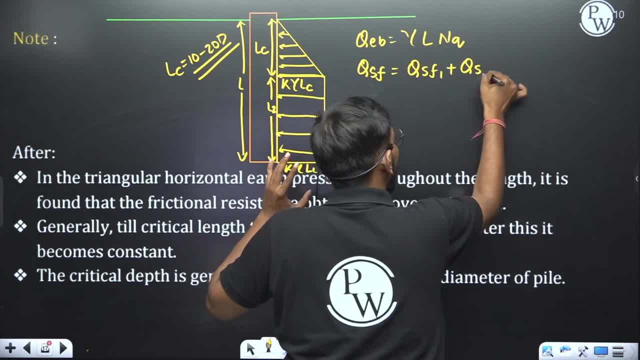 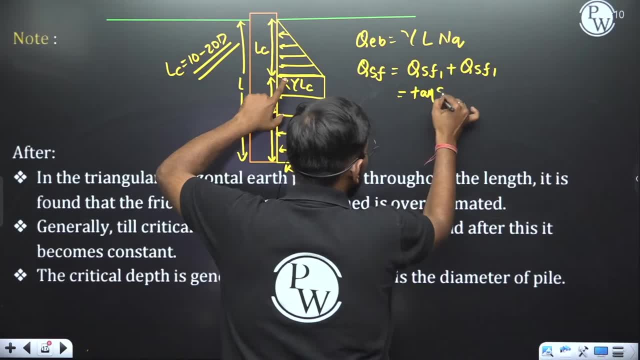 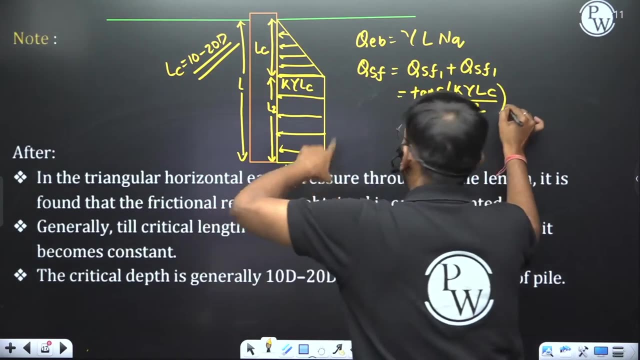 QSF1 and QSF2.. If I am talking about QSF1, then here what am I writing? Tan delta into average stress, K gamma LC divided by 2.. And what is the area on which it is acting? Nothing but pi D. 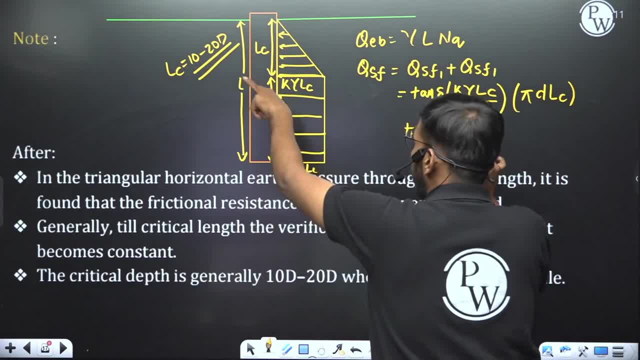 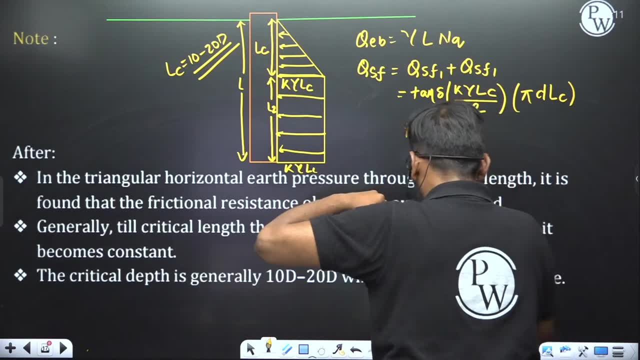 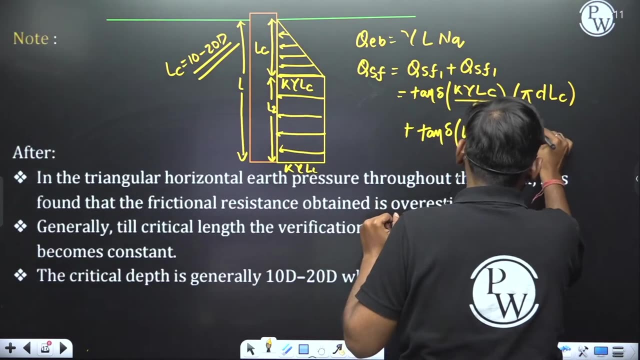 LC. No doubt Plus if I am talking about the second portion, so that is, tan delta K gamma LC. Will this be the average stress? K gamma LC. Will this be your average stress? Multiply with pi D into L2, not LC. 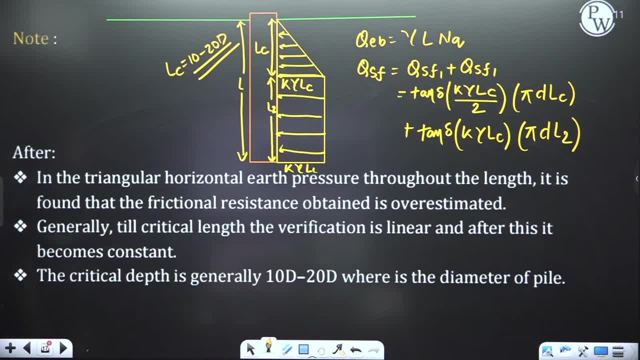 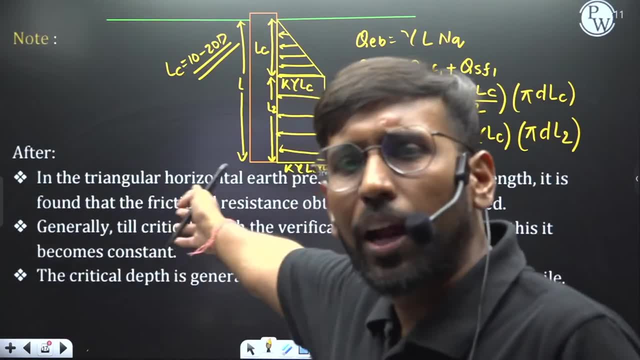 Multiply with pi, D, L2.. Tell me, my friend, did you enjoy it? So, sir, if you know a concept, then the biggest concept, you can learn it. the basic is, the formula is set here, No need to flip anything. 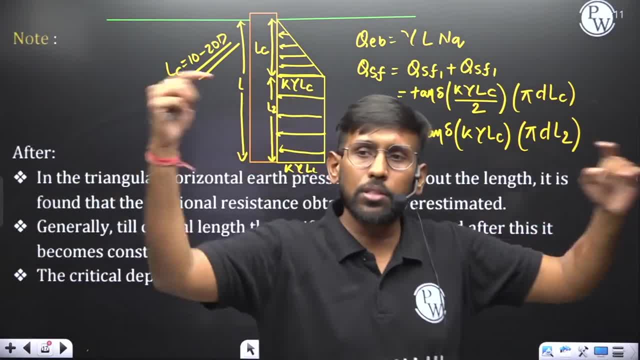 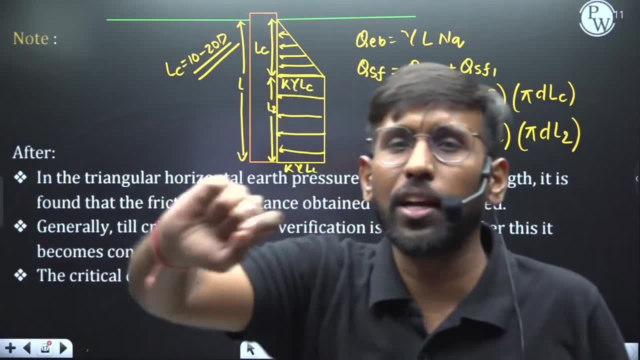 No need to flip anything. Everything settles from here. Everything settles from here, my friend, As I have already told, although it is written in the crash course. but I will not allow such a moment when the mind tells that the mind has crashed. 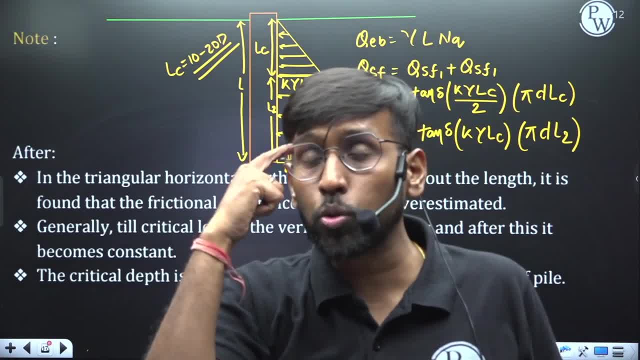 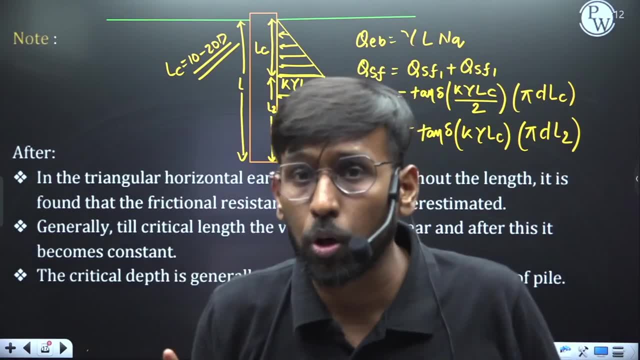 I will not allow for such a moment when the mind tells that the mind has crashed. Geotech: I have come to the end and I tried my level best that it would not have happened that your brain would have crashed in any concept. I tried my best. 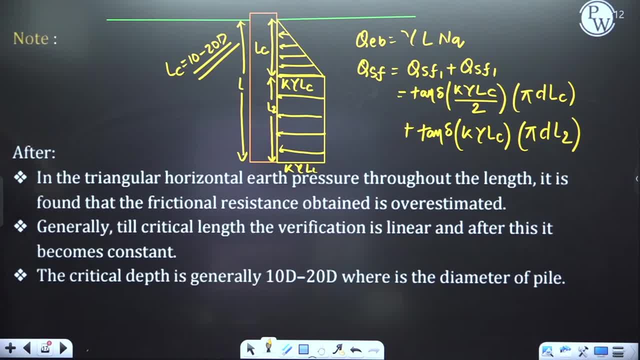 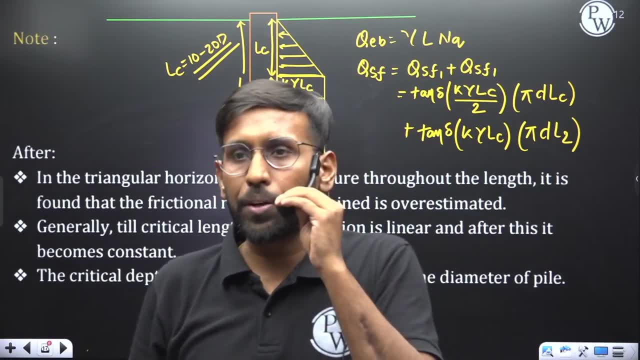 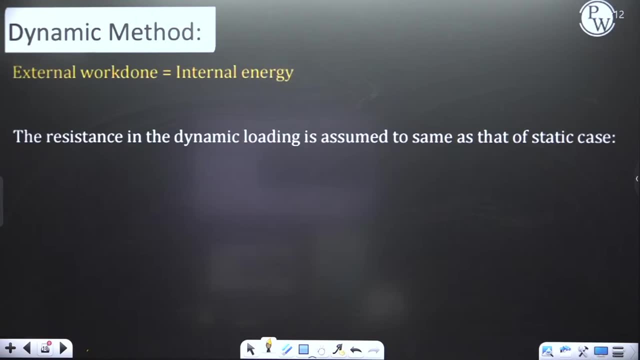 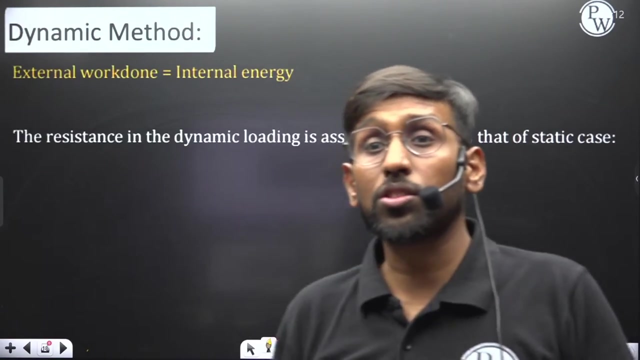 Come on, Come on, Okay, sir. So this phenomenon is called arching effect. We say this phenomenon as arching effect. Okay, So, if I ask you in objective, then Okay, So this is about your analytical method or static method. 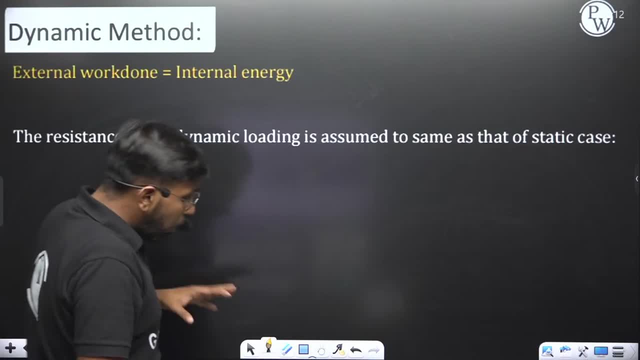 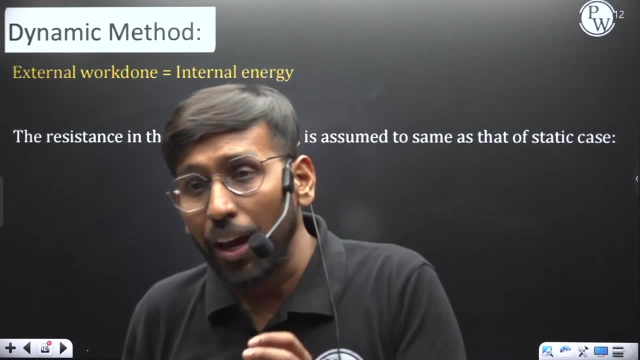 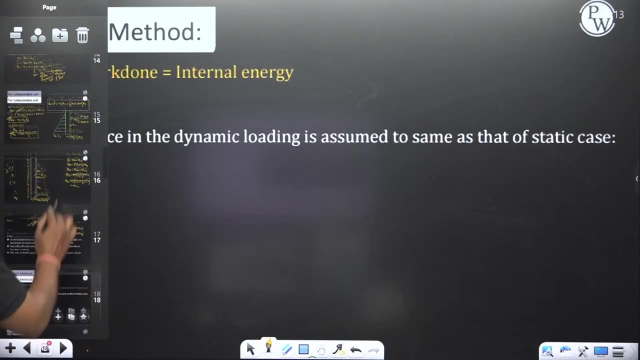 Okay, Now what we are going to learn is the dynamic method. What we are going to learn is the dynamic Motivation is needed. You guys have a lot of motivation. How can you get demotivated so much? How can you get demotivated so much? 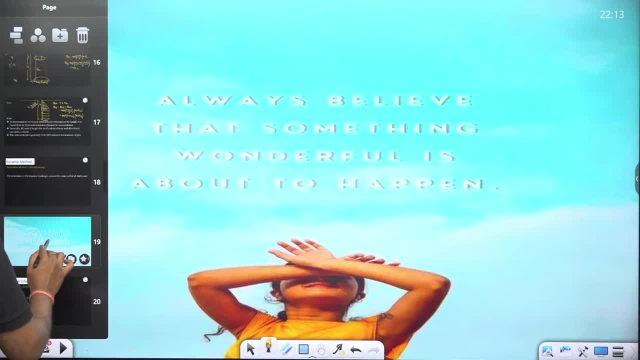 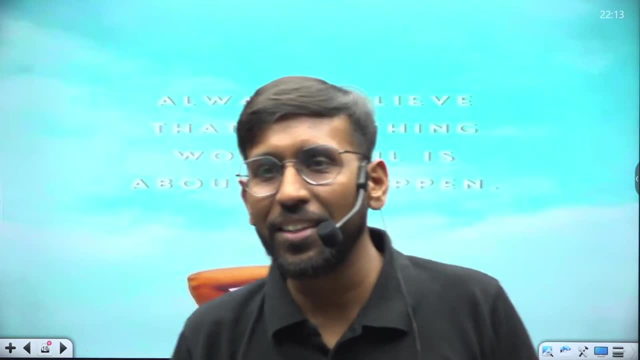 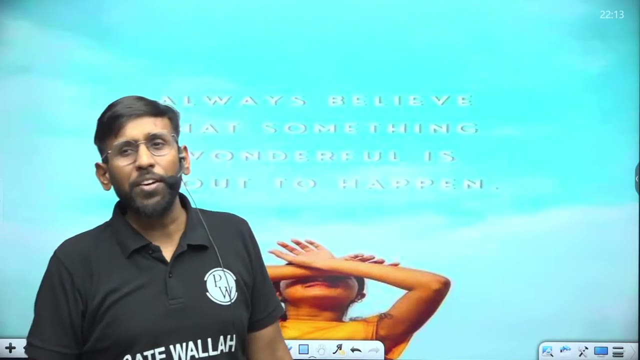 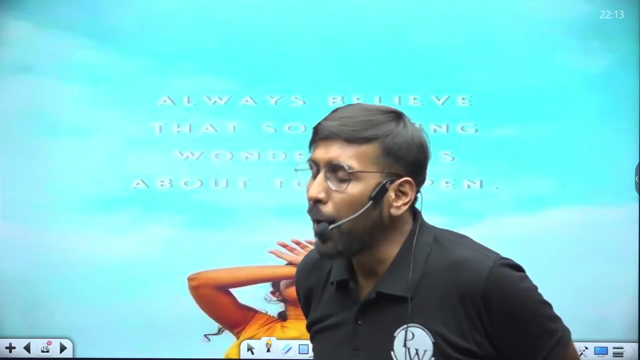 Please bring it up. How can you get demotivated so much? You need motivation every day. See here. So what it says: There is a line: Always believe that something wonderful is about to happen, Right? What does it mean? 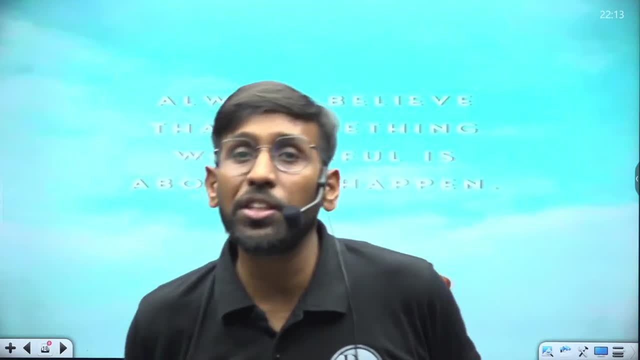 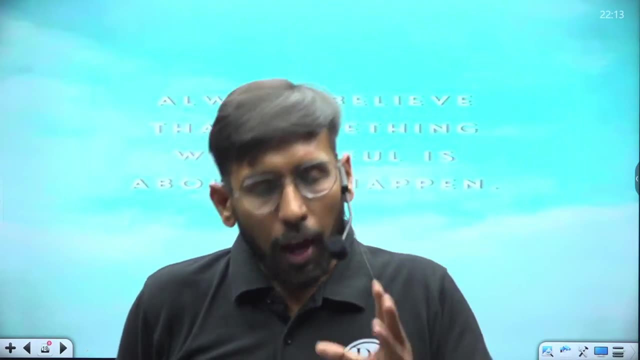 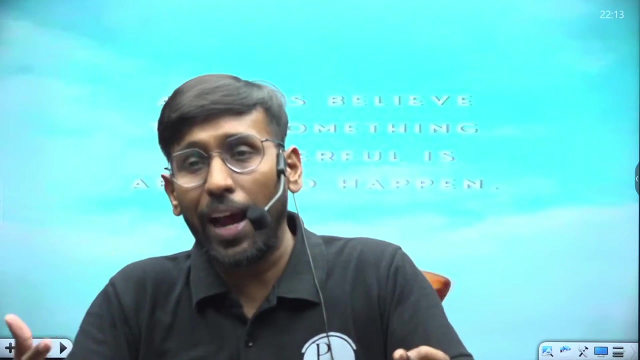 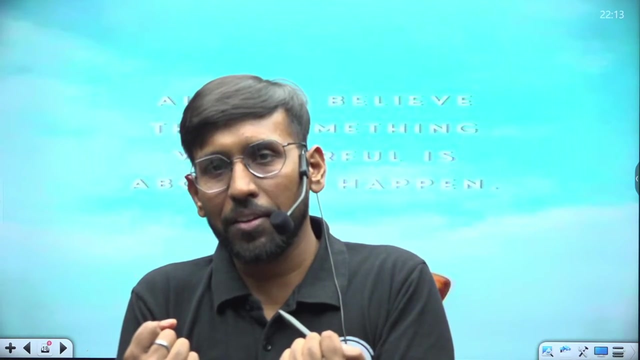 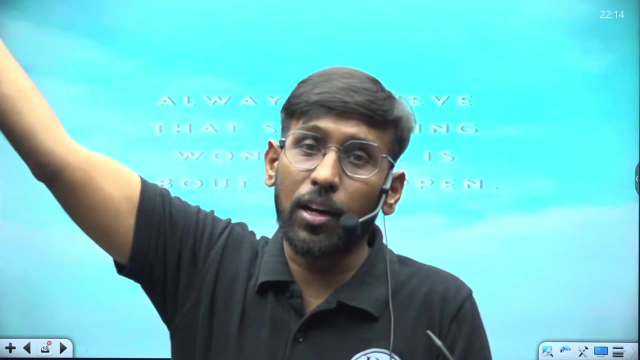 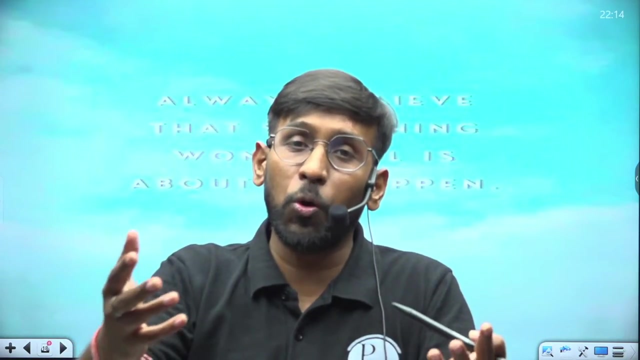 It means that we always have to stay positive. No matter how tough you are in the situation, always think that tomorrow will bring happiness for you. Tomorrow will bring good energy for you. They say good days will come. Good days have come The teachers. you used to pay lakhs of rupees to study. today you are either studying on a free platform or you are studying in a paid course of 5000-6000 rupees. 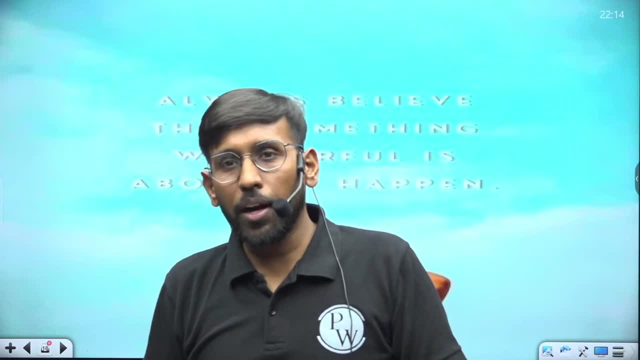 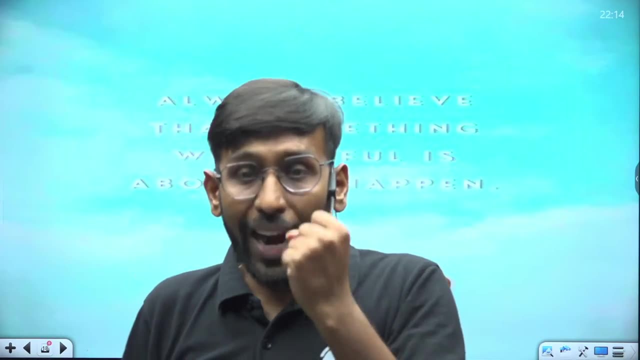 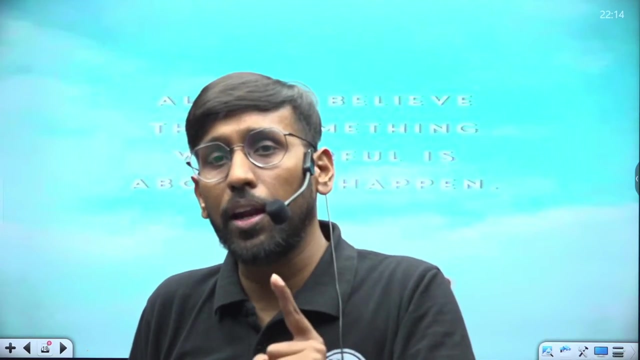 These are good days. What else do you want? So, my friends, the time has come. You have to believe in yourself that, yes, you can do it. That belief you should have in yourself, That belief you should have in yourself, The place we are standing at is the best place. 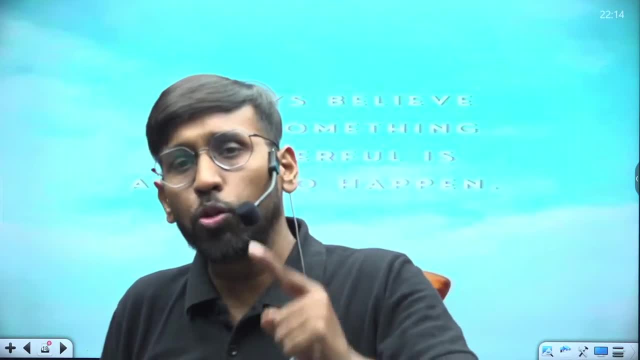 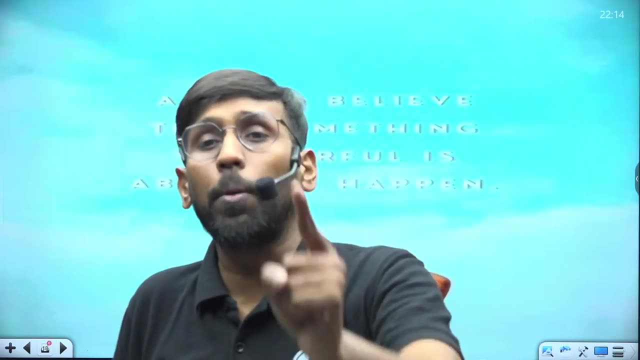 That belief you should have, that if we are there for the next 2-3 months, we will get results in it. But it will only happen when we will not let go of any shortcomings. It will only happen when we will not let go of any shortcomings in our side. 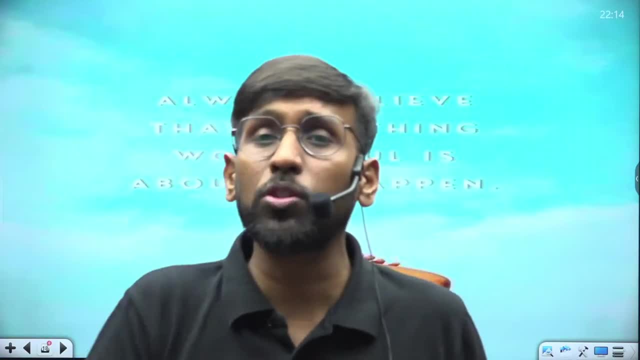 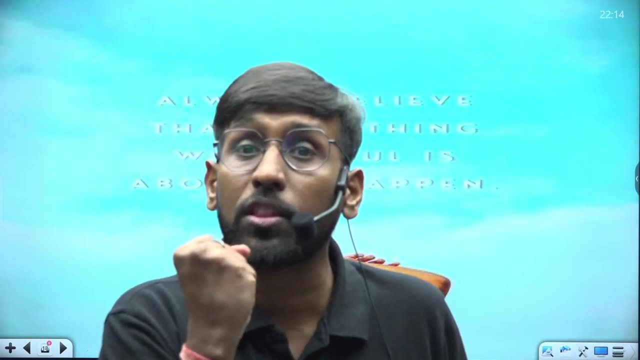 We have to make a promise to ourselves, to give 100% of ourselves. We should not lag on any day. Catch these next three months, Take these three months. tumhara hai aur jo Diwali jeeno ne nahi manayi hai na. 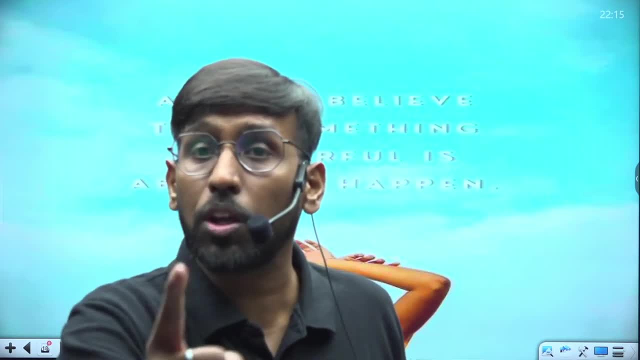 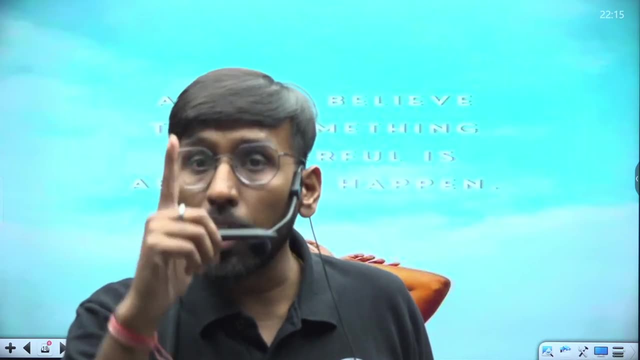 yeh aapko bharosa dilata hu. result wale din tumhari Diwali hogi. result wale din tumhari Holi hogi. yaad rakhna hi baat: be positive in your life. Surya har din set karta hai. 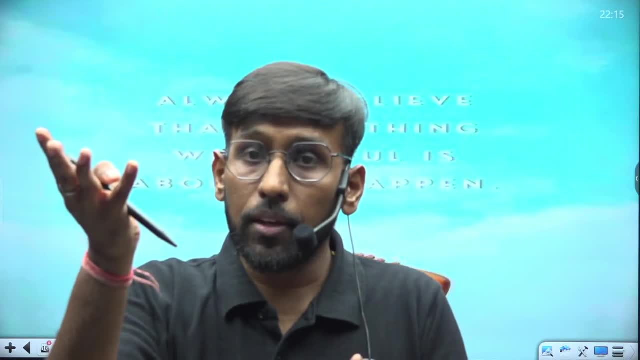 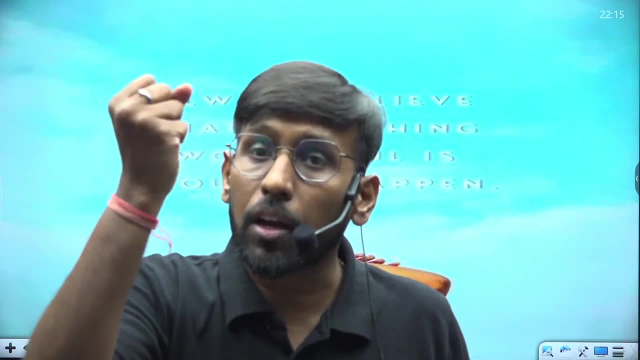 aur agle din purja paida karta hai. har din tumhara saath hoga. aap padhoge, demotivate hogue, lekin kuch aisa aapke saamne khada rahega, aapko wapas se lift karne ke liye. 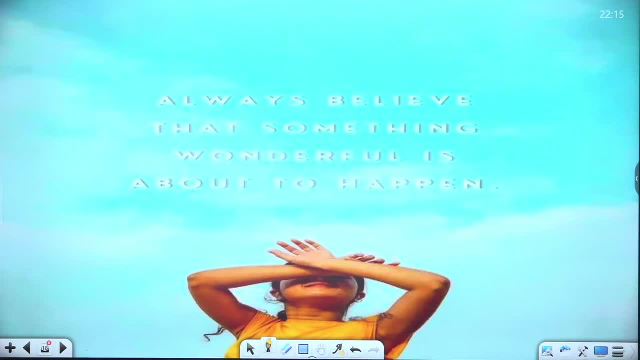 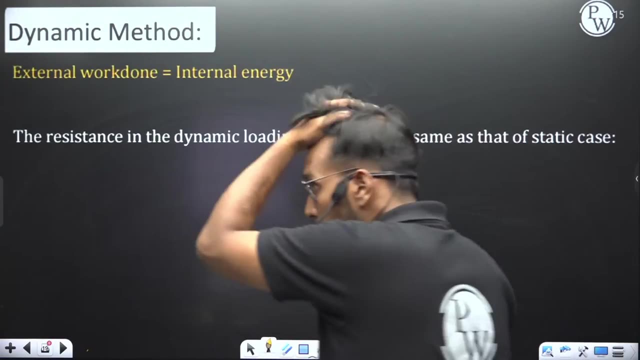 kiyaad rakhna hai. jeevan me baat chal ye, let's start, let's start, dekho aap hai, dekho aap hai. so, mere dost, dynamic method me ham kya kar rahe, jitna ham kya boor rahe. 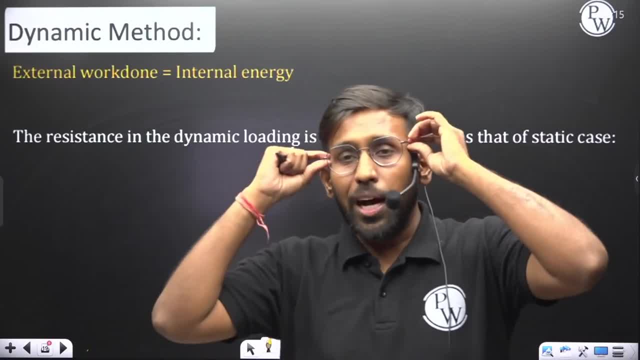 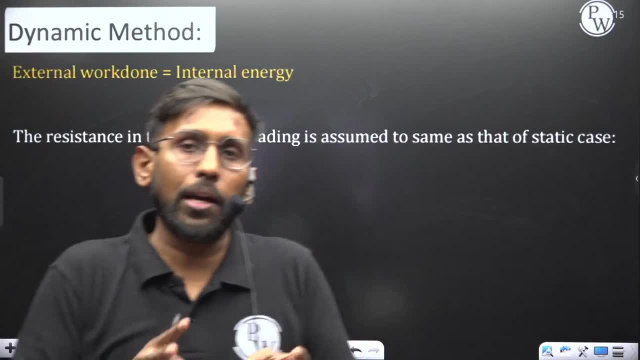 jitna ham kya boor rahe, jitna bhi external work done hai, jo bhi aapka external work done hai, wo saara store ho jaada hai in the form of internal energy theek hai, wo saara store ho jaada hai in the form of. 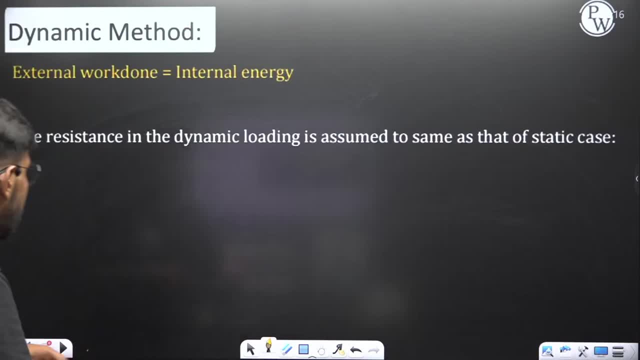 internal energy theek hai. aap samjhoge yahaan pe dhyan se. let us say: ye, aapka pile hai. this is the pile, aur iske upar se ek load aa raha hai. hammer. this is the hammer of weight w falling from a height h. 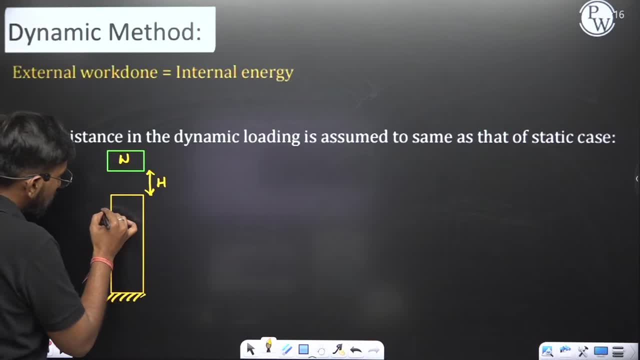 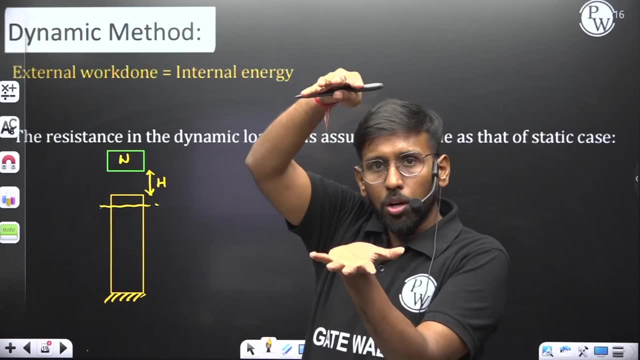 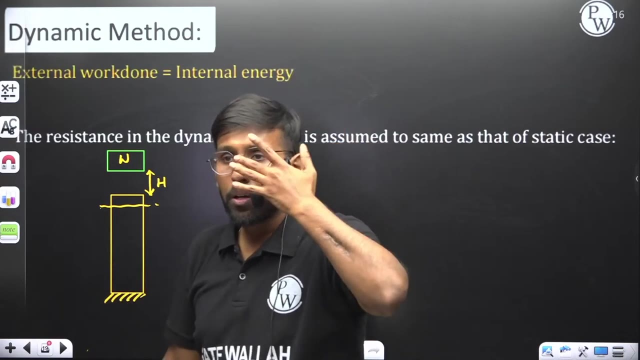 theek hai. toh is height ke height ke height hai se height ke karan. another thing was applied: yeh kuch kneeche jayega and also jo pile hai wo shed karega. the pile will penetrate by some amount in the ground, yes or no? 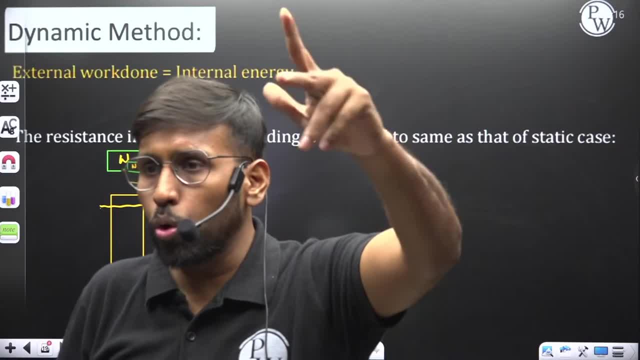 the pile will penetrate by some amount in the ground and also there will be deformation of the pile. dono hog ga dekho h aapo hai. dekho h aapo hai in pile hai dh�o pe dekho h aapo hai. 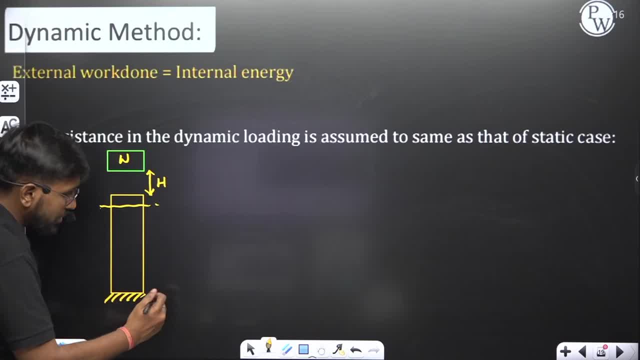 mah sekarang maire dost, so mere dos thikult ko hai pe ha kare. the pile will penetrate inside the. this is the penetration per blow. this is called as S set, or there will be. there will be a load will be applied then further. what will happen? 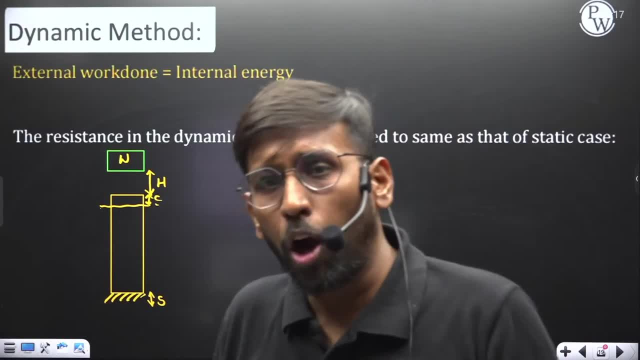 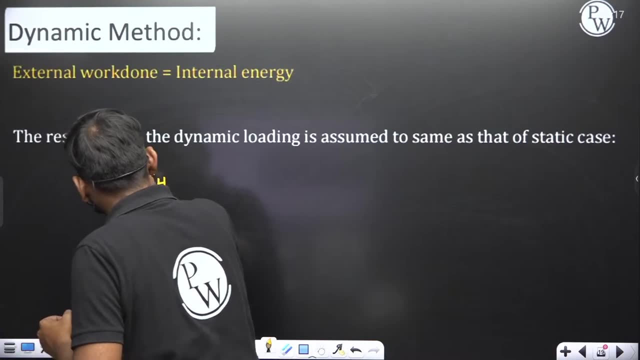 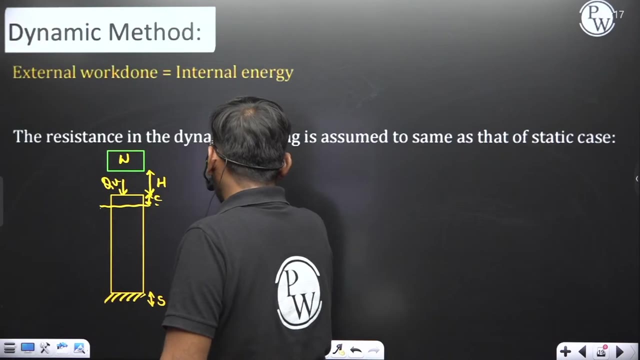 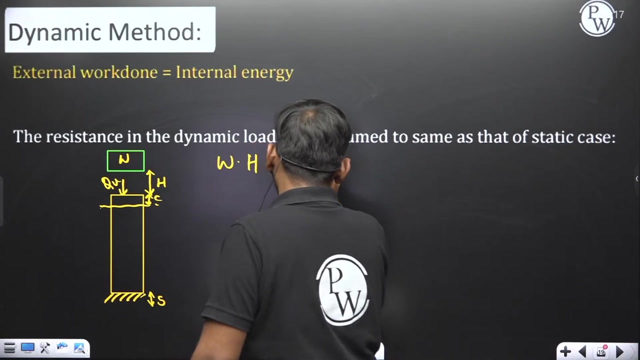 deform will be done, because we are dealing with the deformable body, we are not dealing with the rigid body. if I say the load carrying capacity is, if I say that the load carrying capacity of so what done? external kitna hai or agar me isko equate kar doon. 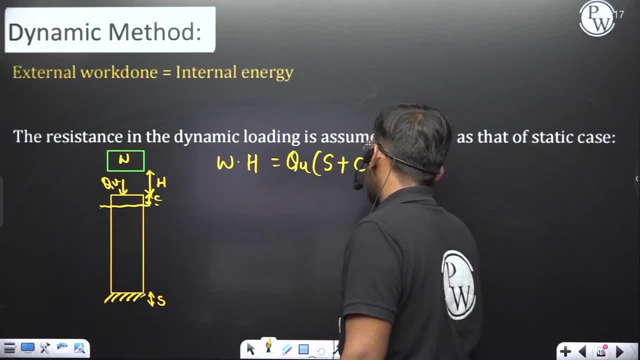 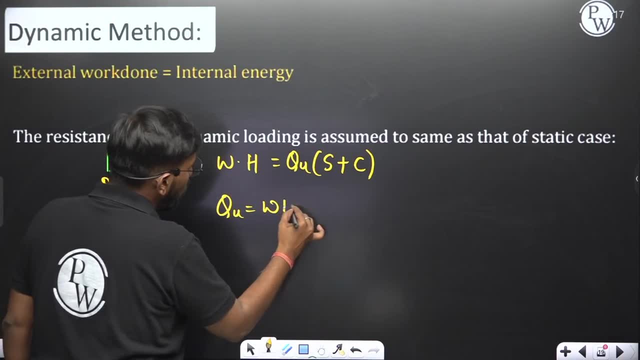 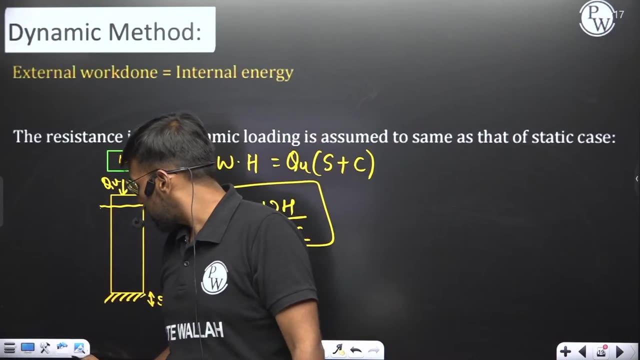 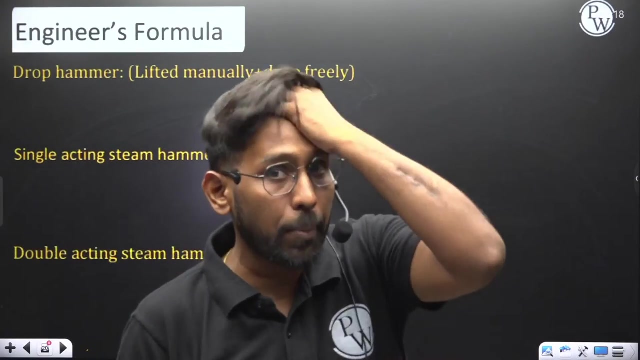 Q ultimate into S plus C, Q ultimate into S plus C. Q ultimate is equal to upon S plus C. a general formula is equal to this way. this is the way to remember see here. so, my friends, here the hammer is of three types. one is drop hammer. 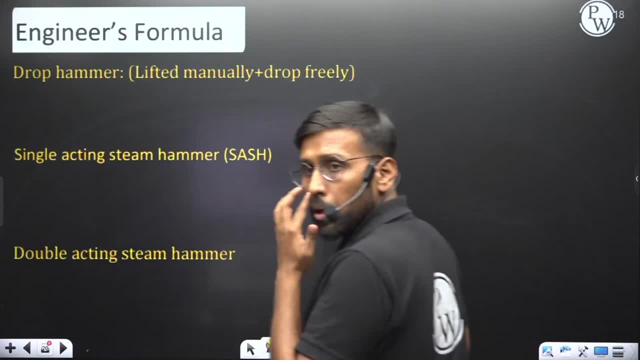 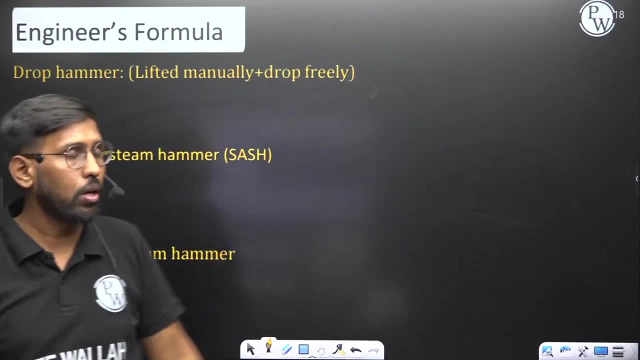 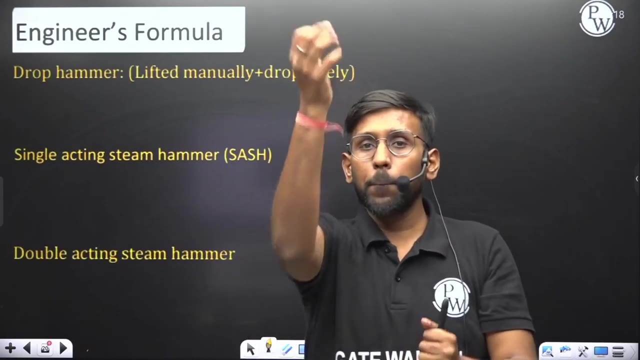 drop hammer means what happened: drop hammer, drop hammer. brother, I do not have to go that much, I do not have to work that much. will volumetric change or not? see here. drop hammer means what happened: lift, you have done free drop. we have lifted the hammer and dropped it freely. 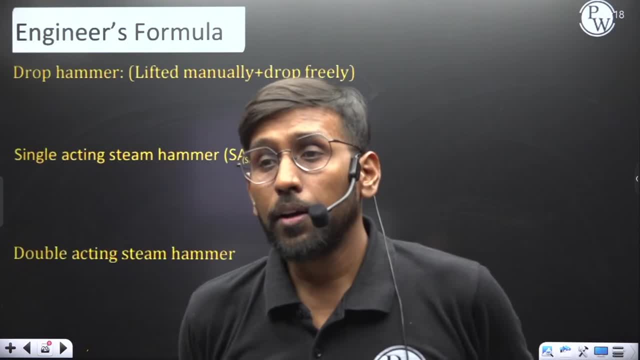 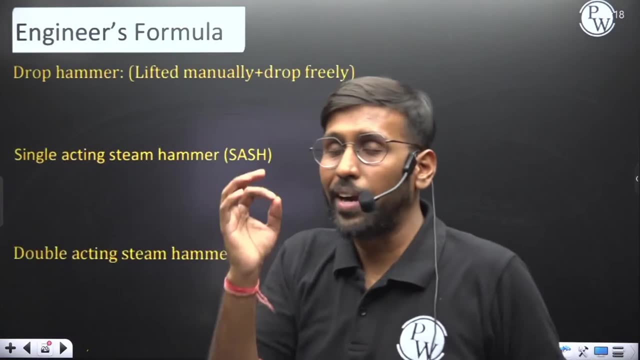 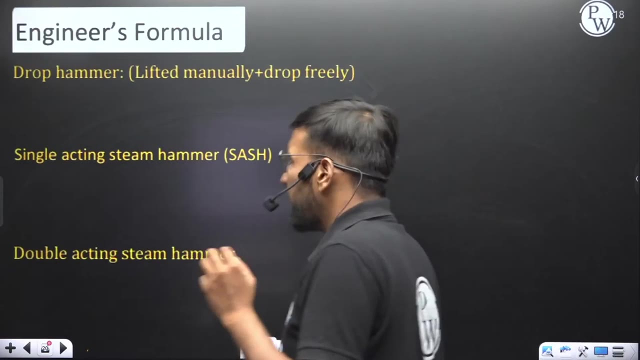 remember what was the test in which you did? you lifted the hammer and dropped it freely. very good, Aditya. very good. standard penetration test: very good, what a great. Amit Bhave- very good, what a great, what a great sir. this feeling came that what happened? this thing you said. 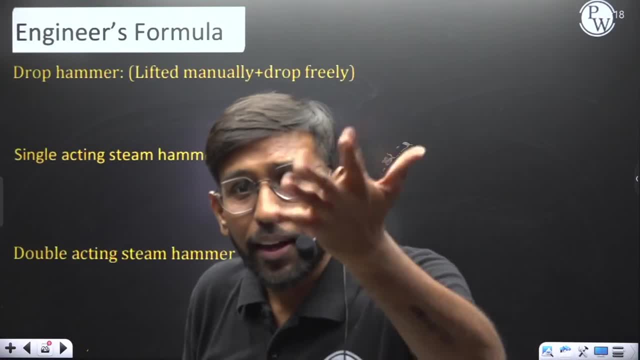 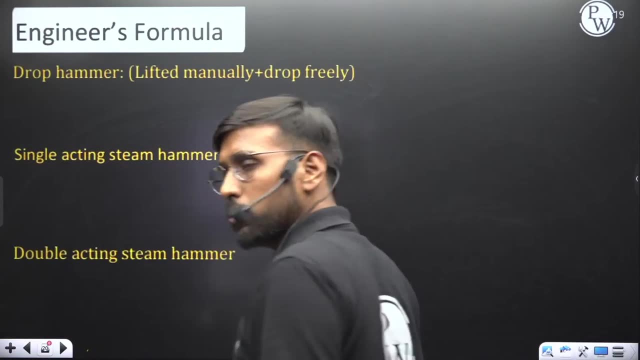 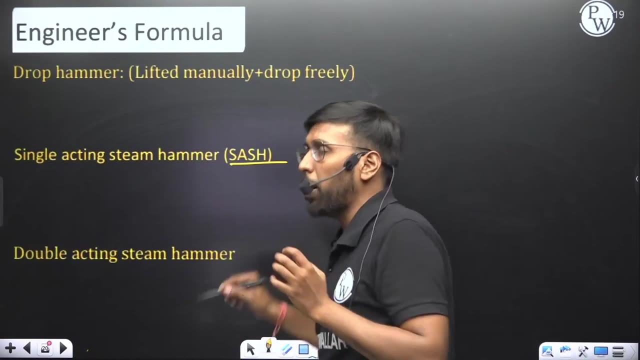 this came from the visualization. this did not come out of nowhere. those who visualized it came to them. the rest come on see here. so this is in the case of drop hammer. ok, now if we talk about the next single acting steam hammer. so what happens in single acting steam hammer? 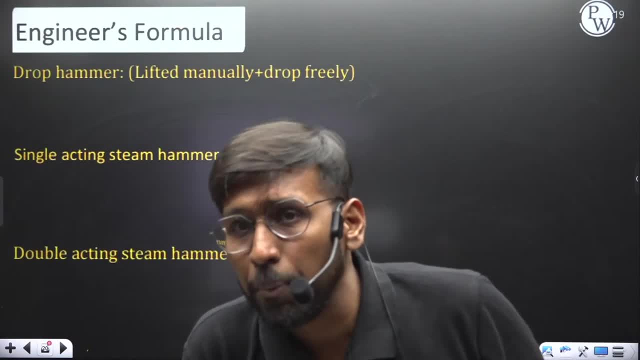 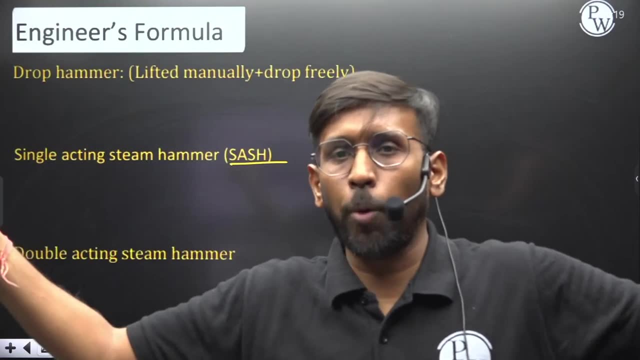 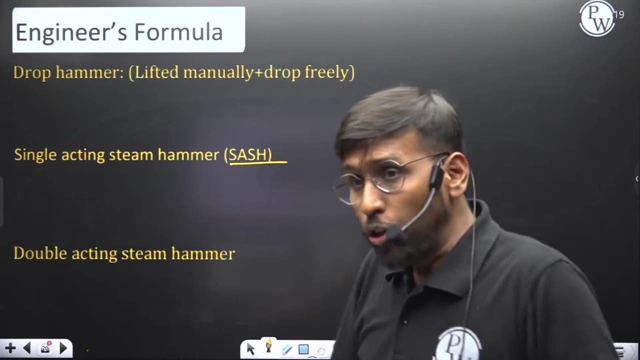 what happens in single acting steam hammer? with the help of the steam you have lifted up. this is not manual lifting. with the help of the steam you lifted up and you dropped it freely. ok. with the help of steam you lifted up and you dropped freely. ok. when talk about the 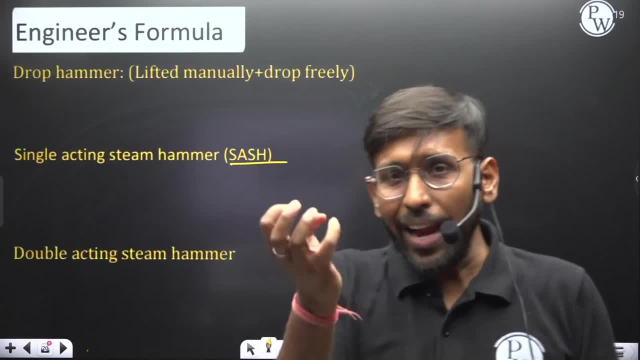 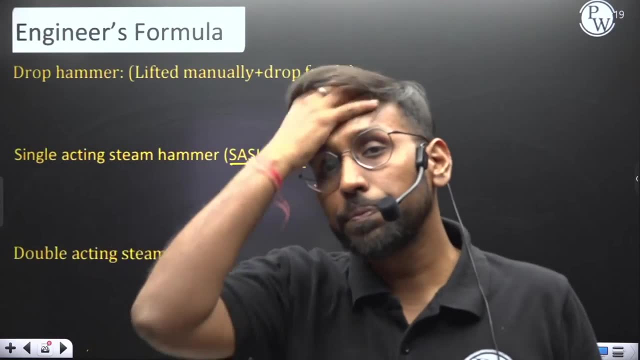 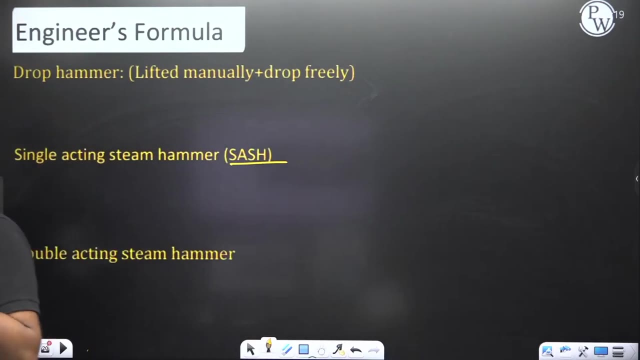 double acting steam hammer. so what will happen to you? in single acting, steam is given andline and drop is free, gonna happen double acting. what will happen in case of double acting steam hammer? what will happen in case of acting stream? ever below, below, below, below, below, below. very good double. 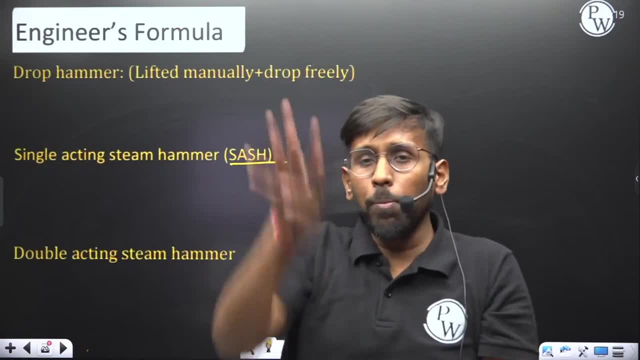 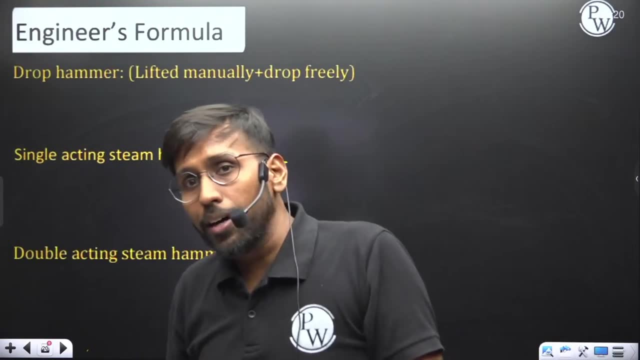 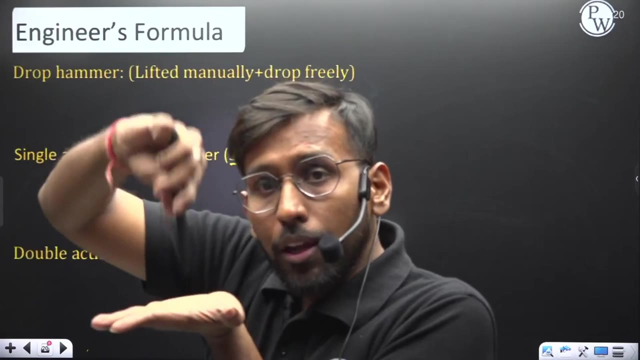 acting yoga. rise we fall, be with the help of stream. rise we fall, be with the help of stream, but the fall karega. so chka dekha na yaha pe the soft, the fall karega. so kya extra load lag raha hoga. the W a jo hammer ka. 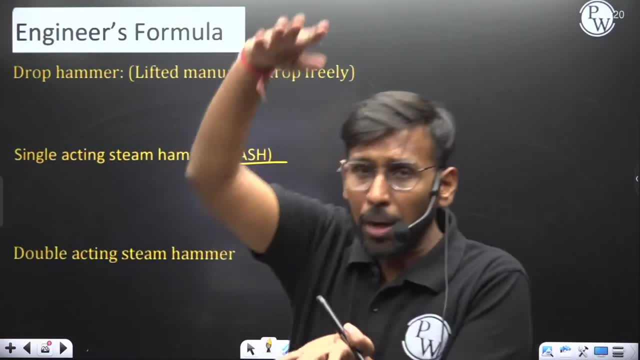 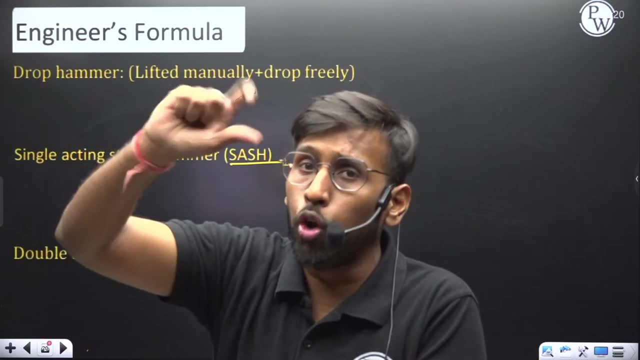 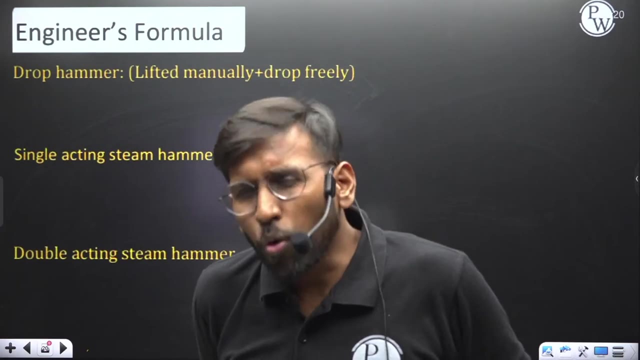 beta both a lucky raha hoga. lakin job stream ke madat se niche raha hoga. topkul acta reiki, aapka extra pressure, extra load raha hoga. bolu, bolu, bolu, bolu, bolu. concept sr rattooth hota nahi hai kuch. 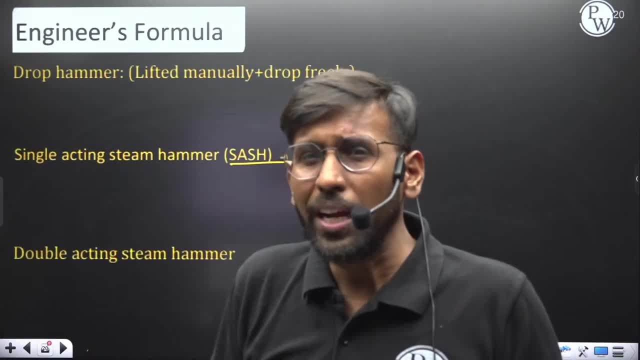 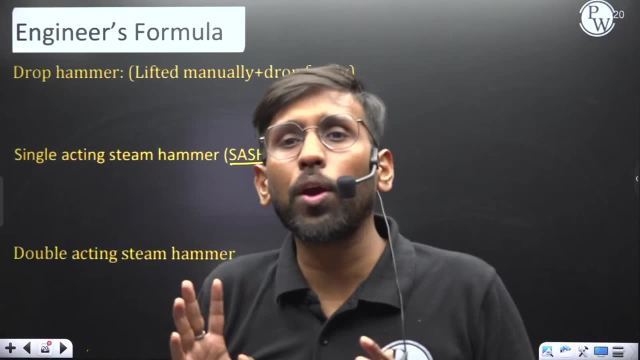 yaha pe sab concept hai. ab mai bolu, yeh sab gate mein nahi pushega, lekin sir, humko pata hona chahiye kya hai. nahi, toh kuch nahi hoga. ab formula yadi nahi ratpa hoga. 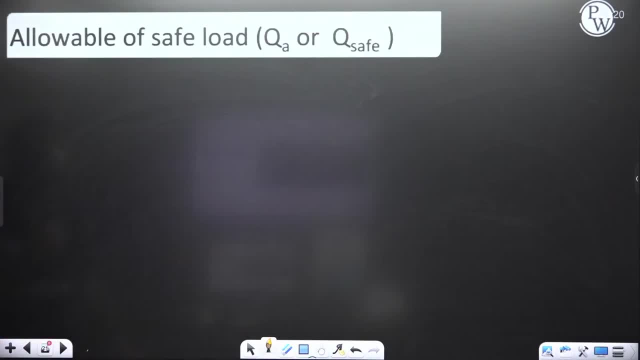 dekha hai. dekho ab yaha pe. so, sir, allowable load and safe load samjhoga yaha pe dhyan se ok. so agar hai baat kar rahe hai q safe, this we write as q ultimate upon factor of safety. isko kya likh rahe hai. 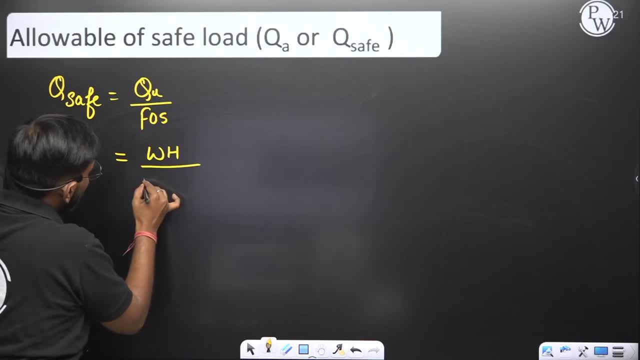 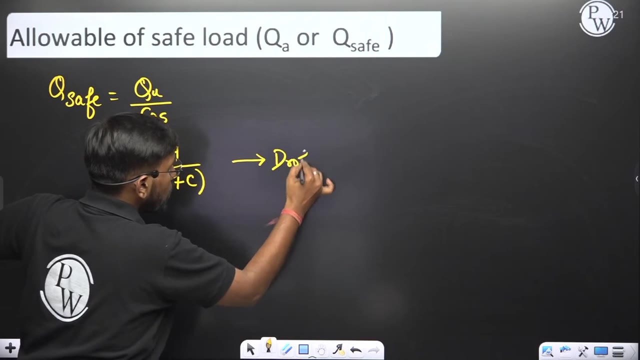 w h upon factor of safety into s plus c. yeh jo formula hai. yeh aara hai for double acting steam hammer, sorry for drop hammer, drop hammer. and single acting steam hammer, theek hai, aur dusra hai mere dosth. and single acting steam hammer, theek hai, aur dusra hai mere dosth. 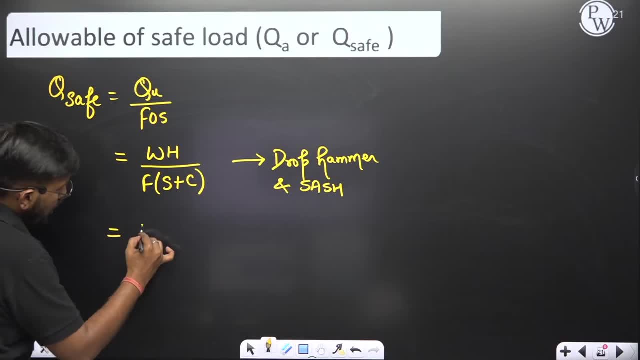 w plus main abhi bola na ki bhaiya jo pressure lag raha hai. uske karan badh jaega, so jo piston hai, that is the pressure of the piston area of piston h upon factor of safety into s plus c. this is in the case of double acting steam hammer. 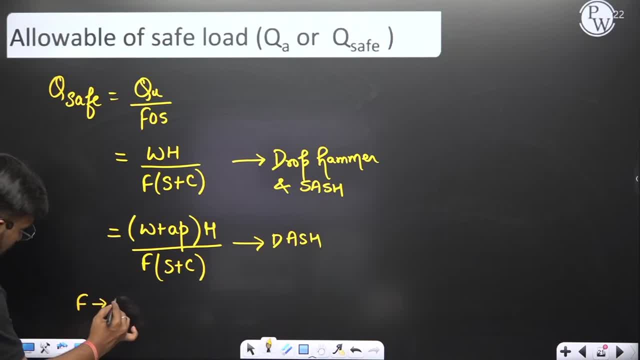 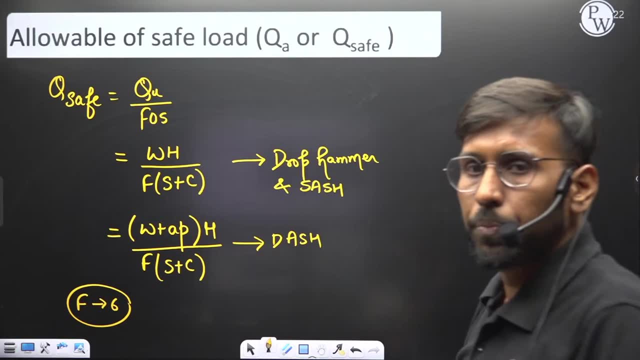 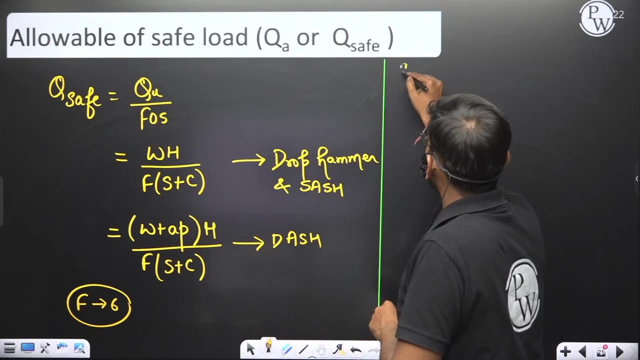 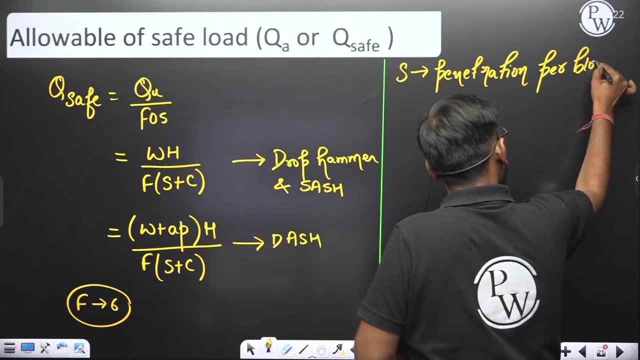 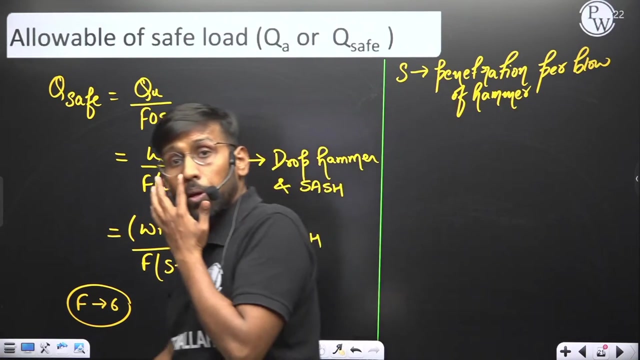 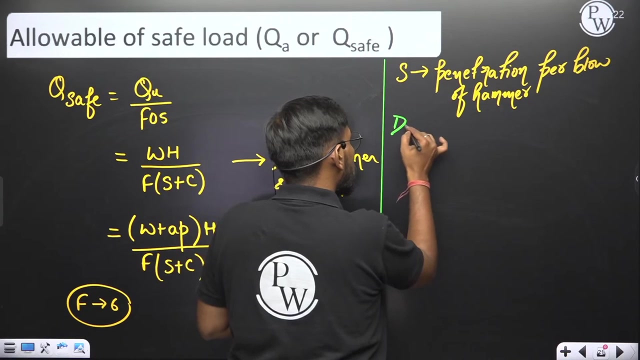 jaha pe factor of safety. kya aap lete ho generally 6 hota six. what is s? s refers to penetration. the pile penetrate karra a the penetration per blow-up hammer. for blow-up hammer, it's a penetration per blow-up hammer. he can have the penetration per blow-up hammer. so, agar aapke pass, drop hammer a if you. 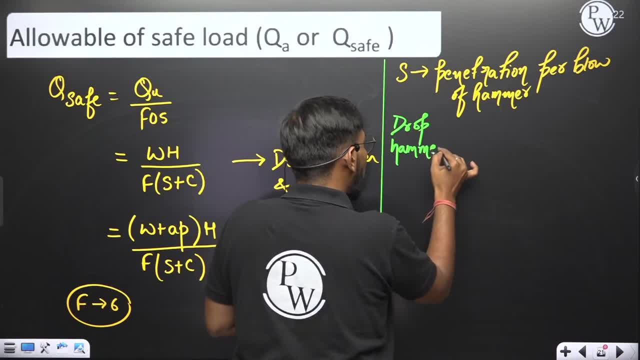 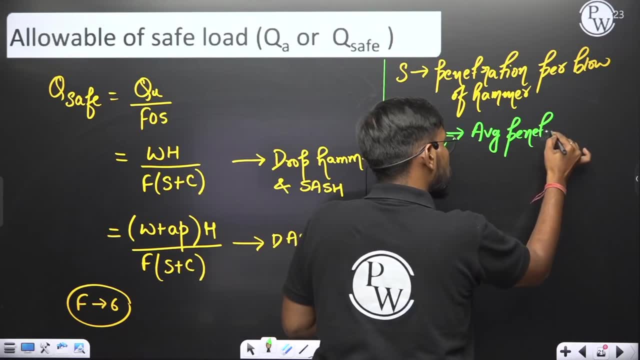 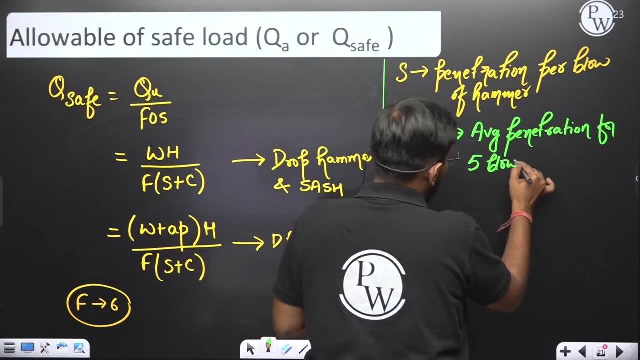 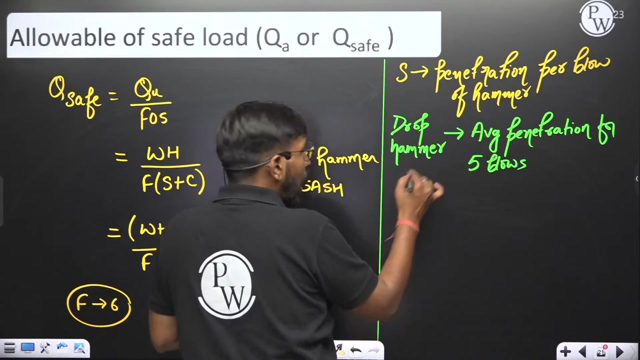 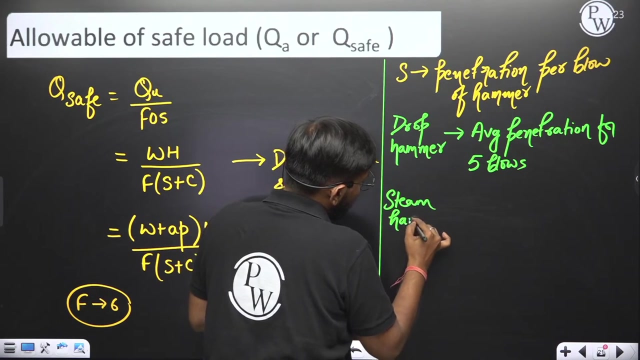 have drop hammer. in the case of the drop hammer, we take the average penetration for five blows. for five blows, average penetration. that is in the case of drop hammer. that is in the case of drop hammer. next, we are talking about seam hammer, whether single or double seam hammer. 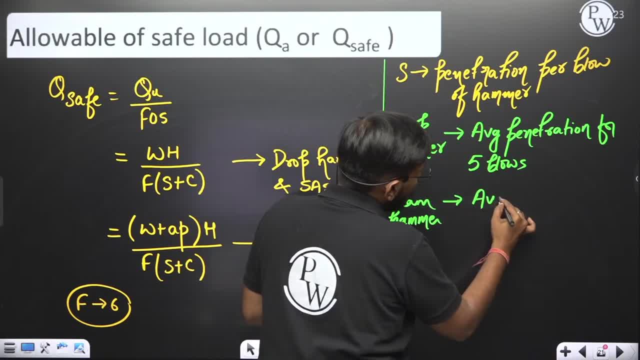 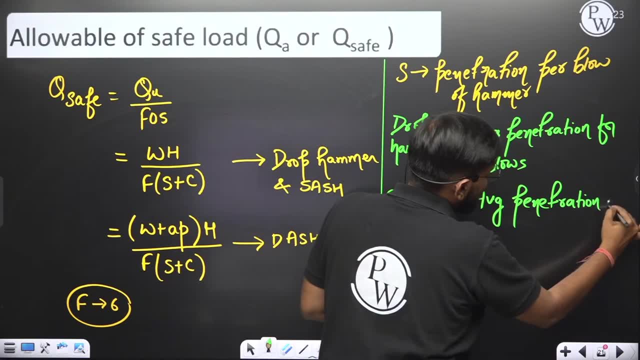 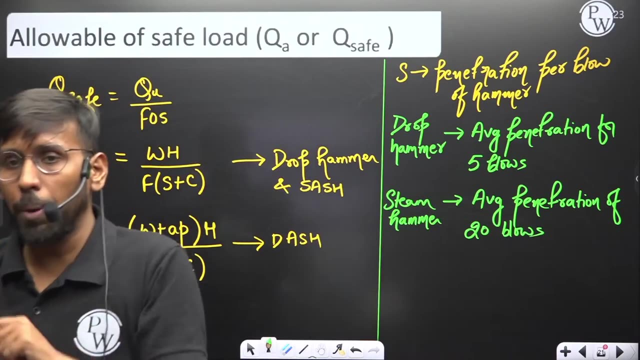 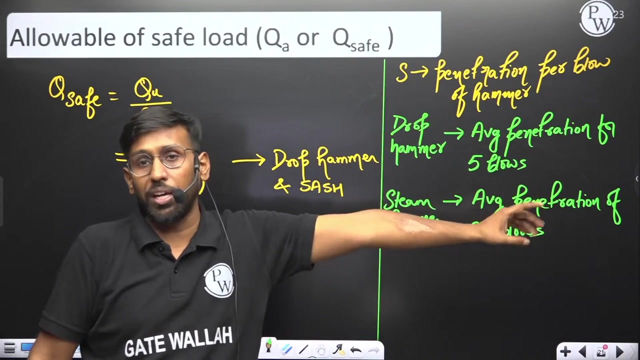 here we will take average penetration of average penetration of twenty blows. average of twenty blows. twenty blows, average penetration of twenty blows. ok, if we take twenty blows, then per blow set we will take the average and then we will tell. in the case of the seam hammer, next is C. 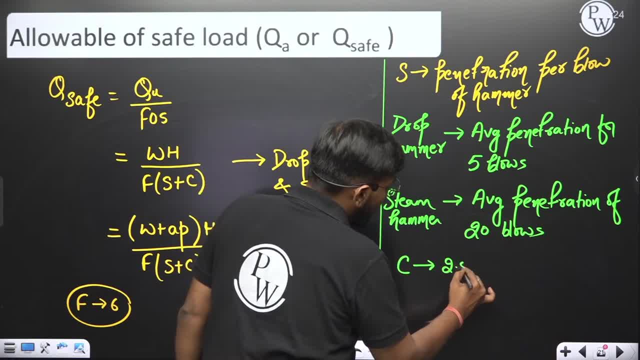 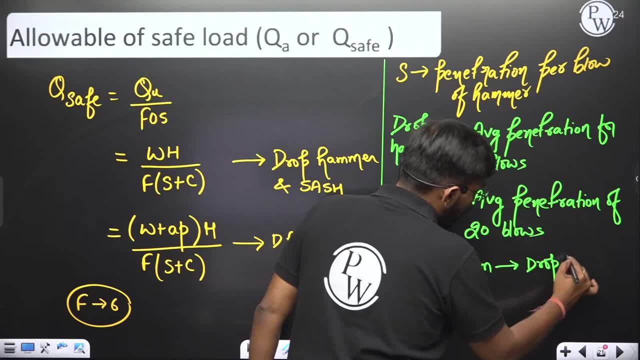 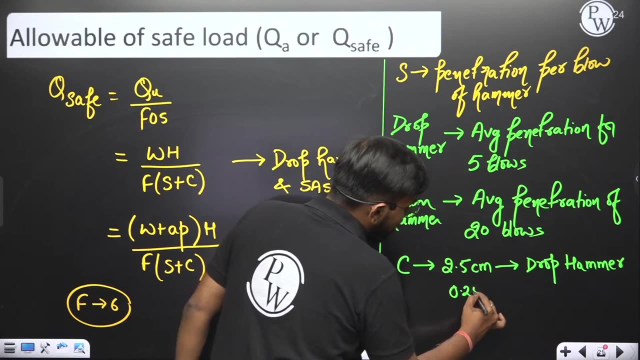 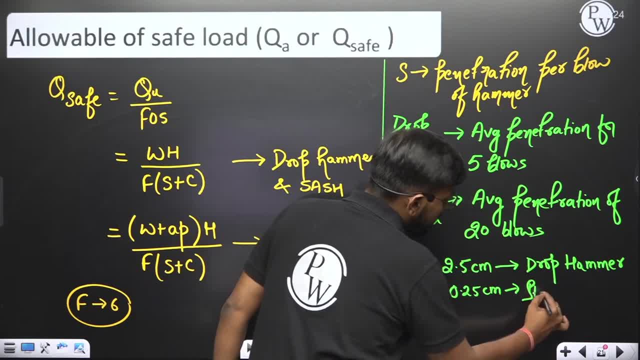 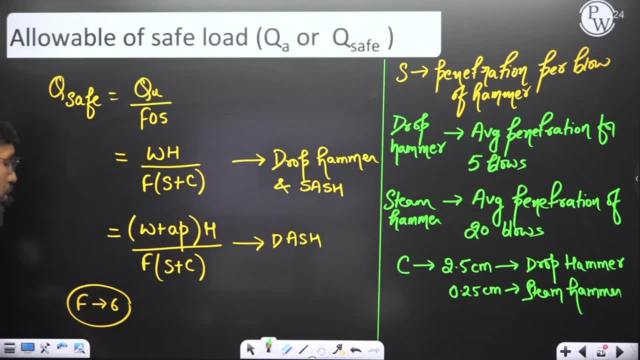 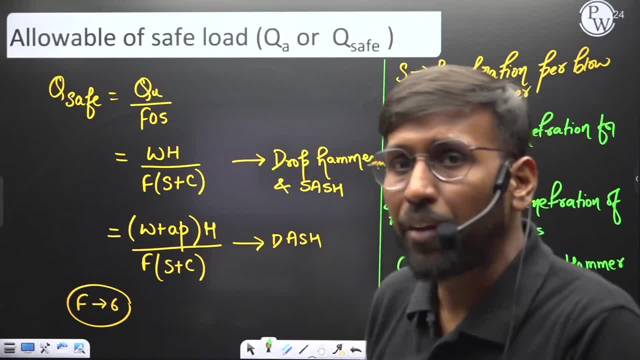 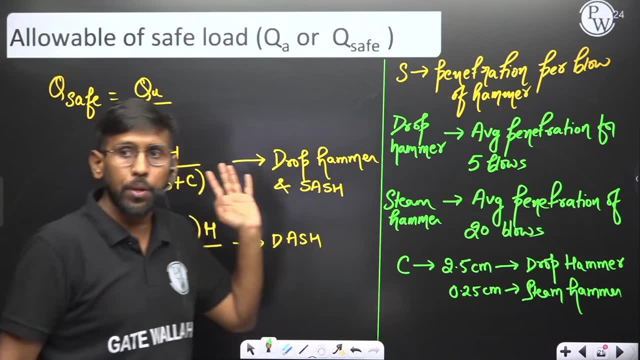 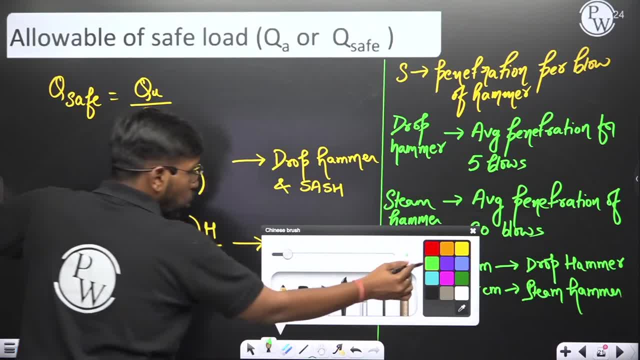 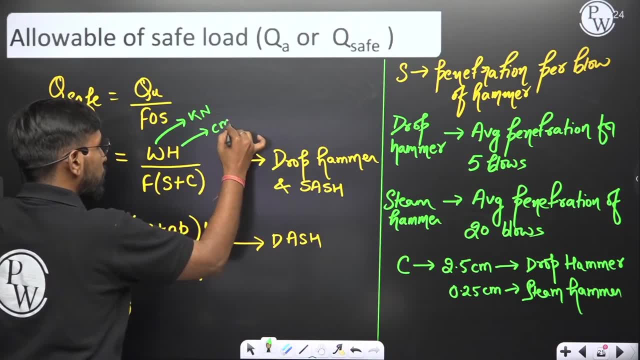 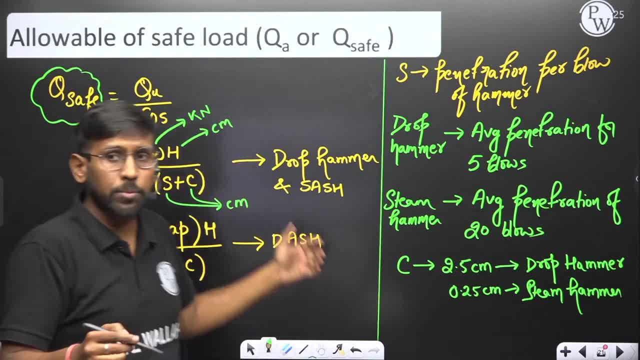 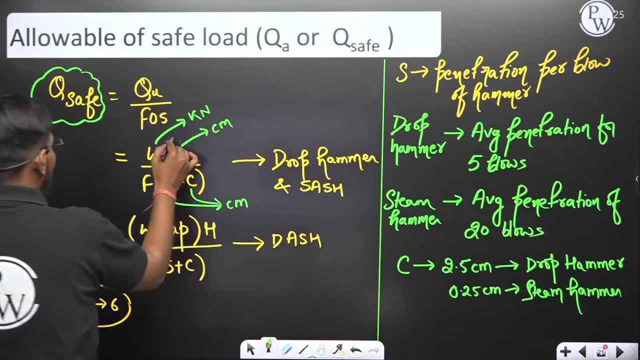 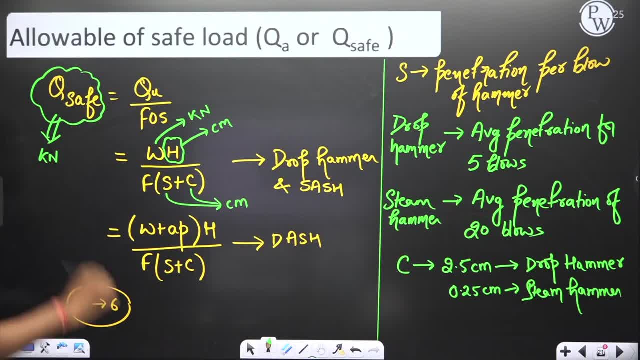 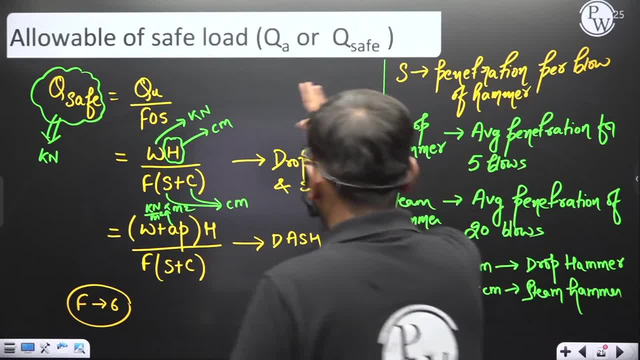 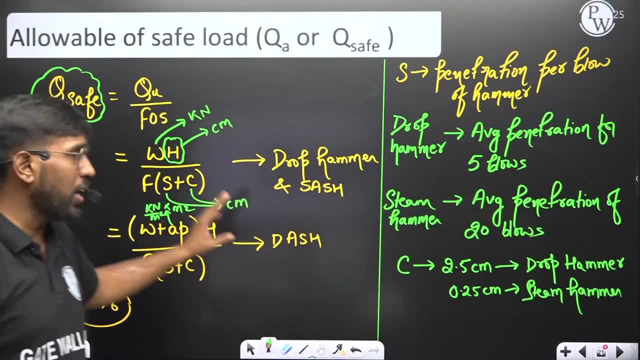 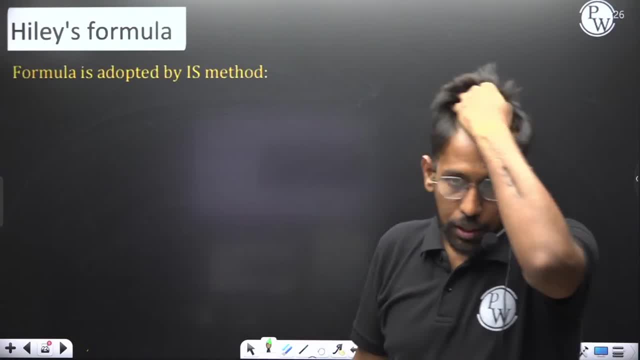 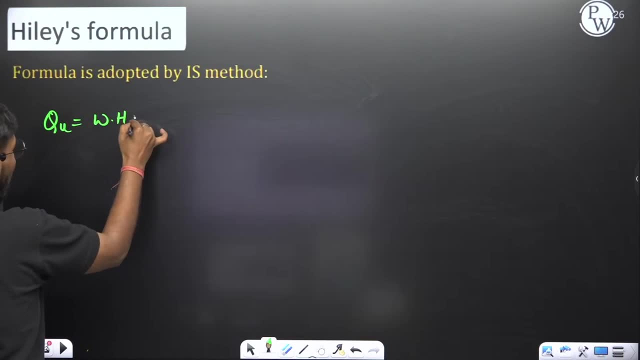 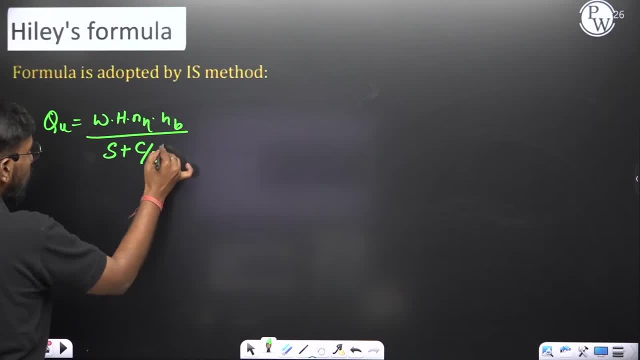 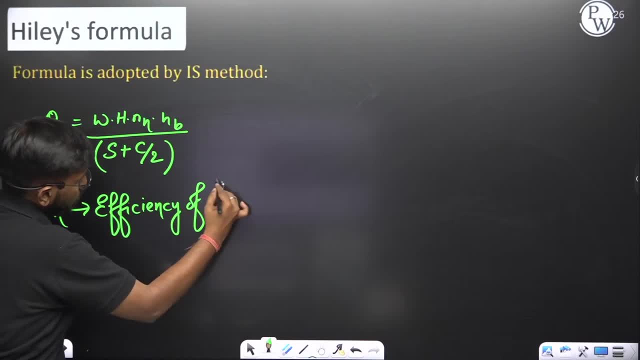 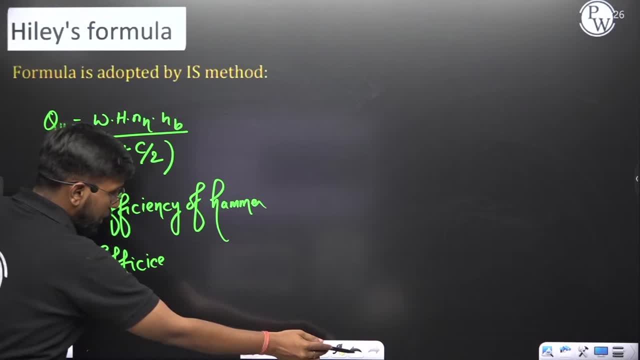 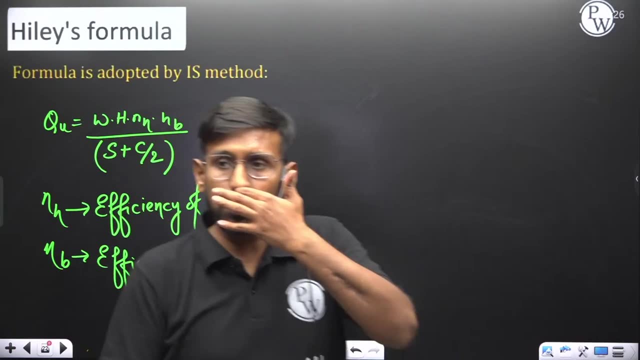 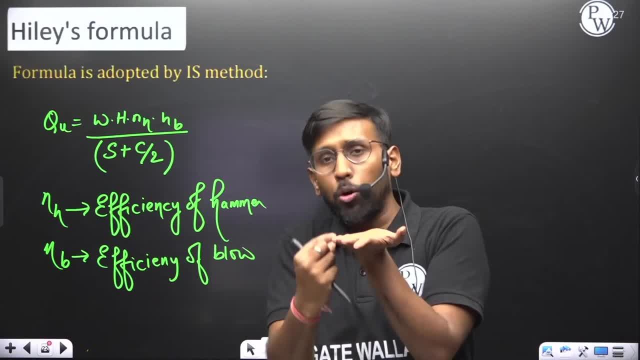 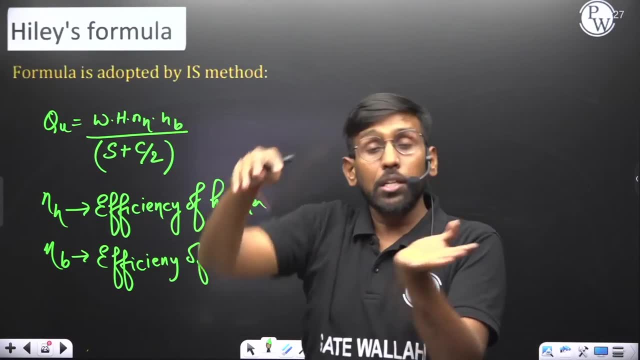 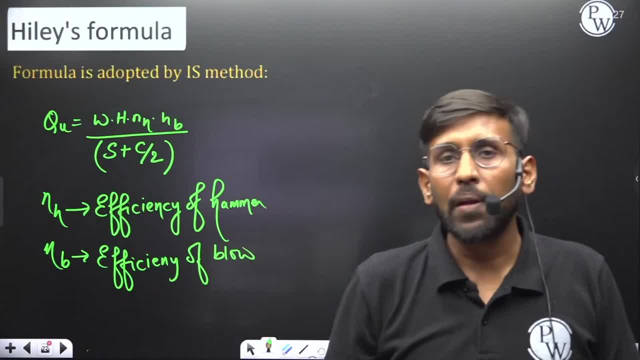 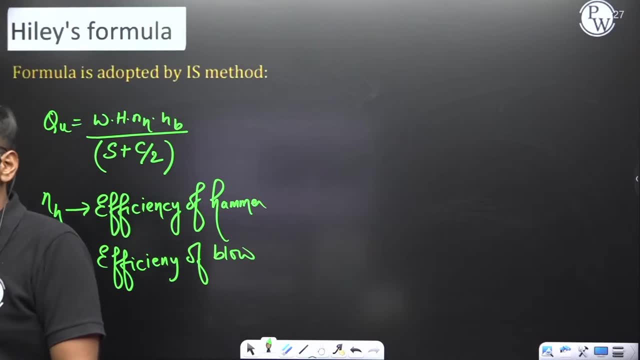 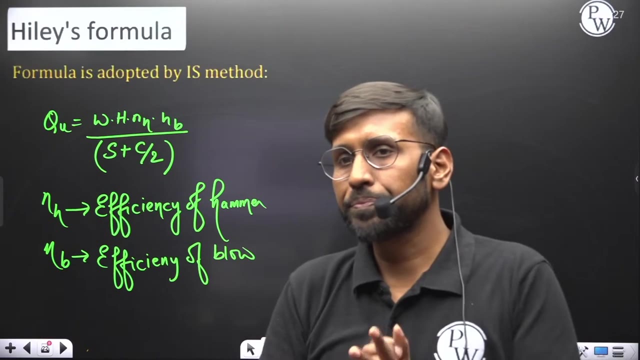 but this is in the case of Healey's formula. this is in the case of Healey's formula right, right, shallow good. this is in the case of Healey's formula. good, sir, Bob, video, right, so direct the wall at a mere dose. yahaan say I'm. look, ask a glass, a wind-up. 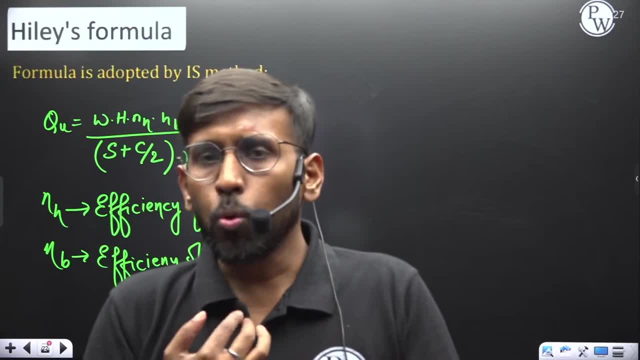 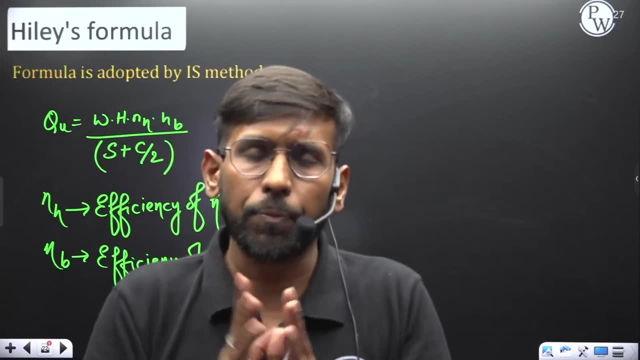 carousel is an a he up. got your field method a whose capella I'm go coach numerical: can I on numerical miracle time, then I above car yahaan. second theory: Bob Caruso theories roughly one hour and numerical- a one-hour, one-hour theory, one-hour numerical. cut them over, it's not any. 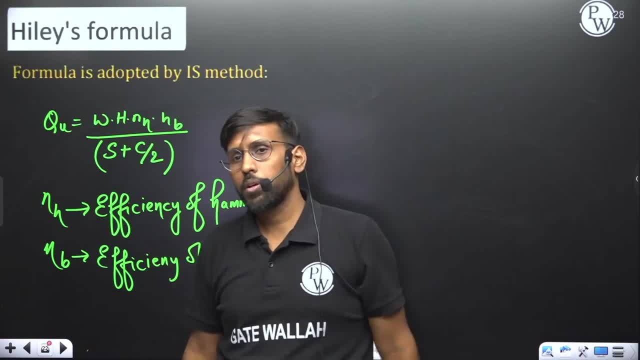 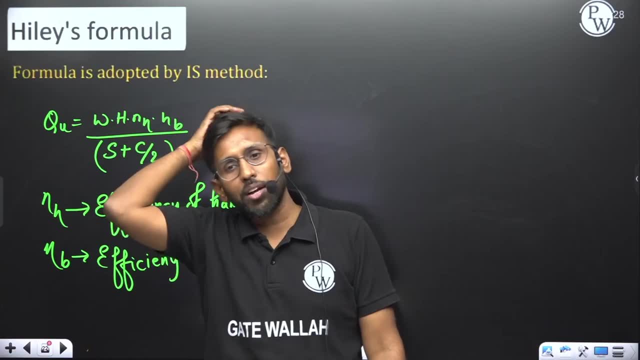 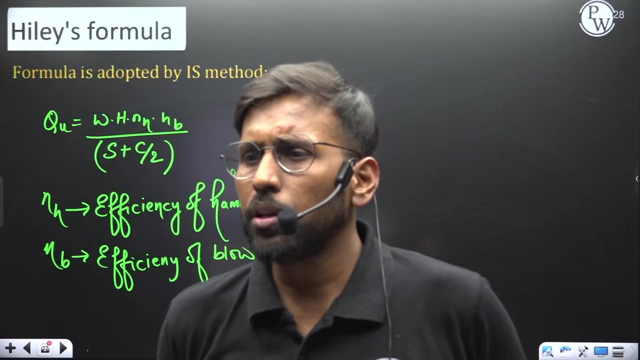 partner. one-hour theory, one-hour numerical over. we'll delete tomorrow, we'll call completely tomorrow. he can't Bolega to circle up. kakri class a casa feeling our a calabco geotech. kakri class a tera me, tera hora cesafiling a re Elle adult in one question up ABS Blanket, padme doubt. 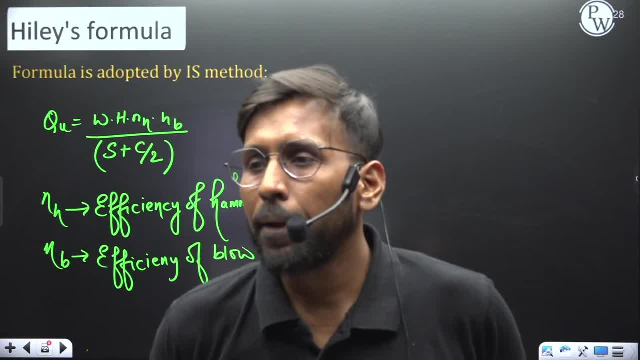 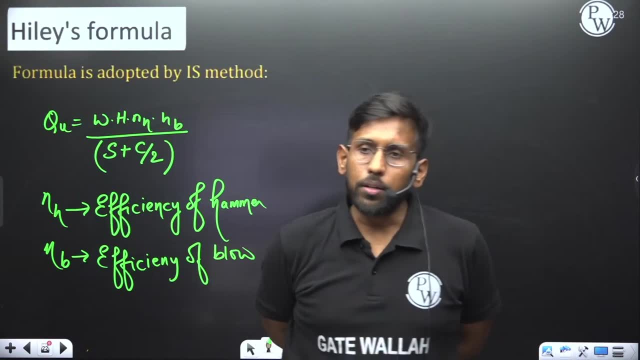 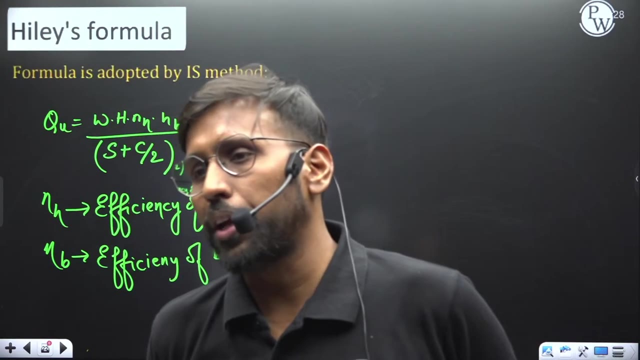 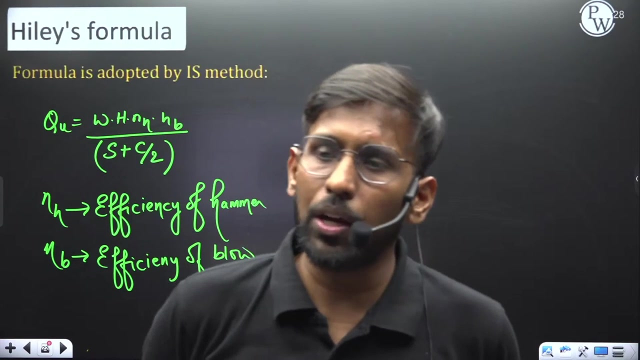 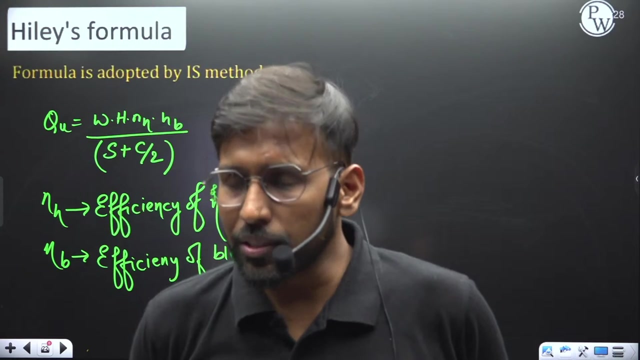 Paul: Ojo, yeah, Bphone Lotto tna re brawling. okay, wife lander the and and going to practice more questions and they, we are going to practice more questions. 630, kind for my day. let out a bar, my bar big, let out a bit, but at all. 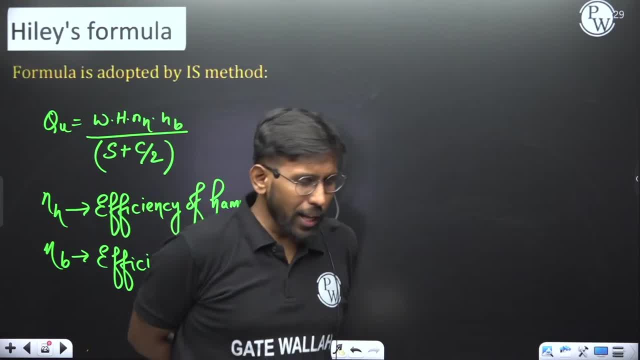 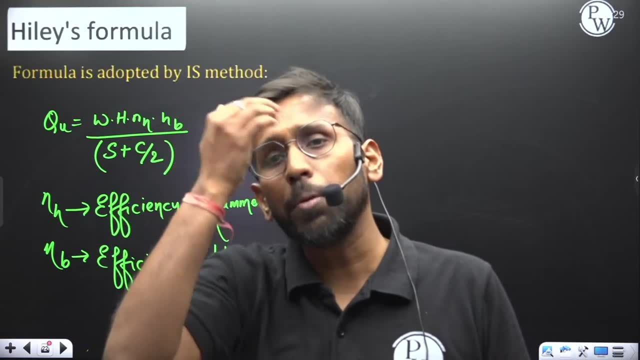 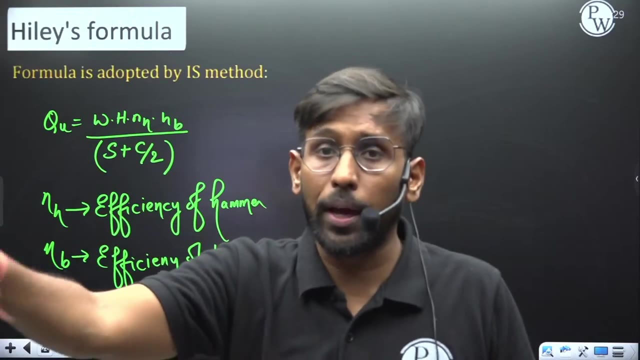 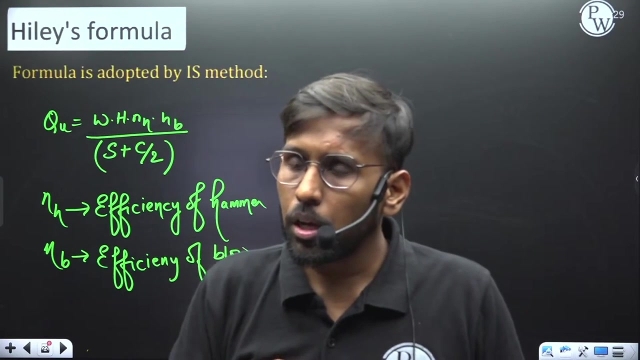 630, Mary Kelsey was Lord pay. but I do the engineering mechanic, true, or I fix 30, base, a target. say engineering mechanic, true, or a hair or a seed in Mary's Lord pay up car structural analysis, Shura. engineering mechanics by Ashwarya sir. structural analysis by Gotham Gupta, sir, okay. 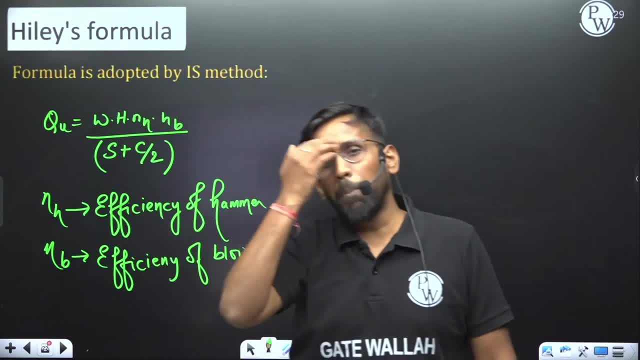 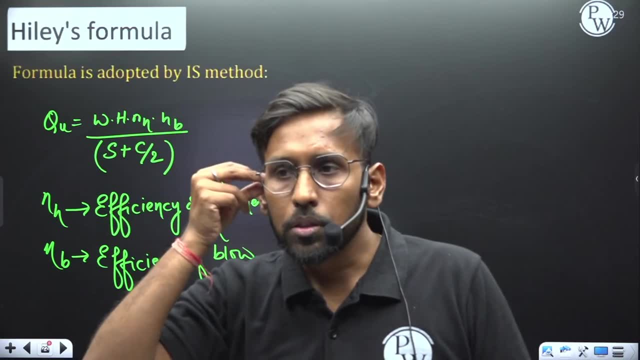 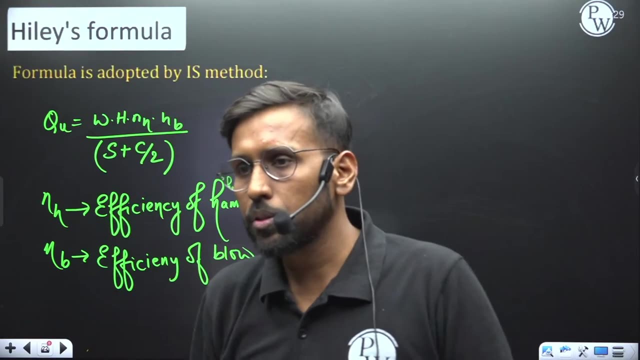 clear a point below below: below my mind: up cup Friday, a Saturday or Sunday. so nice, shoo-kana Chara, da is no Saturday cook here, okay. so from Monday these two subjects are starting. one is structure analysis, other is engineering mechanics. I'm a DPP, a DPP ke bugle me wabbe DPP, dekho na. 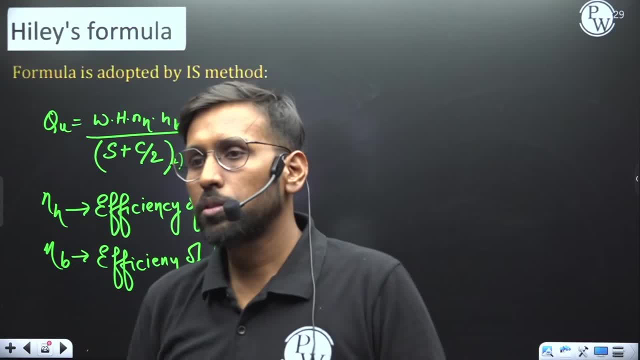 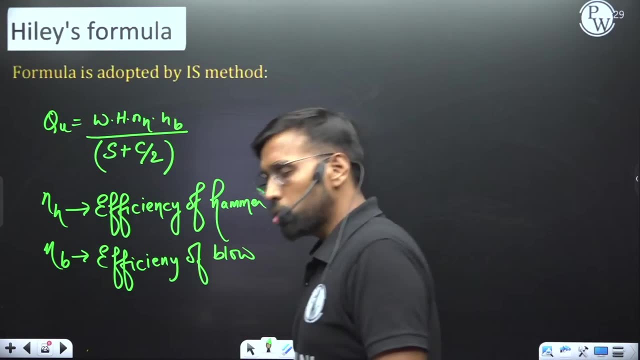 uske bugle me DPP PDF. deko mill jaega rankin slivers, honey part only a rankin up kase padoge hello Tom. abhi toh wa sir karato die som karan bhai. so I'm okay on you to say: 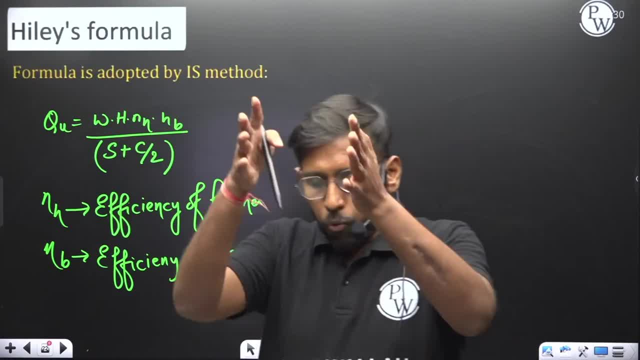 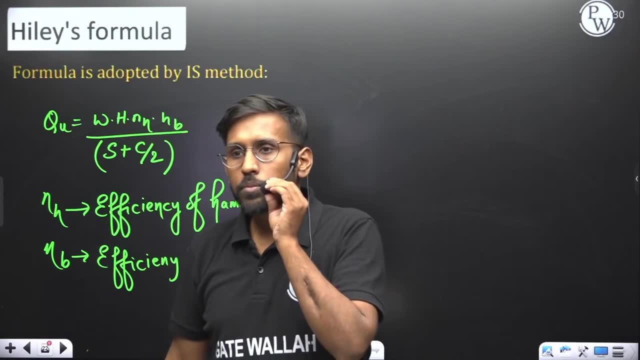 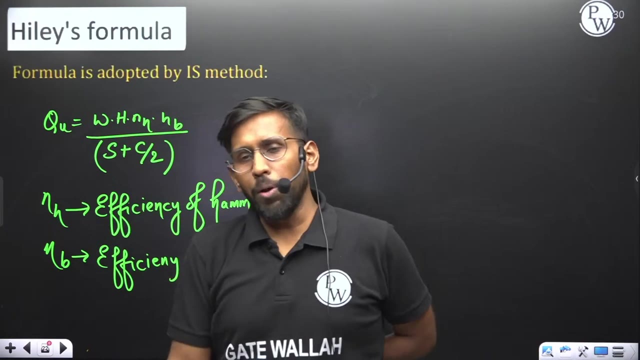 nekara diya hai. DPP session job ka. wo session hoga na Abhiyas ka usi ma che question uthake, mai kar dunga. I will be taking the Abhyas on Saturday, Sunday. Don't worry, Dhibijan Ka Kuch info de dije. 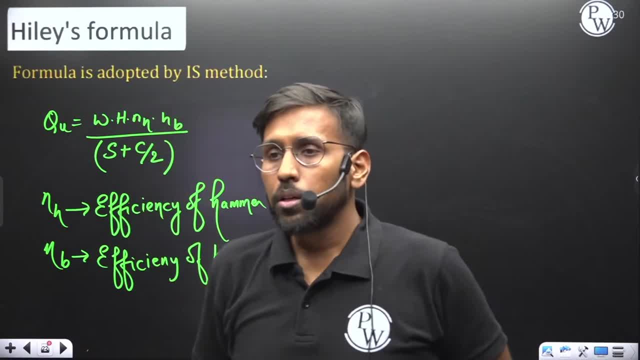 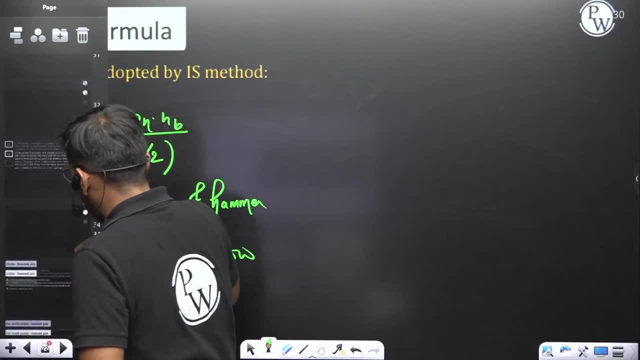 Chale tika. I will take a separate session on that. How to revise Tika. Toh Aaj ke liye apne yayi wind up karte hai. Aaj ke liye apne yayi wind up karte hain. 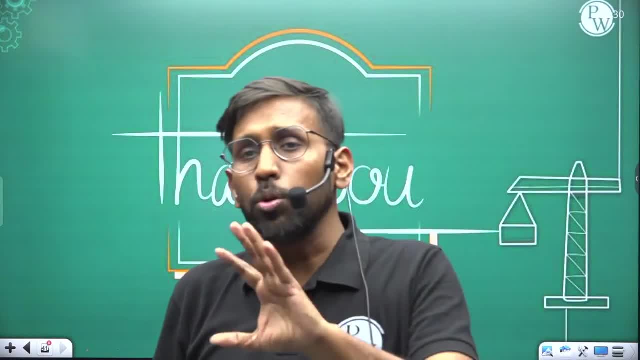 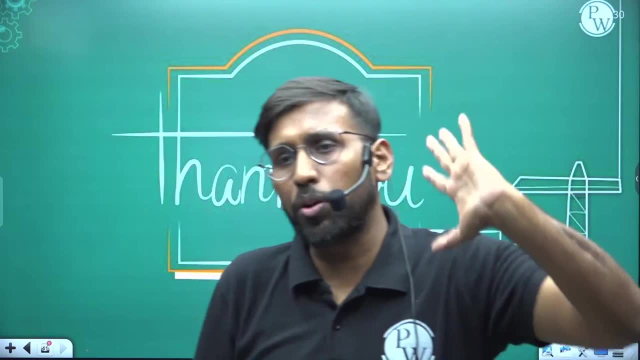 Abha Abhayas mein kebuna Chalo PYQ saara nahi lege. beta, jo important PYQ hai jahaan pe mujhe lagta hai, ki aapko problem ho sattie hai, wo saare PYQ lege. dekho abhyas mein kya, kya hoga, mai bata deta hu important. 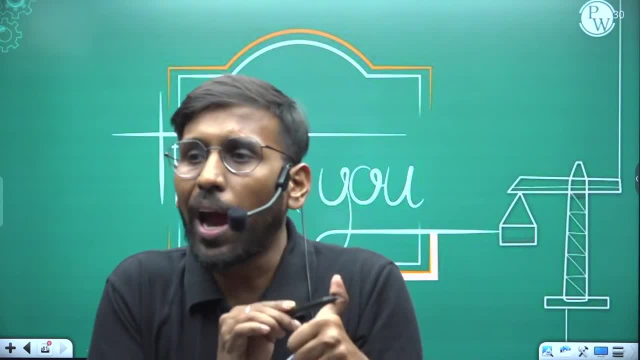 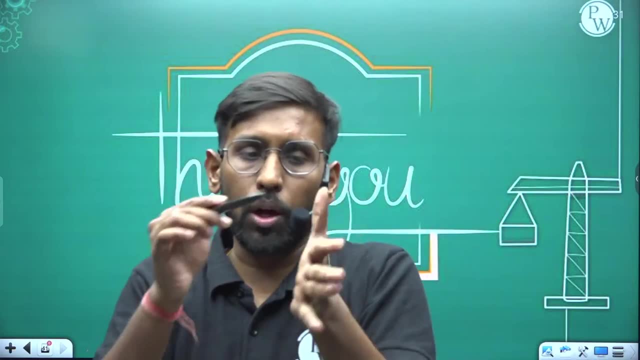 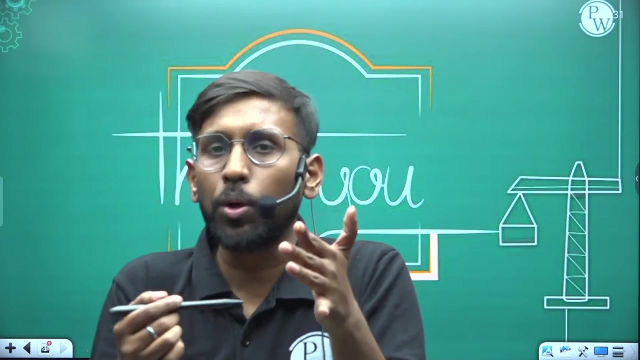 PYQ important DPP questions and some new questions. ye tino mai abhyas mein cover karunga. important PYQ important DPP questions. important, your new questions, jo mujhe lagta hai ki zaruri hai karana, wo mai karadunga thik hai. baaki aap tension mat, lo jaisa aap bole. 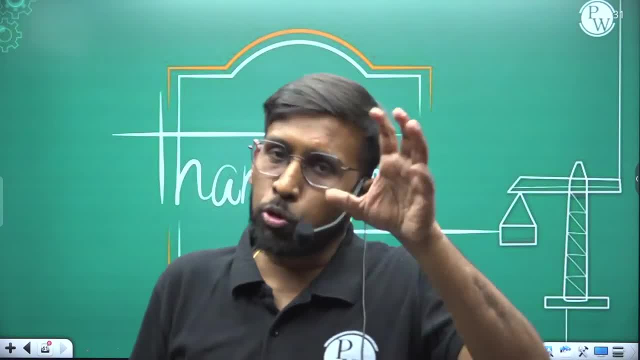 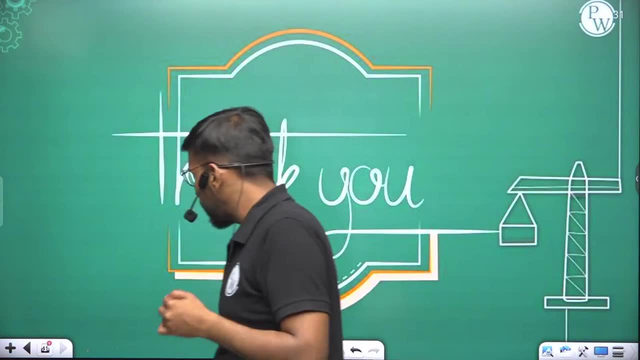 ki sir, shallow foundation mein 3-4 question nahi bane. mujhe pata hai kaun nahi bane hongi to karvaunga. thik hai idam bata denge, thik hai chalo. so thank you so much. bye, bye.